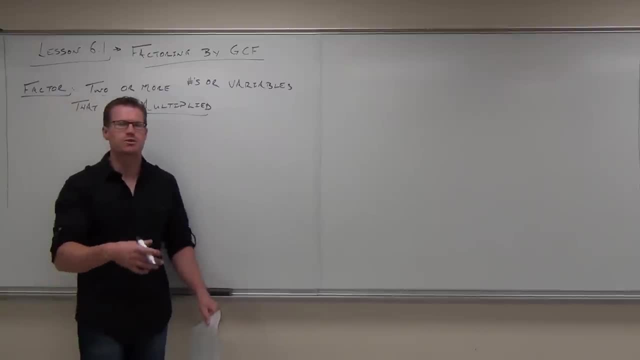 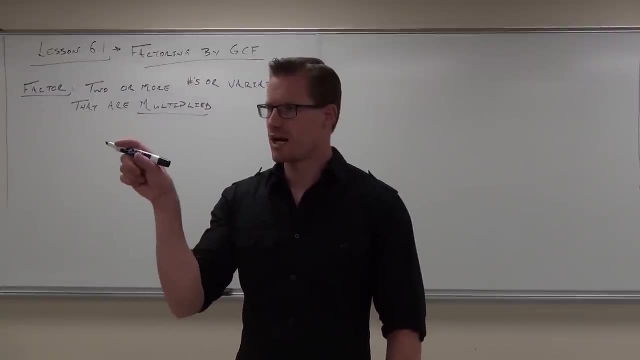 We're talking about the multiplication idea, And the reason why we're talking about that is because when we factor, we're really talking about dividing. You remember this word called distribution. yes, Remember, distribution is the idea of multiplying and you get rid of parentheses. 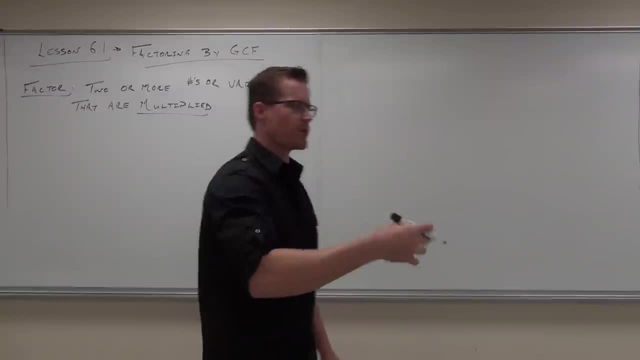 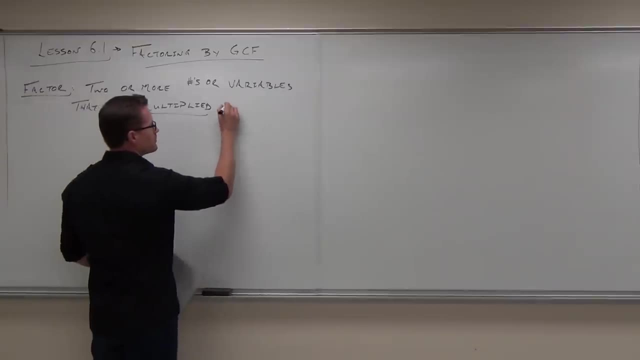 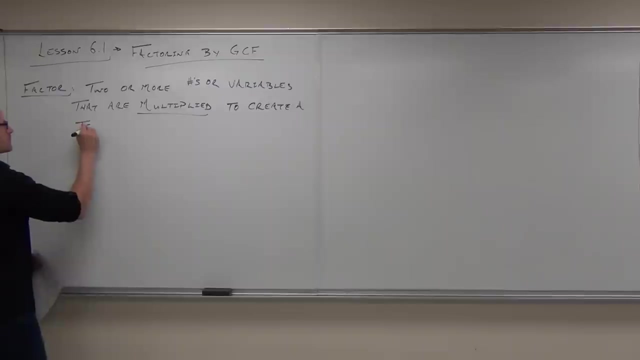 Factoring is the opposite idea. It's dividing to create parentheses. We'll talk about that later. So two or more numbers Or variables that are multiplied to create a term. That's a really long-winded way to explain something that, with an example, I think is going to be really clear. 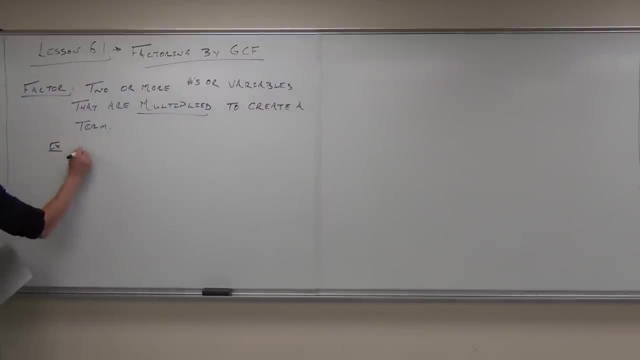 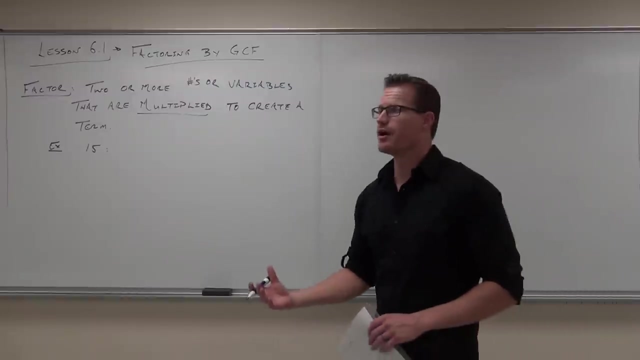 Let's do just a couple very quick examples here, For instance 15.. Number 15 is a composite number. It's not a prime, which means it has some factors in there. Can you give me a factor of 15? 3!. 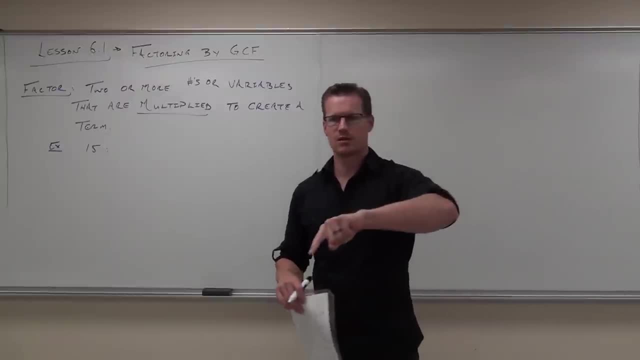 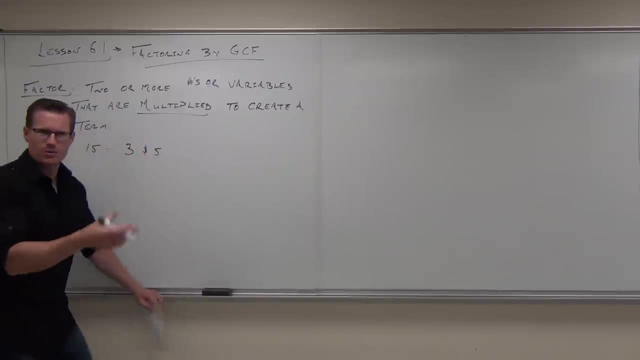 3,. OK. now, factors always come in pairs, So if you give me 3, you also give me. Ah, That's right. So 3 and 5 are two factors that multiply together to create 15.. Are you all right with the idea of factors? I'm not going to spend a lot more time on this, but 3 and 5 are just two examples of factors of 15.. 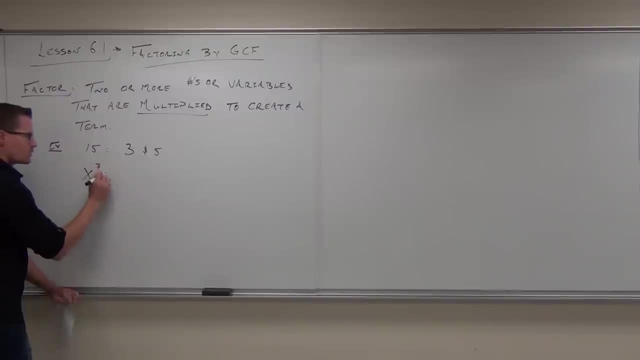 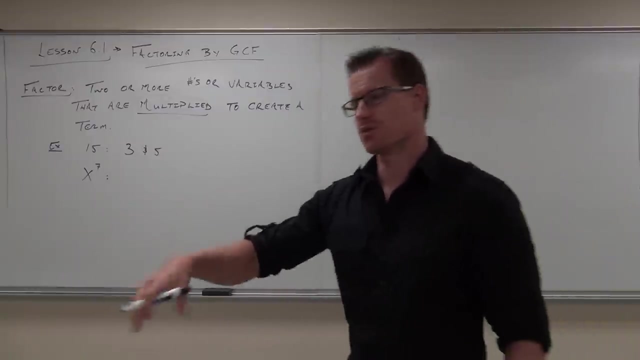 Now, what some people get a little confused on is how in the world do we do this with? can we do it with variables? Well, the idea is: anytime you can take two quantities, whether they be numbers or variables. Well, the idea is: anytime you can take two quantities, whether they be numbers or variables. 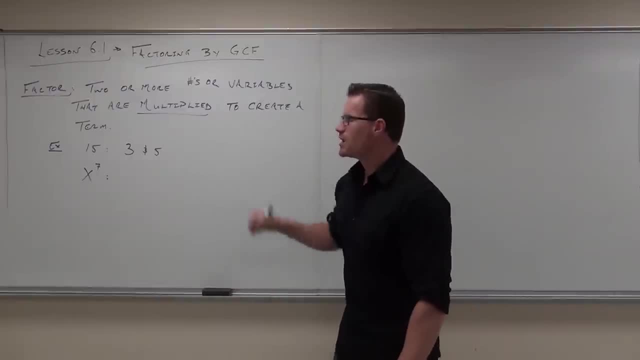 variables and multiply them together: well, those things are factors. So let me give you for instance here, and you'll give me another one: X to the 7th. you all know how to pronounce it. yeah, Say that for me. 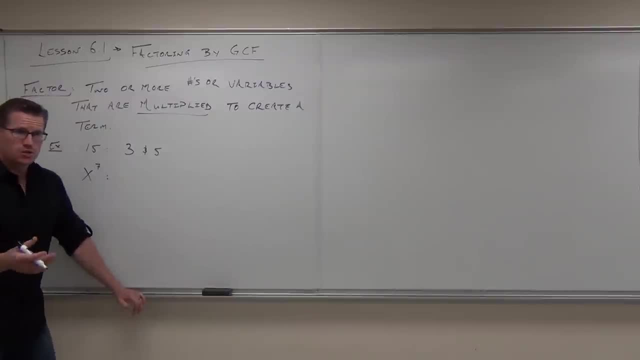 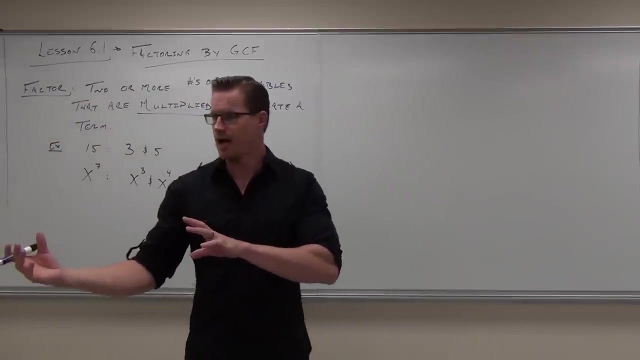 X to the 7th. Perfect, If I can find two quantities, so two variables raised to another power, that when I multiply them together they make X to the 7th. then I've found two factors. For instance, are you aware that X to the 3rd times, X to the 4th, X to the 3rd times? 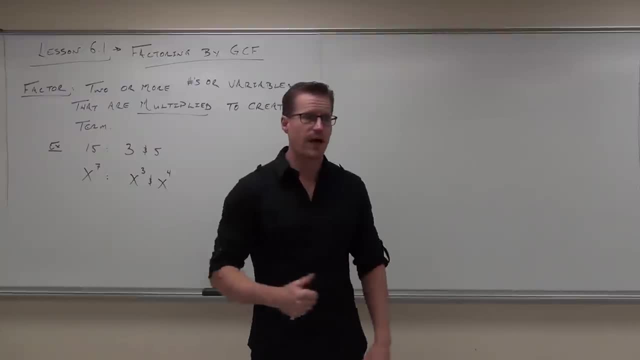 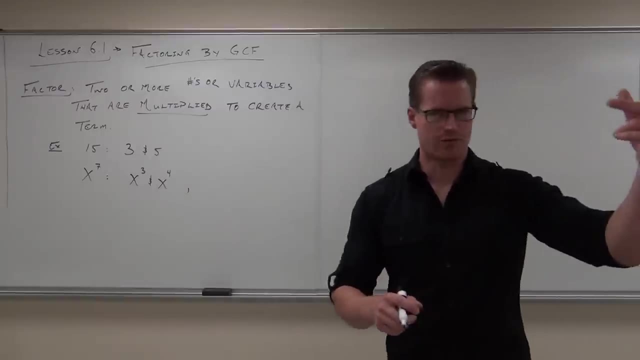 X to the 4th gives you X to the 7th. Are you aware of that one? Then those are two factors of X to the 7th. I want you to give me another one. So give me two sets of two variables: X to whatever power you can think of. that would. 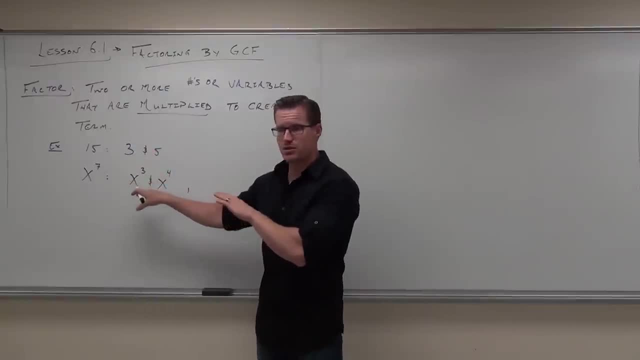 also make up X to the 7th, Because I haven't given you two, but there's several examples we could do. Give me another one: X squared, X squared- okay, X squared. and X Triangle To the 5th. 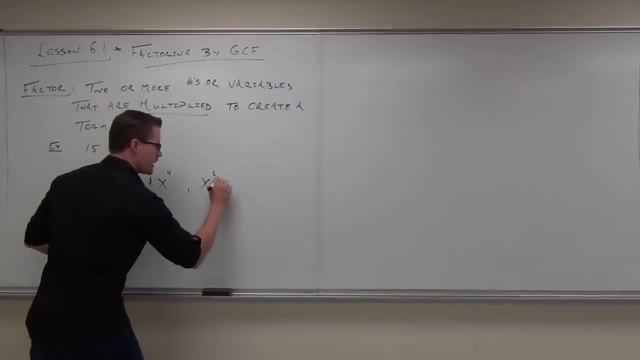 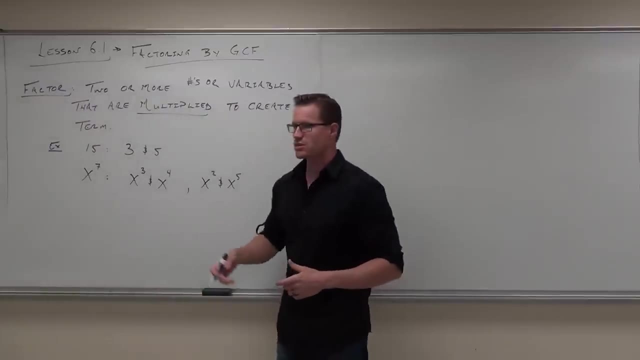 Sure, As long as X squared and X to the 5th multiply together to give me X to the 7th, then those are two different factors of X to the 7th. Show of hands, if you feel, okay with this so far. 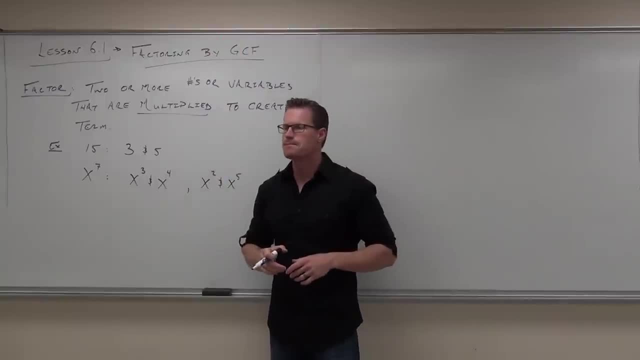 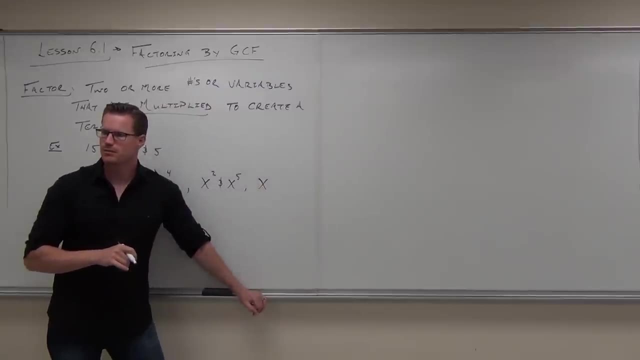 Left side people. are we okay with that so far? How about? let me do more and more? How about? if I give X, what would the other factor have to be X to the 1st? Okay, Perfect, Because this counts as X to the 1st power. 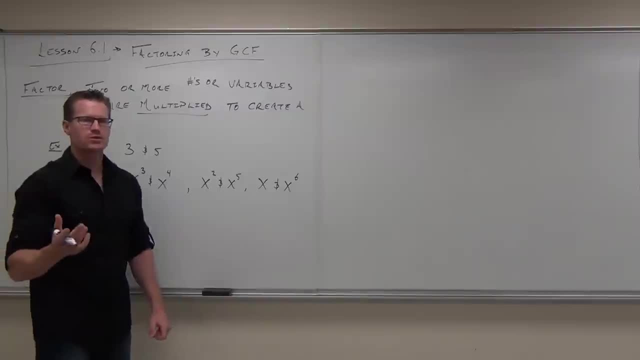 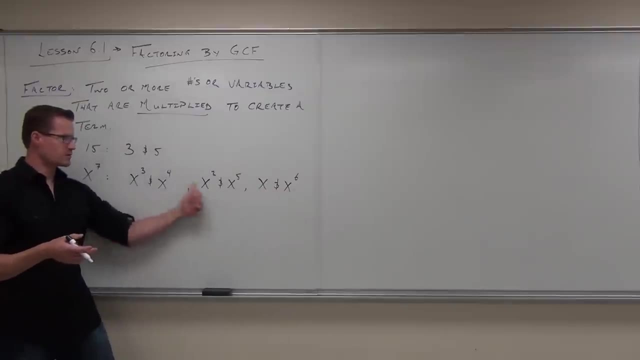 So if I have X and X to the 1st, Well, you know what's interesting is, when we look at this, we have X, That's a factor X to the 6th of the fact, X to the 2nd, the 3rd, the 4th, the 5th. 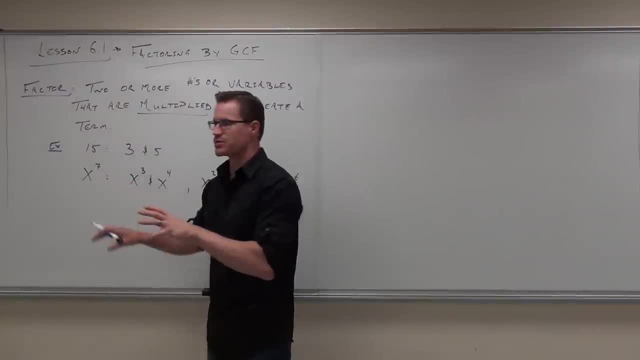 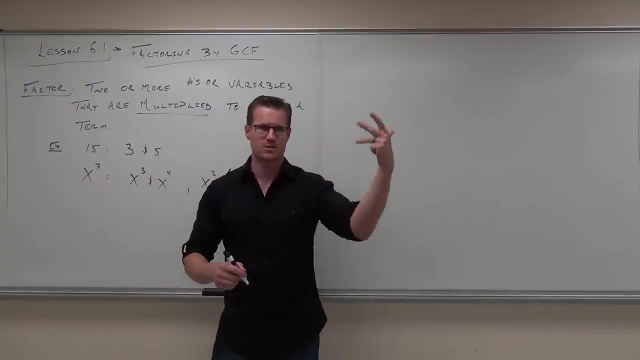 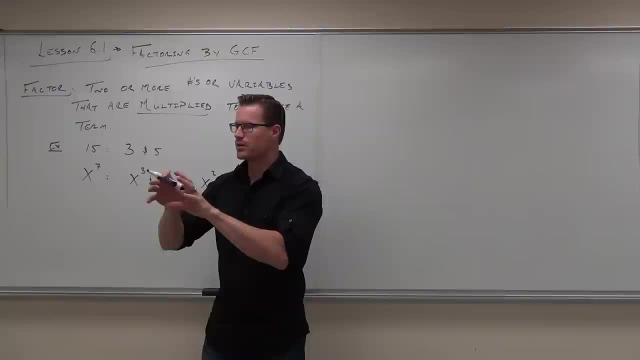 I think I have one too many X's there. We can always break off those X to the 2nd times, X to the 5th. Those are inherently factors. Am I getting through to you guys on this one? Yeah, Okay. 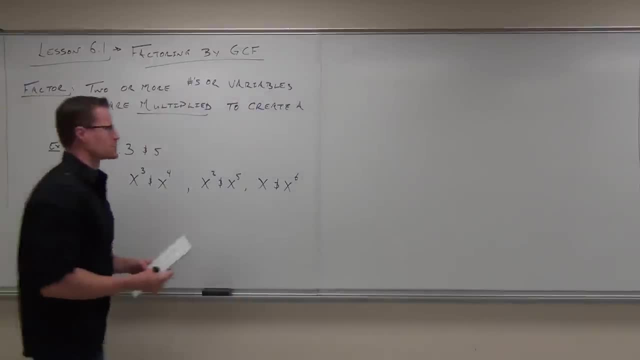 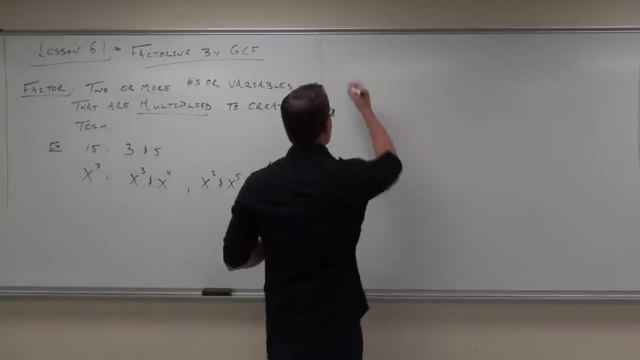 It's going to be important for our next thing Now: common factors. So we've got factors, Now we're going to talk about common factors and, after that, greatest common factors and how to use them. So what does it mean to be a common factor? 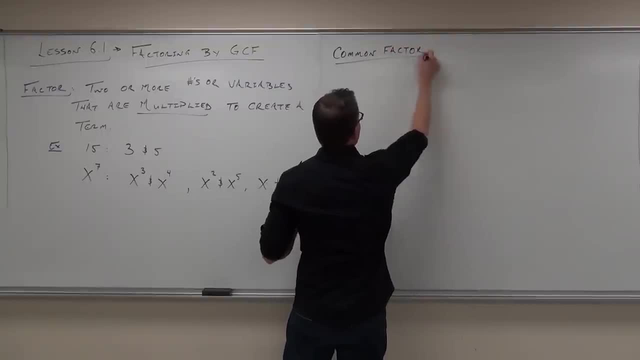 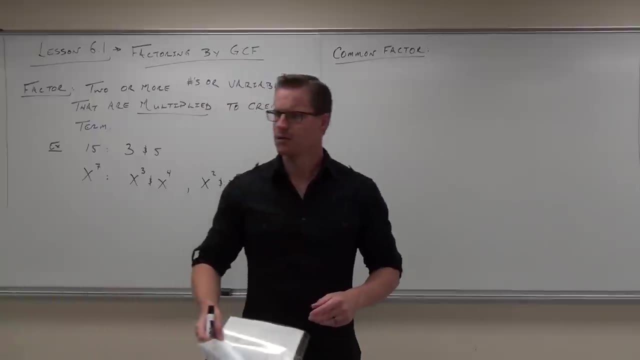 When I say the word common to you, what's that mean in just in English? What's something common, Something they have similar? to Say, what Something they have similar to Something they have similar, Sure, Something they have shared. Well, that's what it means here. 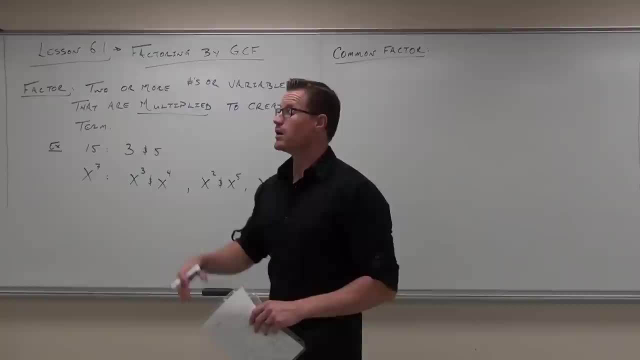 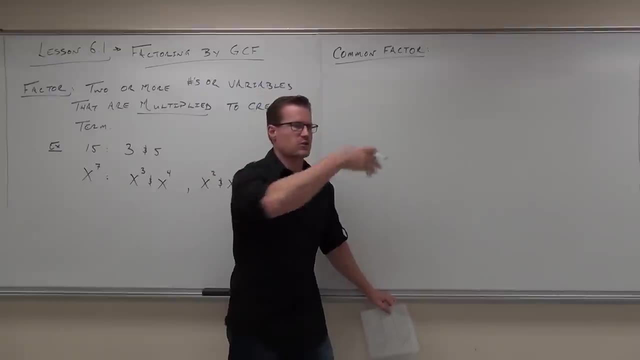 Common kind of means shared. So when we talk about common factors, we're talking about shared factors, And I'll give you an example. So if you want just a basic definition, instead of common factor, think of it like a shared factor. You can write that down. 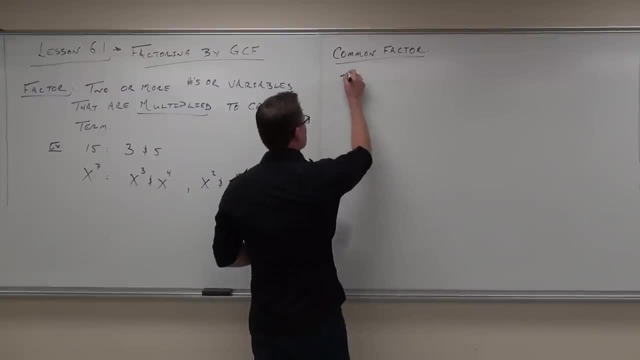 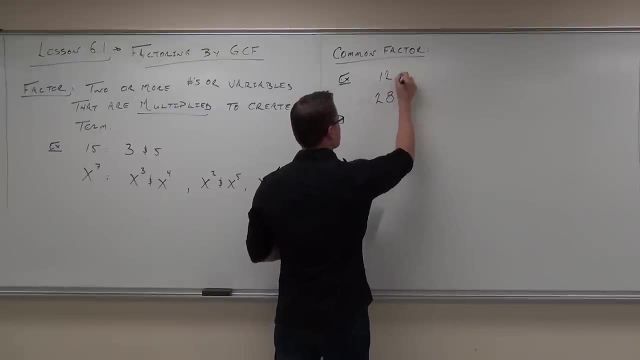 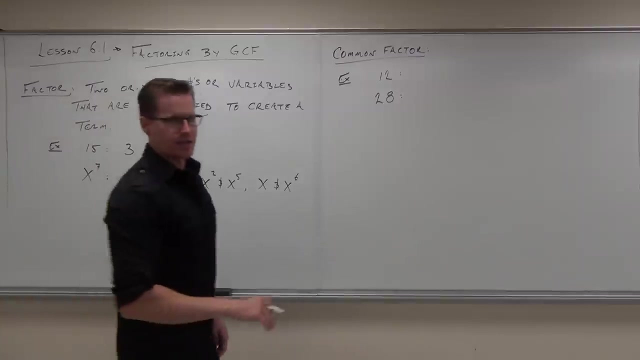 Common factors mean a shared factor. Let me give you an example. What we're going to do right here is we're going to list out all the factors that are common. We're going to list out all the factors that we can think of in 12 or 28,. so all the 12 and 28.. 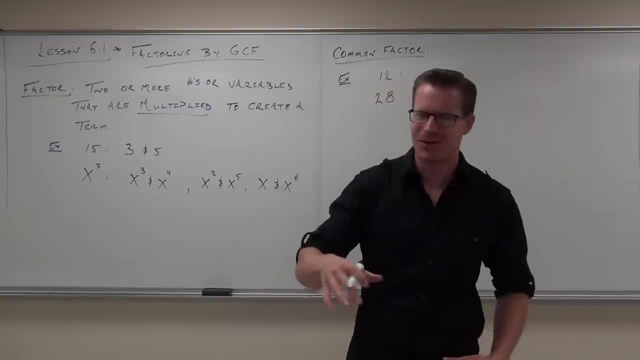 So all those previous classes you had, like math 80,, math 91, all that stuff where you learned about factors, well, we're going to use that right now, But when we get into the actual practice it's going to be much quicker for us. 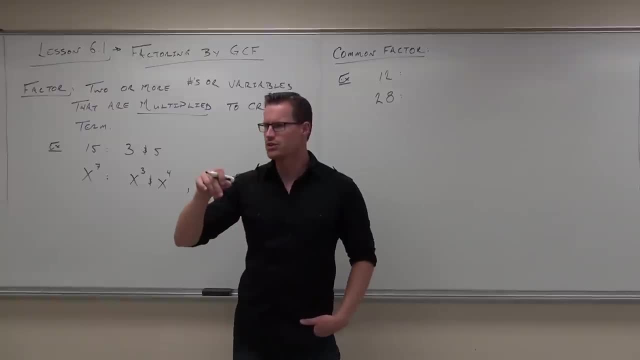 So right now we're going to list them. Let's give me some factors of 12, would you Two and four? Two and six? You know they always come in pairs. Do you know they always come in pairs? Unless you have a perfect square, like 25,, all your factors come in pairs. 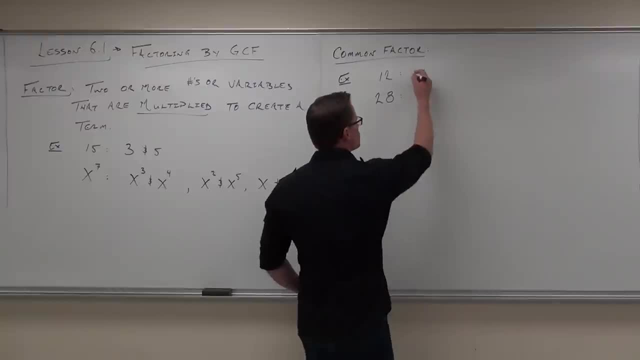 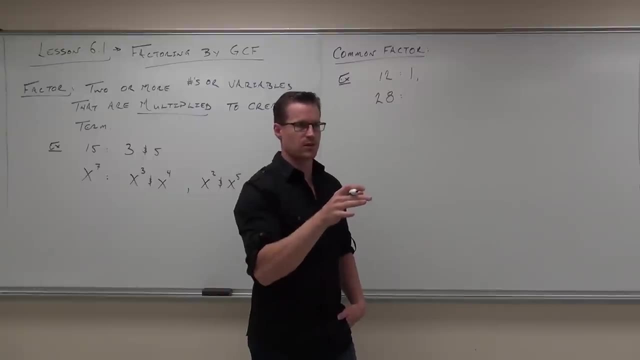 So typically what I'll tell students- if you've had me before, you know this- start with one. Is one a factor of 12?? One goes into any number, right? So one is always a factor. One times what would give you 12?? 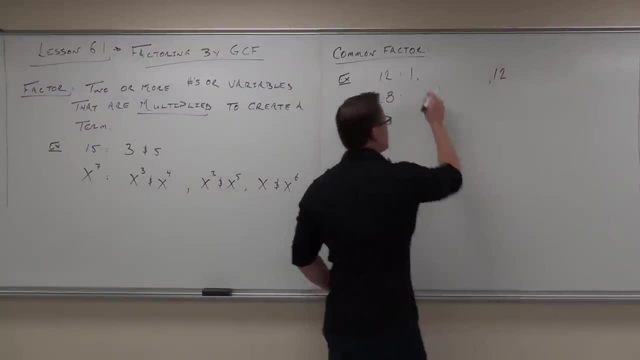 12.. Oh, there we go. So we got two factors already. Does two work? Is two a factor of 12?? Yes, Yes sir. So we got two and Six, Uh-huh, Anything else. Three and four. 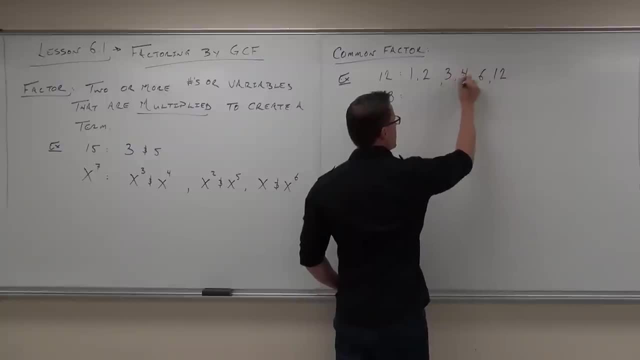 Three and five. As soon as you cross over and get a factor you already have listed, you know you're done For sure. You don't have to keep checking. So we have one, 12. Cool, We got two- six. 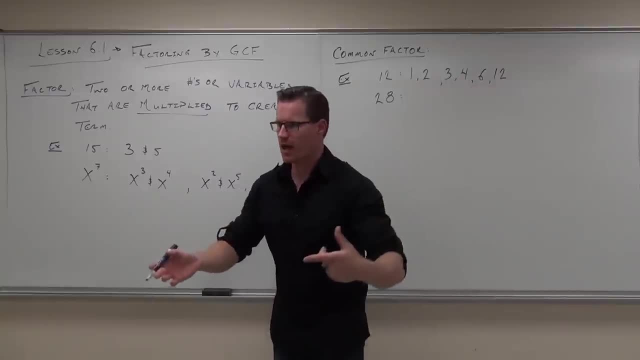 Cool, We got three, four, How about four? Oh, we already have it. As soon as you already have it, you're done with your factors. So, as soon as you cross over and get one, you already have, you're done. 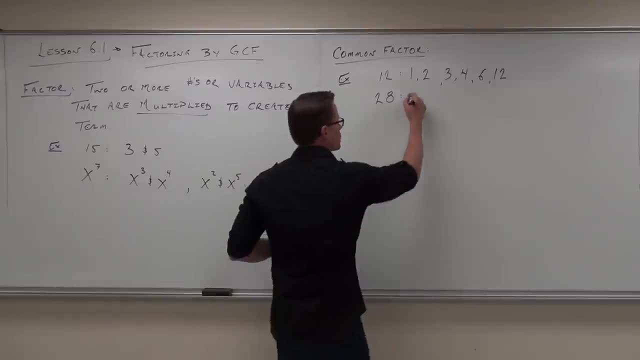 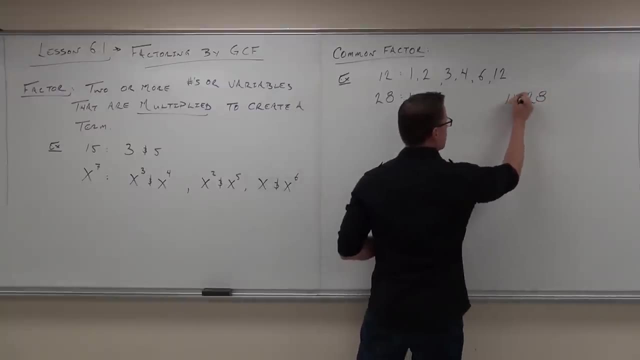 Now let's do 28.. Well, should we start with 28? One, Yeah, Sure. How about two? Is two a factor? Two and what? Four? Four and eight? Uh-huh, How about three? Is three a factor? 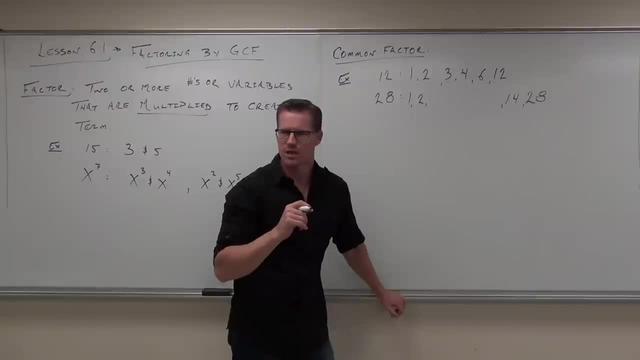 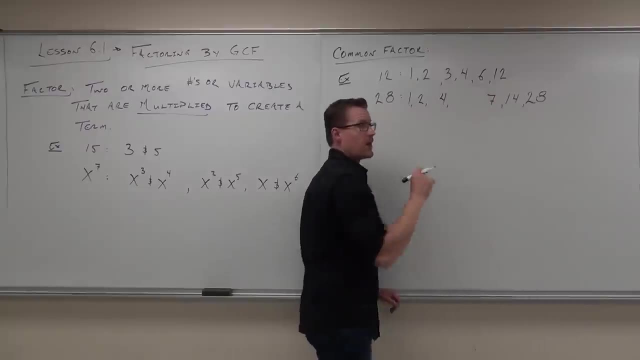 No, No. Does three go into 28 evenly? No, Then it can't be a factor. How about four? Does four work? Yeah, Yeah, Okay. How about five? No. How about six? No, No. How about seven? 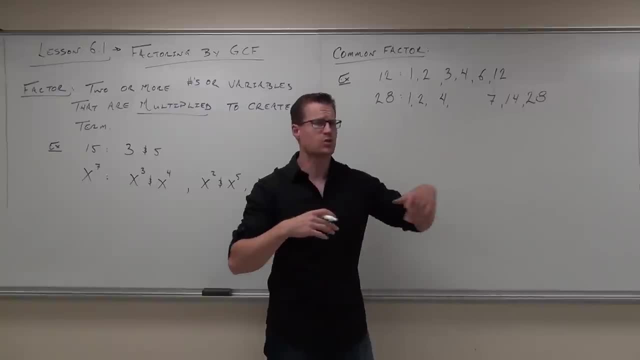 Yes, Is it already on the board? Yes, Then we have listed all of our factors. If you do it in pairs, it's pretty quick like that. Not sure if you're all right with that so far. Now we're going to talk about the common factors. 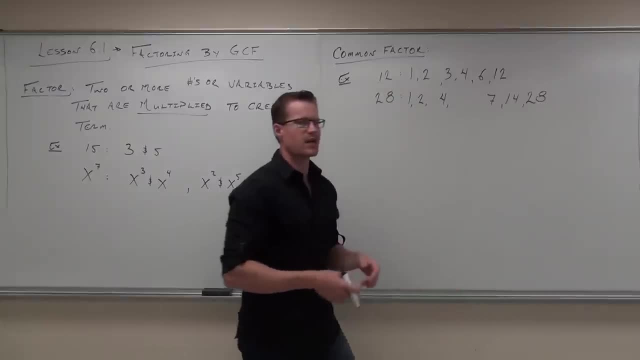 All you got to do, if you've listed them all out, is look for the factors that are the same. Give me one common factor Two. How about one One? Yeah, Does it do anything for it? Not really. It's always going to be one. 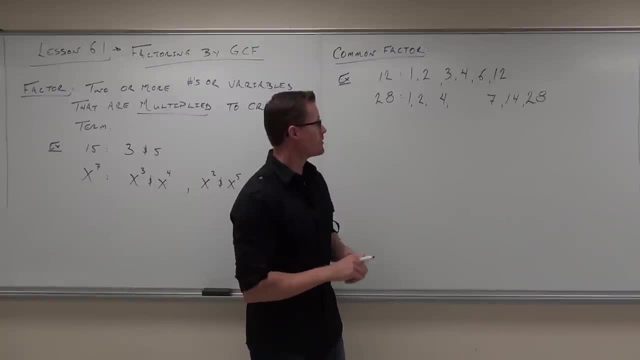 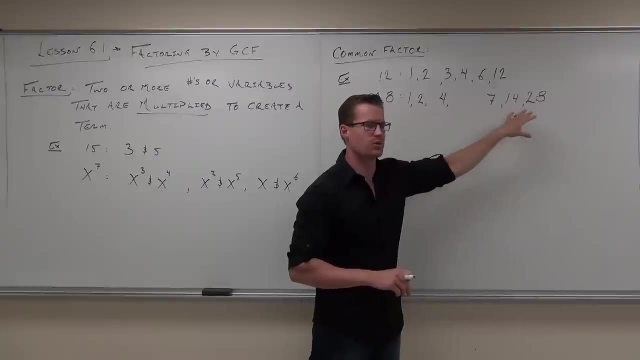 Two, What else? Four, Four, Anything else, No, Okay, So we know one's common, two's common, four's, not three, not six, not 12.. They're not listed in both numbers, But the idea of these factors being shared is the idea. 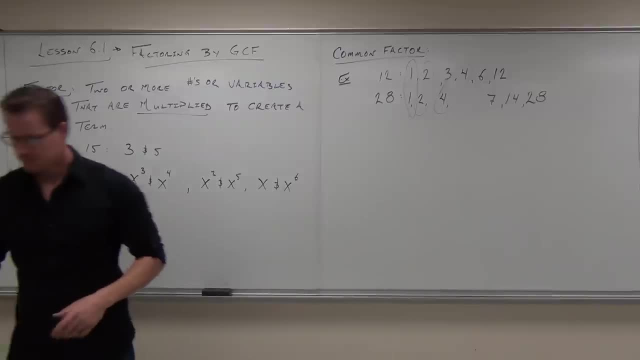 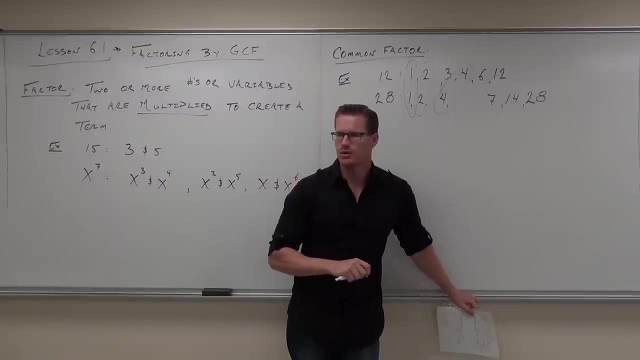 of a common factor. Now, what we're going to get to eventually is the greatest common factor. We can probably talk about it right now. What one of those factors is the biggest? The biggest number Four. That's the greatest common factor. 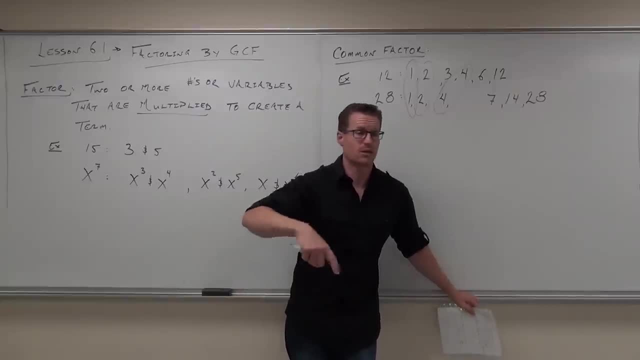 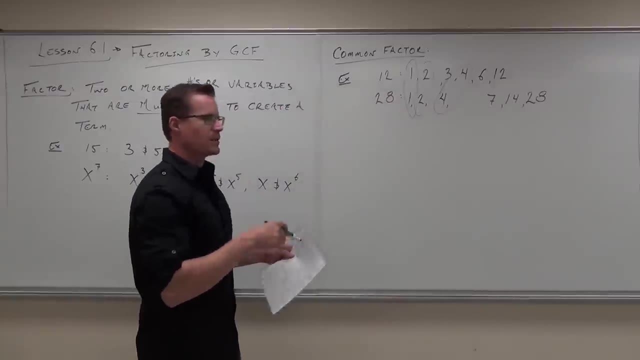 And that's the idea that you're going to be dealing with a lot of this chapter. It's talking about greatest common factor first. Now what's also interesting is we can list out the factors for variables, And I alluded to it over here. 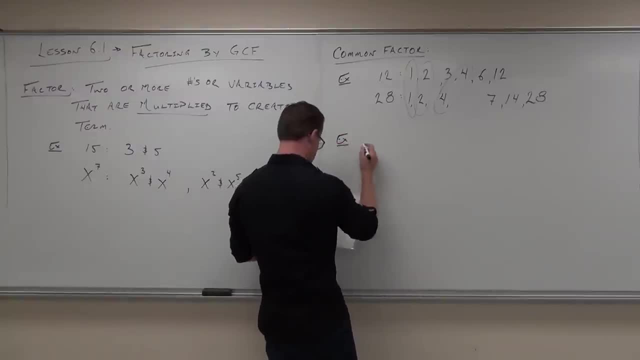 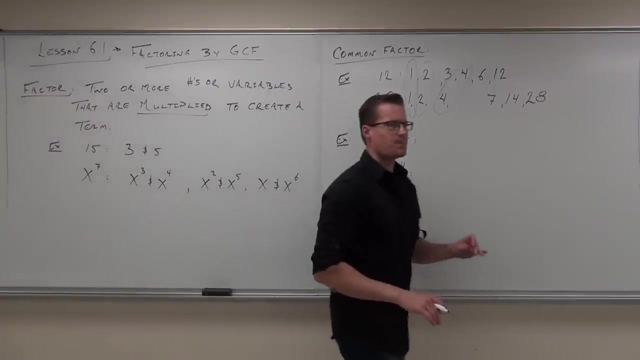 Let's talk about how you would list out the factors for 12x2.. And after that we're going to do 15x to the fourth Okay, And we'll talk specifically about how to deal with these variables. Well, how about this one? 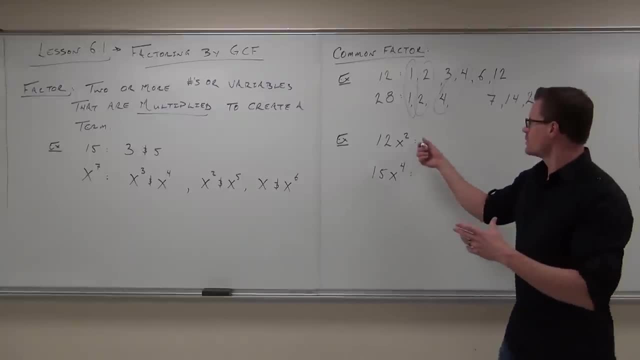 How about with the 12?? Do you realize that all of these factors- 1,, 2,, 3,, 4,, 6, and 12, they're all still going to be factors of 12x? Are you with me on that? 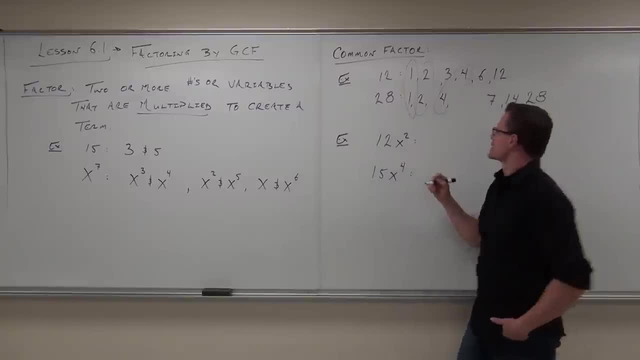 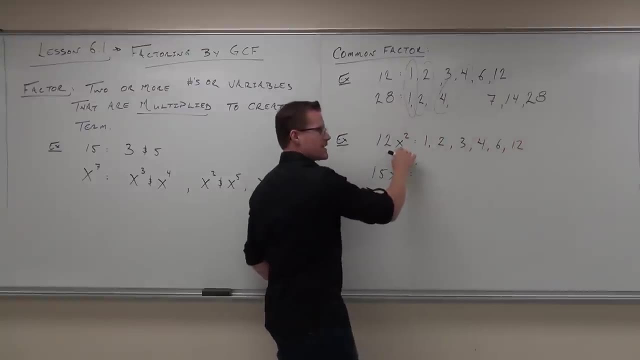 Do you understand why? Why we don't have? why we can list out 1,, 2,, 3,, 4,, 6, and 12.. And even though this has an x squared, these are still factors. Do you guys get that? 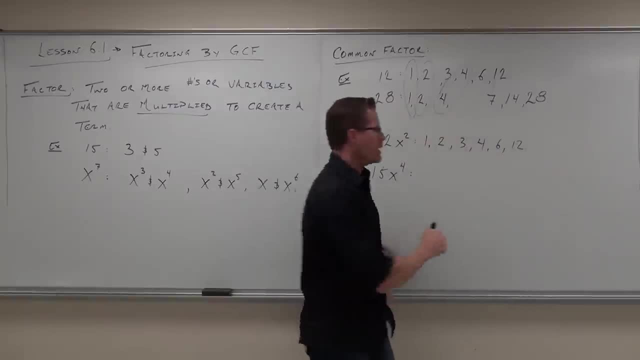 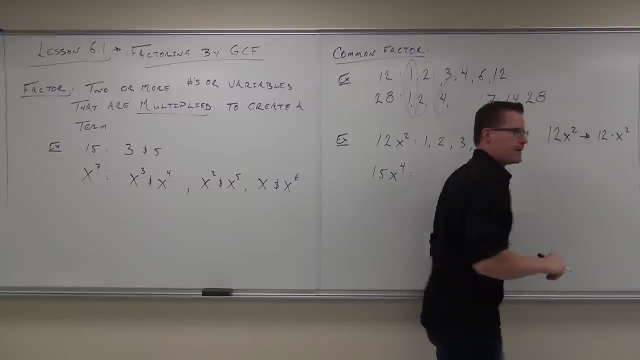 If you're not, if you're like, well, I get it, but you really don't get it. here's why Do you get that 12x squared is the same thing as 12 times x squared, If factors are these pieces that you get to multiply together? 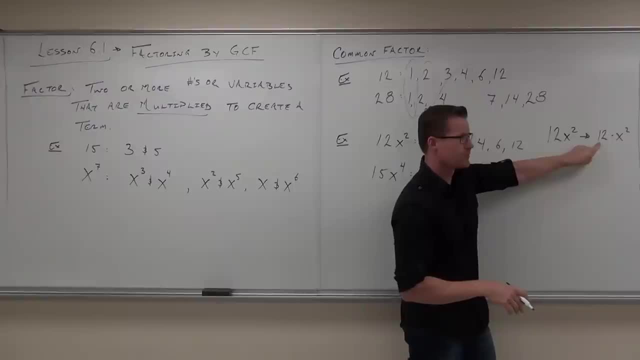 to create a term, then any factor of 12, when you multiply it by something else, will inherently create that same term. So anything that's a factor of 12, and I'm multiplying it, it's going to be a factor of 12x squared. 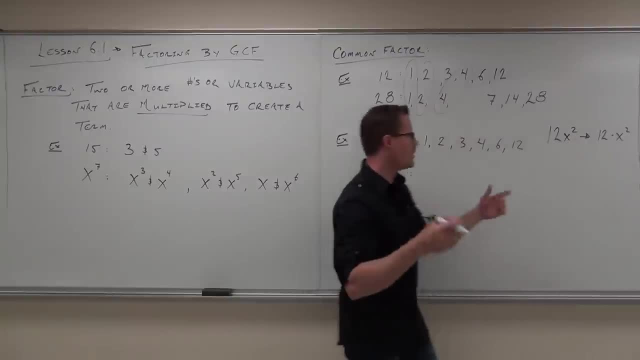 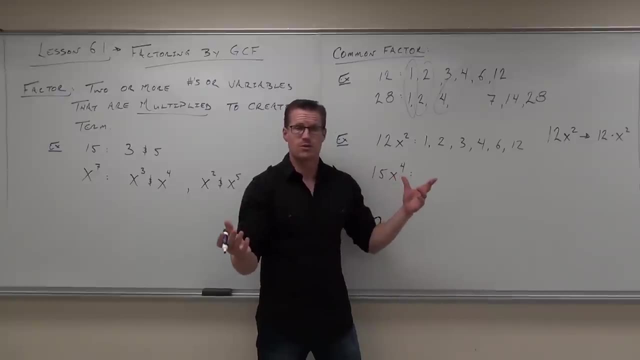 I'm going to multiply it by 12x, just by its very nature. Does that clear things up, if you didn't quite get that? So when we start with the factors of a term that has variables, you always start with just the factors of the numbers itself. 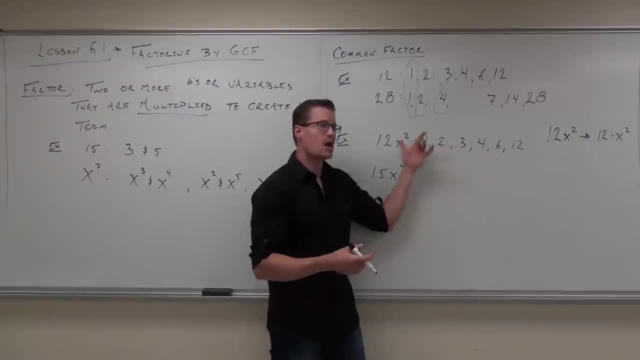 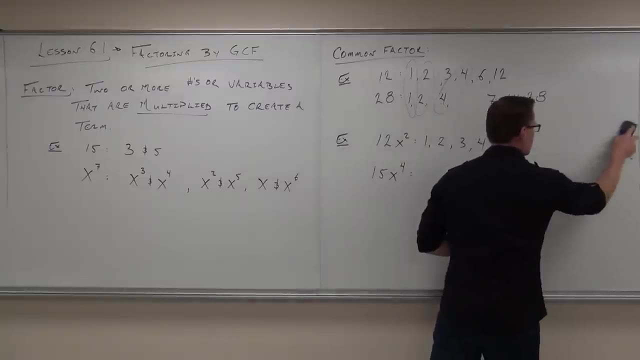 So something like 1,, 2,, 3,, 4,, 6,, 12, cool, that's just the numbers. Now we talk about the variables, So we're just going to tack those on here. Think back over here. 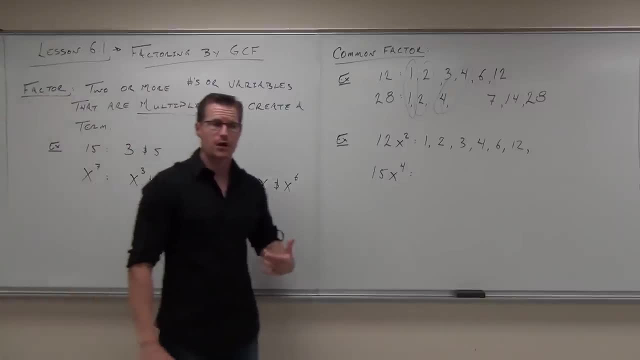 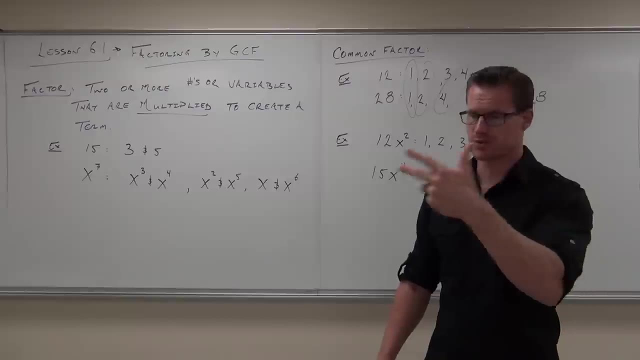 When we had x to the 7,, we had a lot of factors of x to the 7. In fact, we had a lot of factors of x to the 7.. The factors were x, x squared, x to the 3rd, x to the 4th, x to the 5th, x to the 6th. 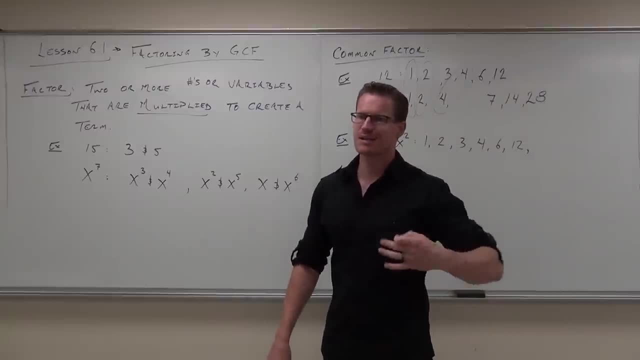 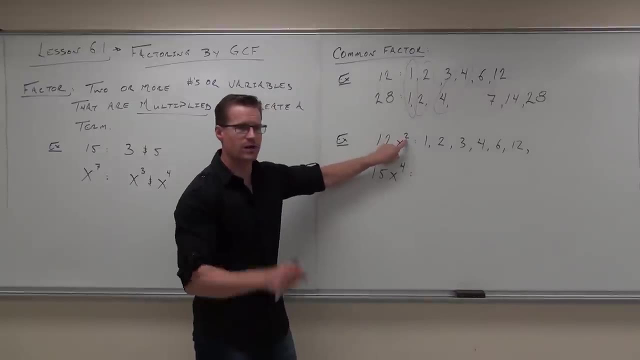 1 is already up there, and x to the 7th. So basically, every power- listen carefully, okay. every power leading up to this largest power is always a factor. So when you list this out, all you got to do is go: okay, well. 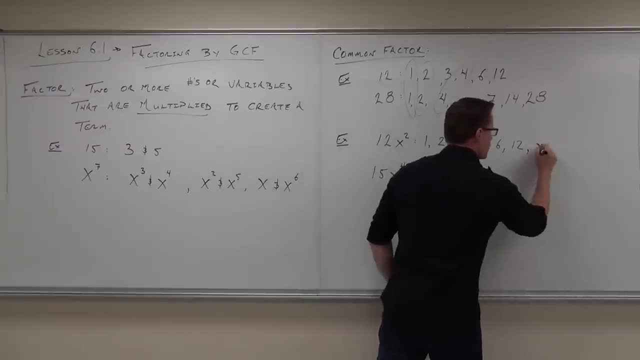 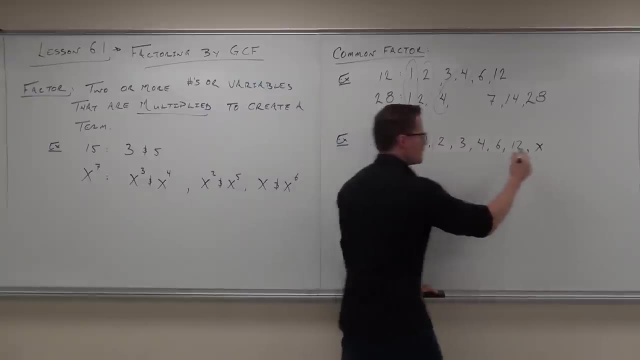 is x to the 1st a factor? Yes. Is x to the 2nd a factor? No. Is it here, Mm-hmm? Yeah, x to the 2nd is a factor. Is x to the 3rd a factor here? 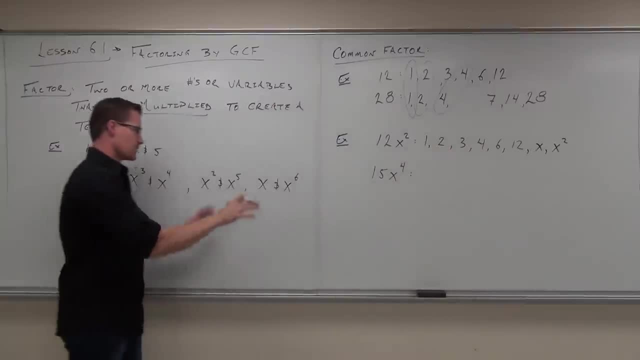 No, that'd be too much, But what you're going to do if I listed this out? okay, I'm going to take a little shortcut. If I listed out all the factors, I would have 1.. 1 goes into anything. 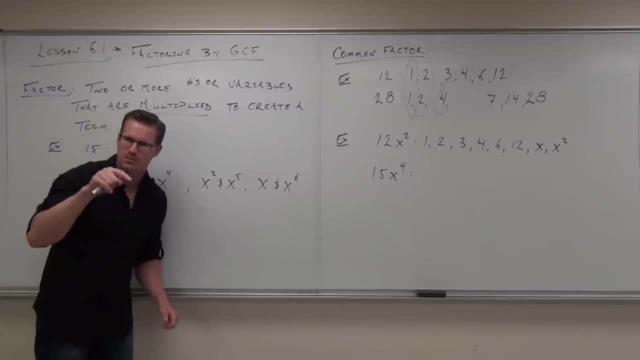 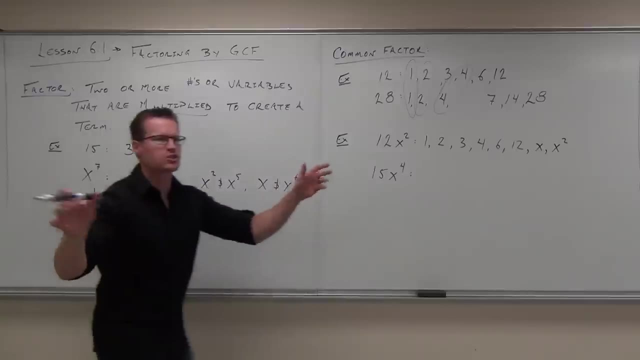 It's always a factor. Remember, factors come in pairs usually, So if I have 1, I would also have x to the 7th. Hey, just listen, Is it true that 1 times x to the 7th gives me x to the 7th? 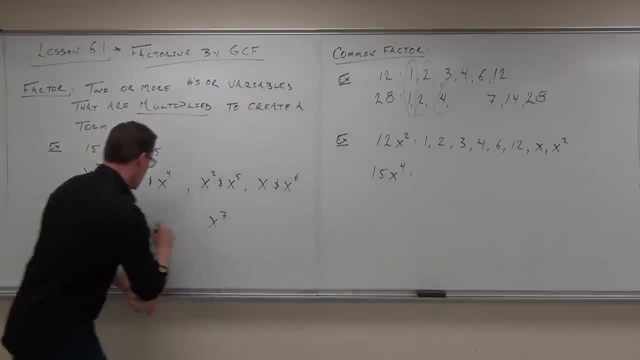 Those are factors. Multiply it together. They have to be factors. If I do x to the, just x to the 1st power, it's got to come in pairs. What else? x to the 6th, That's right. 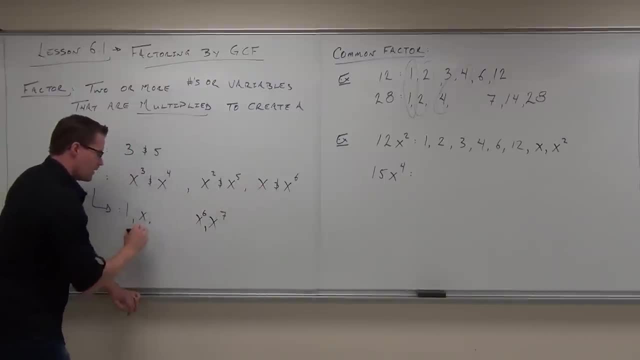 Hey, oh wait, look at that one. How about x to the 2nd? Can I multiply x to the 2nd by something to get x to the 7th? What is it? x to the 5th. 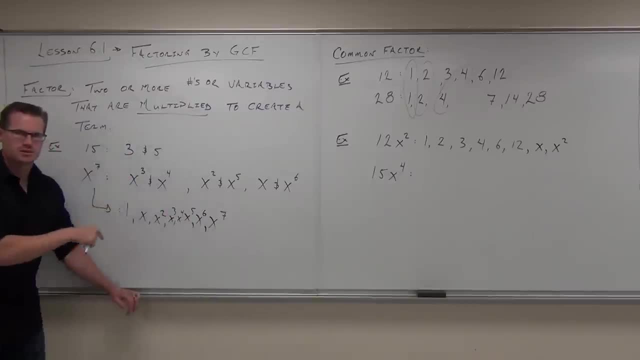 x to the 3rd, Yeah, x to the 4th, x to the 4th. Notice, look at this. What does this do? What this says is, if you do that by pairs, which you said that we already can do, right. 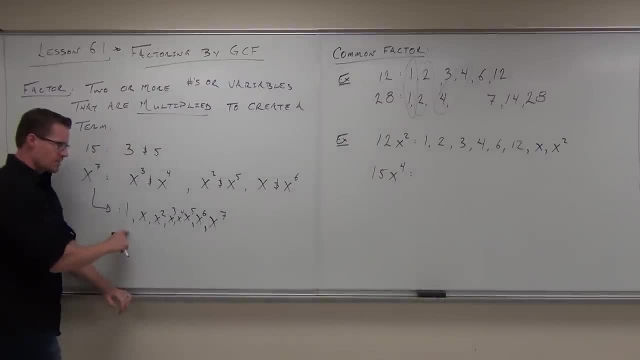 Are you with me? If you do that, then what you have listed out here is 1,, and then every single power of x up until you get to that power. So here we already have the 1. It's built in. 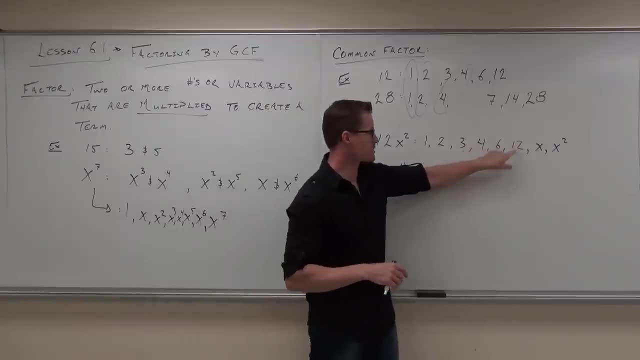 1's there all the time. We have the 2, the 3,, the 4,, the 6,, the 12, all by virtue of having that 12 in that term. Now we also have x. Is that a power underneath x squared? 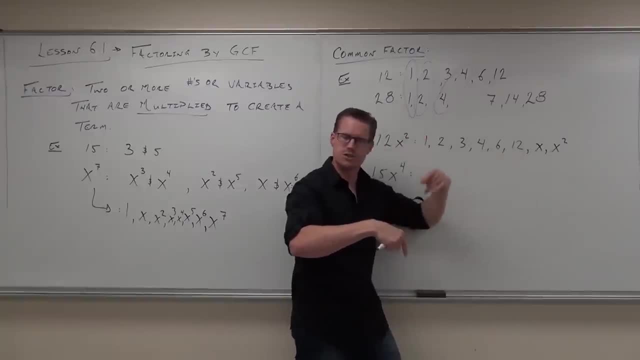 Mm-hmm x to the 2nd. Yeah, So we just list out every single power until we get to that one. Let's try it here. okay, You tell me what I'm going to have for my 15.. 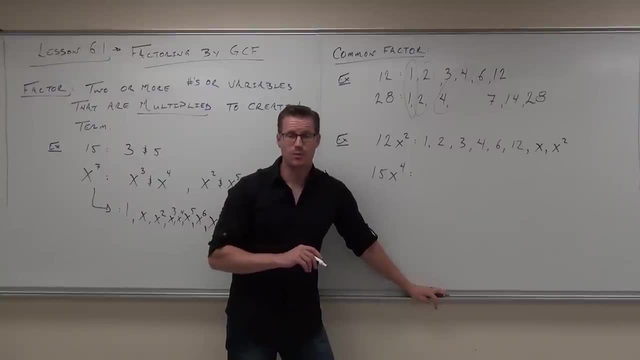 What's the first number that I'm going to put up there? 1. Probably 1, because I need the 15. So we deal with the numbers first. What else? 3. 3 comes with a 5.. Is there anything else? 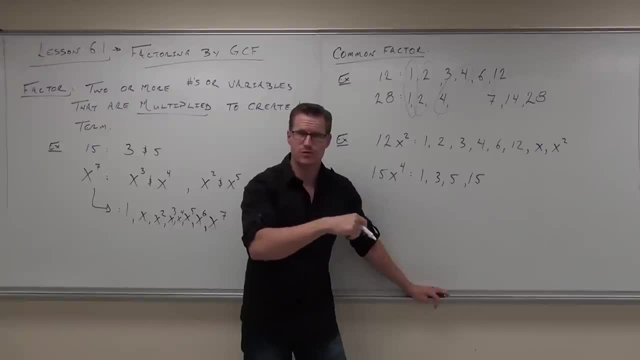 No. So 1 and 15,. 2 doesn't work, 3 works, 4 doesn't work. 5, we already get the 5.. We're done. We're done with our numbers. Now let's try the variables. 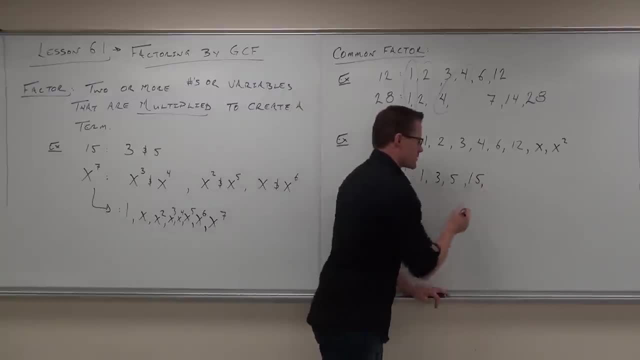 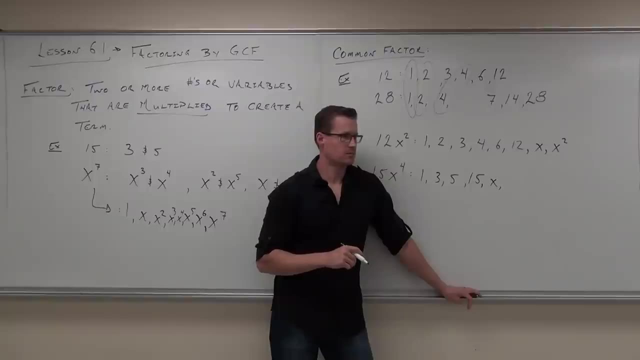 So I want us to list out what the variables are as far as our factors go. What's the first one? x, x. Should I put x squared up there? Mm-hmm, Yeah, Sure, Is it a power under x to the 4th. 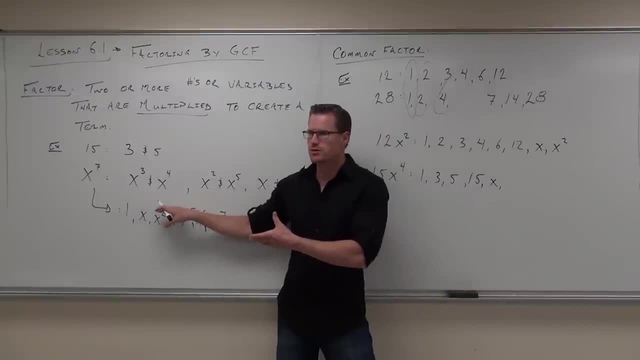 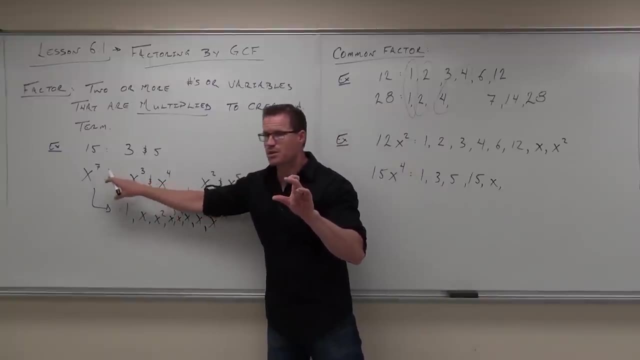 Mm-hmm, Do you guys get that? it's inherently a factor if it's less than that power, Because I can always write it as a power lower than this times. another power there: x to the 3rd. x to the 3rd is lower than x to the 7th multiplied by x to the 4th. 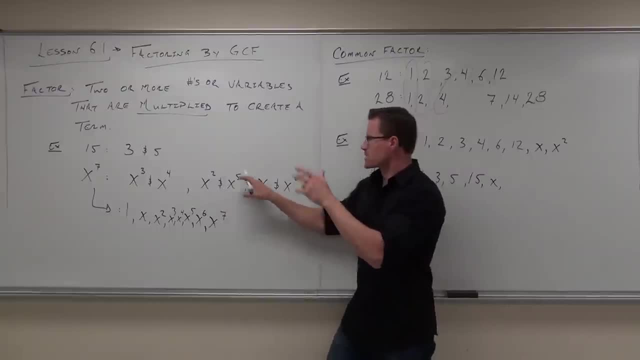 x to the 2nd is lower than x to the 7th multiplied by x to the 5th. x to the 1st is lower than x to the 7th multiplied by x to the 6th. You can always make that up. 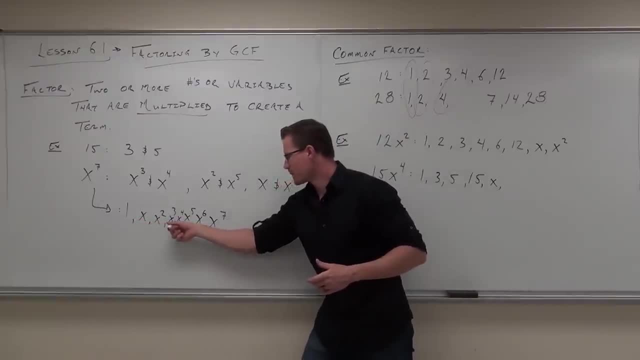 That means that every single power below or equal to that one is going to be a factor. We just list them, It makes it easy. So, x to the 1st, yes. x to the 2nd- yes. How about x to the 3rd? 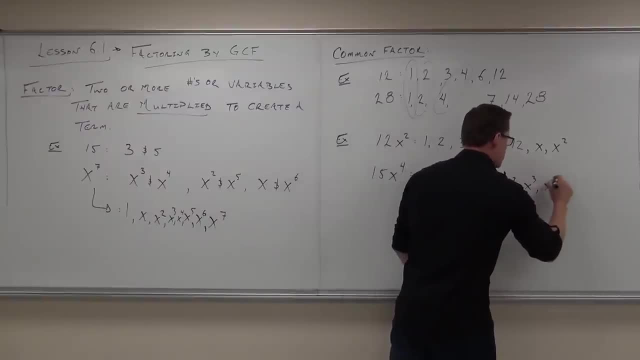 Yes, Of course. How about x to the 4th? Yes, Yes, Yeah, How about x to the 5th? No, x to the 4th? yes, Show of hands if you're okay with the factors as far as variables go. 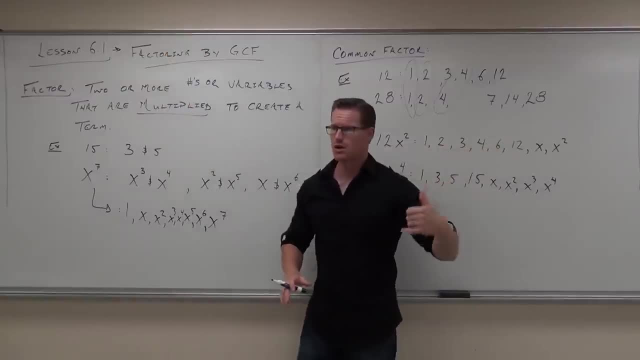 This part? yeah, probably pretty easy. I know. you know that The variables are what I'm talking about right now. That's what people get a little confused when pushing. The one that threw me off was the 12x squared at the very end where you have an x. 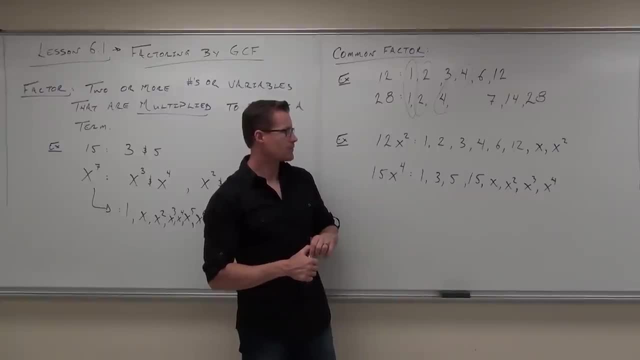 by itself and then the x squared, Because when I see that I'm seeing 3 with the two x's on the end, Okay, Keep in mind that what's going on here is that we're listing out these terms, We're not multiplying all these things together. 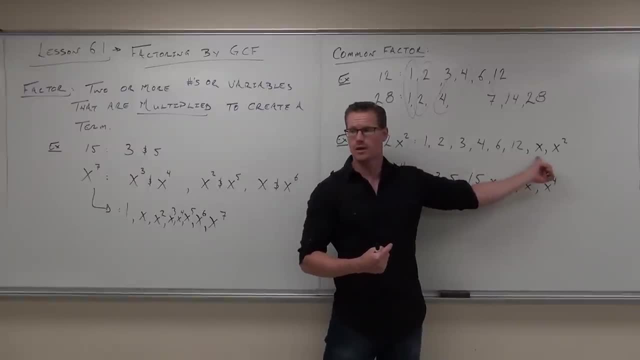 If you multiply all of these things, you're going to get x to the 4th. Okay, All these things, you're going to get way more than 12.. Oh, gotcha, Okay, And you're going to get way more than x squared. 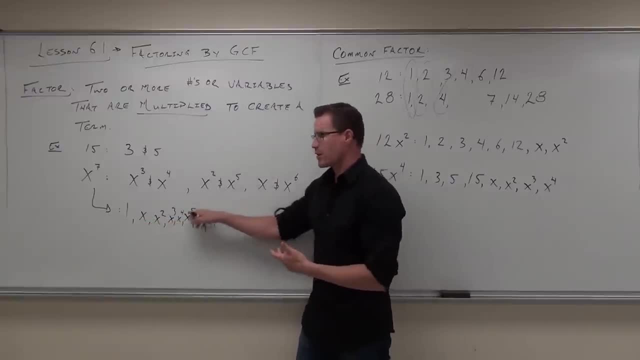 We're just listing them. If you multiply this all out, wow, that's x to the. add all those things up. What we're doing is saying: well, what could we divide by? We can divide by 1.. We can divide by x and x squared and x. 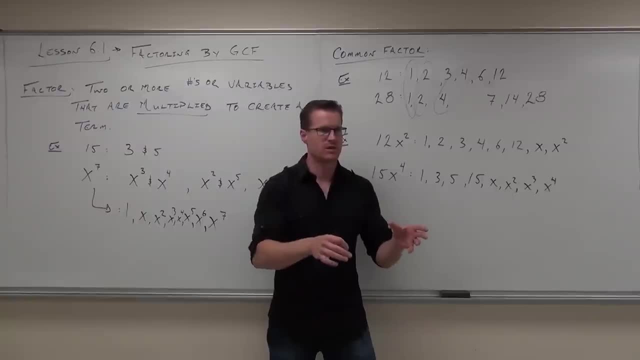 If you can divide by these things, they are factors, because that means that when you multiply two things together, they give you that term. So we're not multiplying these things, We're listing them right now. Did that clear that up for you? 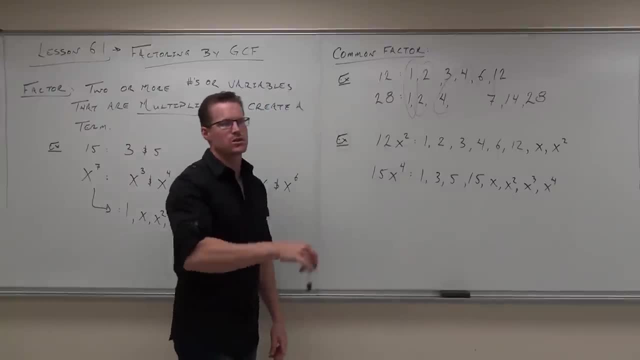 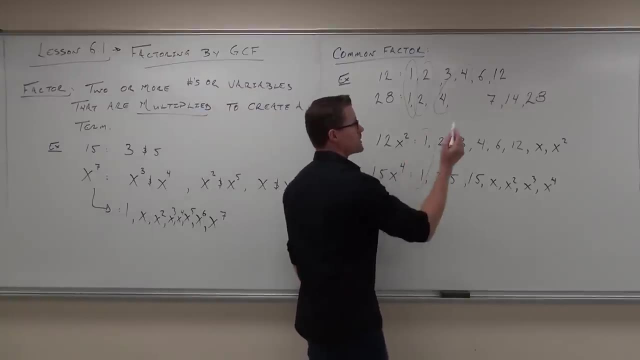 Okay, Now let's talk about the common factors, And this is where it's going to get important. What are some common factors here? What do you see? One, One, One, Three, Three, Great Three, Anything else. 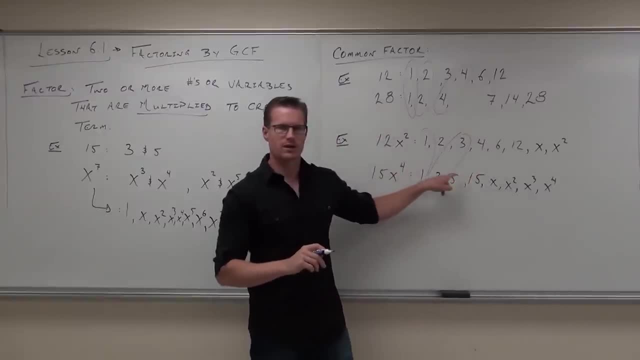 X. Oh, So as far as the numbers go, anything else besides 1 and 3?? No, What's the? listen carefully. okay, This is where we're going to jump to the greatest common factor. What's the biggest number? 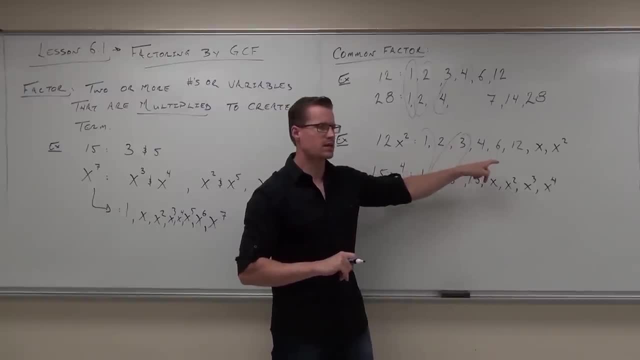 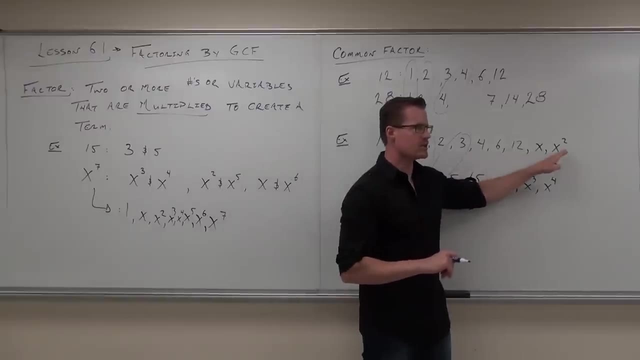 Three. Good, Now we look at the variables almost independently. So do we have common factors? Yes, Yeah, This is weird, though right, Every power is going to be listed up to the largest one, So X is a common factor. 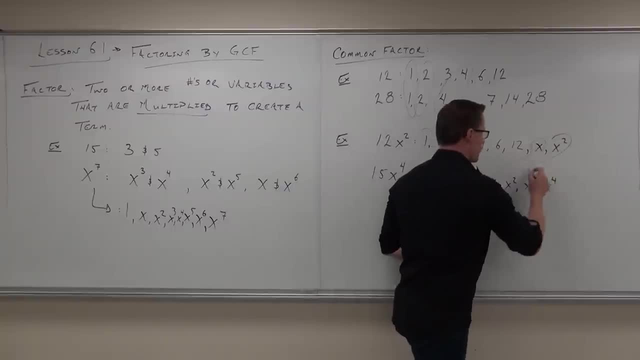 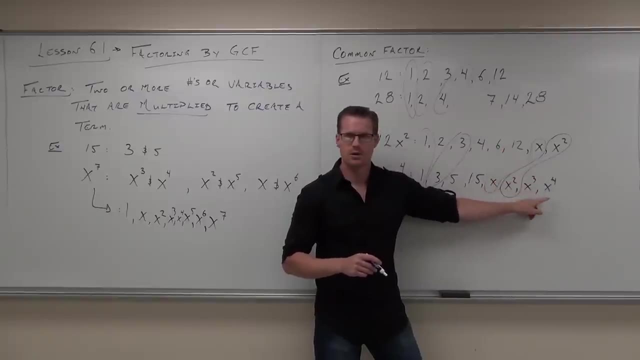 What else is a common factor? X squared. Now, how about X to the third? Is that a common factor? No, Is it in both places? No, No. How about X to the fourth? No, No. Okay, What's bigger? X or X squared? 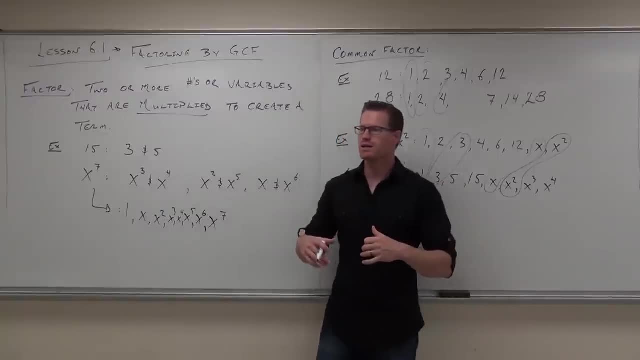 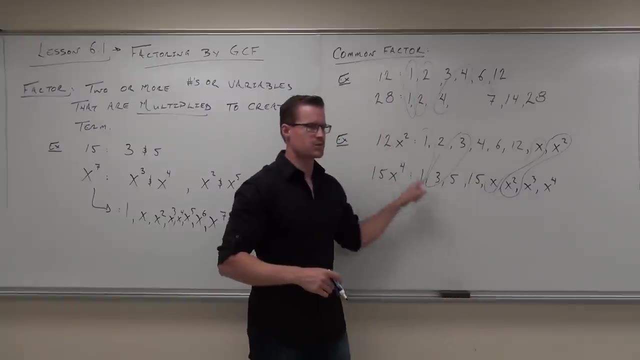 X squared. Same question as what's bigger, 1 or 3?? So when we get to talk about the greatest common factor, here's what you do: and listen carefully, You find the greatest common factor of the numbers. That would be 3.. 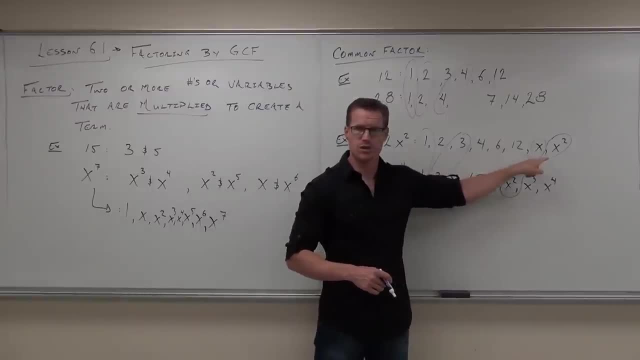 You with me. You find the greatest common factor of the variables. What's bigger Variables? You put those two together, So the 3 and the X squared. Why not the X, Because it's not going to be X squared. 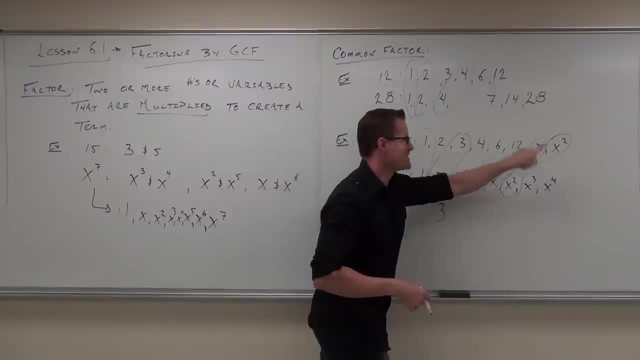 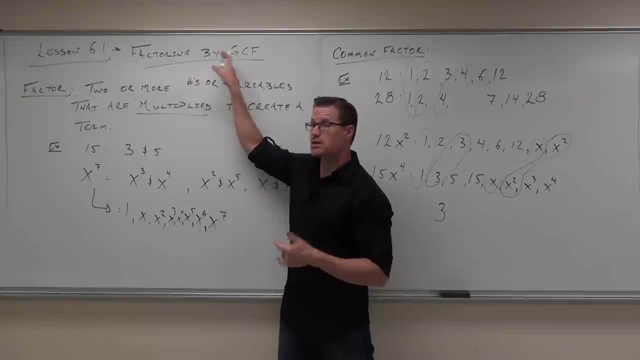 The biggest. Why not the X? to the fourth? Because it's not common, It's not there. You take the biggest one that's shared by both. That, by definition, is the greatest common shared factor. So what we do, we do the numbers, we do the variables. 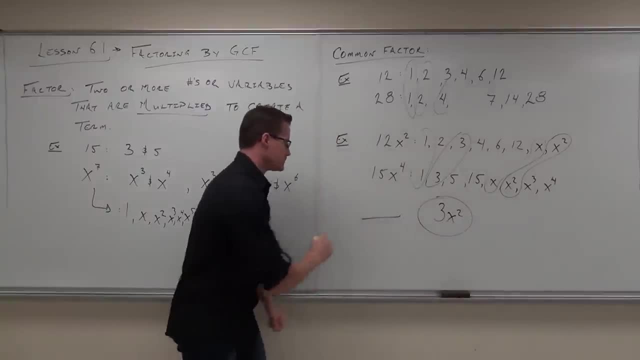 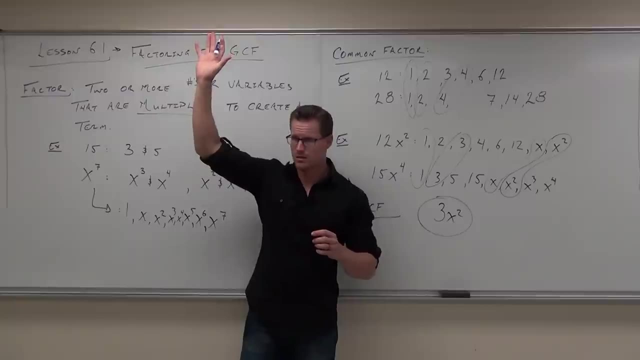 we put them together. This, right here, is the idea of the GCF. What I want to know is that: does that make sense to you? Show of hands. if it does, Do you feel okay with that? Yes, yes, yes. 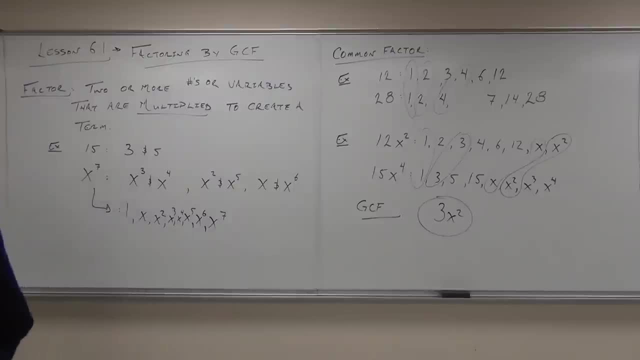 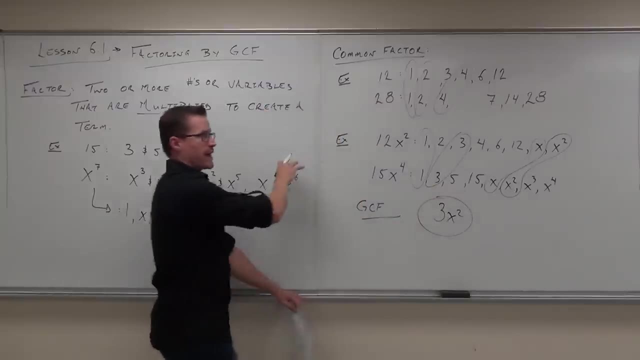 Destiny. yes, Okay, cool, Kind of cheated and went a little bit ahead. So when we're talking about this, we know what a factor is. Factors are those pieces that are multiplied together to give us terms. All about multiplication- Common factors when they're shared. and now we've jumped to the greatest common factor. 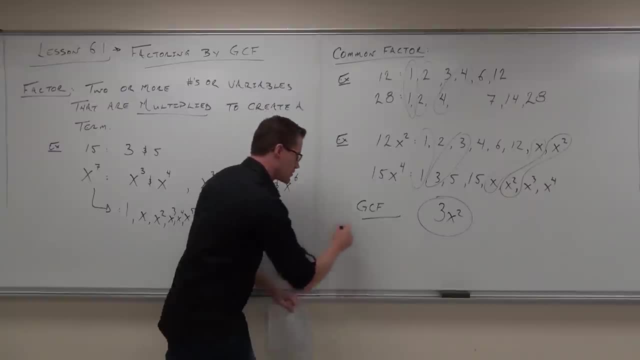 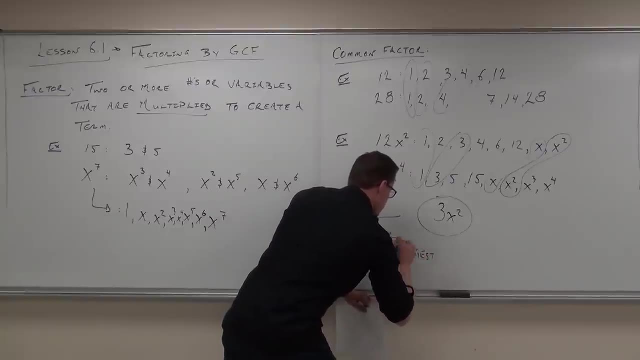 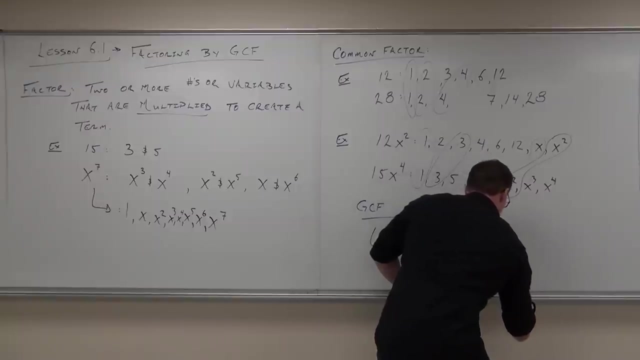 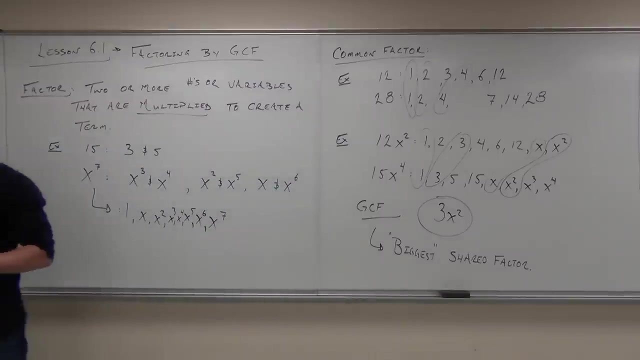 The greatest common factor is the biggest shared factor. So when we say GCF, what we mean here is the biggest shared factor. And right now, what I'd like to do, I'd like to just go over some examples and get us really. 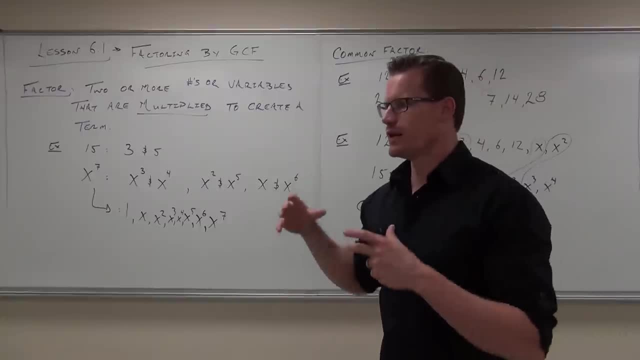 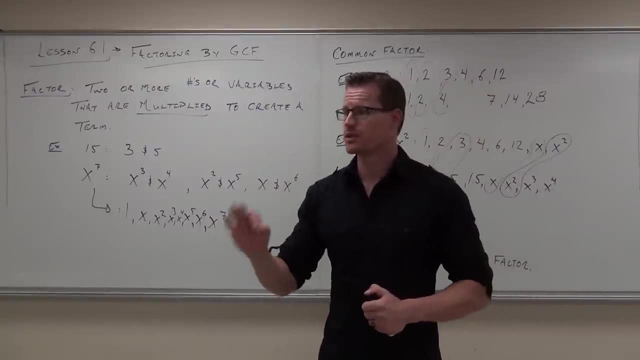 really, really good at finding this. If we fail at finding GCF, we're going to fail at factoring. This is huge for us. It's the very first step of your time is factoring the GCF whenever we talk about that. 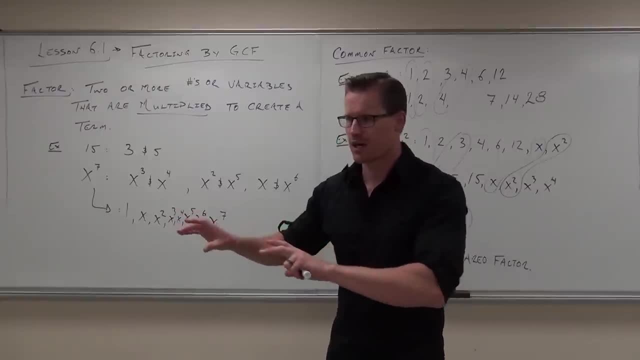 I'm getting through to you. So let's practice. We're not going to even worry about variables right now, We're just going to do some numbers, Just finding GCF. Are there any questions? No, Okay, All right, All right. 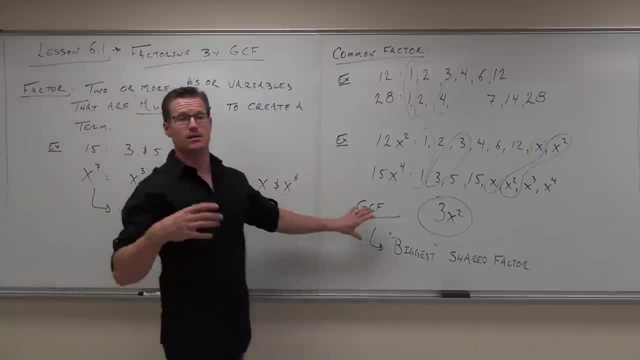 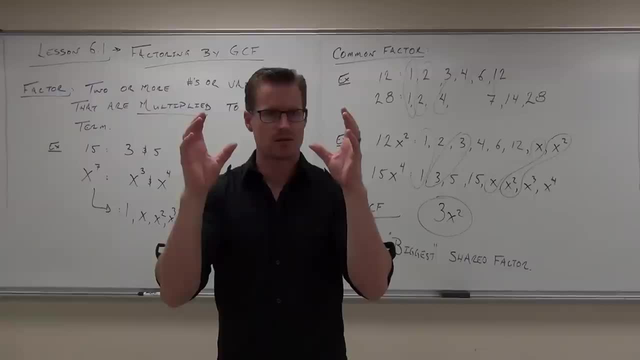 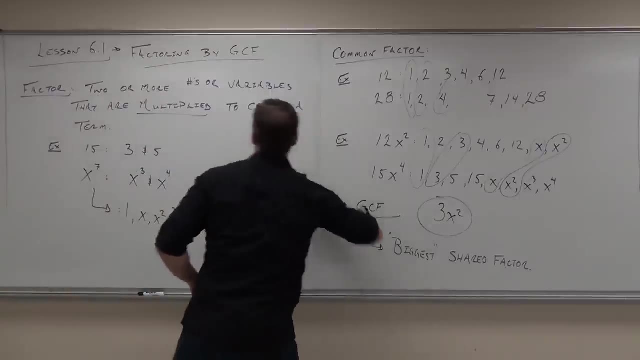 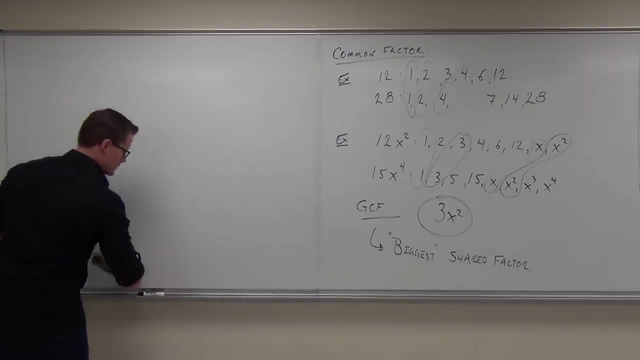 that the greatest common factor is just this biggest thing that's shared by both these terms. Do you understand that? The biggest factor? Okay, Good, It's shared by both terms. All right, All right. Well, if we're going to talk about the greatest common factor, this biggest shared factor, 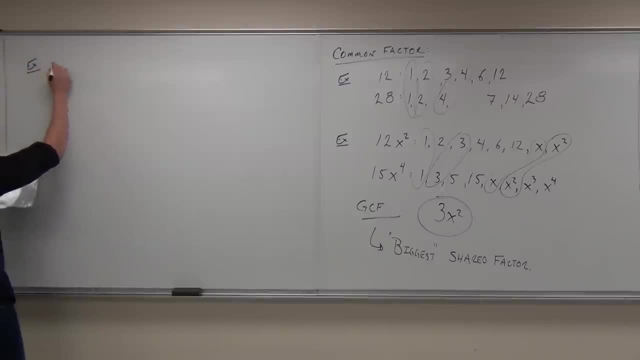 we've got to have at least two numbers, So let's start with 45 and 75.. Yeah, it looks like a 75 to me, doesn't it? I said, oh jeez, come on Leonard. 75.. 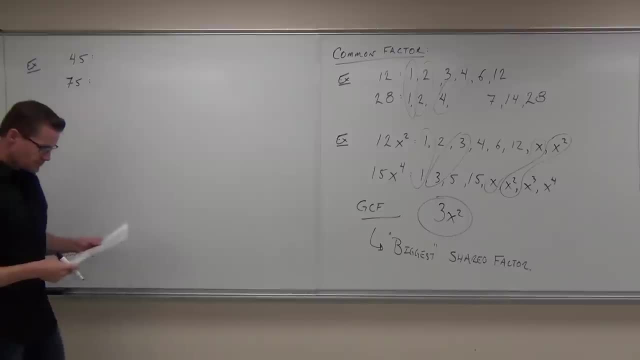 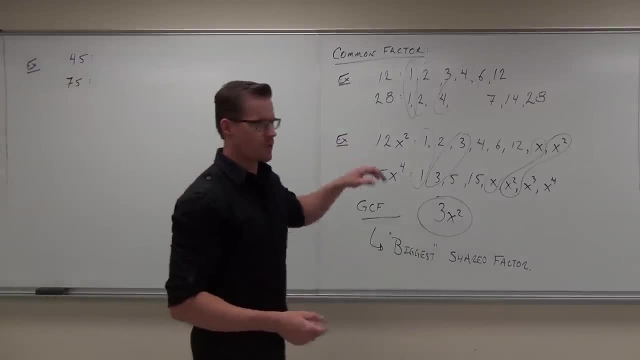 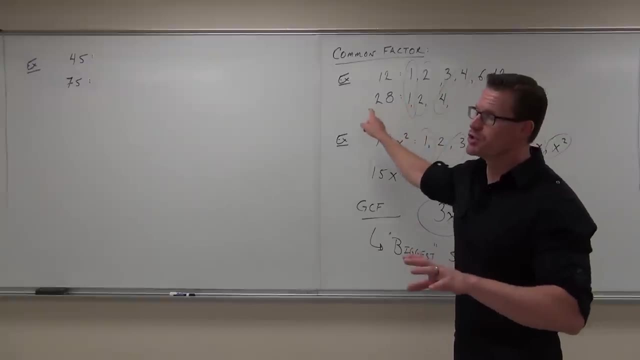 I'm going to give you two ways to do this. The first way is the way that you already know. I'm going to go very fast through that. method one This: listen them all out. That's your first method. You should know how to do that from a previous class. 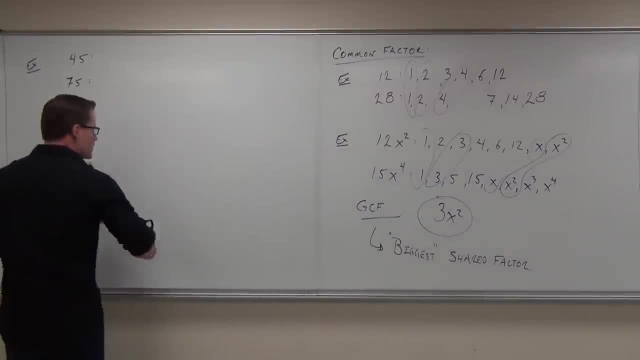 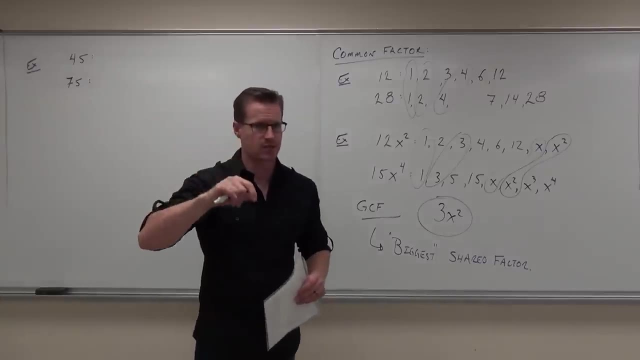 The second method some teachers gloss over, so I'll make sure you at least see it once. The first method is: man, just listen them all out. So if you have trouble with finding the GCF, just in your head, by the way, we need the greatest, so I don't want you to just give me one all the time. 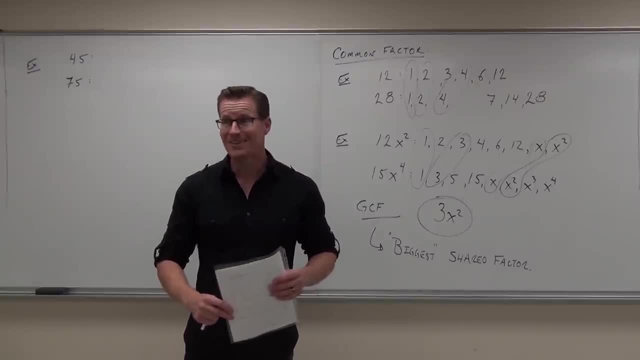 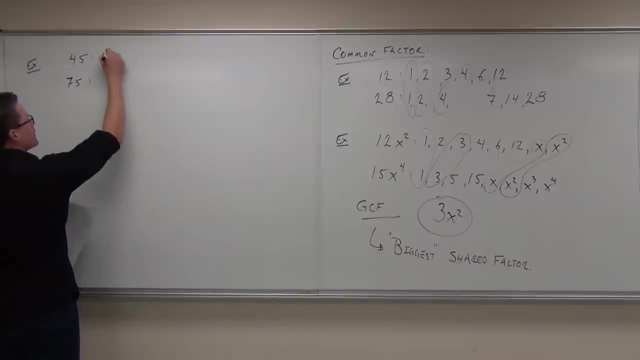 What's the greatest common factor One? No, That's the A factor. Is it the biggest one? It's definitely not, unless you have two relatively prime numbers, But no. So if we're going to list these out, we've got 1 and we've got 45.. 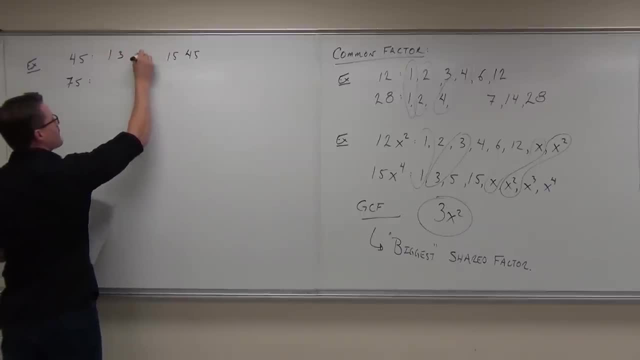 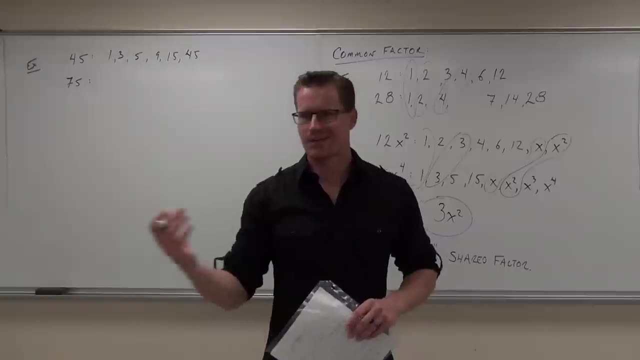 We'd have 3 and we'd have 15.. We'd have 5 and we'd have 9.. Did I miss any? Am I good? Can you think of any more? I can't think of any more. So 1,, 3,, 5,, 9,, 15,, 45, I think I have them all. 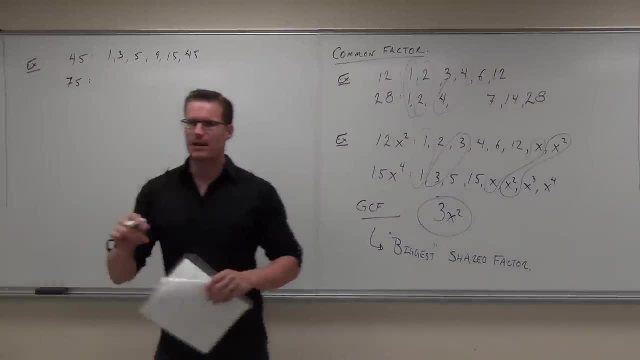 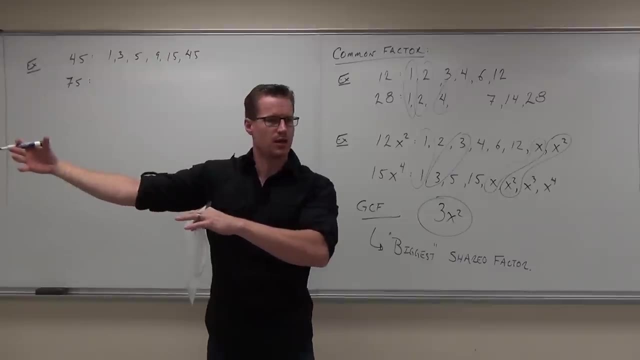 Let's do 75.. Again, my job right now is not to Teach you how to do this. This should be there already. My job is to teach you what to do with it afterwards. You follow So the next one. we've got 1,, we've got 75. 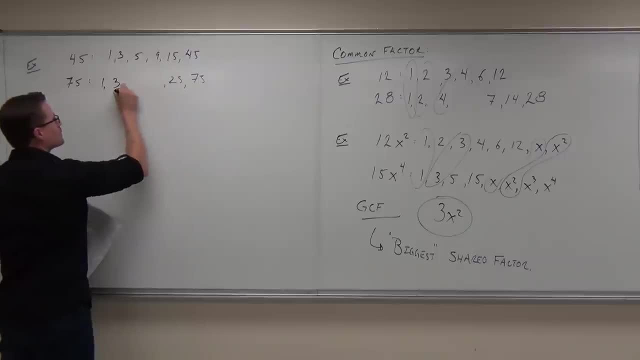 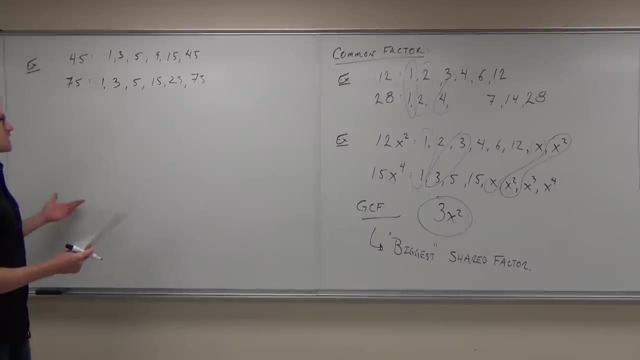 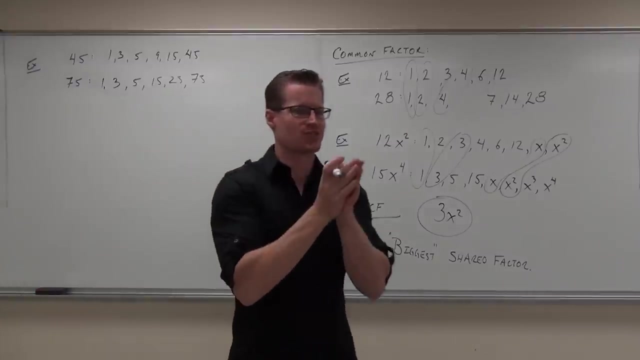 What else? 3 and 25.. Yep, 3 and 25.. Perfect, What else? 5 and 15.. Okay, anything else? Can you think of any more than that? That's all I have written down. Okay, Well, do we have any common factors? 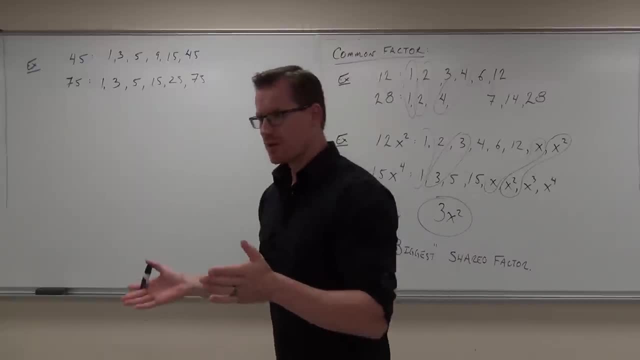 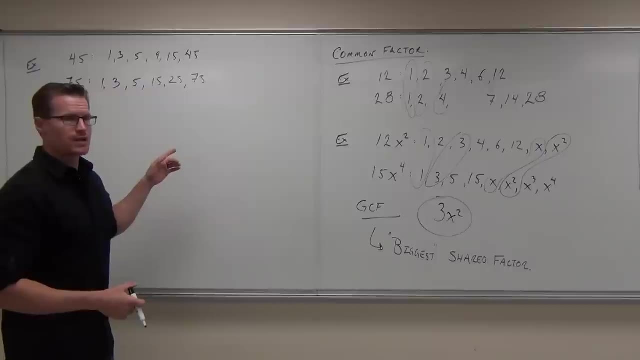 What's the first one? 1.. Is it the biggest one? No, Are you always going to have 1? Yes, Of course you are. 3, is that the biggest one? No, 5? No. Tell you what if 3 and 5 are both here? 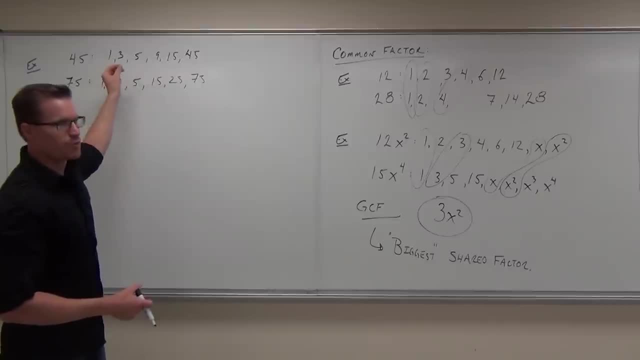 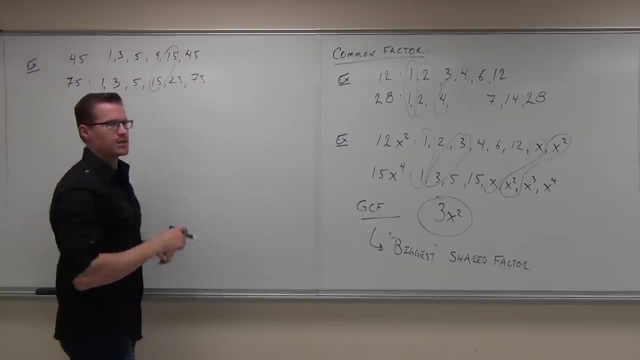 that means you have something bigger, Because if they're both multiplied to give you 15,, you're going to have a 15.. 15, is that the biggest one? Yes, So right now we know our GCF is 15.. 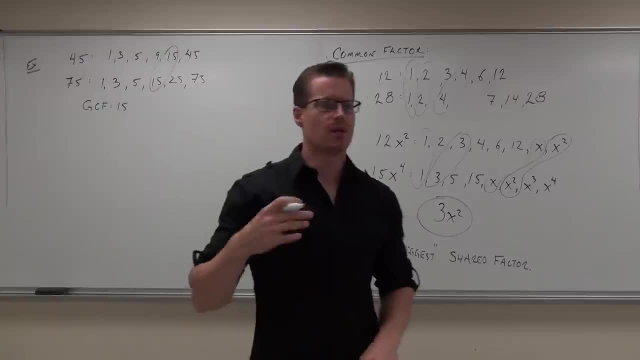 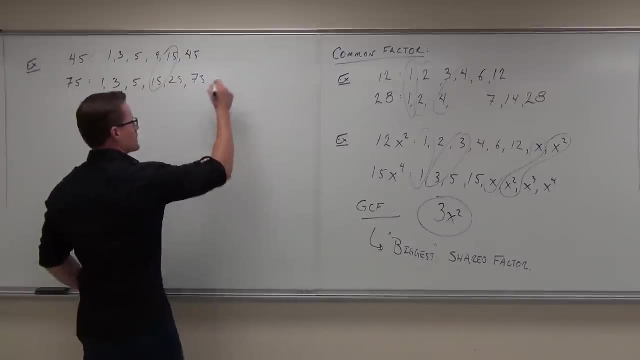 For small numbers. that's probably the way to go. We'll give you another way to do this, Not hard, just a little bit more kind of advanced thinking. I'll use some number theory here. So if I had 45, another way we could do this- 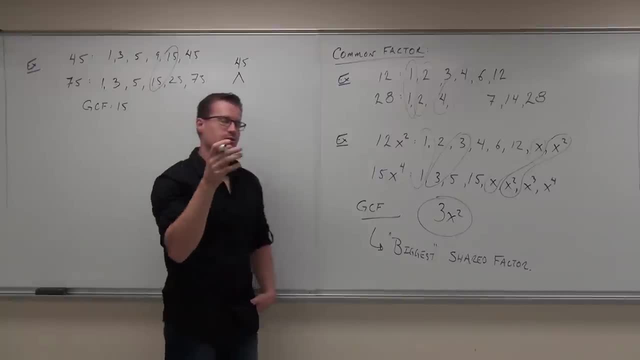 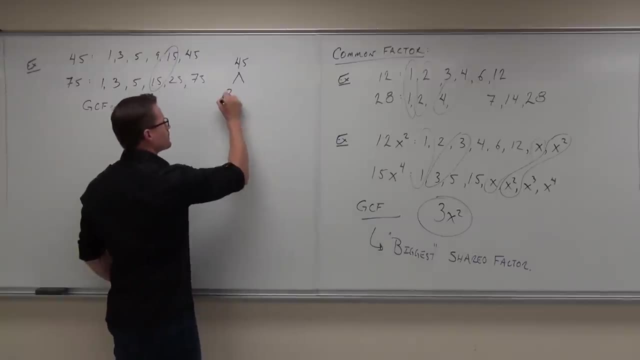 you could do this with a number tree, Number trees with factor trees with greatest common factors, and prime factorization says you start with the smallest prime numbers and you break it down until you have only prime numbers. here, For instance, 3 squared times 5 would be the prime factorization. 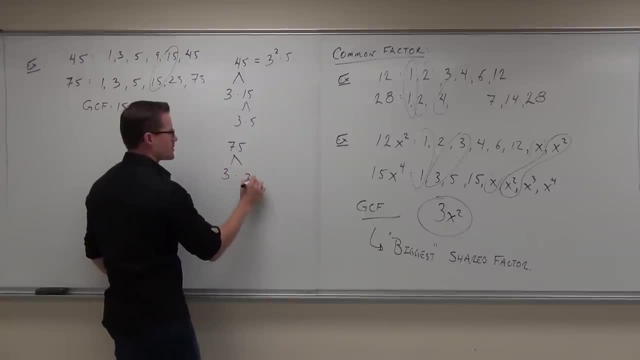 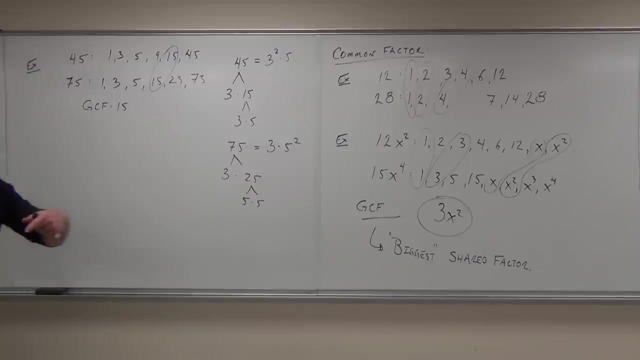 If you did 75, it'd start off really similar. You'd have 3 times 25 and that would give you 5 times 5.. So we would have 3 times 5 squared. I want to know if that makes sense to you. 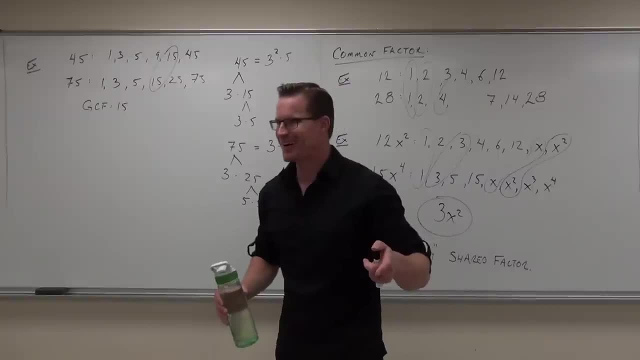 Have you seen that before? Yes, You might not remember exactly how to do it, but you've seen it before. You start with the smallest prime. it's not the biggest one, So you start with 2.. If there's no 2's, you go to 3.. 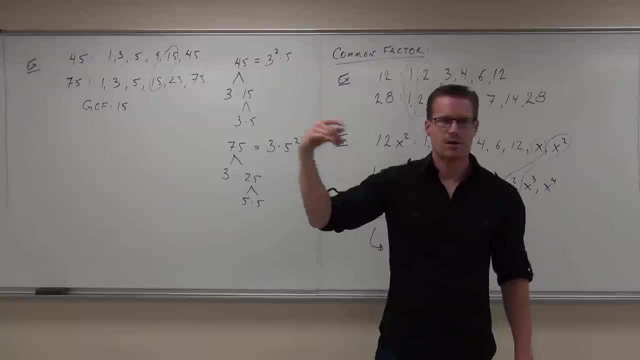 Then you go to 5, then you go to 7,, 9,, 11,, then 13 and so forth and so on. Well, if we did this, we got 3 squared times 5,. we got 3 times 5 squared. 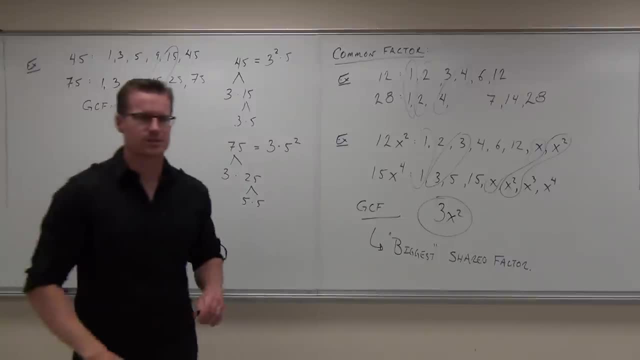 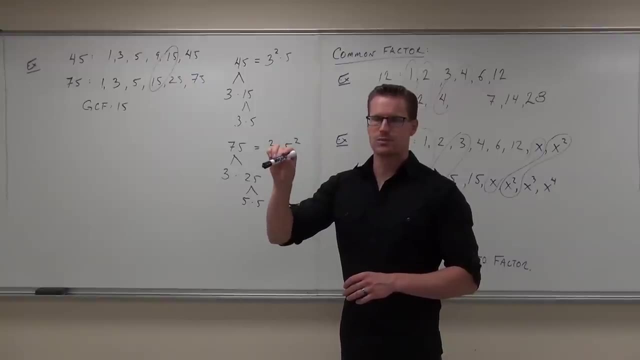 The GCF will always, always, always be the smallest powers of every. I hope some of you guys are not listening right now. This is a really good thing to do. I'll tell you right off the bat: it's probably the best way to go. 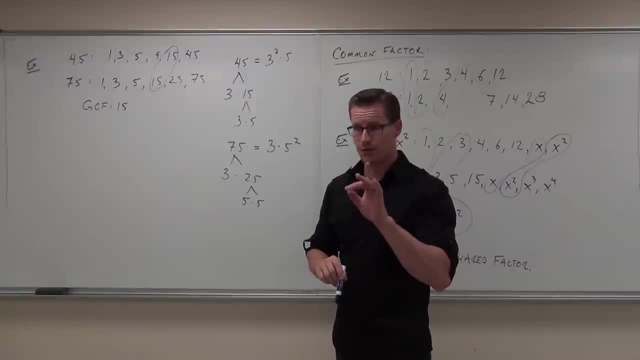 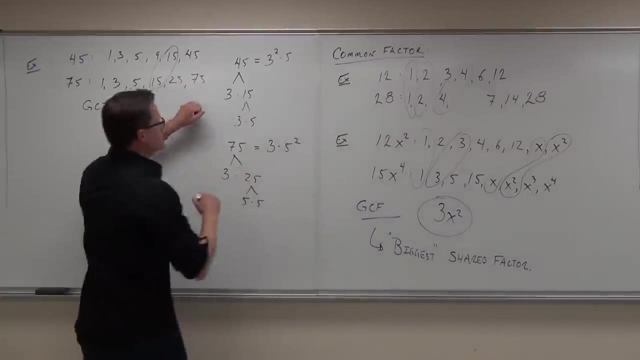 Take the smallest power of every different factor. The factors that I see here are 3 and 5, and then 3 and 5 again. Do you see that You can always find the GCF by doing this? What's smaller? folks smaller. 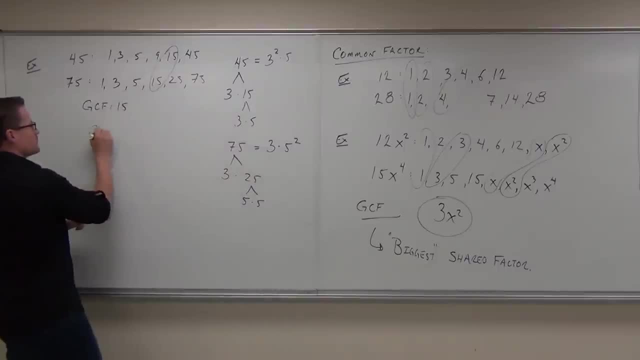 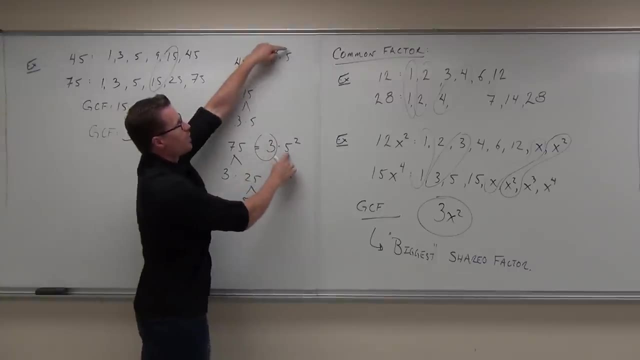 3 squared or 3? 3. 3. So GCF should be- yeah, I'm sorry, which one- 3. 3. That's smaller times. what's smaller? 5 or 5 squared 5.. 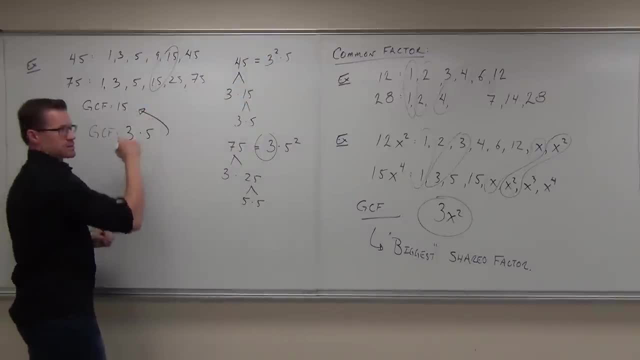 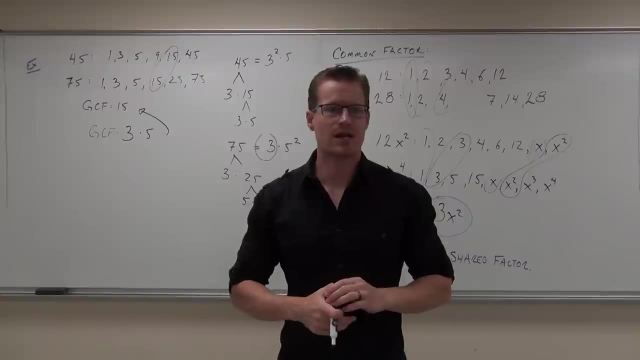 5. What's 3 times 5? 15. 15. Always, always works. Why that's nice is because if I give you really big numbers, like, let's do the greatest common factor of 196,, 2,187 or 84.. 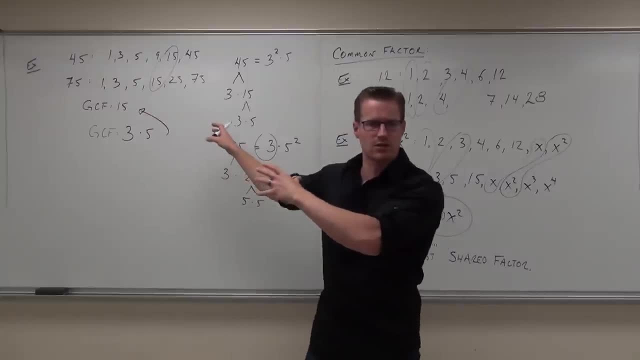 You don't want to do that in your head. You're going to want to write out every single factor of 2, whatever I said, even though I just made it up. You don't want to do that. No, but prime factorization is pretty quick. 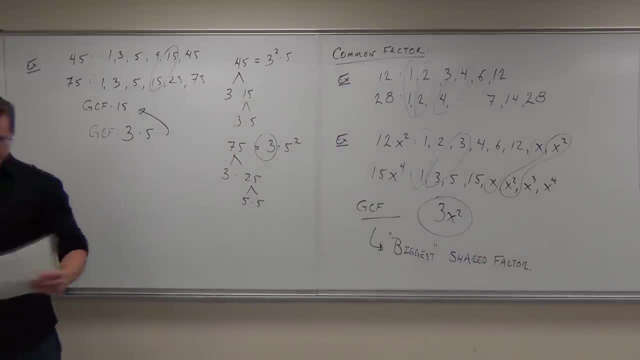 That's another way that you can go. Okay, Let's move on just a little bit. How about? how about 32 and 33?? 32 and 33.. 32 and 33.. What are the factors of 32?? 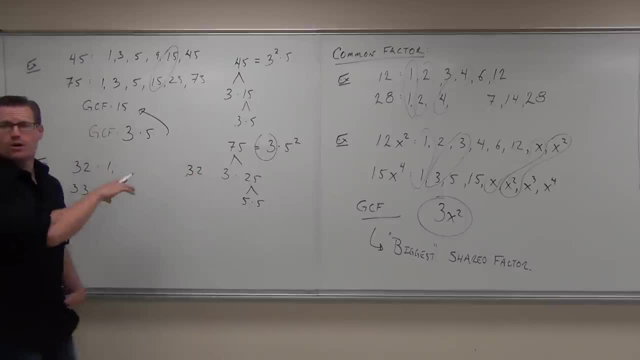 1 and 32.. 1 and 32, I'll give you that one, I'll do the hard one for you, okay. 1 and 32, I got it. I got your back 2 and 16.. 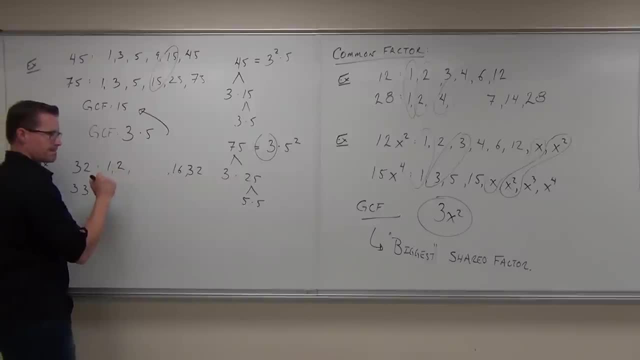 Give me another one. Give me someone else: 4 and 8.. 4 and 8.. 4 and 8.. How about 5?, 6?, No, 7?, 8? Already up there, Already got it, so we're done. 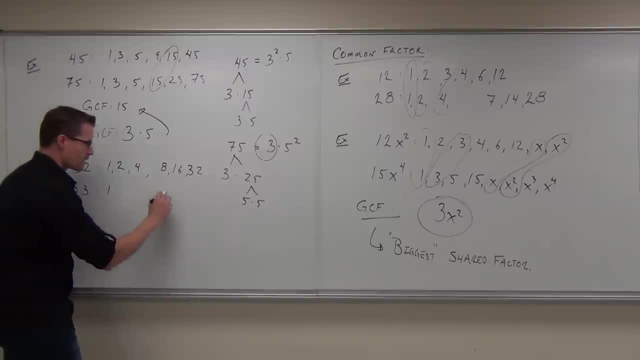 33 is going to be a little bit quicker here. We got 1 and we got 33.. Anything else, 4 doesn't work. 4 doesn't work. 5 doesn't work, 6 doesn't work. 7 doesn't work. 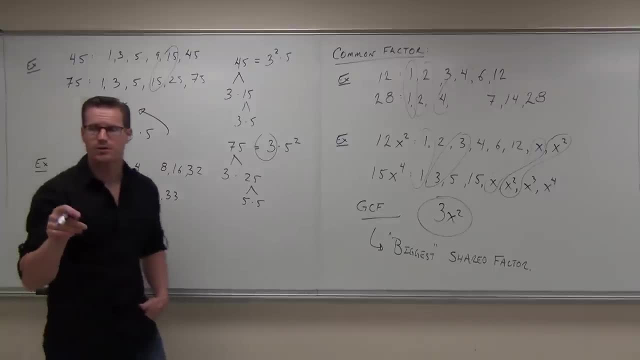 8 doesn't work, 9 doesn't work, 10 doesn't work, 11 does, but it's already up there, so we're done. Here's my question: Are there any common factors? Any common factors? Well, 1.. 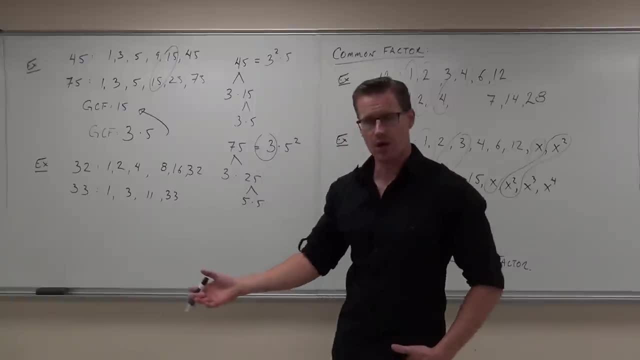 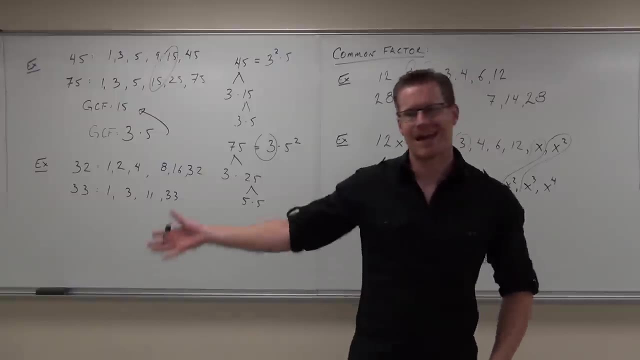 1. There's always at least one common factor, and it's 1.. So are there cases where you can have two numbers which only have a greatest common factor of 1?? Yeah, It's called. if you want to fancy words. 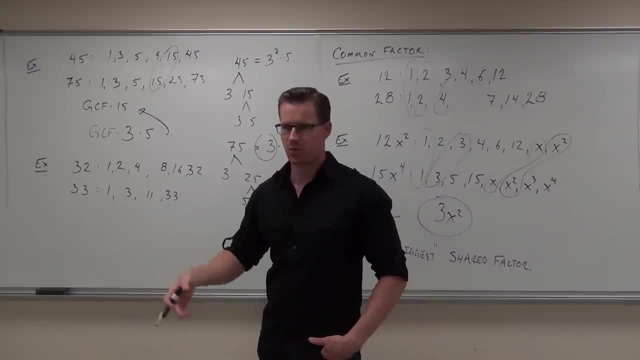 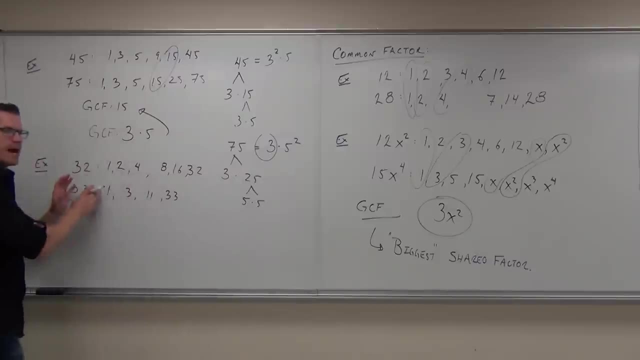 it's called relatively prime. It means that they have no common factors besides 1. Nothing will be common that you can factor out of those two numbers. This right here- this is what we're looking to have after we've factored is numbers. 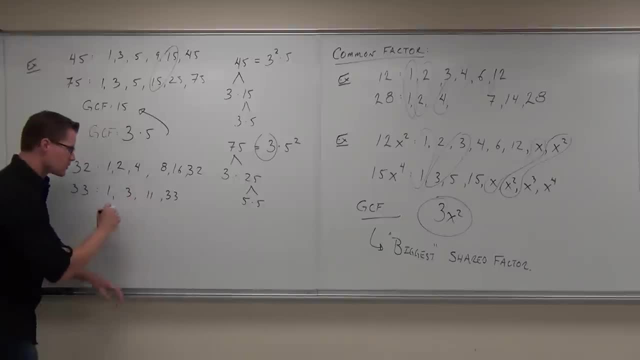 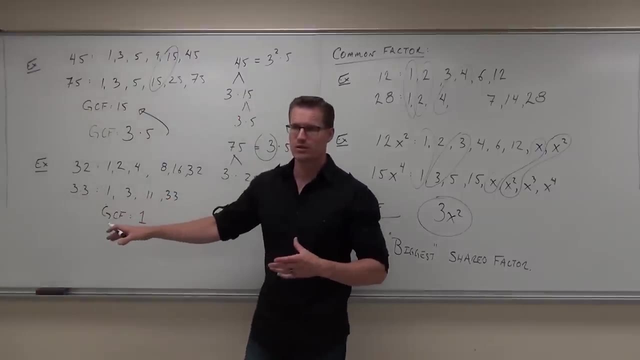 that are relatively prime. Okay That no other number goes into it besides 1.. So here, when you have a GCF of 1, it means that if I have two terms with those numbers, I'm not going to be able to factor it the way that I want. 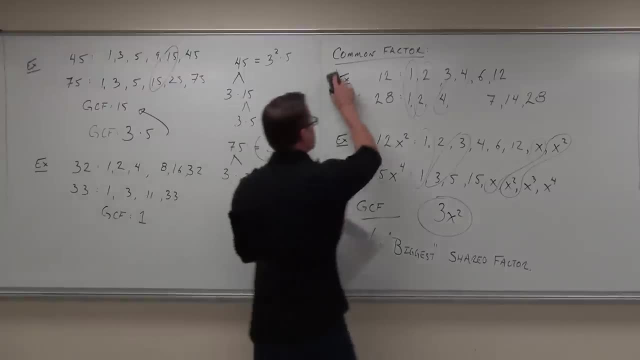 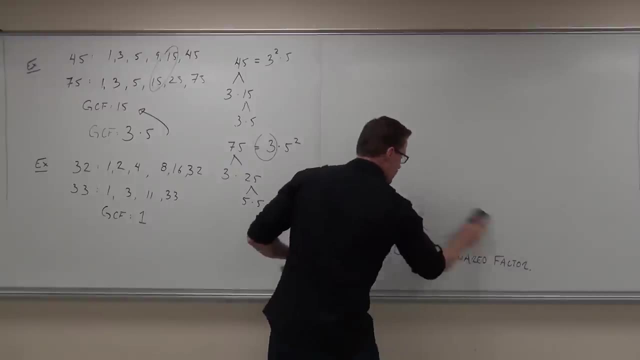 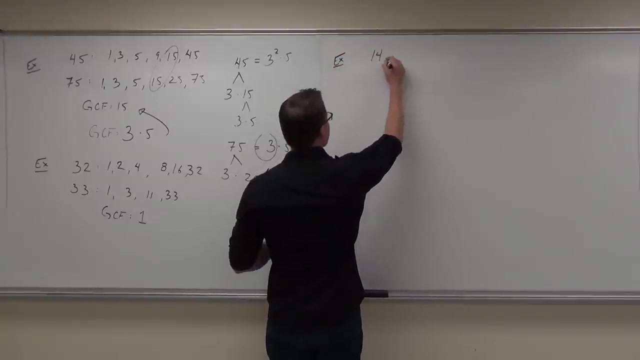 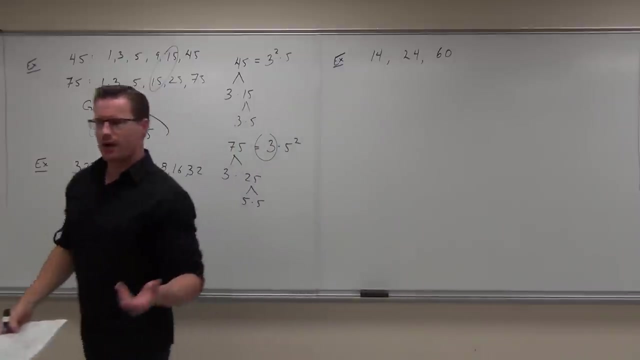 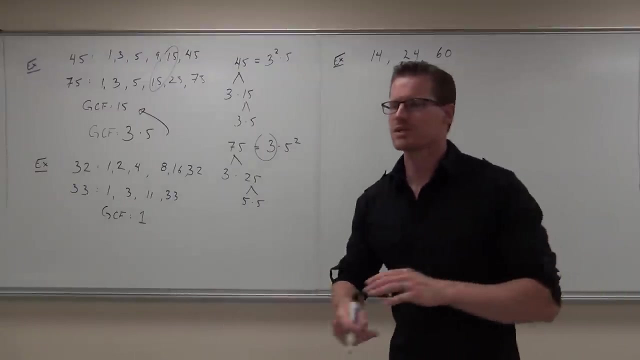 How about if I have a? oh, let's see How about 14,, 24, and 60?? Are we able to find the greatest common factor of three numbers? Is that possible? It means the same thing. It just means: hey, let's find the biggest number, that will go. 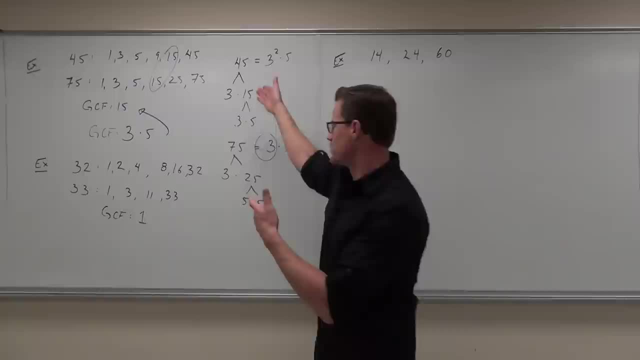 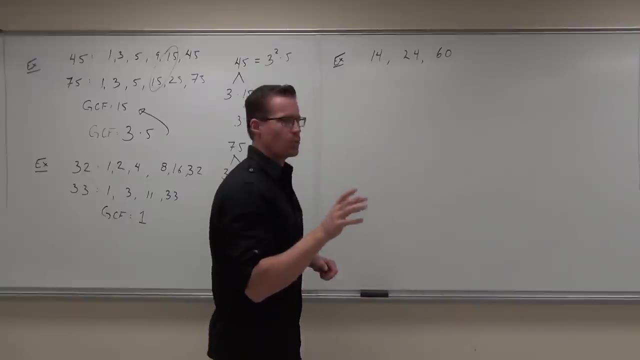 into all three, So you can do it the same way that you did before. You can do it this way. You can list out all the factors, if you want to, and find them. Just find them. So one if you want to do it kind of quickly. 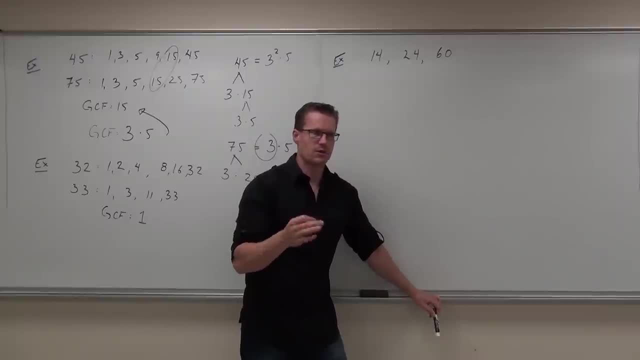 if you want to do it quickly and not write everything down, I'll give you a little helpful hint here: Start with the one that has the least number of factors. For instance, if I was going to do this in my head and I didn't want to write all of them down. 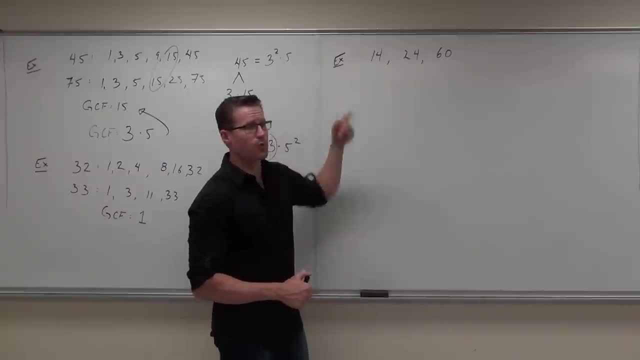 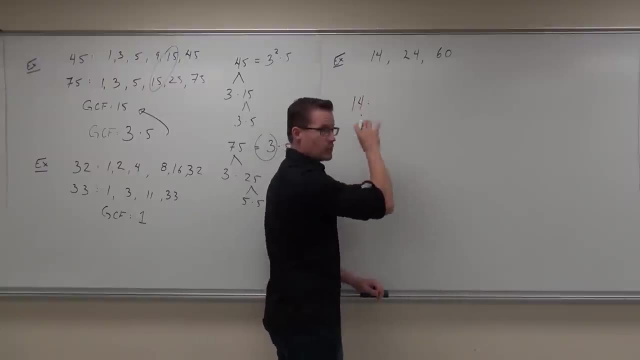 because I don't like doing that. okay, I'd start probably with 14.. Okay, here's what I'd do. I'd say 14, I'd write them out, so I don't miss any. You don't want to miss any. 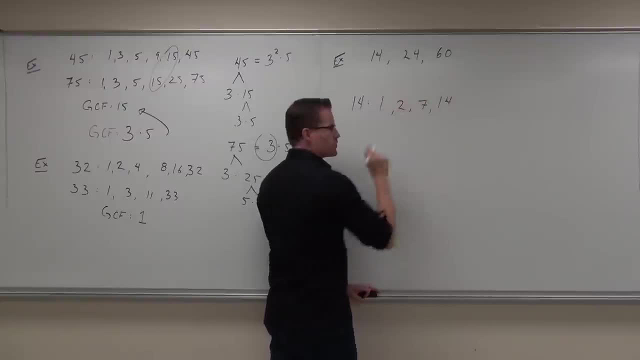 I'd have 1,, I'd have 14,, I'd have 2, and I'd have 7.. Would we agree? those are all the factors. Yes, Okay, To be a greatest common factor of three numbers. do you get that? they have to go into all three of them? 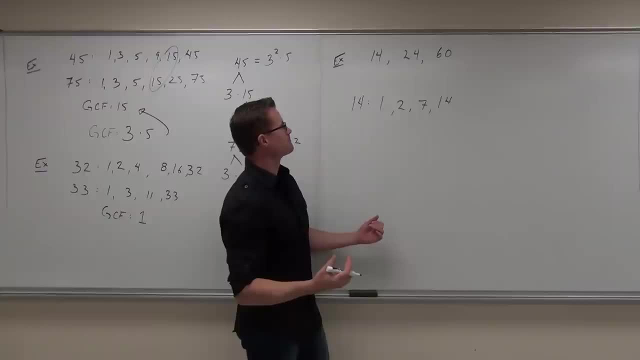 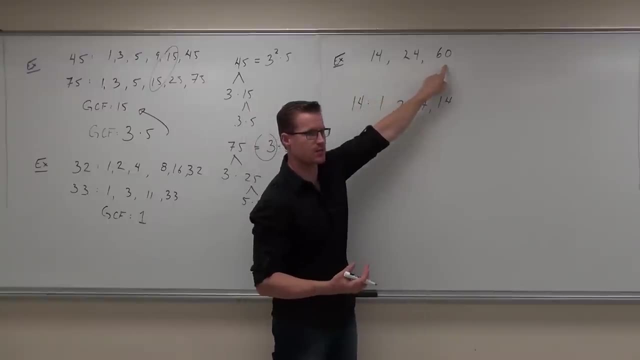 Yes. So if I'm let's see like here, 6 goes into both 24 and 60, doesn't it? But does it go into 14?? No, It can't be the GCF, It's got to go into all three. 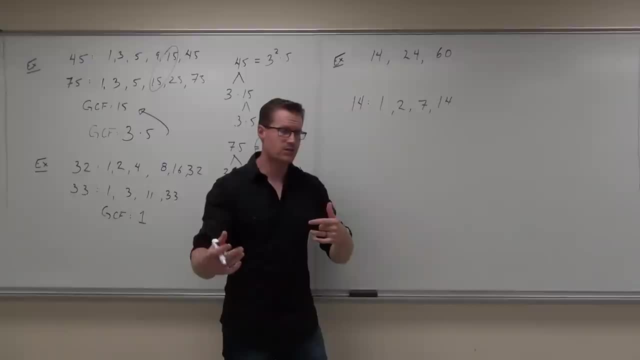 So if you pick the number with the least number of factors, sometimes you can cheat a little bit. 1,- do I care about 1? No, Okay. 2. Does 2 go into 14? Yes, Obviously. Does 2 go into 24?? 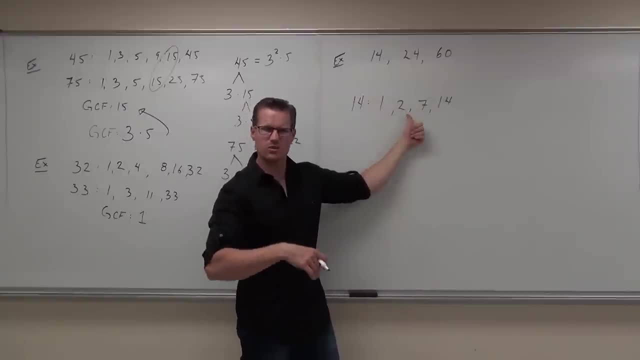 Yes. Does 2 go into 60?? Yes, Potentially. that's it. Check the other ones just to be sure that there's nothing bigger. Does 7 go into 24?? No, 7 goes into 21,. it can't go into 24.. 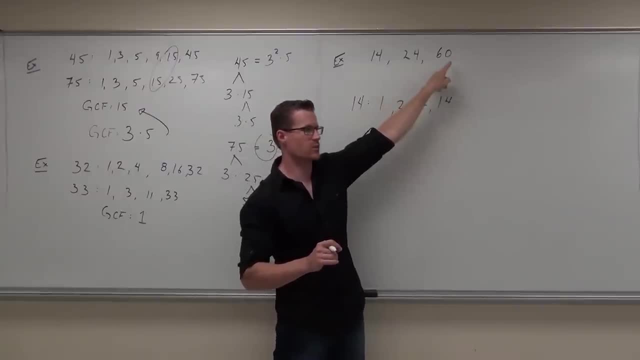 Does 7 go into 24? No, Do we care if it goes into 60 once we've determined it doesn't go into 24? No, So this doesn't matter. Does 14 go into 24? No, You have quickly found the GCF just by the process of elimination. 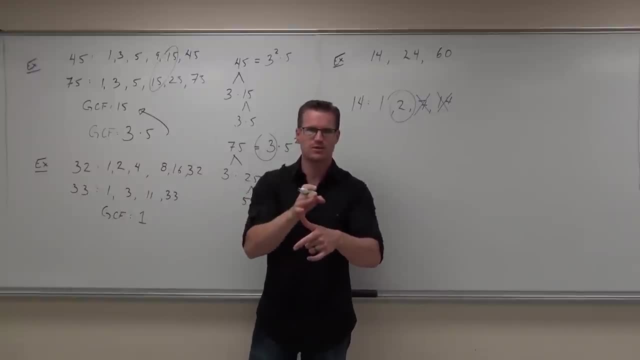 Pick the one. pick the number that has the least number of factors. Just check the factors. If they don't go into both numbers, then they're not the GCF Show of hands. if that made sense to you, Could you have done it this way and listed them all? 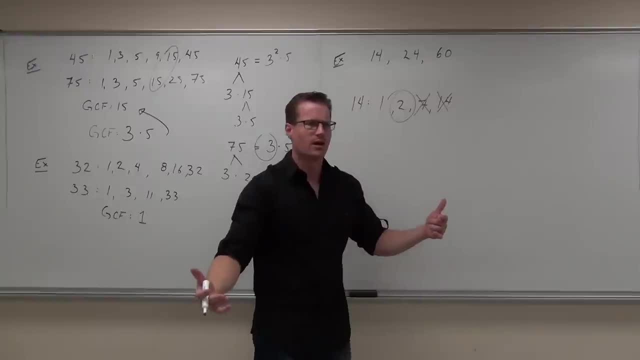 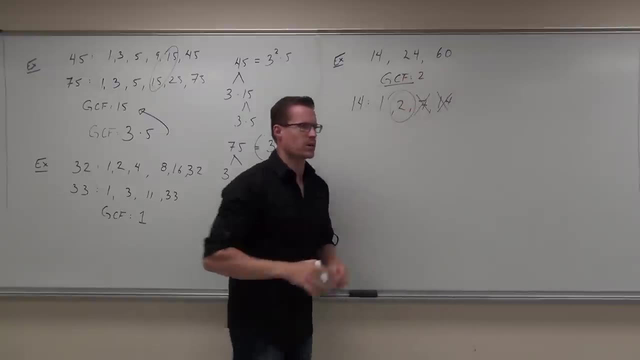 Absolutely. But I'm trying to save you guys some time. I'm saving your lives. right, Lives are time. I'm saving your lives. So the GCF for these ones, just a very quick way to do it. Okay, I kind of previewed this a little bit in the example that was right here before. 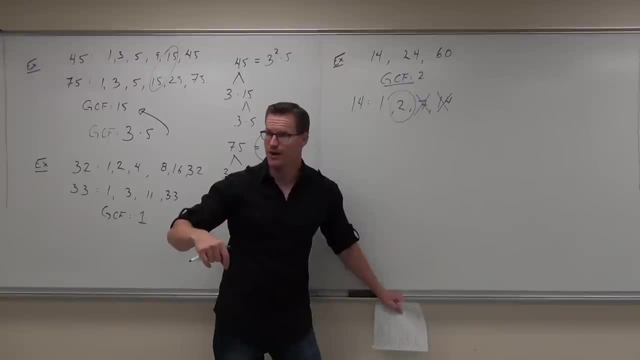 We're going to talk about variables, and then we're going to put all this stuff together and learn how to factor. Are you ready? Yes, This is like. this is the good stuff. So here we go. Next example: let's talk about the variables. If I wanted to find the GCF: GCF of x squared x to the fourth and x to the fifth. GCF of x squared x to the fourth and x to the fifth. For those of you who get this idea already, this is a really easy question. 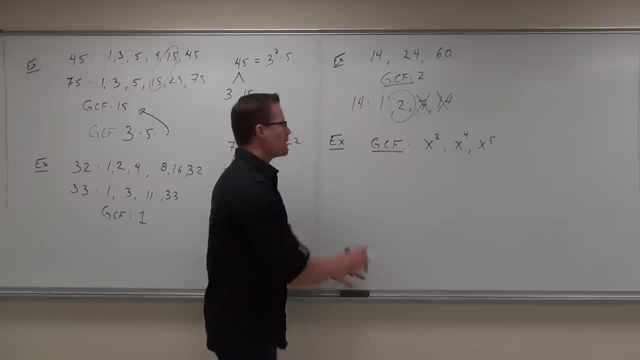 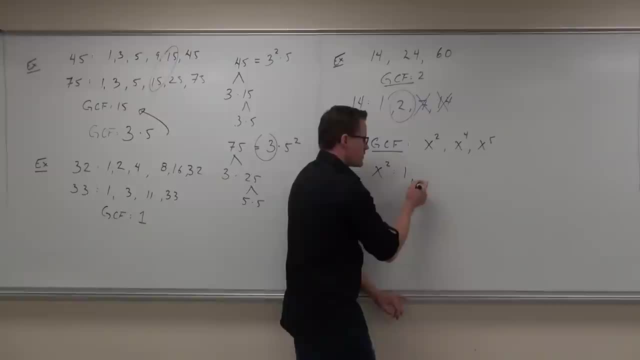 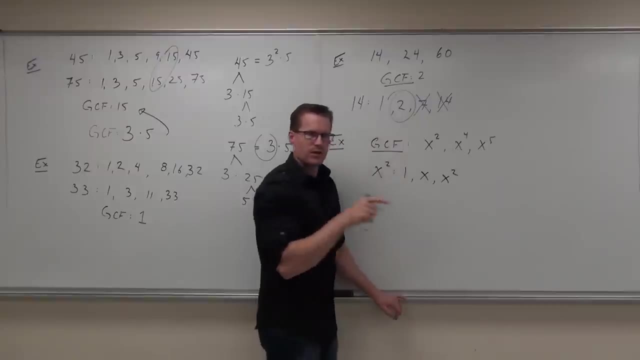 How would I do this? Well, there's always a one, But then I'm just going to have all the powers leading up to my largest power. That's what I'm going to have. Let's look at this real careful. Do you understand that? one's always a factor. 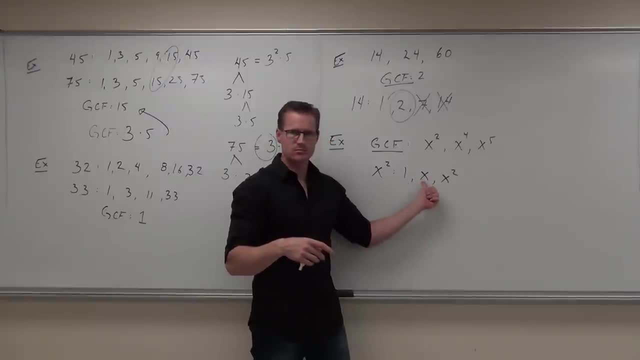 Yes, Always divides everything. Is x a factor? It's a power of x less than two. Is x squared a factor? Of course it is, Because one times that gives me this This term, If I'm going to do x to the fourth, well, I'm just going to have one. 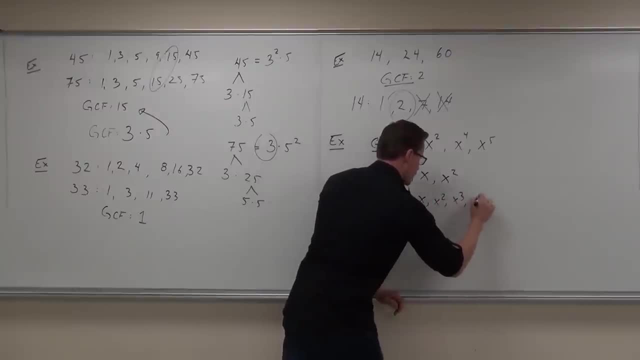 But I'm going to have x and x squared and x to the third and x to the fourth, Every power leading up to x to the fourth. If I do x to the fifth, I'm going to have one and x and x squared and x to the third and x to the fourth and x to the fifth. 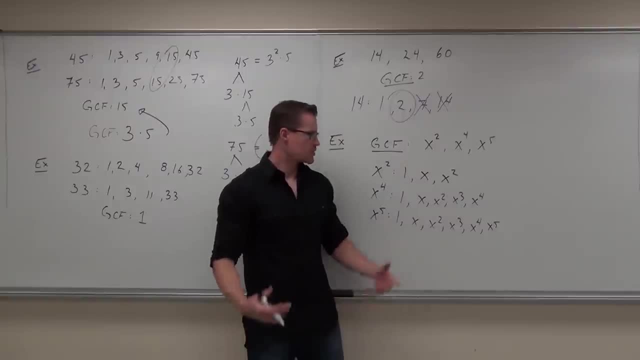 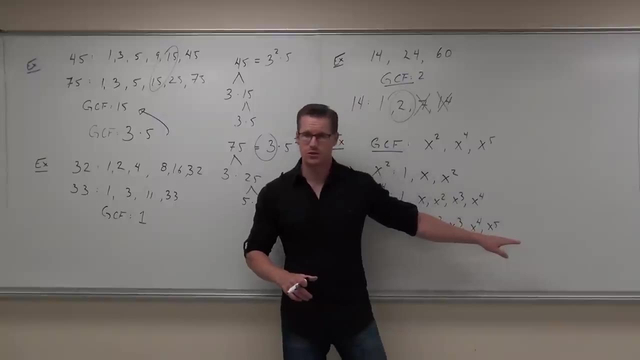 I hope so. Did I do it right? Okay, Then here's my question: Do we have any shared factors? Is it x to the fifth? No, I'll tell you what a lot of students, when they're first learning this, they look at it and go: oh yeah, x to the fifth, it's the biggest number. 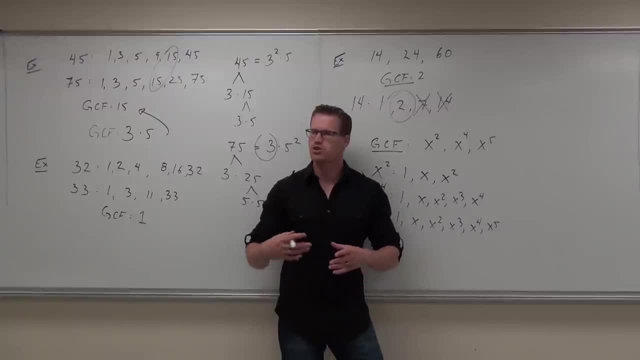 It's the biggest one. Obviously, that's going to be it. It's greatest, No, Greatest shared. So all of these have at least x squared, correct? Yes, Well, that's really what we're looking for. We're looking for all of them have at least this much. 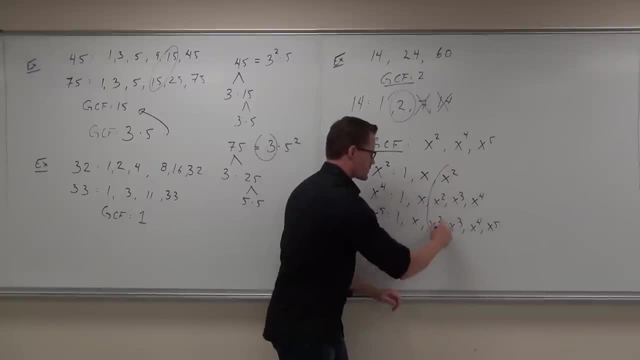 If you look here, the biggest one that's actually shared is right there. I don't care that. that's x to the third and it's shared there. I don't care That doesn't have it. so it's not the greatest common. 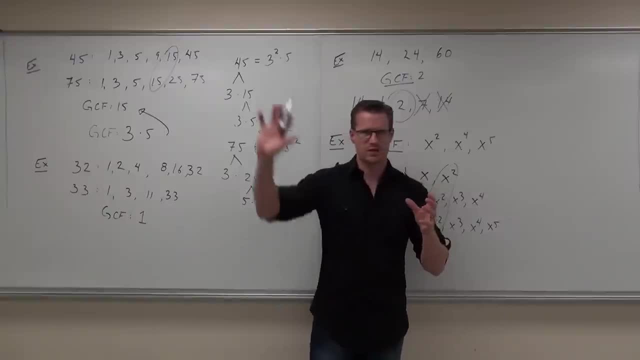 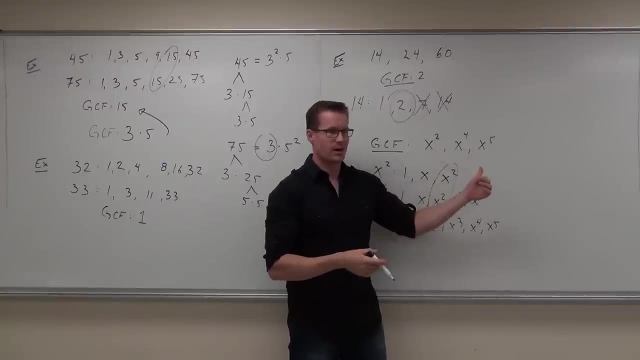 Common means shared, The greatest common factor. That's what we're looking for. Show of hands. if you feel okay with that idea, Cool. So in our case it becomes really easy. You look at these ones well, I know it seems funny, but take the smallest power. 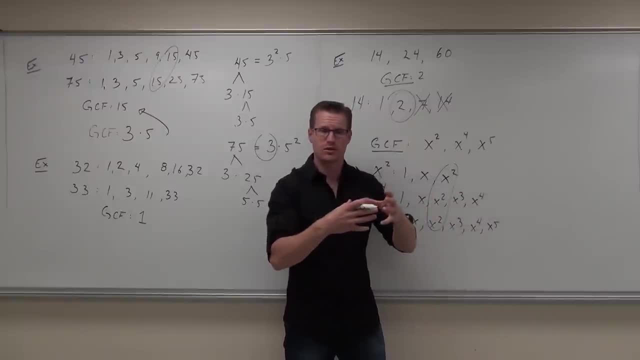 If you take the smallest power that's listed right here, that's the shared. That's the one that's shared. You can't do x to the fifth because that doesn't have x to the fifth. It has, by the most x squared. 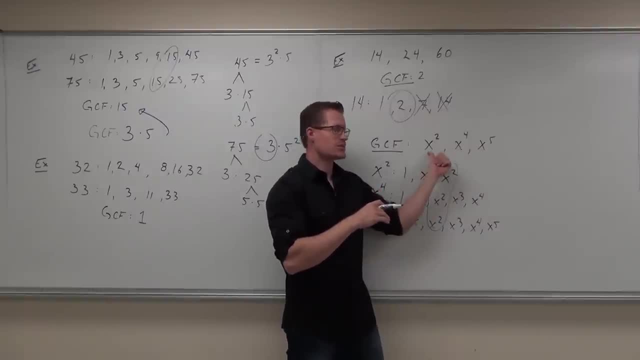 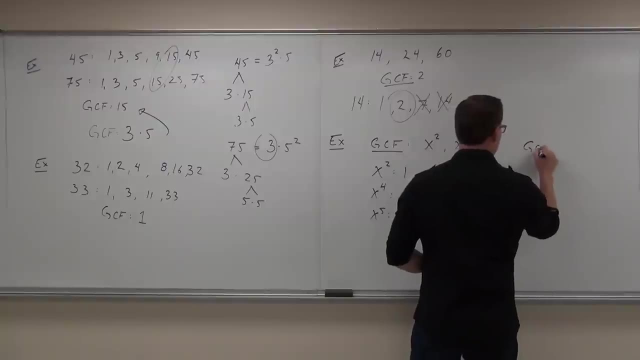 Does this have? this has x squared. yeah, Does this have at least x squared? Does this have at least x squared in it? Then that's your question. So, gcf, here would be x squared. I want you to try one. 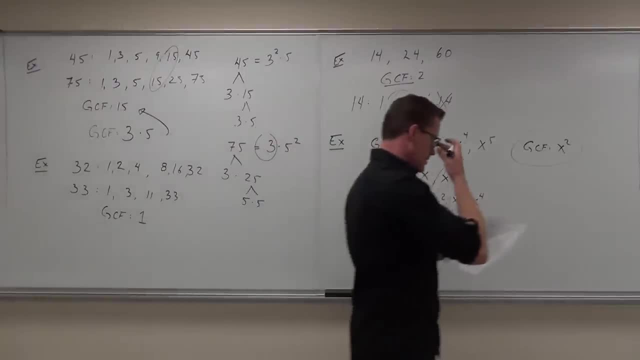 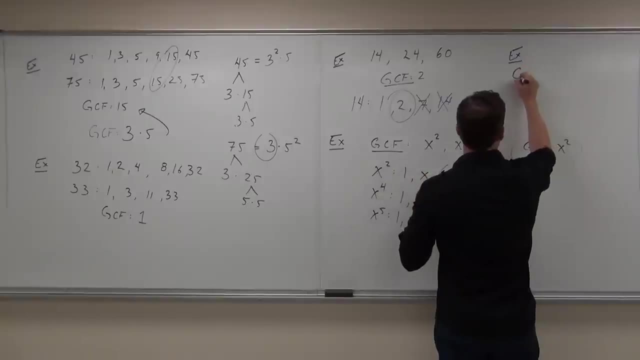 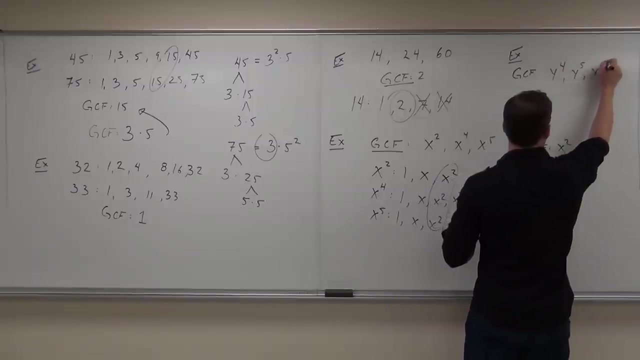 Just real quick, to make sure that you all get the hang of it, Let's do a couple examples. What I want from you is I want the gcf of y to the fourth, y to the fifth and y to the eighth, And then I want the gcf of x. 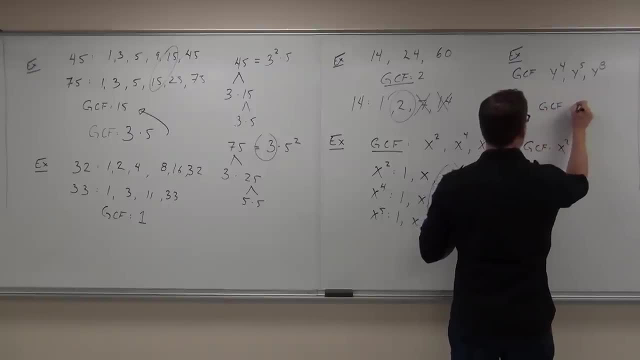 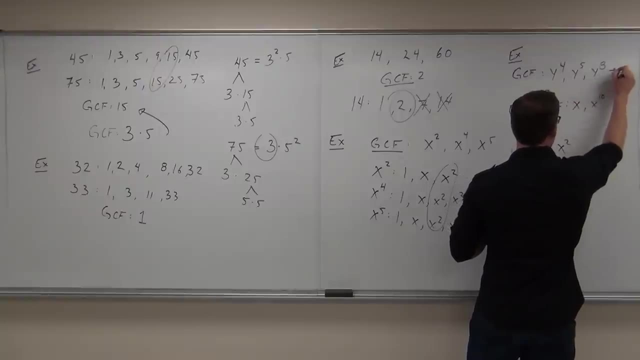 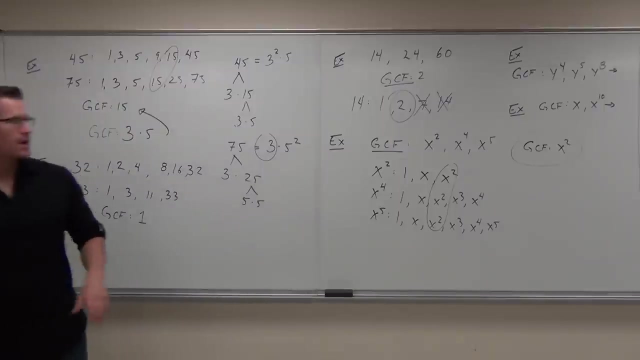 And then I want the gcf of y to the fourth, y to the fifth and x to the tenth, And you can just write it right next to this. If you need to list out all the factors like I did here, do it until it really makes sense. 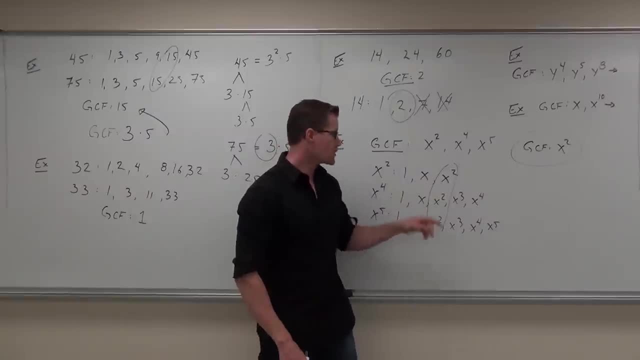 Don't do shortcuts right now, because this is imperative. you understand this. So if you need to list them out, list every power of x up until that number. List every power of x. List every power of x up until that number. Look for the biggest one. 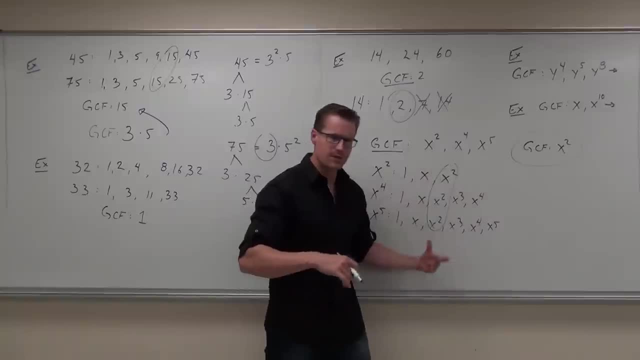 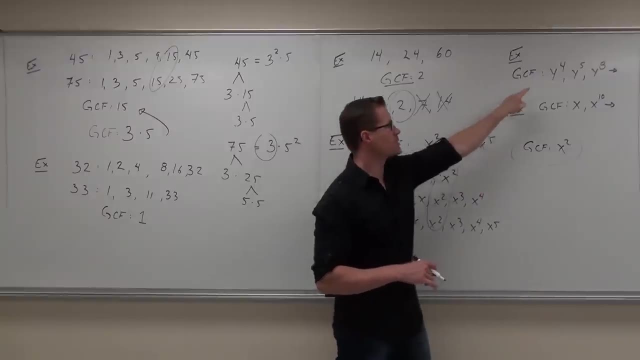 That's your gcf. You can do that every time. Once you understand this concept, though, you can go very, very fast on that. Does anyone need more time on these? Have you figured out the gcf for y to the fourth, y to the fifth and y to the eighth? 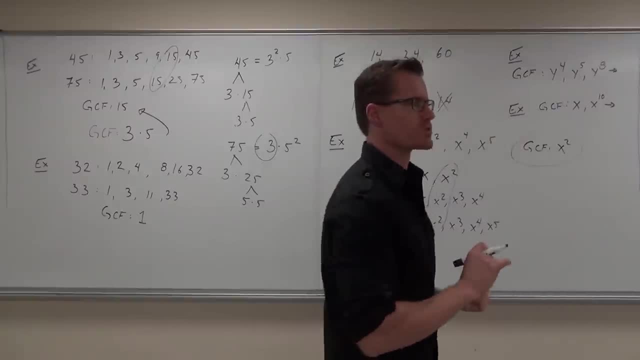 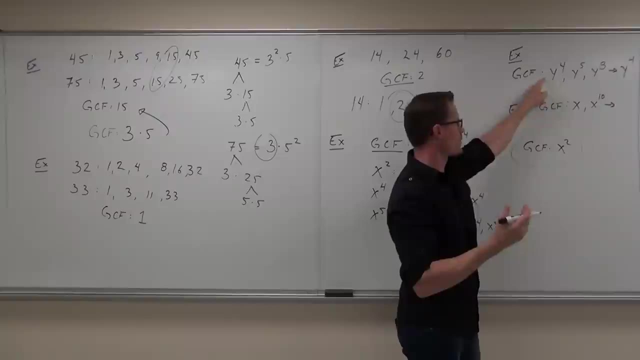 What's the biggest power that's shared by all three of those terms? What is it? Y to the fourth- Perfect, That's right. You can't go any bigger, because that doesn't have any more than y to the fourth. It's kind of like going out to lunch with your friends. 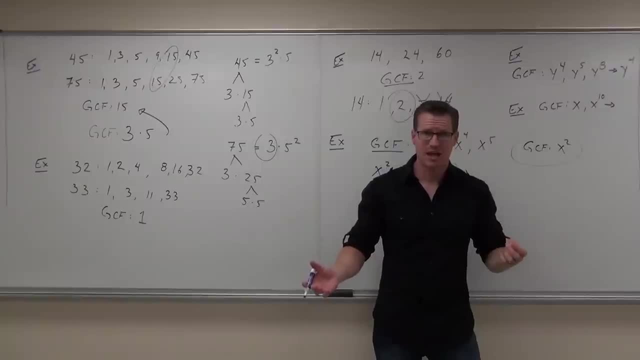 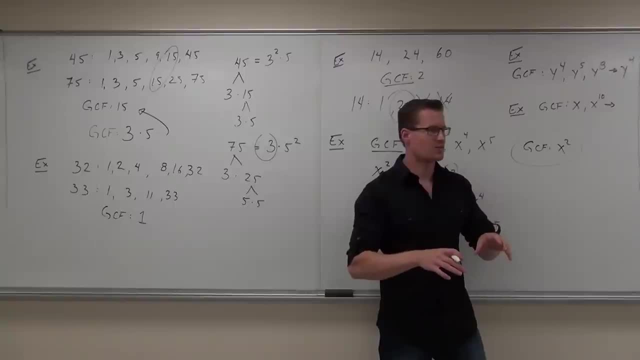 And you go: let's go to this place where it costs $5.. Can I eat? I have $4.. Can I eat? No, Let's go to this place that has $8.. Can I eat? Screw you guys, It sucks. 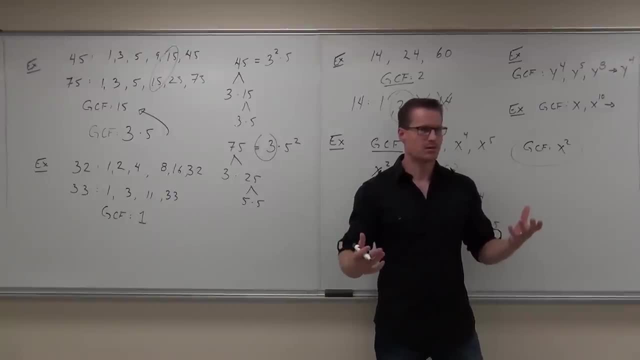 Where's everyone going to be able to eat At the $4 restaurant? That's my type of living, folks. You've got to go where everyone can eat, So go where the power. The power is shared by all, Y to the fourth. 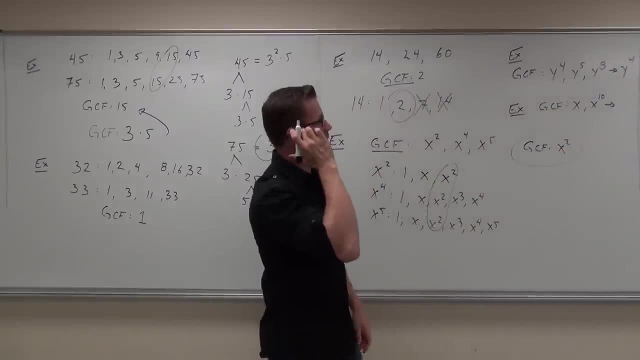 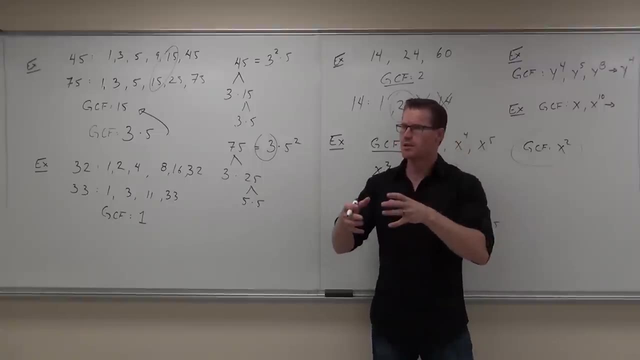 Hopefully that analogy made sense to you. How about X and X to the? Oh wow, How many X's are here. What power of X is that One? X to the tenth? What's the greatest common factor? X. You can't go any bigger than that, because this guy only has $1. 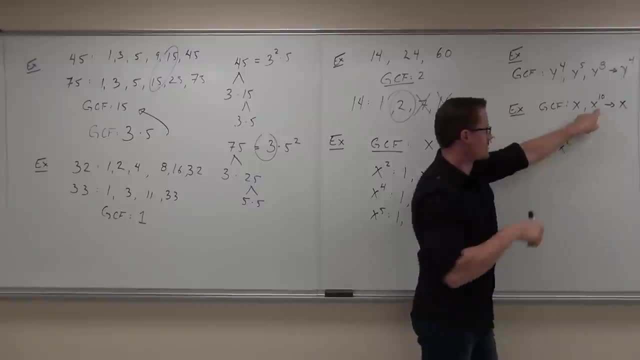 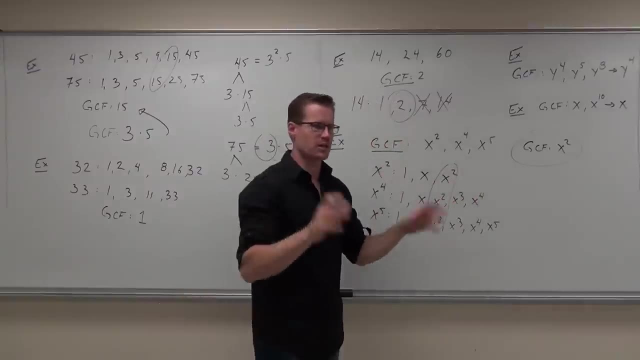 Poor guy. That's it. That has more, sure, But you need to go with the largest factor that is shared by all the terms that are listed. Have I explained it well enough for you guys to understand it? Now we're going to put the idea together. 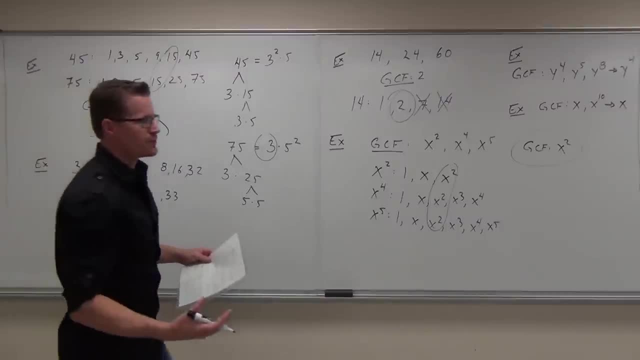 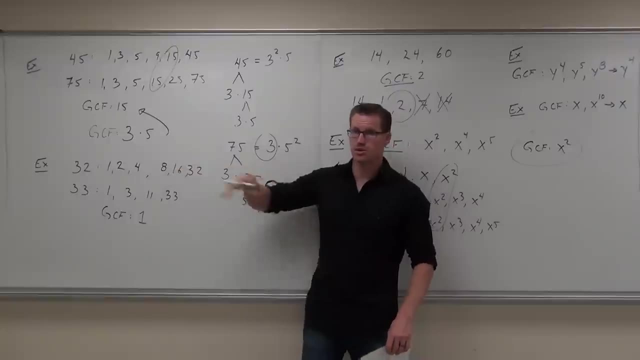 We're going to talk about the greatest common factor of these terms. that involve both numbers and variables, but it's no different than what you've done. Did you guys get the numbers? Did you get the variables? Do the same thing. You should put them together at the end. 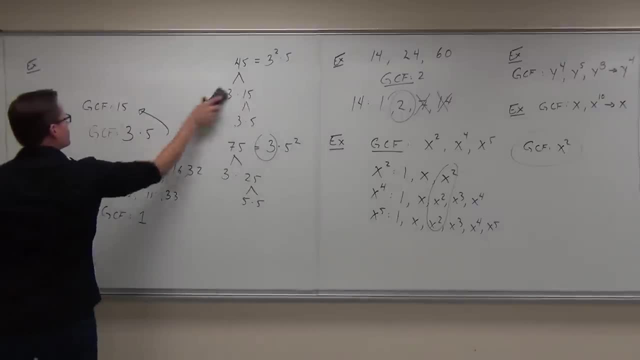 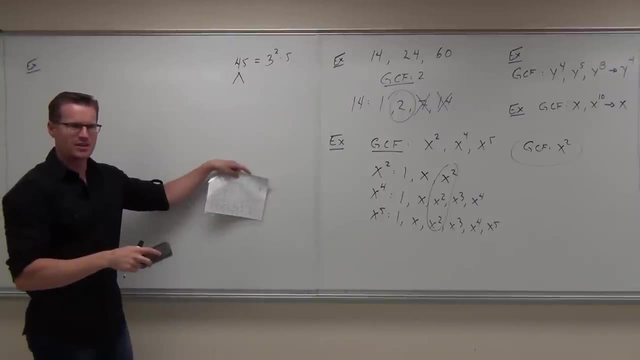 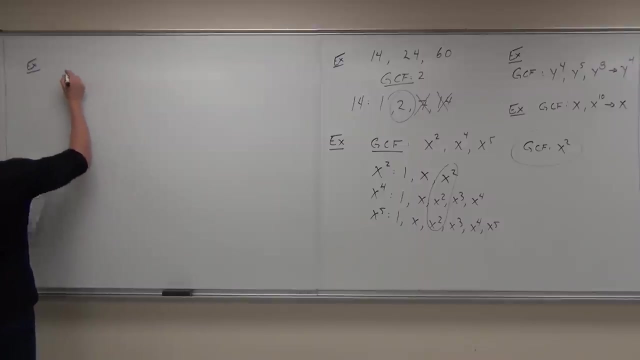 So let's talk about that real quick. Did you know about that? by the way? If you didn't, isn't that kind of neat Works every time. It's really awesome. I like it. So we're going to find the GCF here. 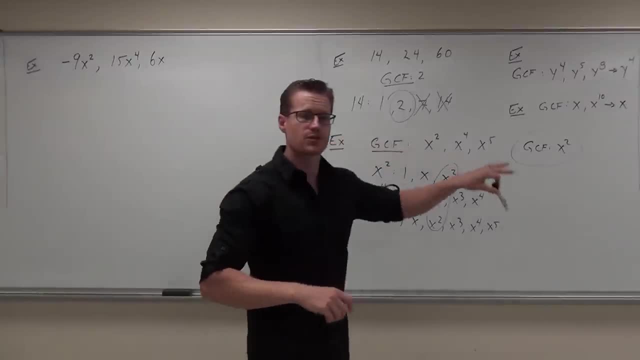 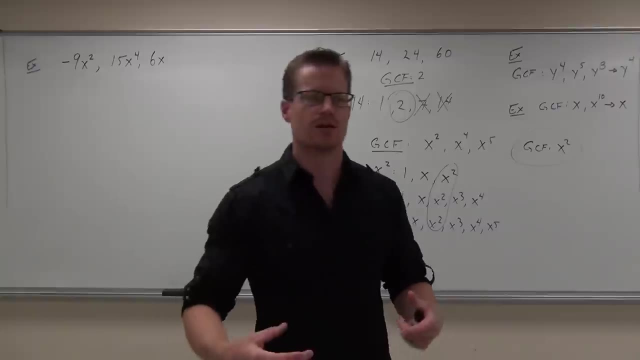 I'm going to stop just writing out all the factors. We're going to get to the point where this is going to be very easy for us to do in our heads, because we're so good at doing factors and numbers and listing factors in our heads and variables. 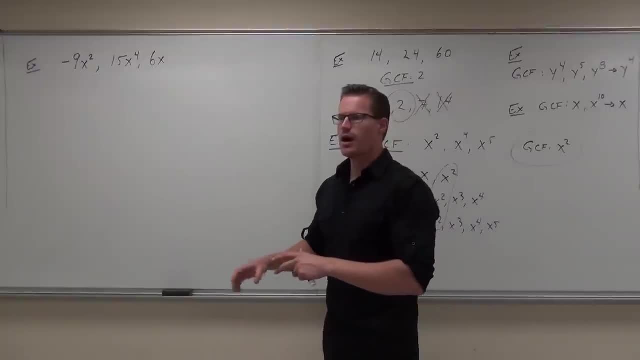 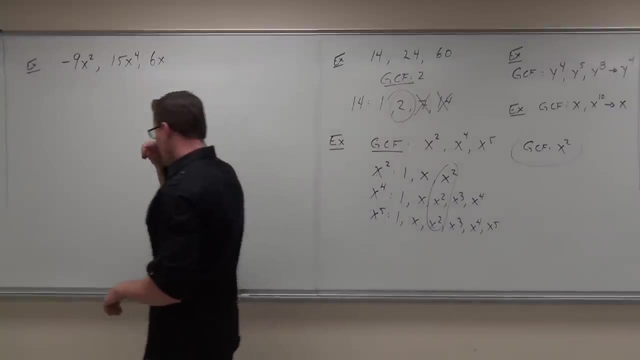 So we're going to stop listing out everything. It's going to take way too long And the idea is get the greatest common factor quickly and then use that to factor. We're going to be doing that in a minute. So what I want you to do here, when you're factoring out the greatest common factor, 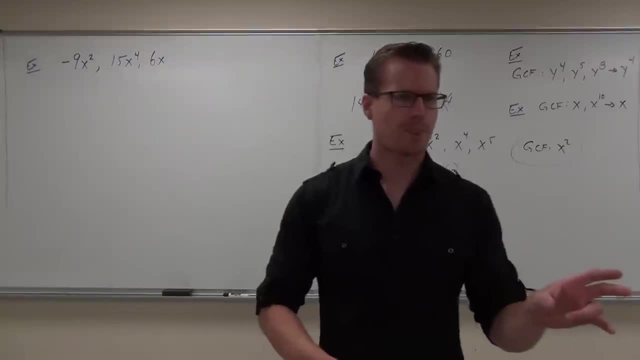 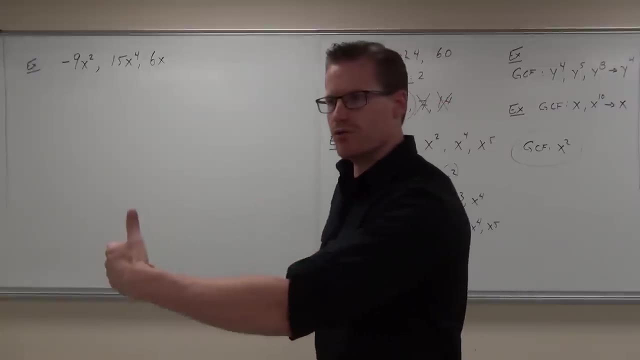 when you're looking for the greatest common factor, do the numbers first, then do the variables and just combine them. So I remember that we had an example like that, right, It kind of cheated and went in advance. I'll do that from time to time. 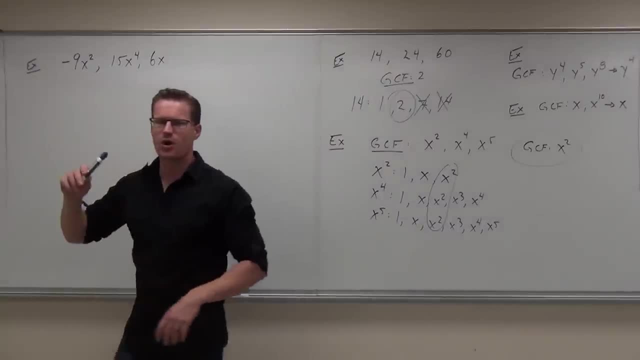 Let's look at the numbers. The numbers here are: what are the coefficients? What are the coefficients? The coefficients is what they're called. What's the coefficients? Negative 9.. Negative 9 is one of them. Someone else? what's another coefficient? 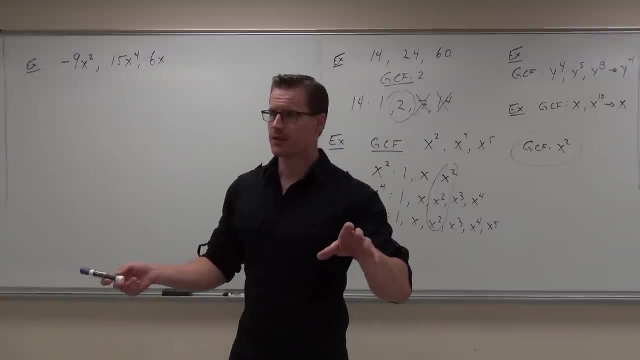 15., 15. And then is there a number that goes into all three of those numbers: 3.. You can always answer yes, because it's 1. I want the biggest number that goes into all three, 3. 3 does. 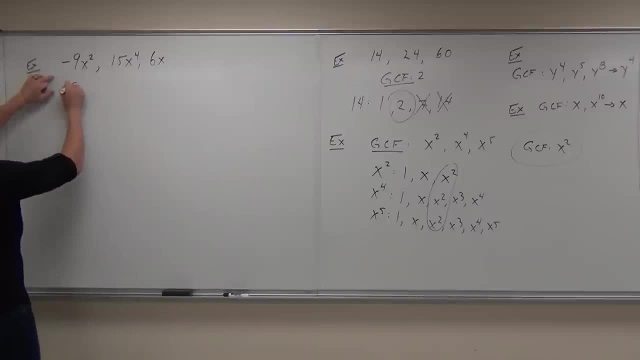 Sure. So 1 is not going to help us, 6 doesn't work. So when we write out GCF, we can do it in a two-part process. We do the numbers first, So 3.. It's true, right. 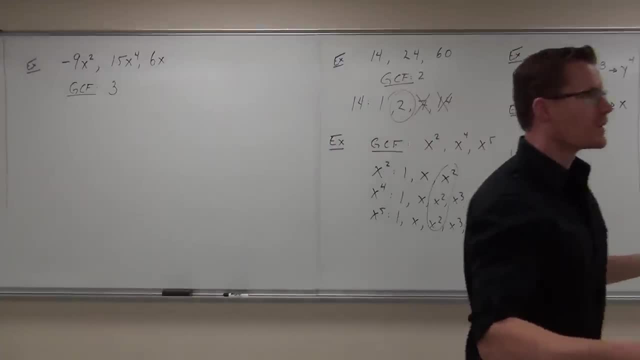 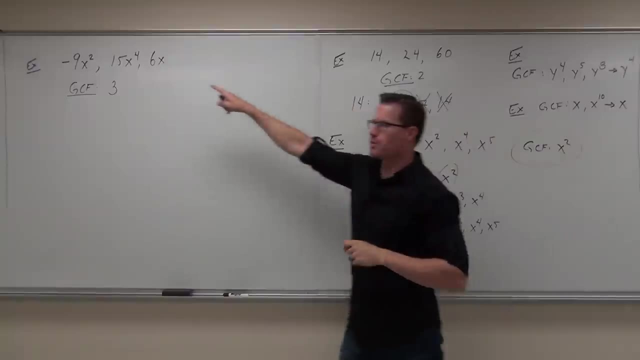 3 goes into 9,, 15, and 6.. We're good And then we do the variable. So when we're looking at the variables, it's basically doing this process first, exactly the same. Just like we got the 2,, we got the 3.. 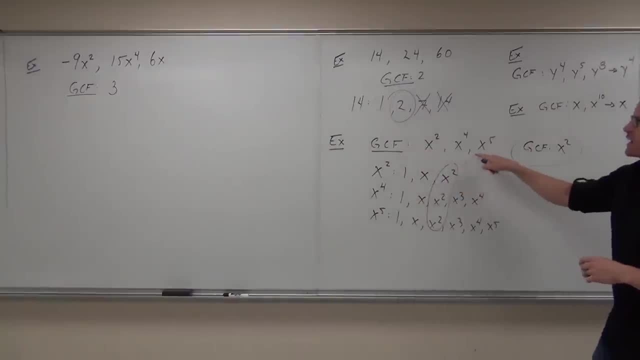 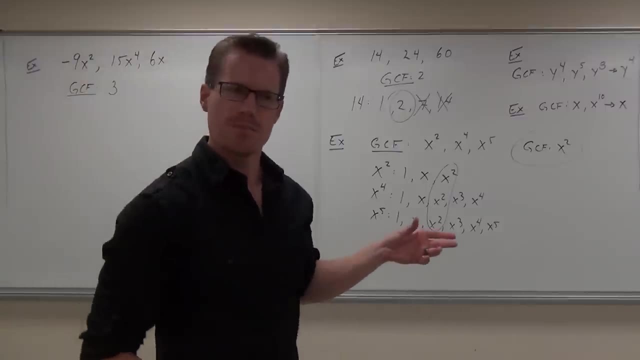 Do the same thing, Then do the variables, Just like. we got the x squared here, or the x. What's the greatest common factor, as it refers to the variables? in this case, What is it? x, That's right. That's got more. 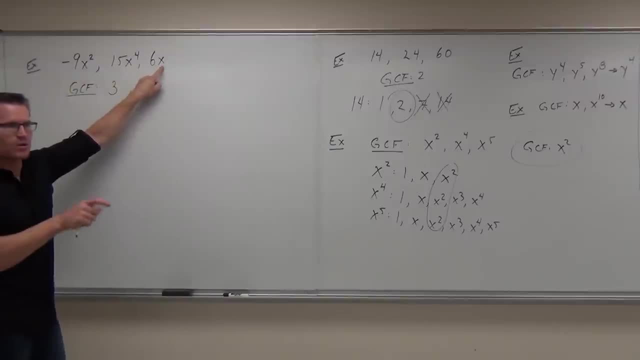 That's got more, But well, that's the smallest one. So we have to go with the guy who's got the smallest amount of money here. This guy's only got a buck. So, yeah, these guys have at least one x, but we're going with the greatest common thing. 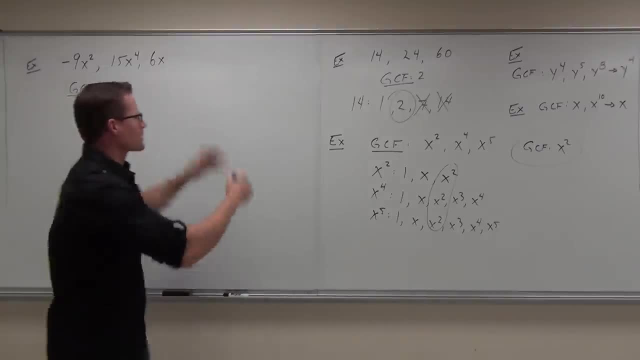 It has to be shared. So if I can list out x to the fourth, that would take this guy out of the picture and that guy out of the picture. x to the squared would. this guy would have it, but that guy wouldn't. 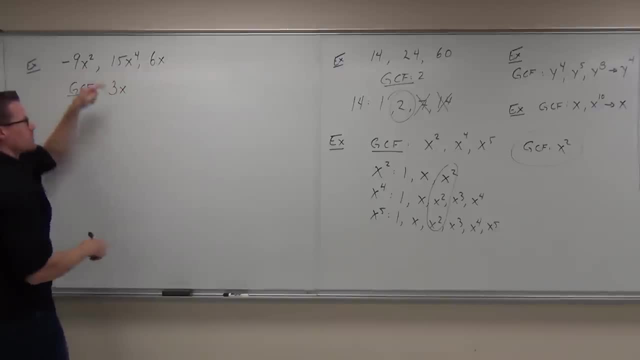 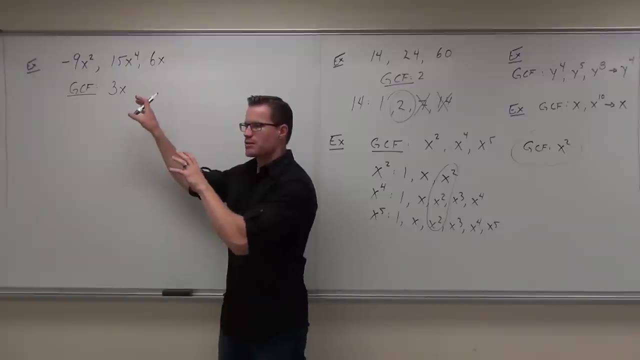 So x to the first power is, as far as our variable is concerned, the greatest common factor. What that means is, when we put our numbers and our variables together, the greatest common factor is 3x, 3x. Does 3x go into this term? 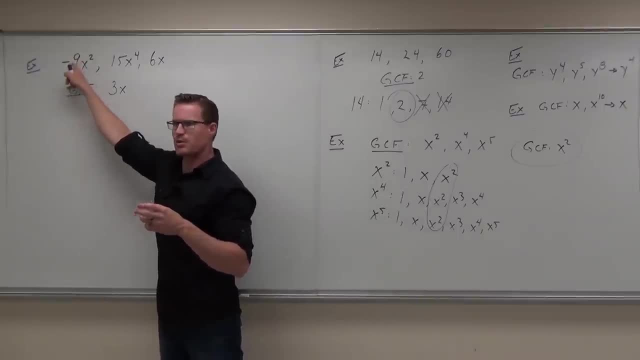 Yes, I'm sure it does, Remember it goes in means divides, because a factor is multiplication, so the inverse of that is division. Does 3x divide 15x to the fourth? Yes, Yeah, of course. Does it divide 6x? 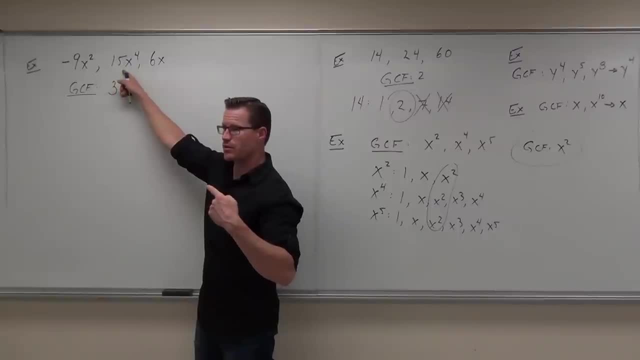 Yes, Yeah, Notice how. if this was a square, would x squared divide x? No Too big, Too big. If that was a four, would that divide? No too big. That's a problem. I think I said four and wrote two, didn't I? 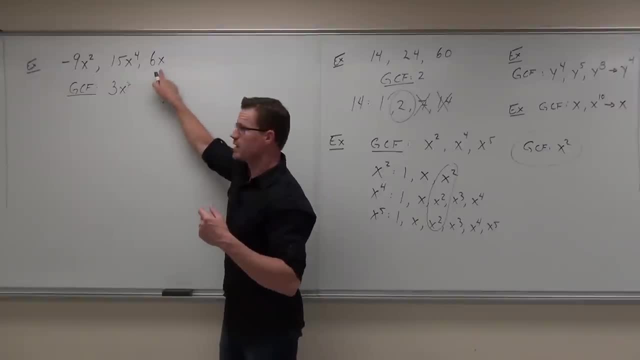 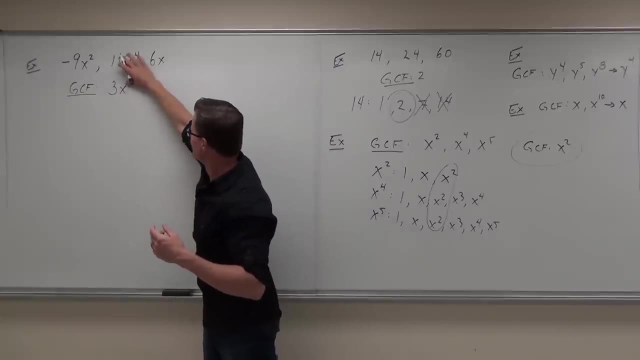 Oh well, Yeah, Yeah, Yeah, Yeah, Yeah, Yeah, Yeah. No, you said two, I did. You said two, firsts were two. Didn't write four. I got it right. Yes, Yeah, Yes. 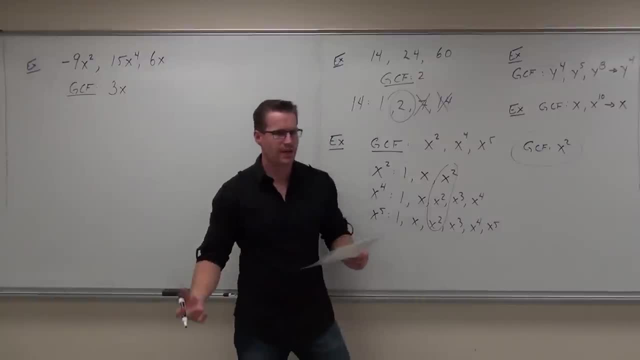 Perfect. Tell you what I'm going to do: one more with you, Kind of a more advanced one. It looks more advanced, It's not harder, It's the same exact thing. Then I'm going to have you do a couple on your own. 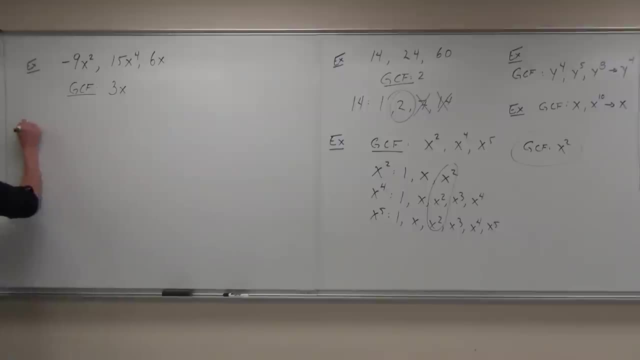 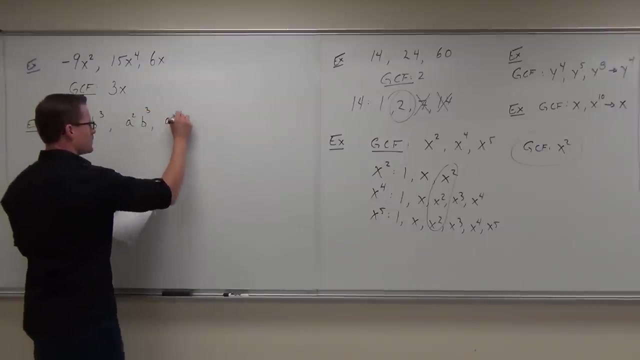 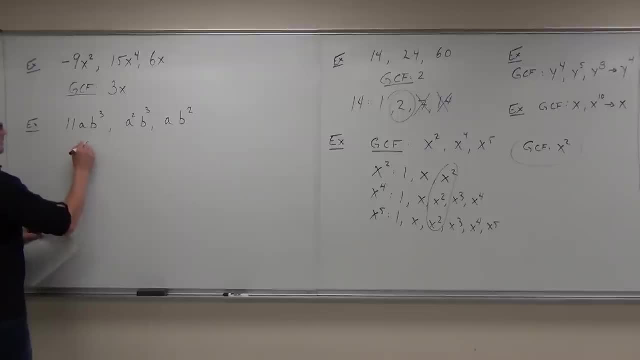 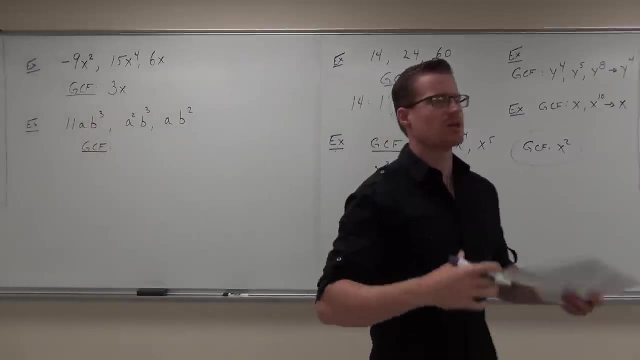 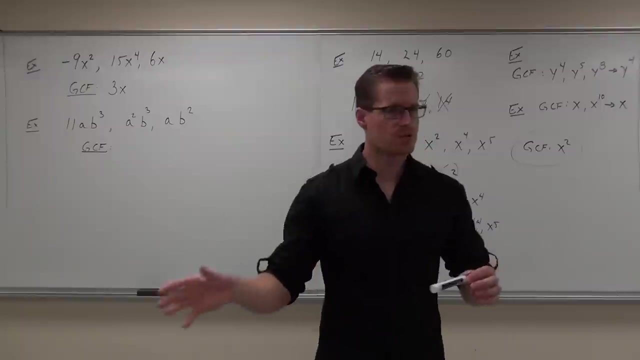 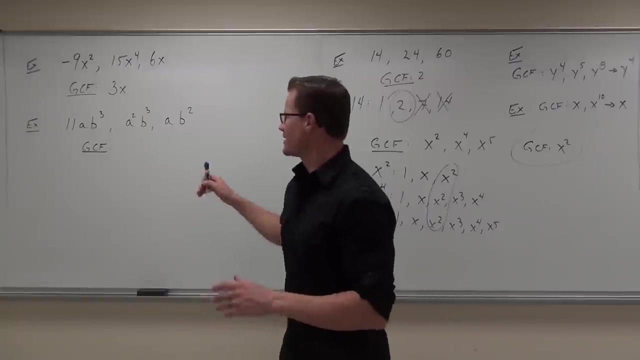 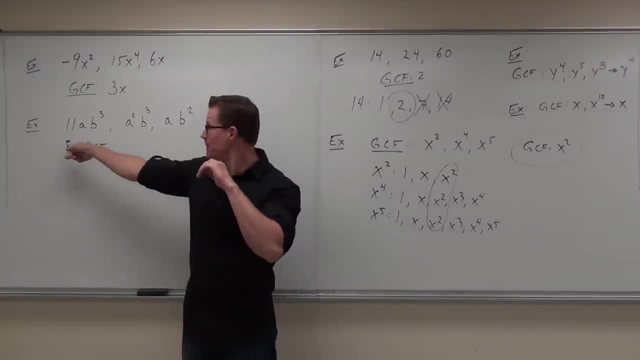 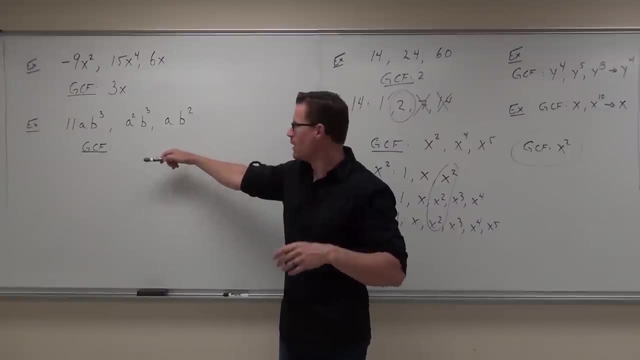 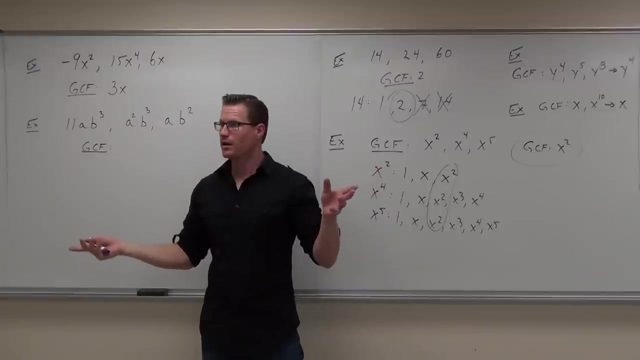 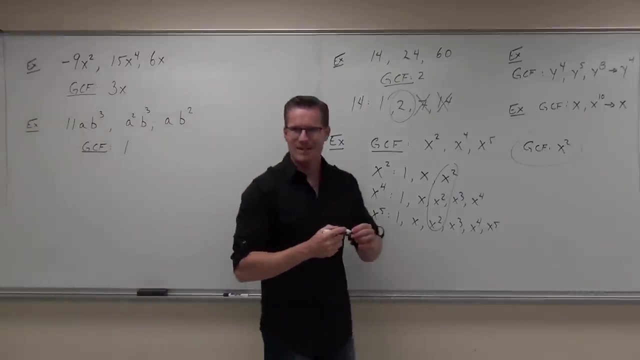 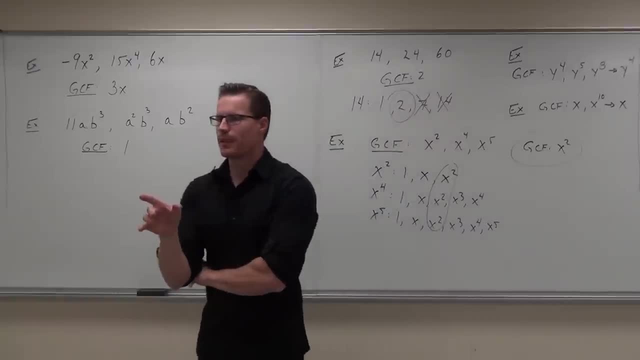 Okay, Okay, Okay. So we're gonna go over to the A's and our B's. You know what? Just like we can do our numbers independently of our variables, you can do each variable independently of themselves, because it's all being multiplied together. 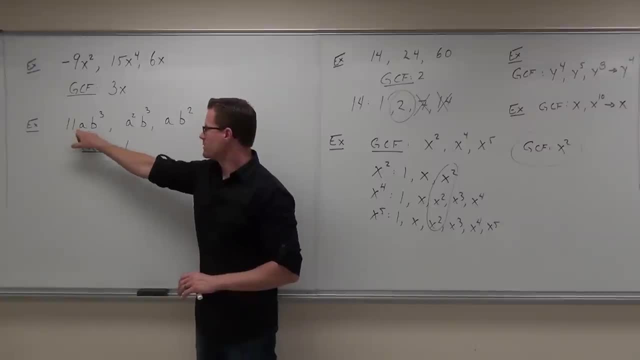 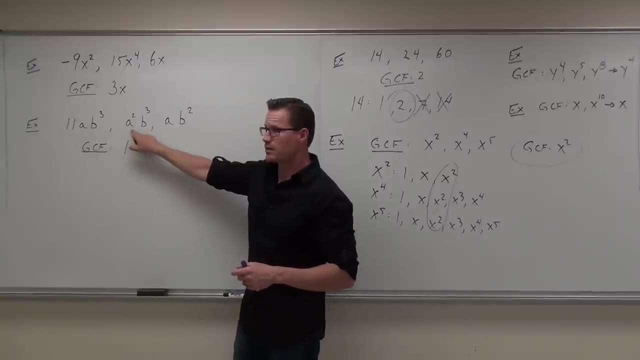 So don't worry about the B's right now. Look at the A's. I've got A to what power One? Do you know that you're done right now? Yeah, A to the second, Yeah, Okay. what's in common to you? 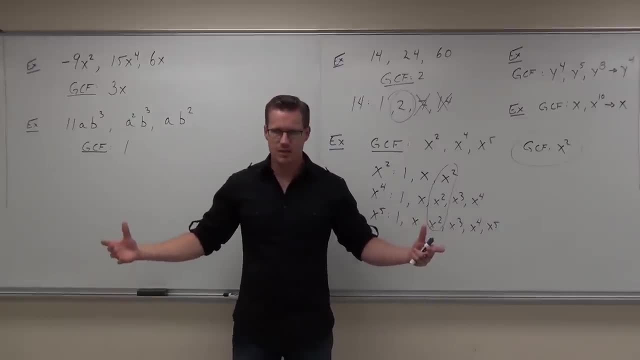 All three of those Like: A to the 1. Not A to the second, persupur城, Not a to the fourth, because I have one, two, three, four, Not that, No, no, don't do that okay. 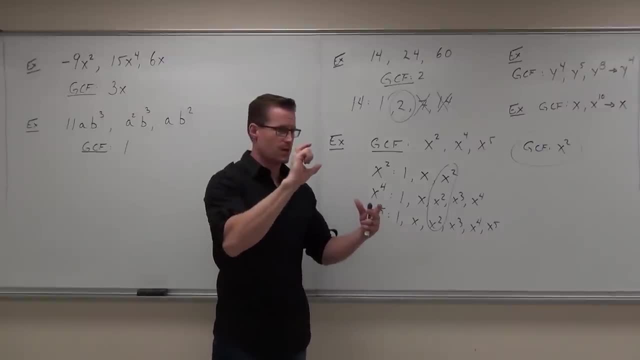 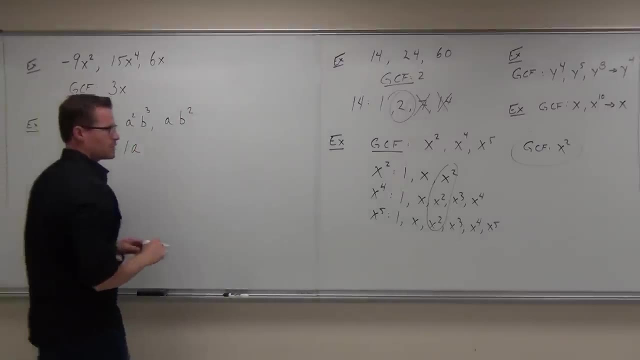 You're looking at these independently, saying what's the biggest value of a power of a that's going to go into all three, And that would be a to the first. Are you with me on this one, Are you sure? Guys in the middle, yes, no. 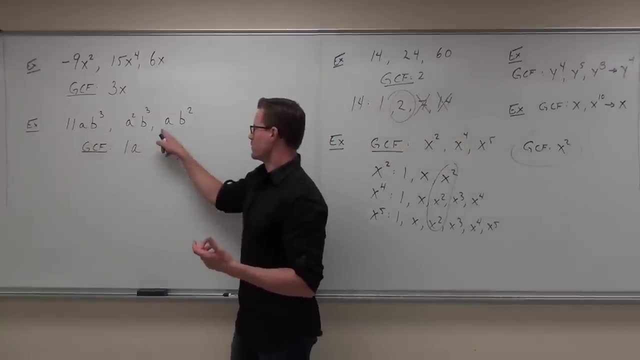 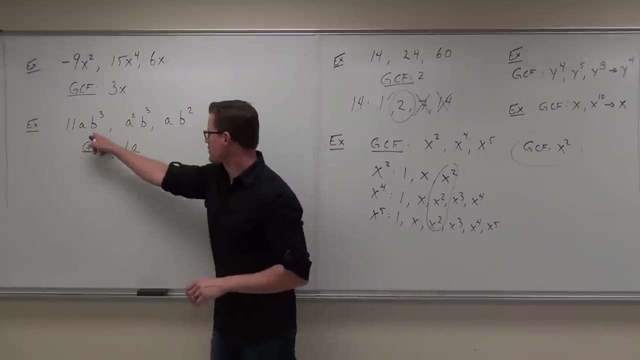 Okay, we're all good. So one goes into all the coefficients: A to the first power. well, that's the greatest common. Let's do the b. I have b to the third, I have b to the third and I have b squared. 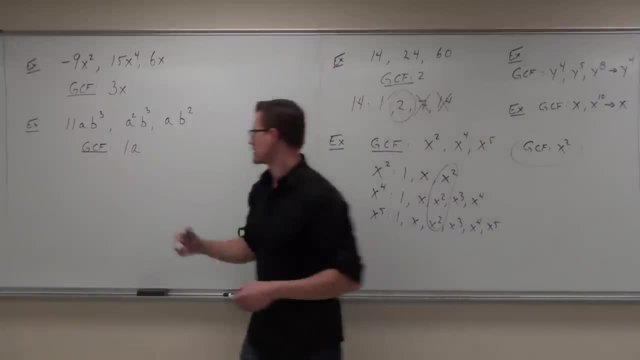 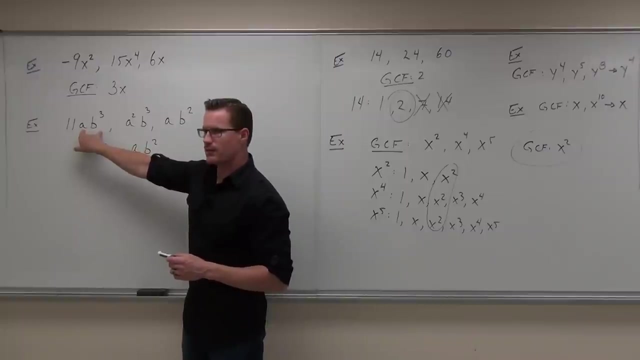 What's the biggest one that goes into all of them. Perfect Erase this one. That is our GCF. You know what? You should always check it too. You should always check it. Does a, b squared divide this? In fact, if I divided it, 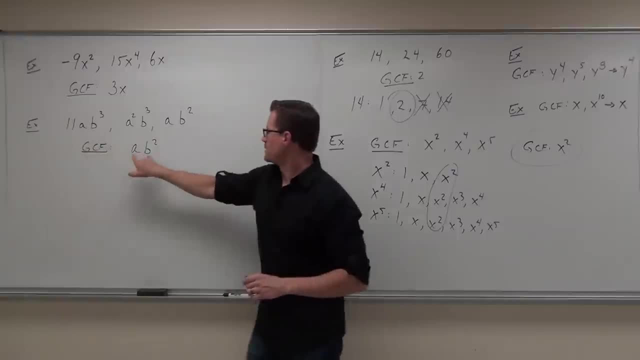 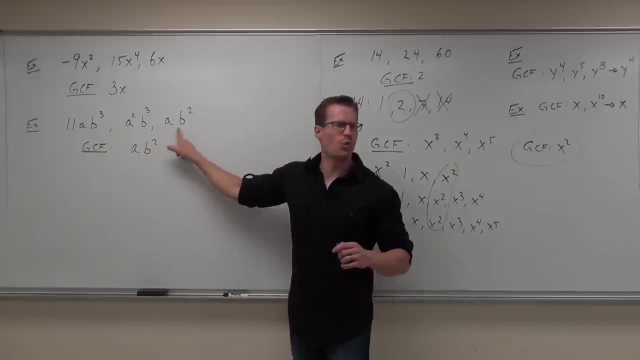 I would have b to the first power left over. Are you with me on that one? Does this divide this? Yes, I would have a times b if I divided that. Does this divide this? I would have what One One? Are you ready to try some on your own? 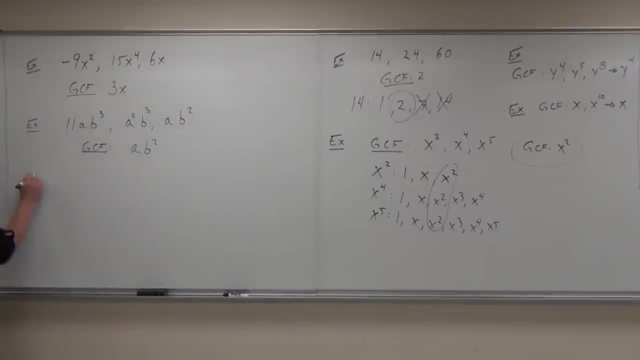 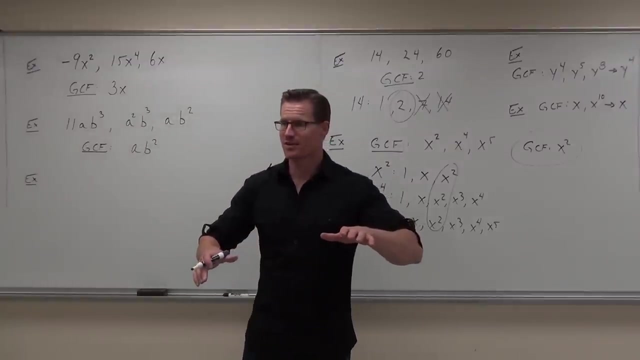 Yes, Yay, Easy, medium, hard, Medium- What do you think? Medium Medium: You're still learning it, right? Yeah, Is it going to take practice? Yes, I bet you it's going to take some practice. 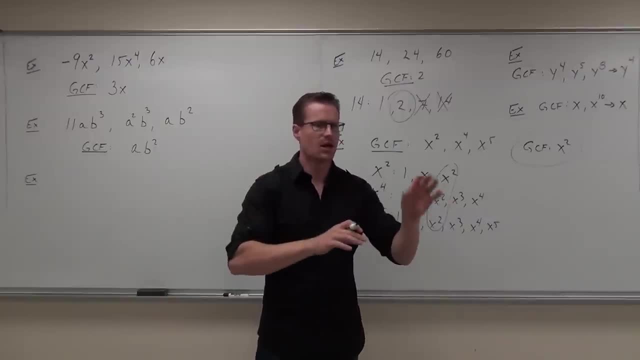 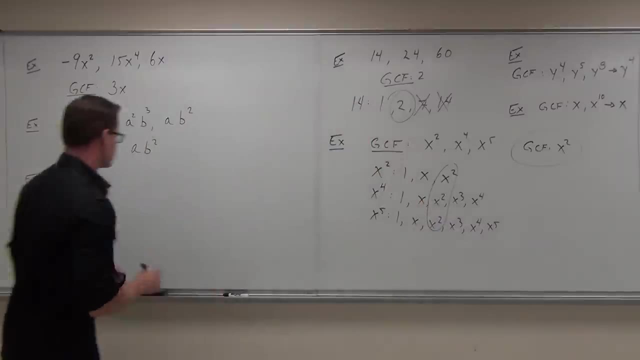 Do the numbers, Do the variables. You can do each variable independently. Just don't start picking the biggest power that you see. That's a problem. Pick the biggest power that's shared by all of them and you get it right every time. 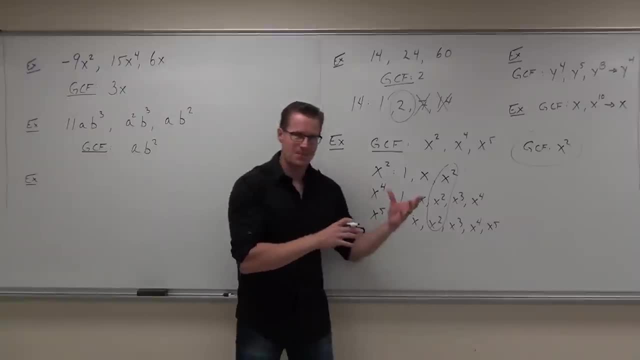 I hope you understand that doing this, doing this- is so important for what we're going to do next, because you can't factor unless you know how to find the greatest common factor. I mean, it's right there. You've got to know how to do it. 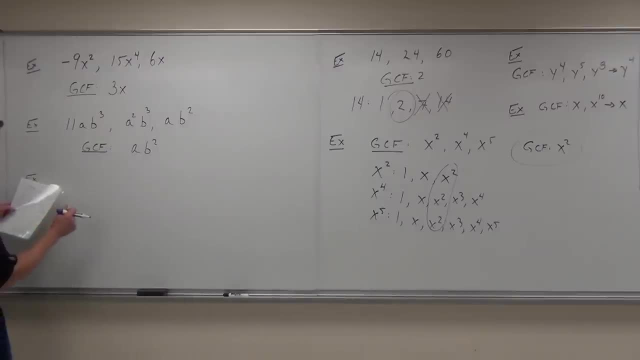 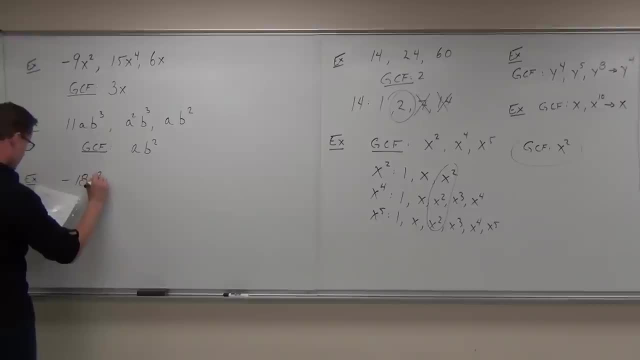 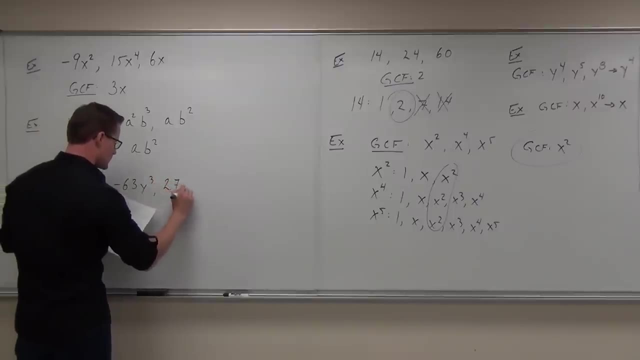 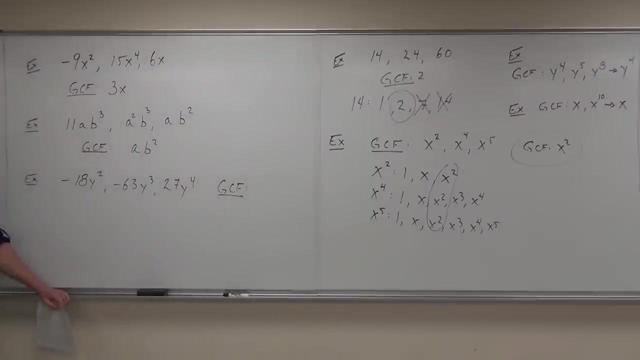 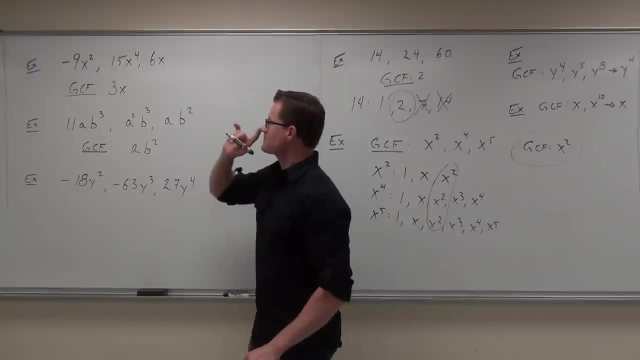 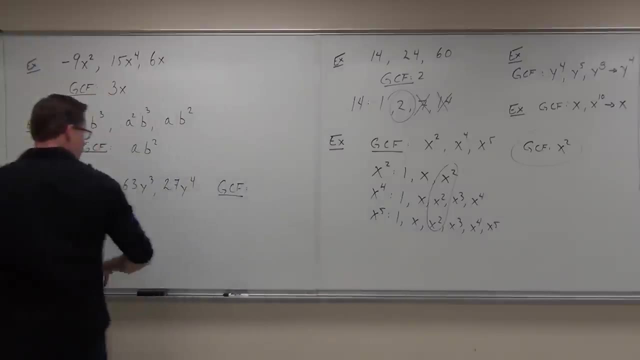 One thing I want you to look at here. Did you notice how that negative had nothing to do with what that was? It's interesting, right, Okay, And we'll talk more about how to use that to your advantage when we actually get into factoring. 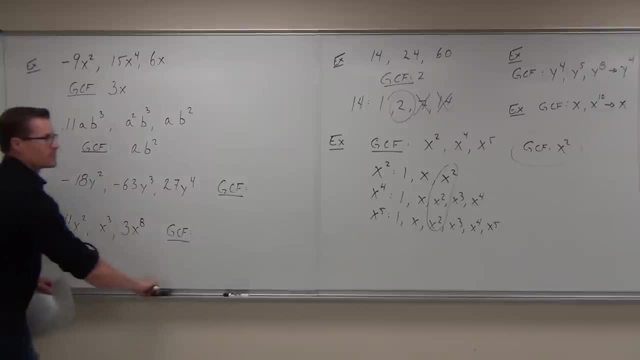 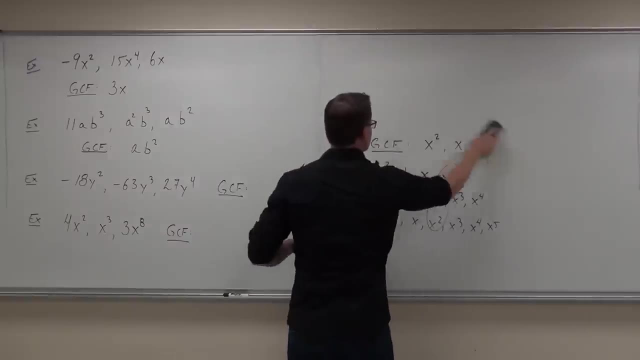 So I want the GCF here, I want the GCF here, And I'll give you one more just for funsies. And I'll give you one more just for funsies, And I'll give you one more just for funsies. 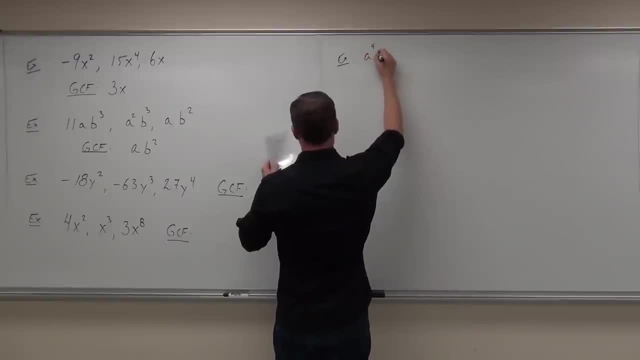 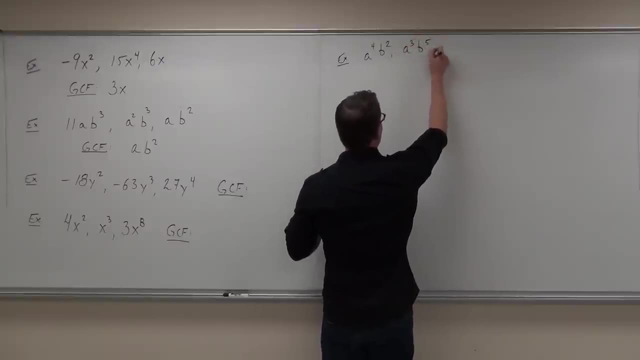 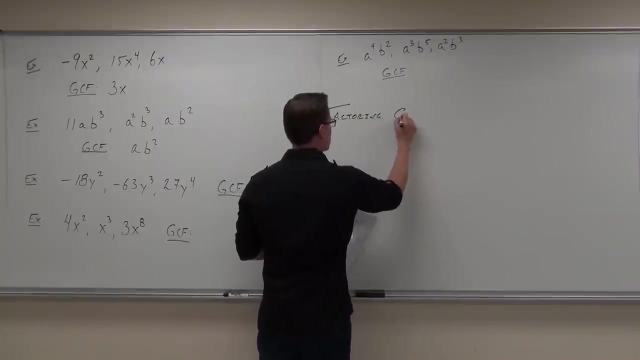 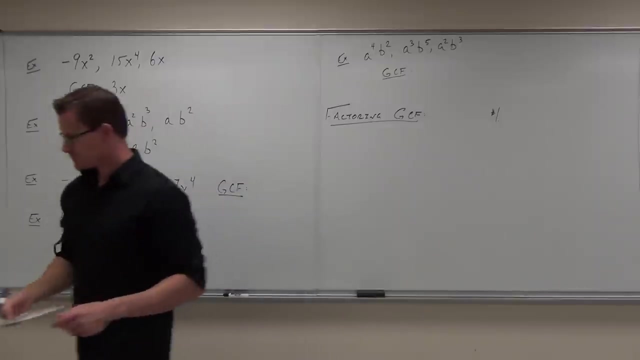 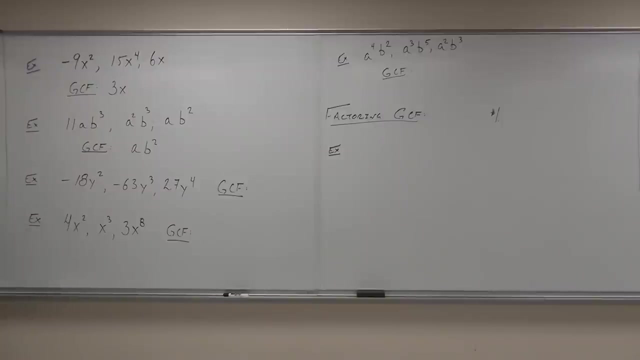 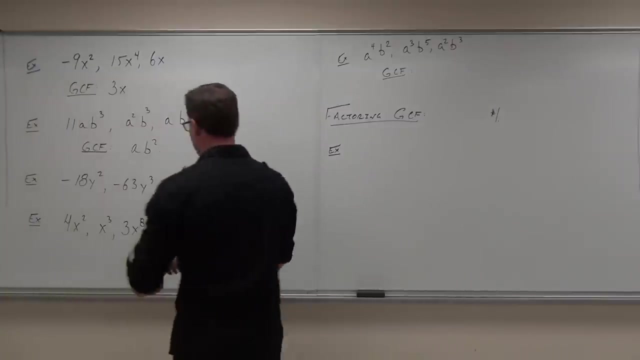 Actually, some of you might be done, just have to write them down. huh, They can go pretty quickly. They can go pretty quickly. Oh man, let's look at the first example. Have I given you enough time to complete these, or at least do the first two? 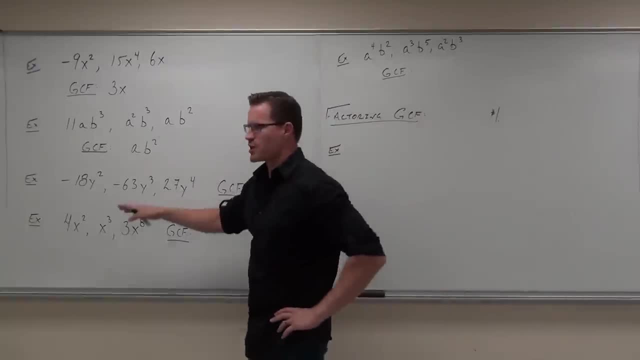 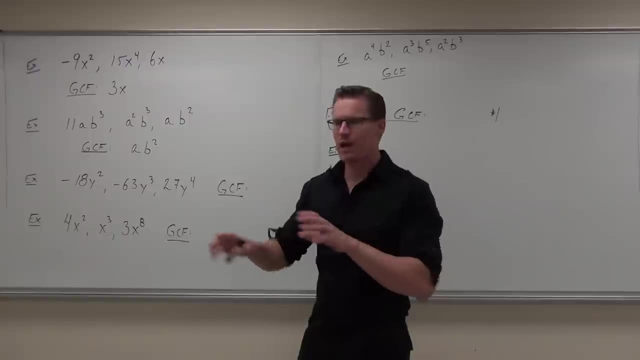 All right, first example: what should we do? Should we look at all of this or just the numbers? first, The numbers Eighteen. do I need to worry about the negatives When we're factoring, when we're actually factoring? I'll show you how to do that appropriately. 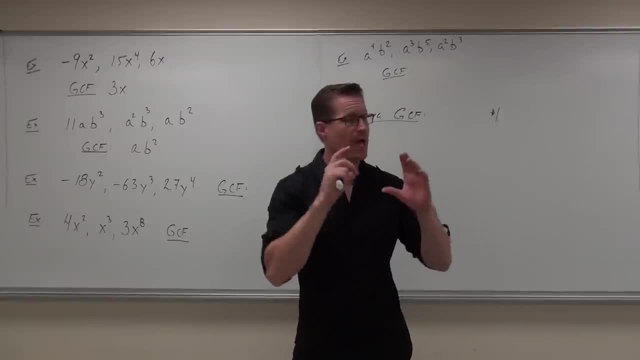 But right now, no, It's not going to affect the actual absolute value of what you factor anyway. So eighteen, sixty-three, twenty-seven, oh man, have you found something that goes into all of those Nine, Nine, Nine goes into all of them. 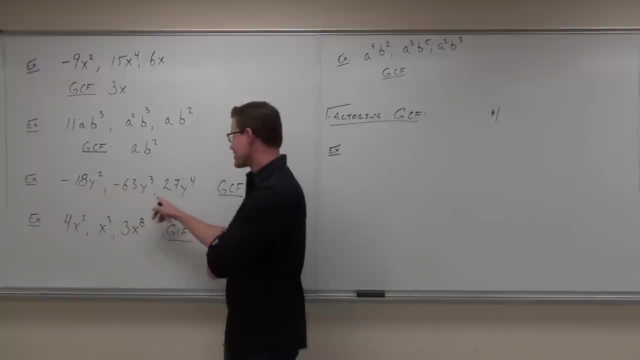 You know, you could check it with maybe this one, or maybe this one, because it has the least number of factors. This has one, three, nine, twenty-seven, twenty-seven, twenty-nine, twenty-nine, twenty-nine, twenty-nine, twenty-nine, twenty-nine. 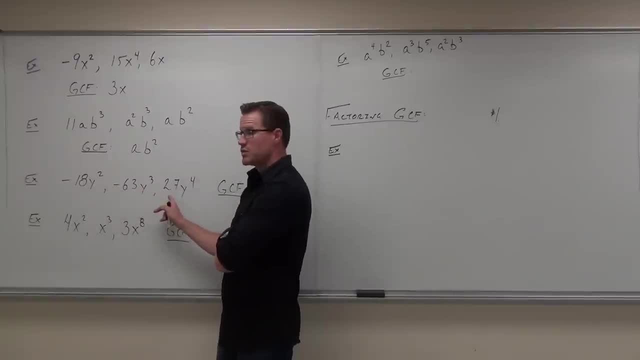 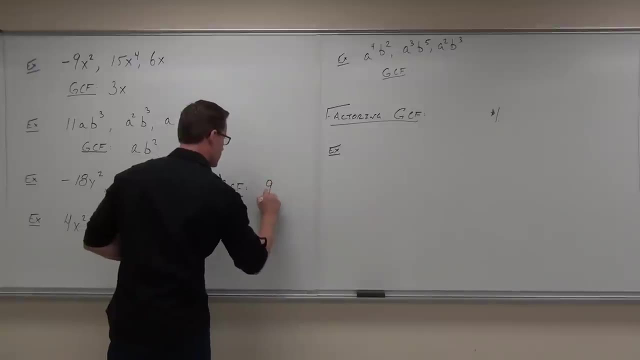 Twenty-seven: Does twenty-seven work here? No, No, No, Maybe go to the nine. Does nine work here? Yes, Does nine work here? Yes? Hey, you're done, It's nine Now. variables at this point should be really easy. 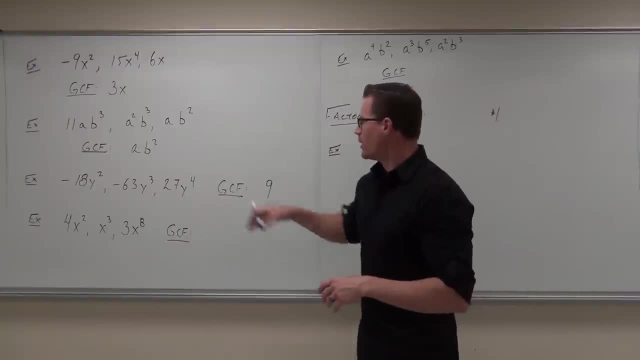 It's easy, It looks, I mean you think it's going to be harder. It's not. The numbers are harder. What's the greatest common factor as far as variables are concerned that are shared by all three? What is it? 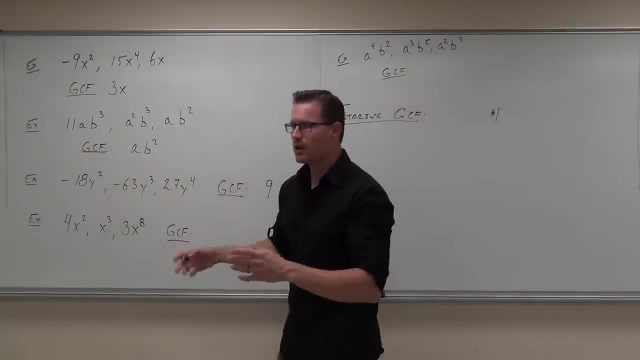 Y squared. Perfect, That's exactly right. You don't add them all up and get y to the ninth or something. You just get, well, the one that's right, The one that's shared by all, one squared Show of hands. if you've got nine, one squared. 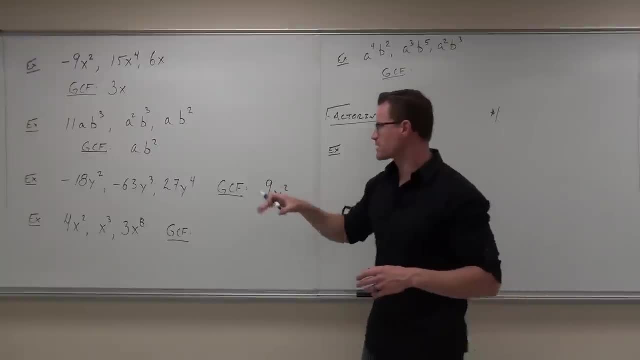 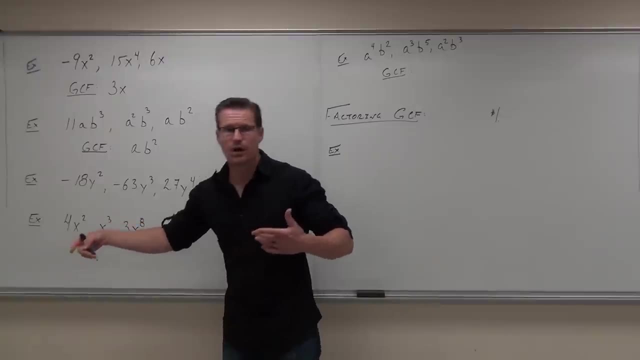 Brilliant, Very well done. Okay, how about the next one? Numbers first. We've got four. We've got One. We've got three, Three, What's the number as far as your GCF? One, One. We can write down the one just to keep in our head that we did our numbers. 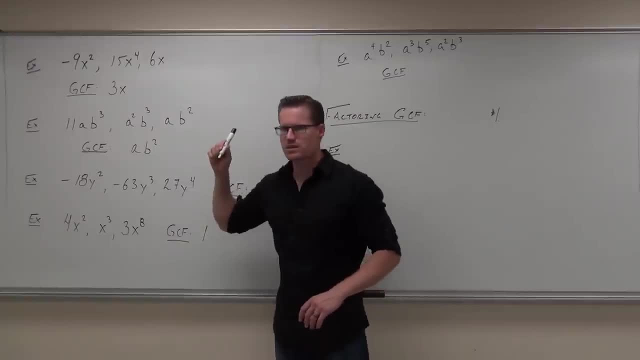 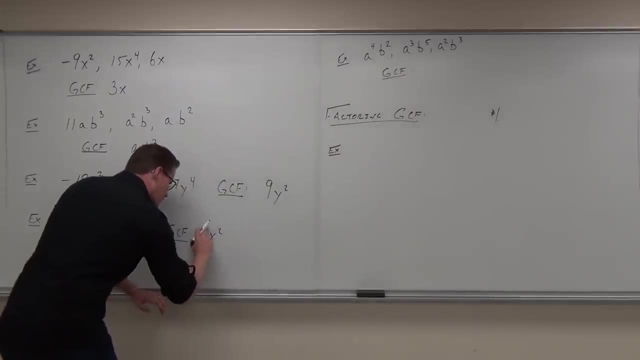 Now the variables at x squared: x to the third, x to the eighth. what is the greatest common variable? X squared. So we're going to have one x squared. Erase the one, We don't need it. But let's double check. 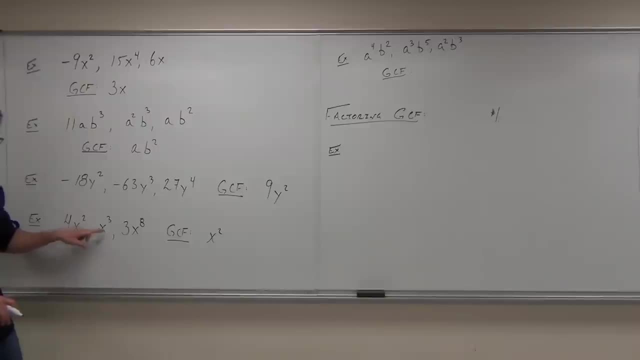 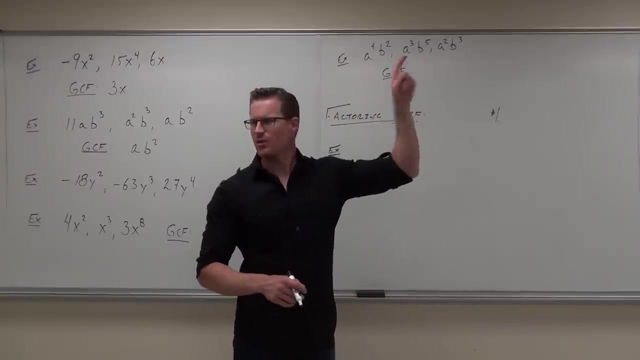 Does x squared go into this? Yes, Yeah, Does x squared go into this? Yes, Go into this, Yes. Good, Did you get to that. one Kind of fun right? What's the greatest common factor as far as the number is concerned? 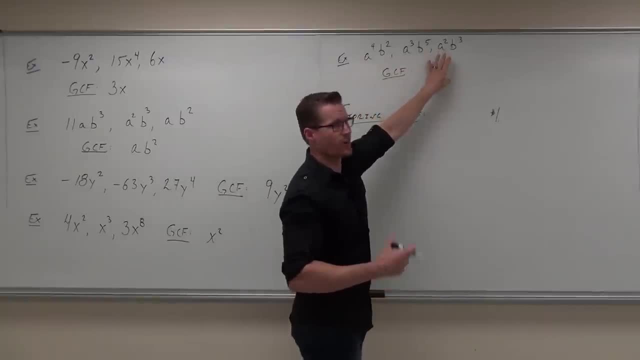 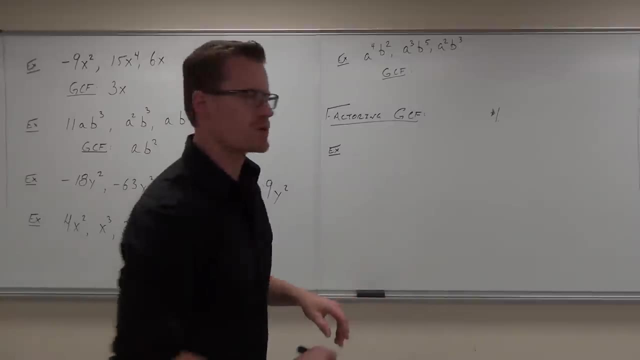 One. Yeah, There are no coefficients besides one, So you're going to have a one. You don't even need to write it. if you don't want to, Let's talk about the a's. Remember, you can do the a's and the b's, or any variables, independently of each other. 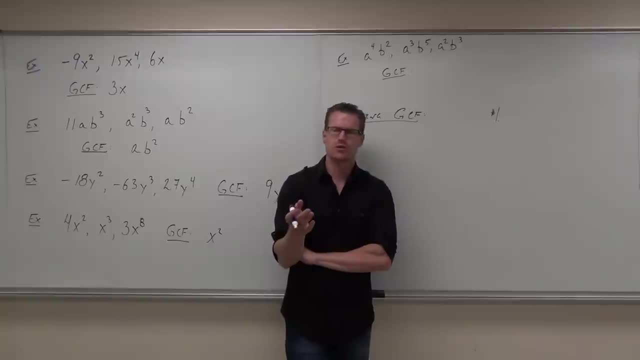 So look at the a's first. What's the greatest common factor in reference to, in regards to the powers of a? A squared, A squared, Beautiful. Why is it a squared and not a? to the fourth, Because that is the most. 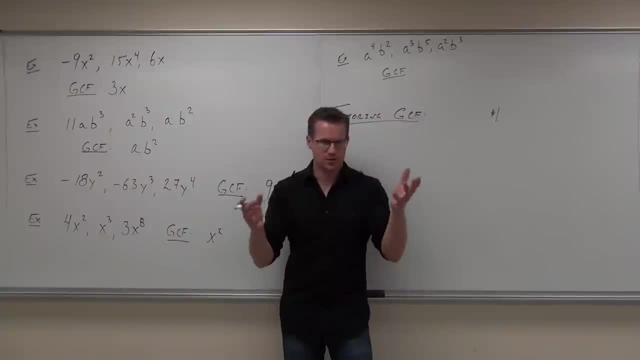 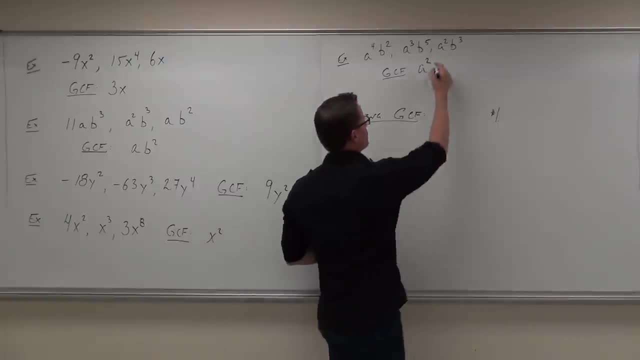 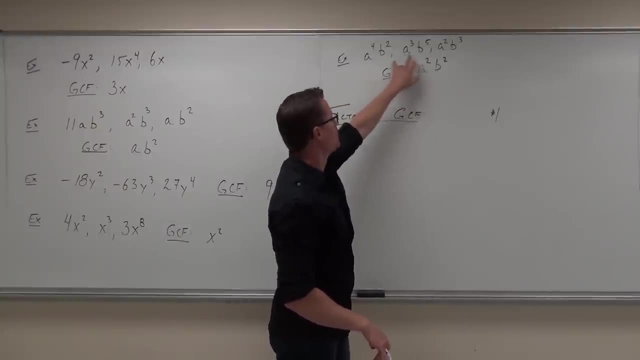 How about the b's, B squared? Sure, Yes, Does that have at least this in it? Yeah, You can divide, right? Yeah, Have we gone over any of the powers? No, Okay, So we're good. That's our greatest common factor. 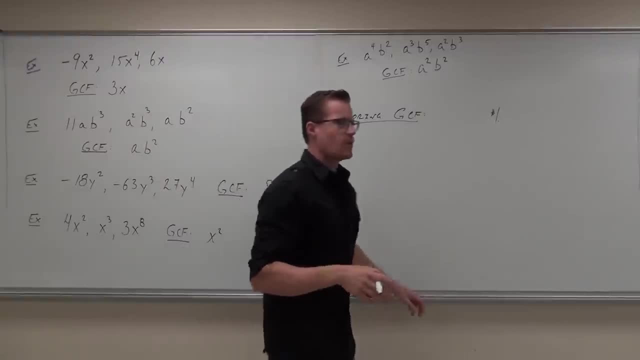 So thanks for giving that one Perfect. We're going to go just over a couple examples about how to use this Really. I want to just get the steps in your head That way next time we come in. this is going to be just- we're going to be money on this. 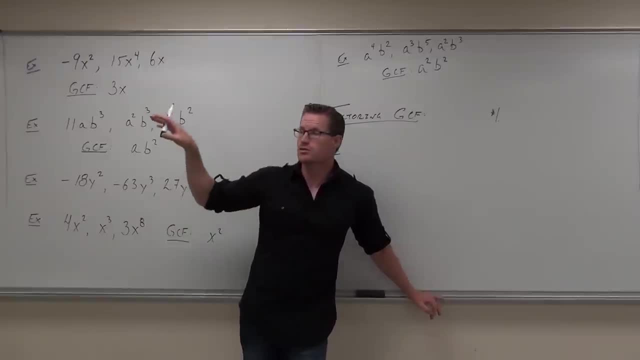 Do you feel okay about finding the factors of numbers? Yes, Variables. Put them together. If you can do this, you can factor, And here's how we do it. By the way, what I'll do sometimes, when I first introduce something, I'll give you an. 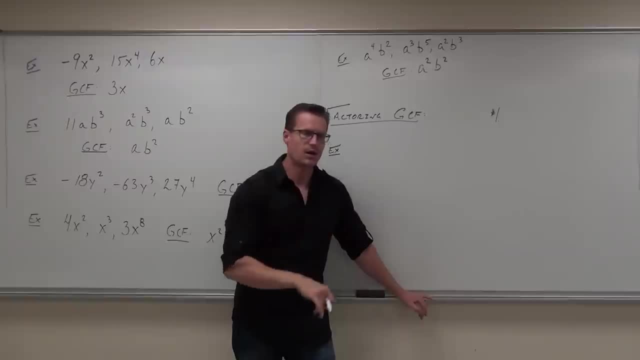 example, and I'll give you the steps on how to do it so you can refer back to how to do this later. So let's start with something very simple. Some of you might have- I'm guessing you have seen this before. Let's do something like 6x plus 14.. 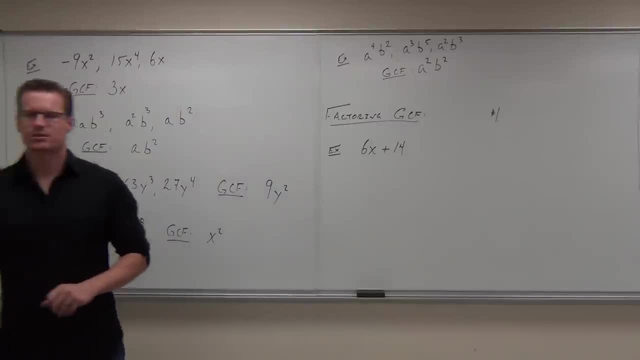 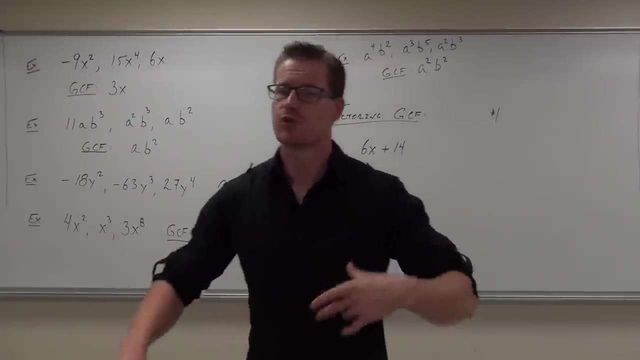 6x plus 14.. Now, instead of just listing out the factors we're going to be factoring, We're going to be using that greatest common factor, finding the greatest common factor to our advantage. Now here's the deal. You already know what distribution is correct. 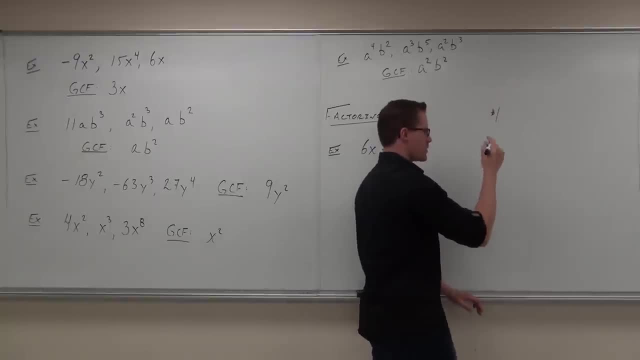 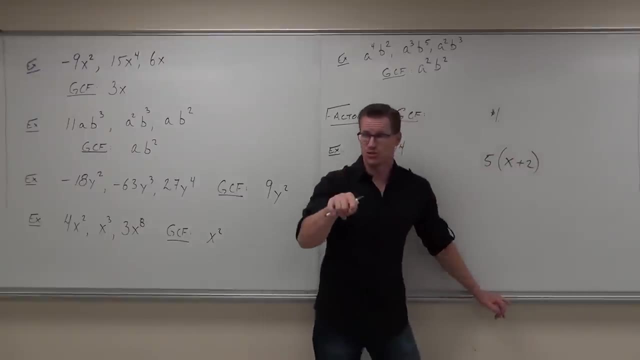 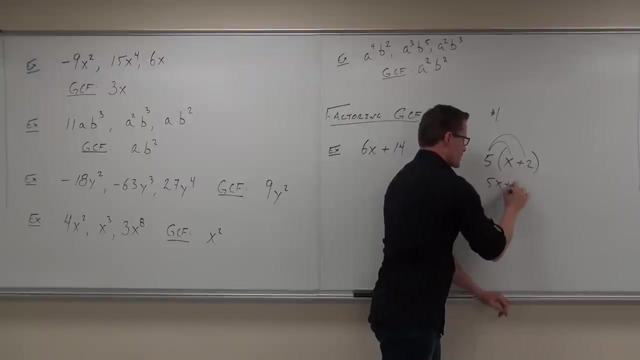 Yes, So if I gave you, you don't need to write this down, Just watch, I'm erasing them anyway. If I gave you 5 times x plus 2 and I said distribute, you would multiply this here. you would multiply this here and you would get 5x plus 10.. 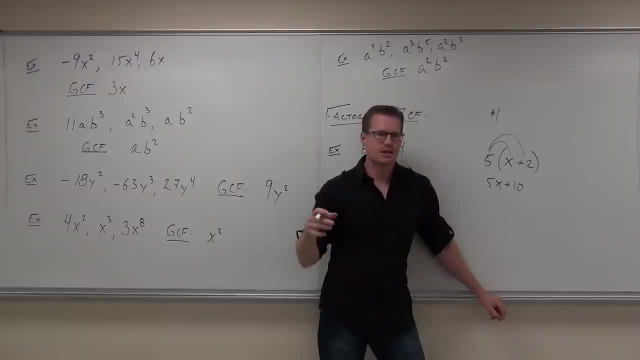 Yes, no, Yes, What we're doing in factoring is literally going opposite of that, in reverse of that. So, whereas distribution is multiplication to get rid of parentheses- Okay, focus up here for a second- Whereas distribution is multiplication to get rid of parentheses, factoring is the. 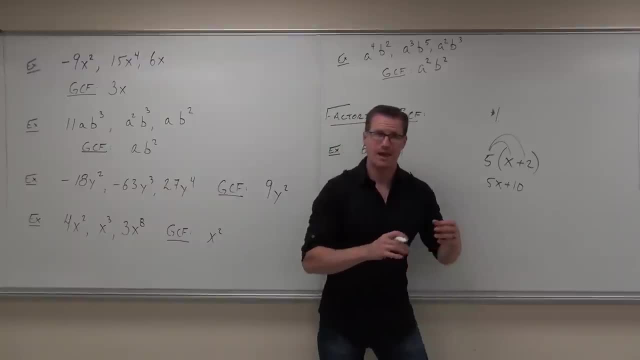 opposite, What's the opposite of multiplication, Distribution, And that means we're going to be creating parentheses. So when you factor, you're basically going not from here to here, which you're used to, you're going from here to here. 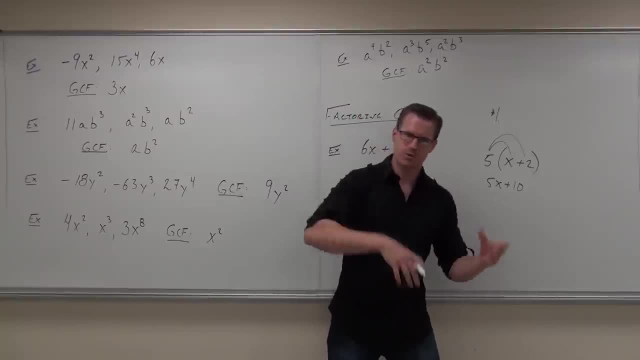 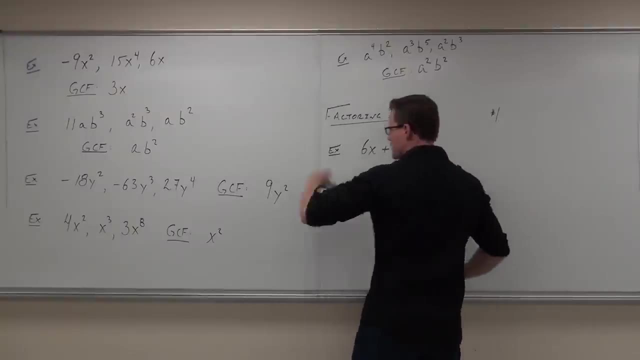 You're going in reverse. So we're not multiplying, we're dividing. We're not getting rid of parentheses, we're creating them. Quick head nod if you feel okay with the idea of that, Good, So step number one: all this stuff we've been doing is step number one. 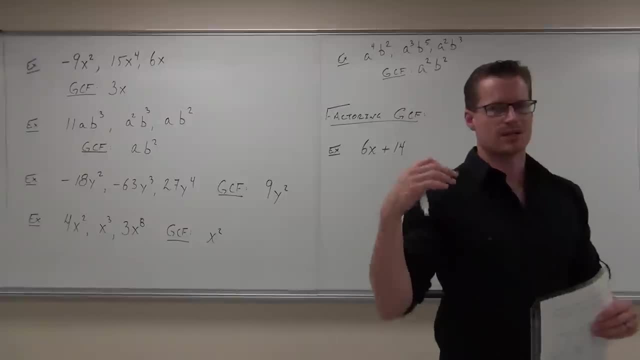 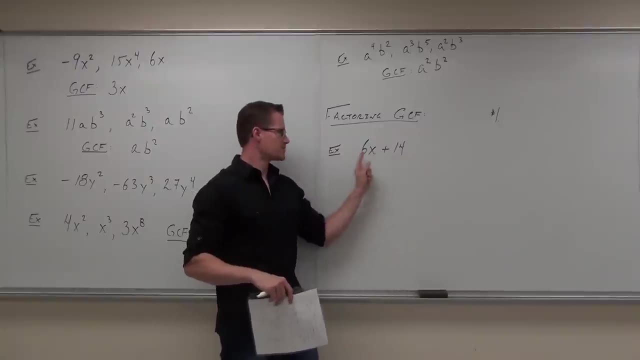 So find the GCF of all the terms. I am expecting that you understand what a term is When we look at this term term, Not term term. term Terms are those pieces of a mathematical expression that are separated by pluses and. 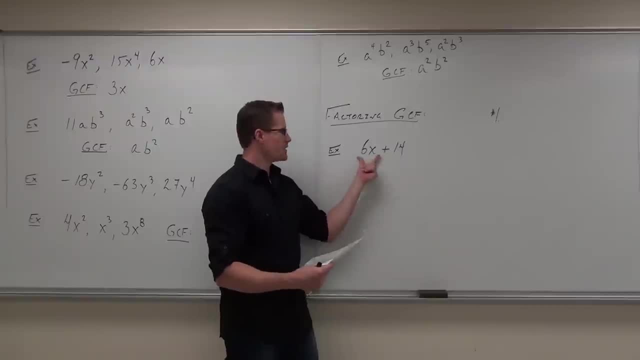 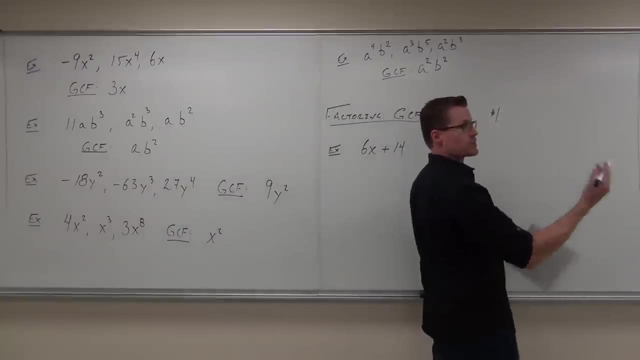 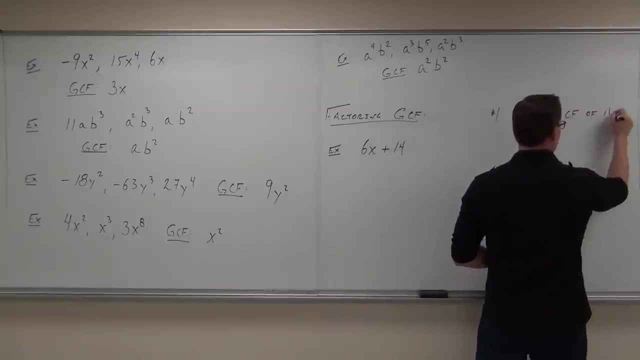 minuses. So when you look at this problem, this expression, this is one term, That's one term. You all all right with that one, Yeah, Okay. so what we're going to do? first, find the GCF of all the terms. 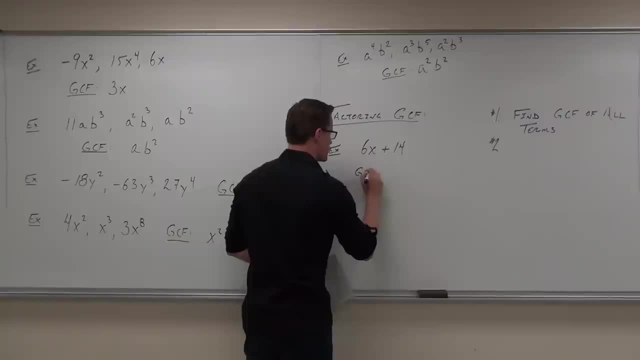 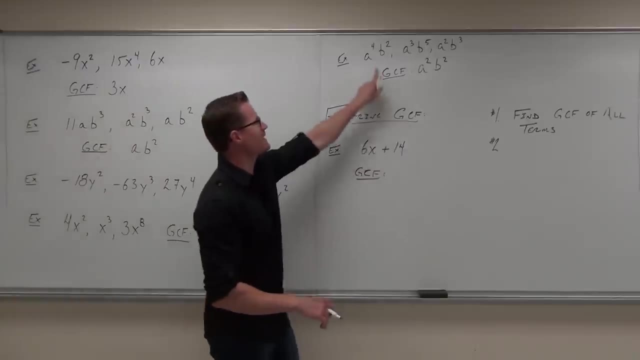 Well, let's do that. Let's do the GCF of all the terms. Tell me GCF. can you look at 6x and 14, just pretend it's like this. okay, Pretend it's like that. Can you look at 6x and 14 and tell me a greatest common factor? 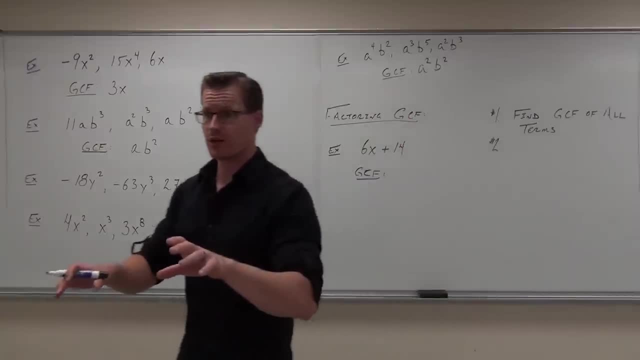 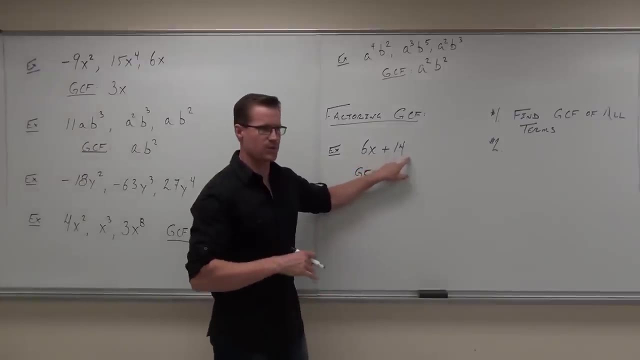 Two, Two. What about variables? Are there any variables that are shared? No, Ah. so it's not like this or this where we have shared variables. This has an x, this don't have an x. It can't be in the GCF. 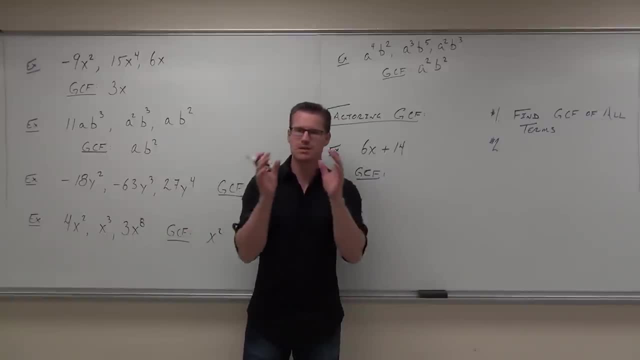 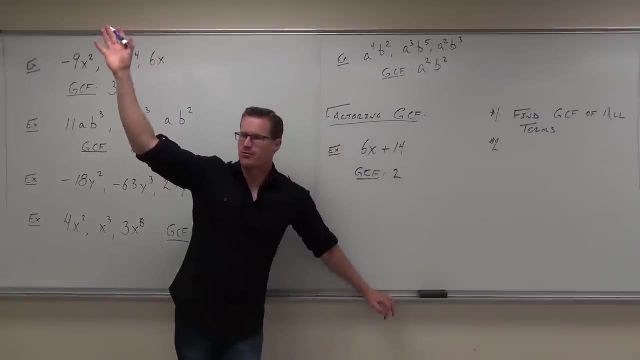 What did you say? the GCF was again Two. It's the biggest factor that goes into both of these Show of hands. if you're okay with that, The number came first. We had no variables, so we're good. Step number two: 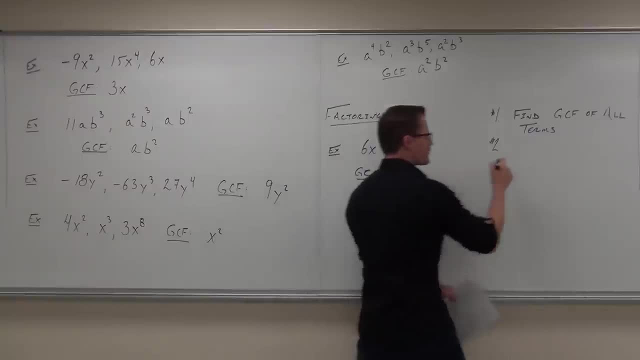 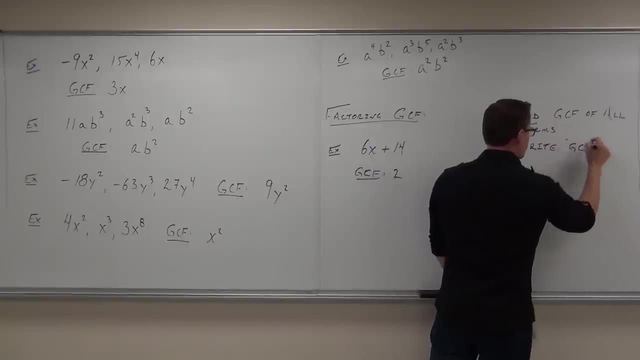 What you're going to do with step number two. after you've found the GCF, write the GCF in front of some parentheses. Okay, Okay, Okay. So step number two says: I'm sorry one more time. What's our GCF? 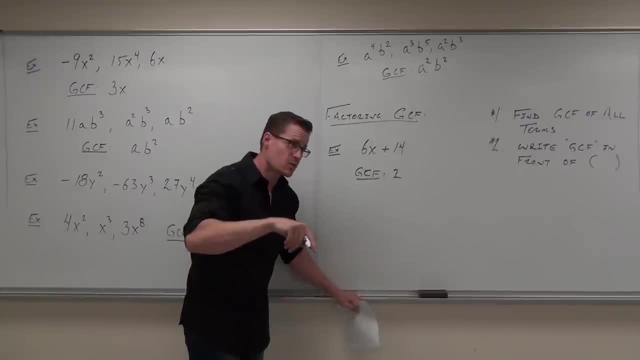 Two, Two And factoring, It gets rid of parentheses or it creates parentheses, Creates, Creates. So we're going to do our GCF and then we're going to put a set of parentheses. This is what I mean by step number two. 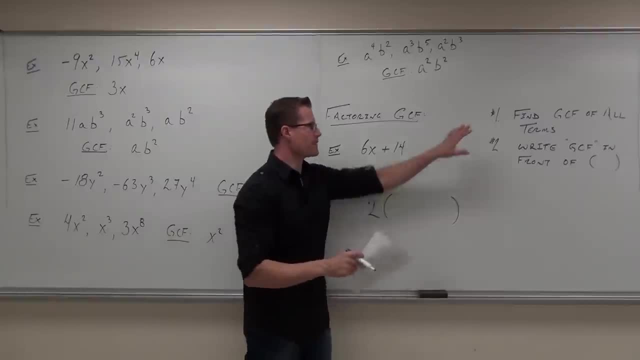 So step number one: find GCF. Oh my gosh, we should be so good at that right now. right, We spent an entire hour finding GCF. Now write the GCF in front of some parentheses, because that's what we're creating here. 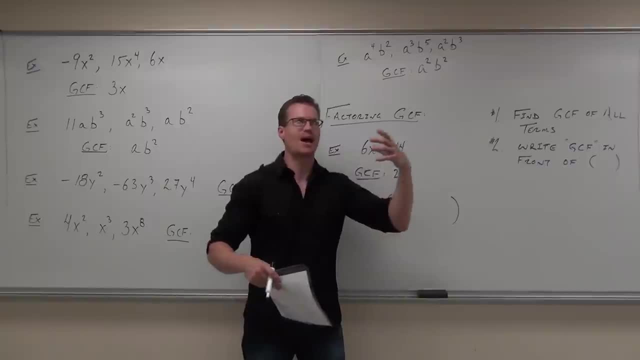 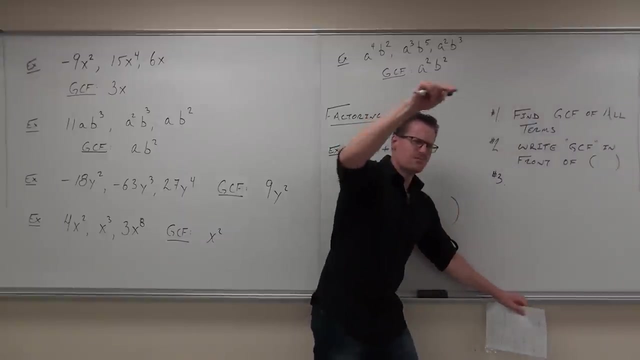 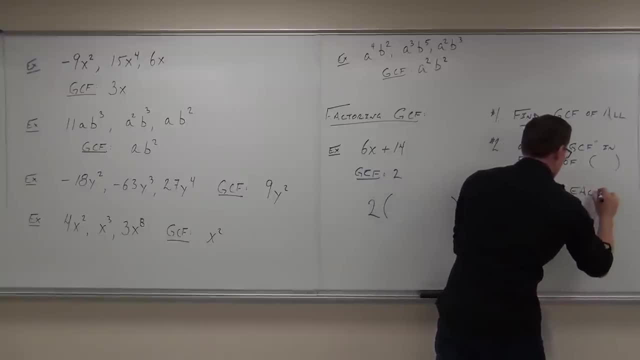 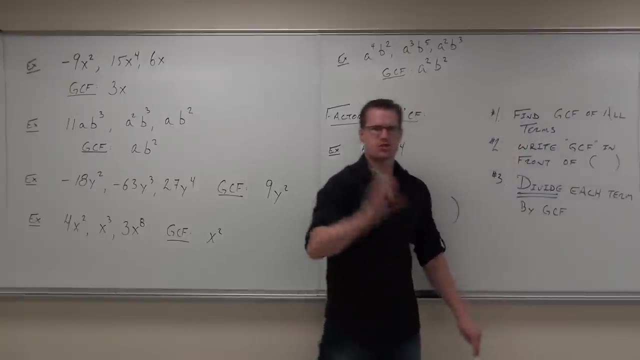 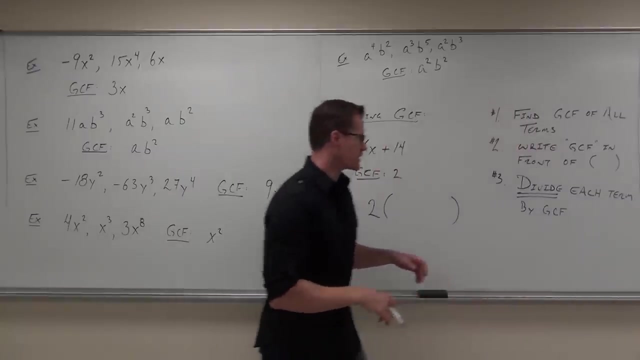 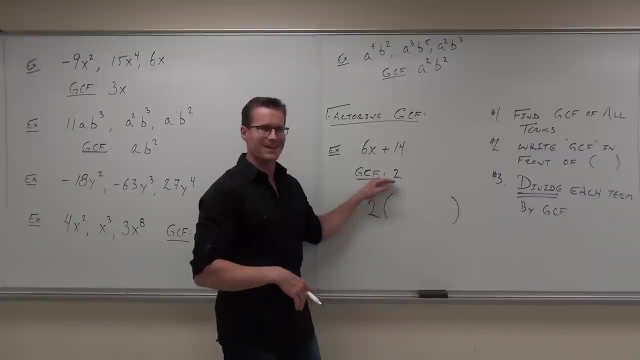 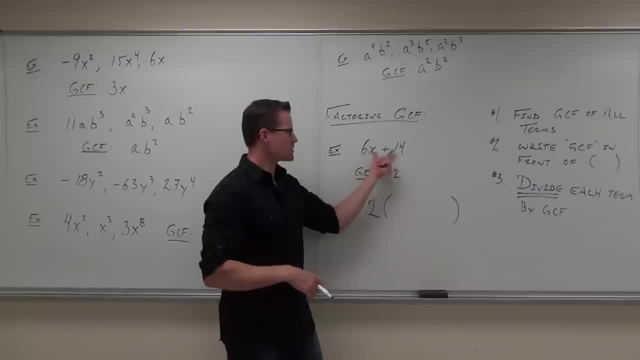 Okay, Okay, Okay, Alright, Here's the presentation for today. You know us, Where do you live, But where do you live? Hey, Which town? New school 45? Oh, K K, Please, teasing, Please, teasing. 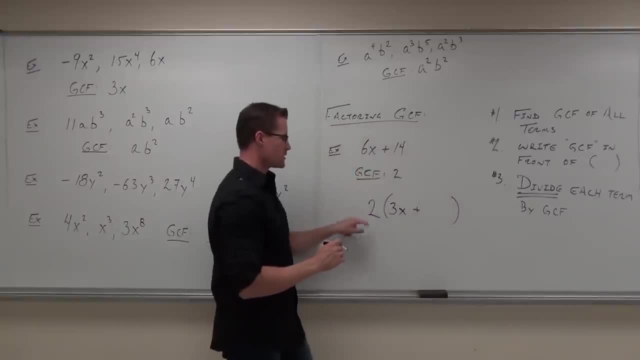 Don't be worried about that. Okay, Let's fix that up. We've already watched that week. Please tag that You've missed the next webcast, essere. Thank you. That, ladies and gentlemen, is factor Step number four. just check your work. 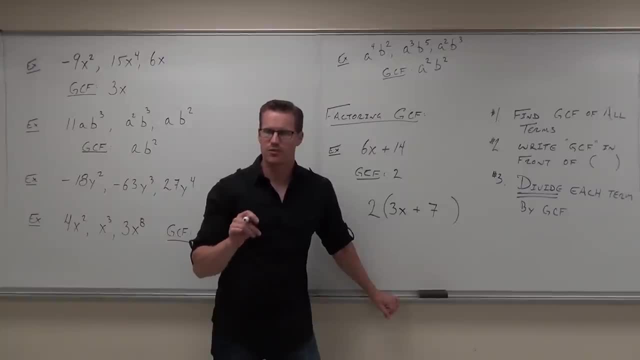 Make sure you have it right. Do not go any further until you have it right. Here's how you check. Okay, listen, Here's how you check whether you have it right. The first thing you do, you distribute to make sure this is accurate. 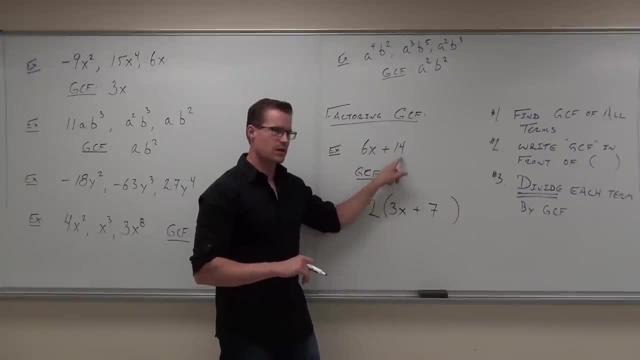 Is 2 times 3x, 6x? Yes. Is 2 times 7, 14?? Yes, The next thing you do, you make absolutely certain that you have found the GCF. What that means is that the remember the special word I gave you phrase. it's called: 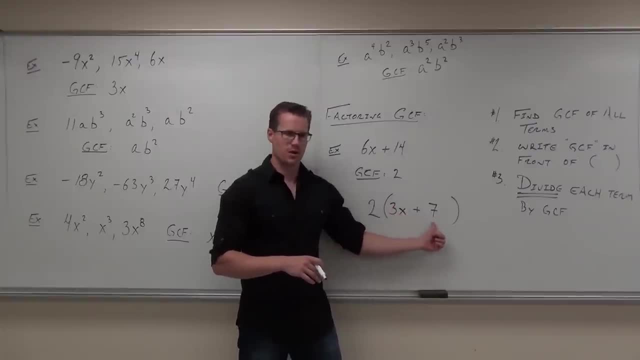 relatively prime. You remember that These numbers have to be relatively prime. If they're not, you've made a mistake. Can you divide 3 and 7 by anything besides 1?? No, That's good. Are there any shared variables here? 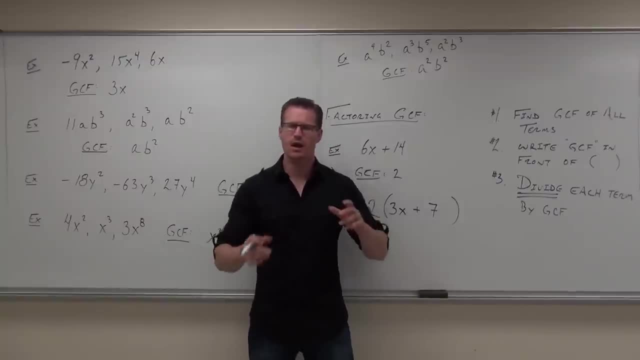 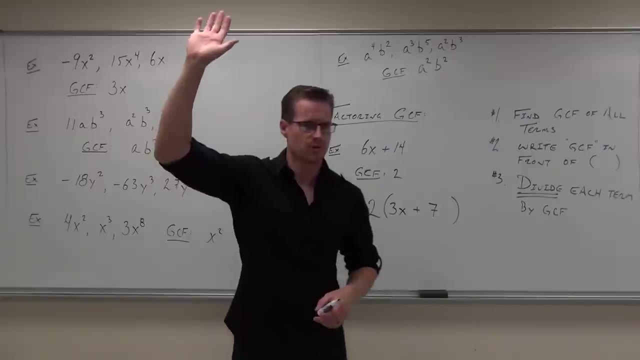 No, That means you've factored the GCF correctly. That's the whole idea. Step number four: if you want to write step four, it's just check your work and that's the two ways that you do it. Show of hands, if today has made sense for you. 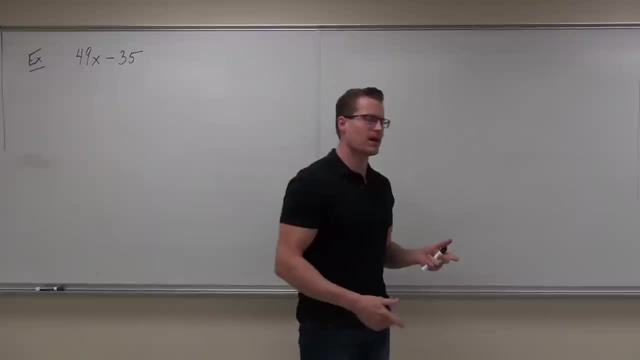 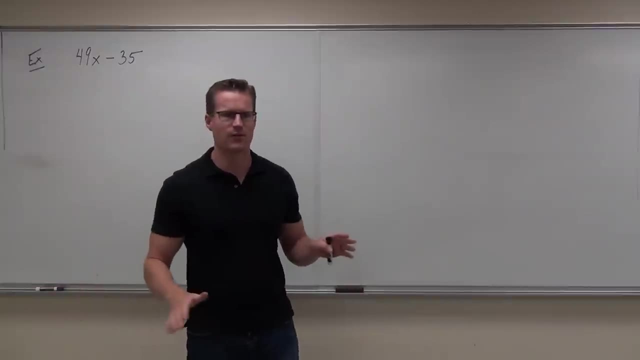 Good, Okay, so we're going to continue factoring. The very first- I'm going to say this probably 100 times- the very first step in factoring anything that you're going to factor is always finding the GCF, if there is one. 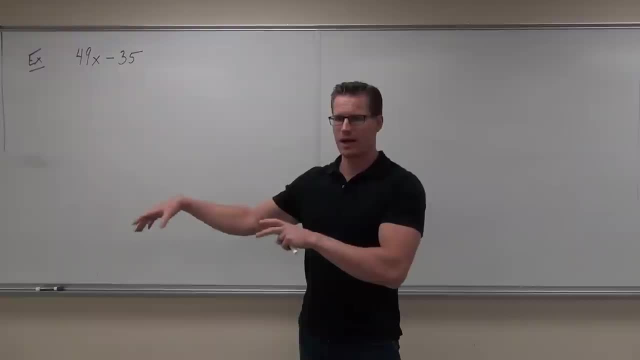 That is your first step, No matter what else I teach you for the rest of the semester. whenever you're involved in factoring, the very first thing you need to check for is what GCF, GCF. That's number one. 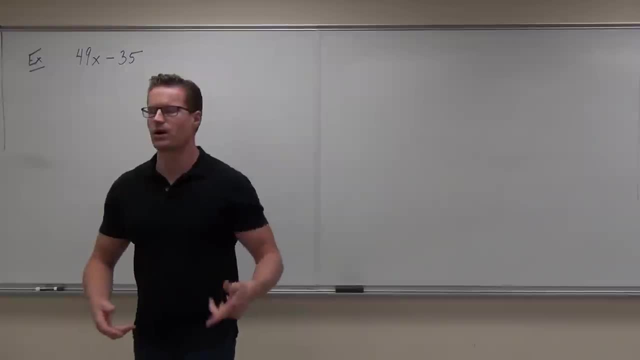 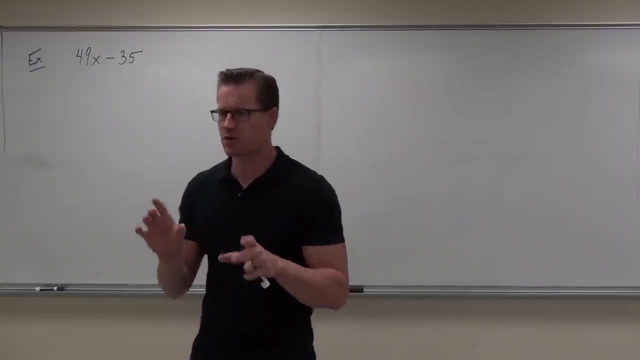 In our case, up here. the idea is- I'll lead you through this because it's been a while since we've done any of this. The very first idea is: look at how many terms you have. Remember. terms are those things, those pieces of a math expression that are separated by 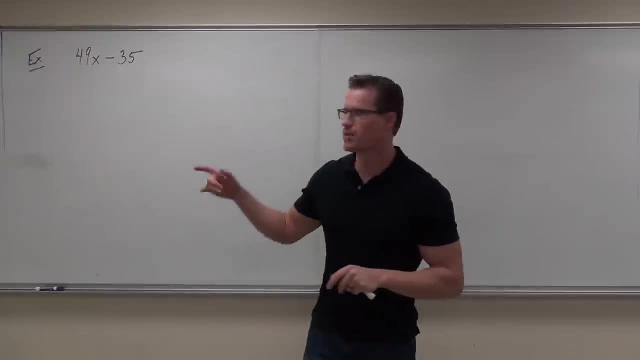 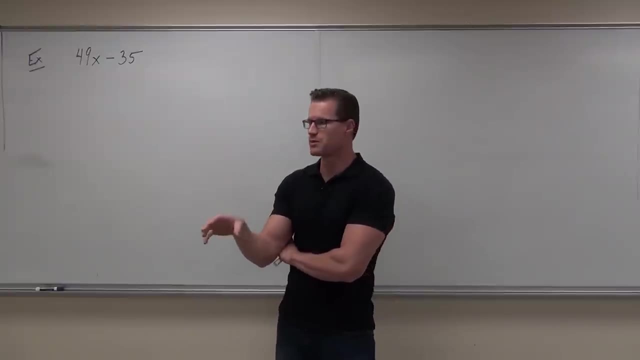 pluses and or minuses. Pluses or minuses, how many terms do I have? We look at those two terms and basically we just find the GCF, like we practiced so many times before with those two terms. Remember that we're looking for numbers first and then variables, and we put those two things. 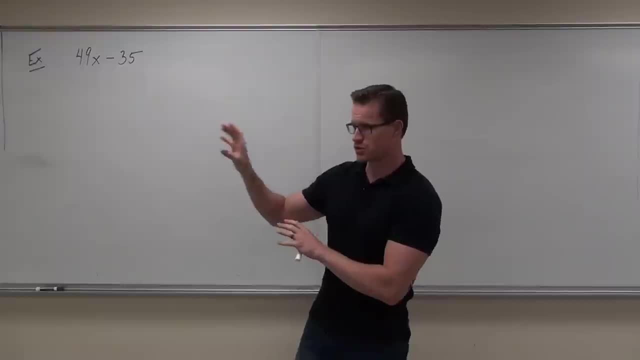 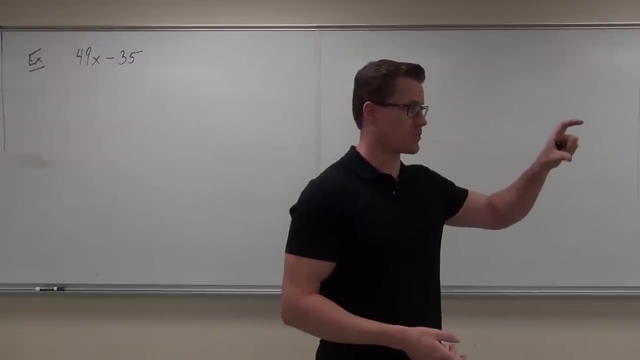 together. When we look at 49x minus 35,, those two terms, the 49x and the 35,, we think of a number, Any number that can go into both of those terms, and the biggest number, the greatest number that goes into factoring. 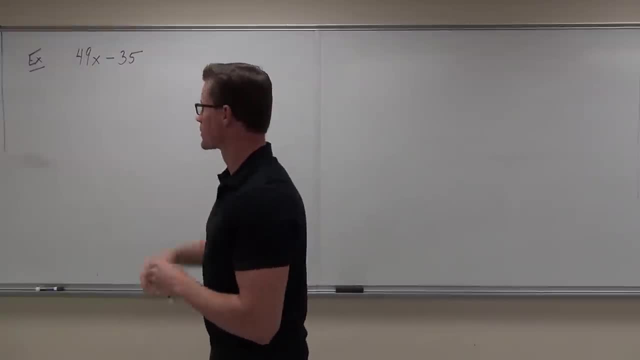 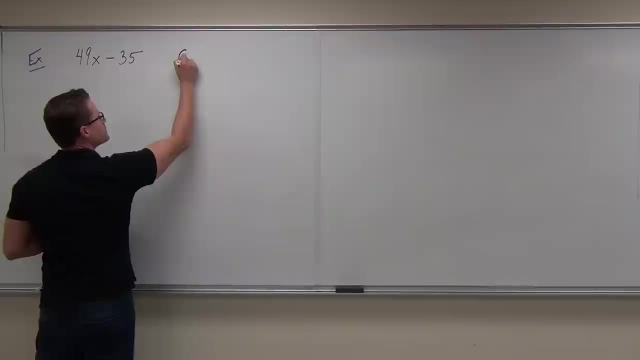 Factors? both of those terms common, greatest common factor? What number goes into both of those? So I'm not going to rewrite the steps I gave to you last time, but the idea is, once you have determined what the GCF is, you can write it down. 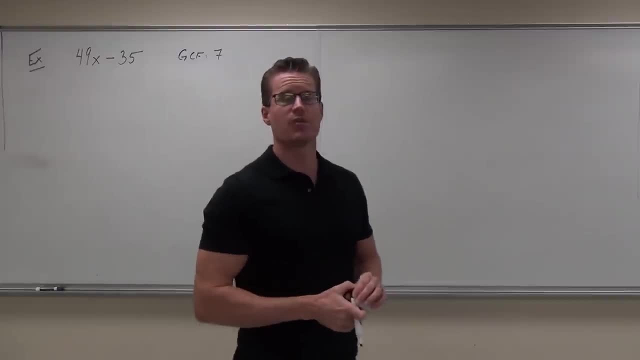 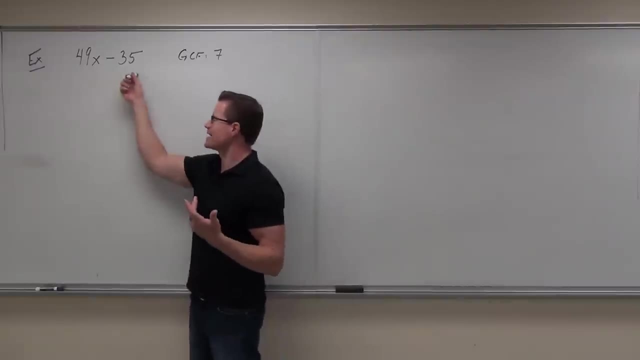 You don't really have to, but you can just keep in your mind. We get the number first, Then we look for any variables. Are there any variables common to both of these terms? So, while this has an x, that one doesn't, we say no, there's no variable, that's common. 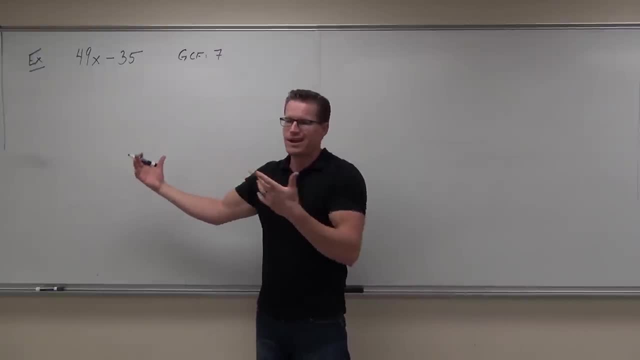 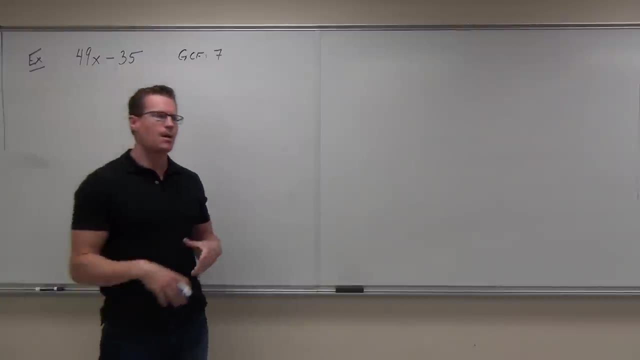 to both. Hence our GCF for this expression. Okay, It's just 7.. Show of hands if you feel okay with that. so far, Cool deal. Now the next step I gave you was: well, factoring is the opposite of the inverse of distribution. 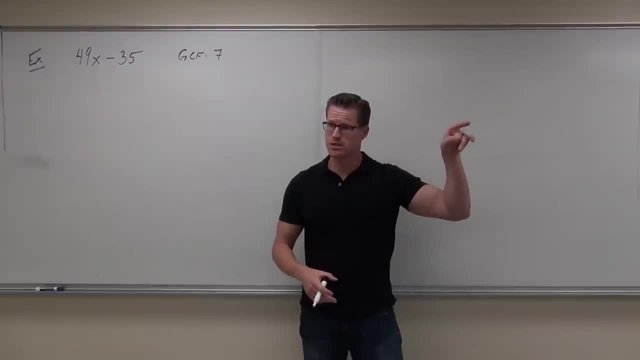 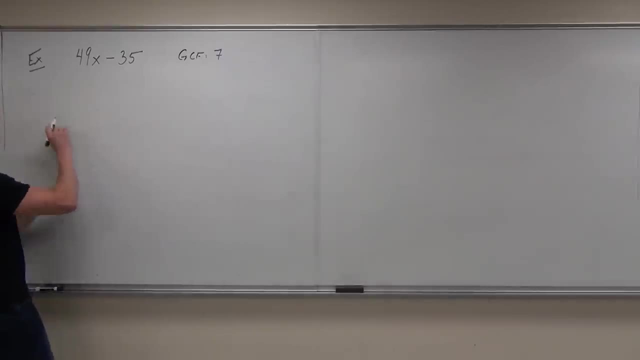 So where distribution multiplies and gets rid of parentheses, factoring divides and creates them. So we're really creating parentheses every time. we factor That always if you factor something you're going to create parentheses. So when we've determined our GCF is 7, what I've said to do is put that 7, the GCF, right. 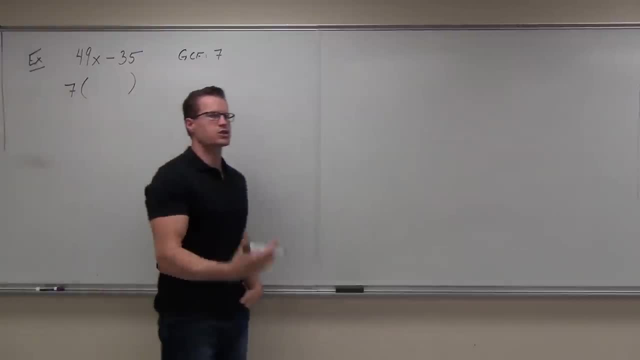 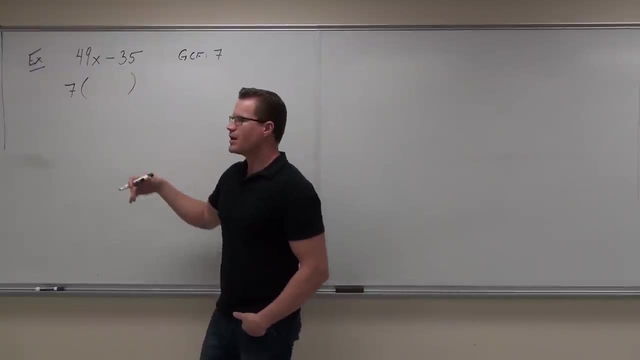 out front And then create a set of parentheses. What you're saying here is: I'm going the opposite of distribution. I'm going to create parentheses and divide to get my inner two terms here. So basically, since distribution is multiply, factoring is divide to get these two terms. 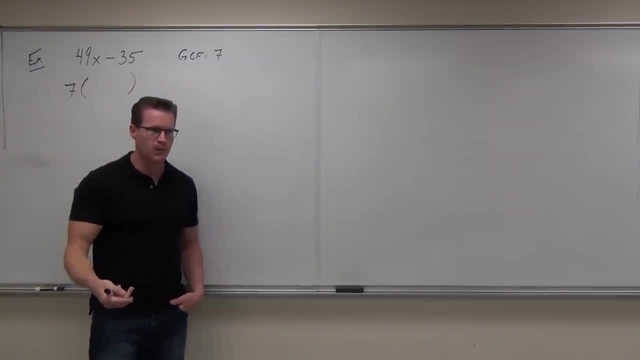 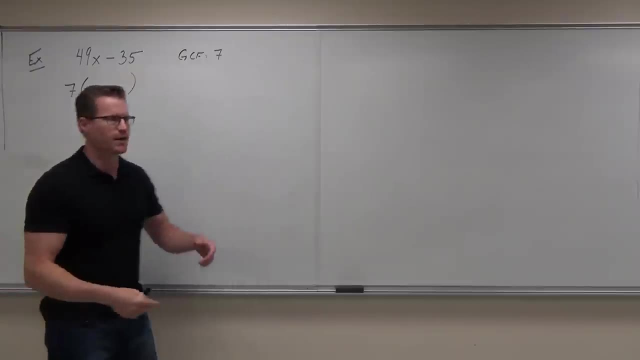 we're just going to divide. What are we going to divide by Why That's it, That's the GCF, That's what actually divides into both of those terms. So we're going to take that. Sometimes you can do it in your head. 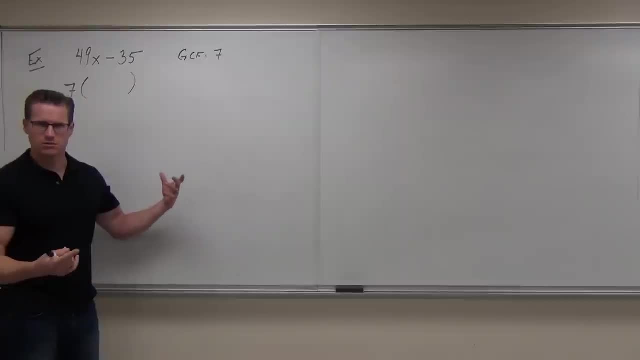 When they get more advanced. I'll show you some methods on how to write this out so that you can see really what's going on. Basically, you do it term by term. Can you do 49x divided by 7? What is it? 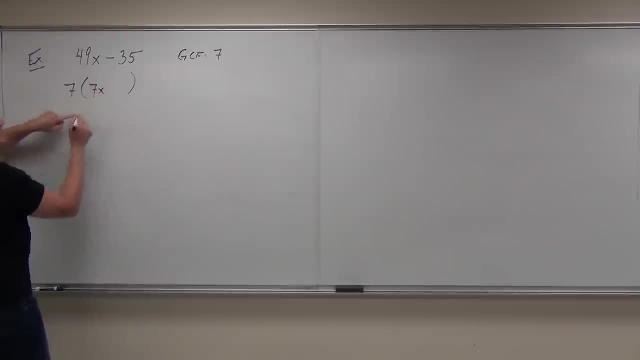 7x. That goes right here. That's our very first term, So it's just these two terms divided by our GCF, and we put our remaining two terms inside our parentheses. Can you check your work? Yes, Yeah, If factoring is the opposite of distribution, that means to check our work. we just have. 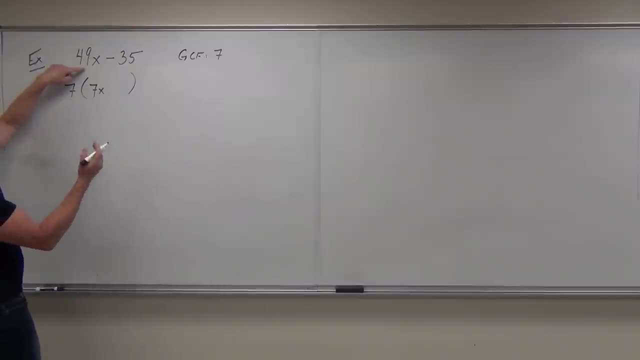 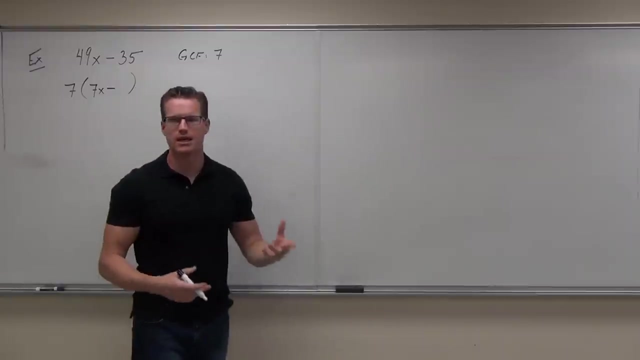 to distribute. Yeah Yeah, If we do 49x, we know we got it right. Also, this sign is going to be the same unless we start factoring out negatives- and we're going to talk about that in a little bit- But generally, if you're factoring out positive numbers, your signs don't change. 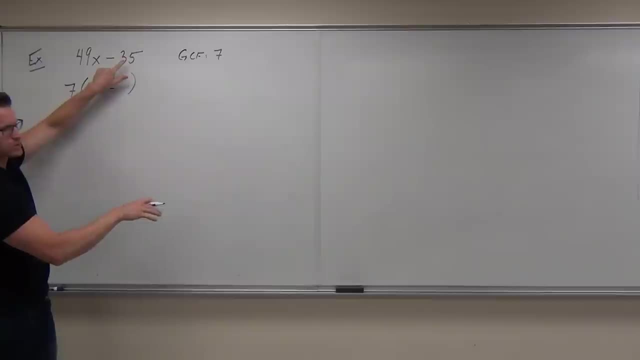 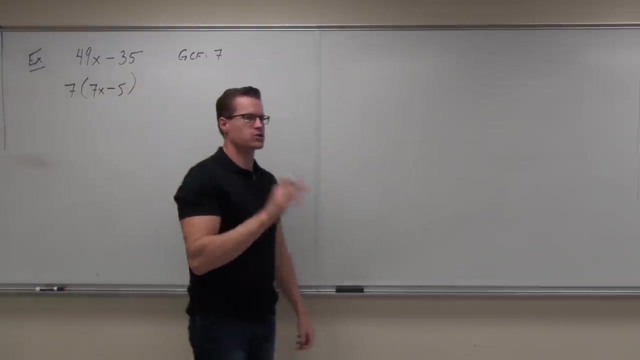 Now we get to the next one. What's 35?? Remember, we're dividing, We're factoring: What's 35 divided by 7? 5.. And you always double check your work. Don't go any further. It'd be so silly to go further, because right now this is the problem, right? 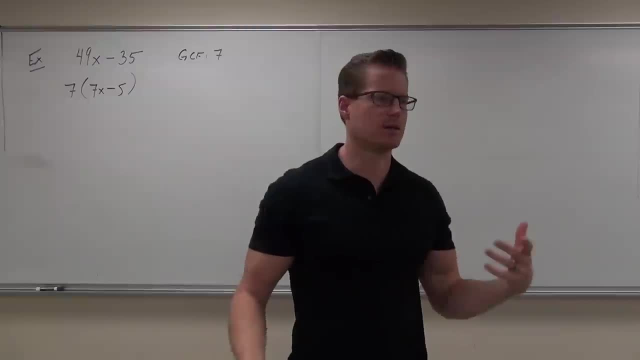 It's. can you factor or not Later on in chapter 7,, 8,, 9,, 10,, 11,, 12, 13,. you're going to be factoring, but that's a small part of the puzzle. 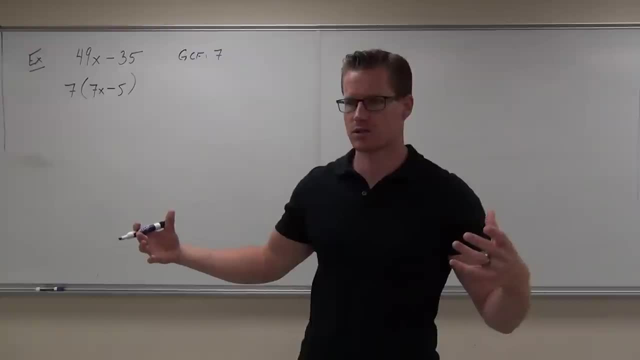 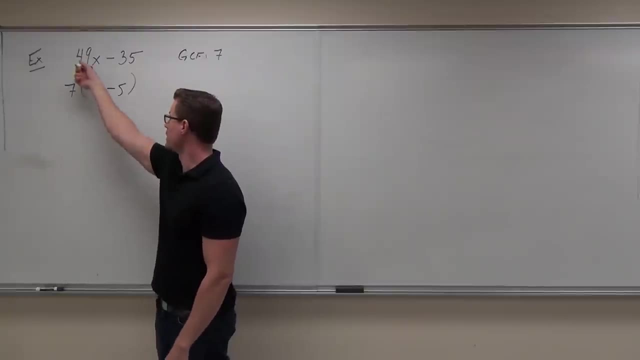 So don't just assume you have it right and go on and get the whole problem wrong, because you'll waste a lot of time there. Make sure you've got it right. So first thing we check for: Does this work? Is 7 times 7x 49, 7 times we can't consider it negative. 5, I know it's minus- we can consider. 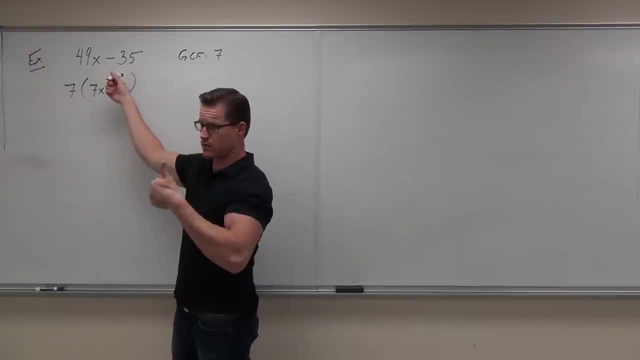 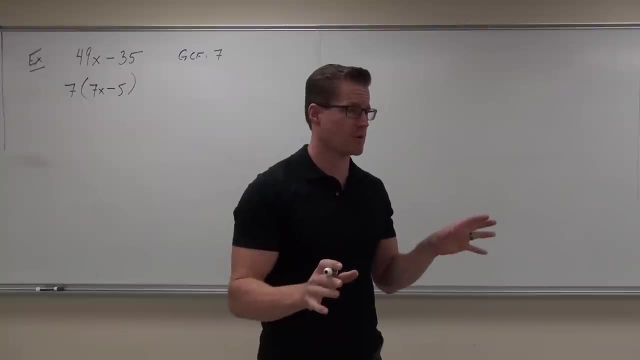 it negative 5.. 7 times negative 5, is that the minus 35 that we want? Yes, Cool, Are these? there was a key word there: Relatively prime. Are they relatively prime? Yes, Which means the only thing that goes into both those terms is 1.. 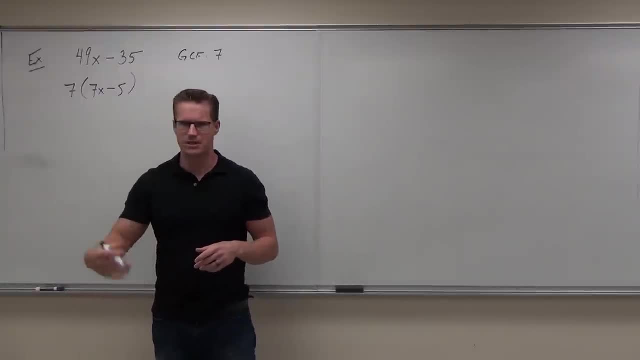 That's the idea of factoring. Do you guys feel okay with the factoring? I know it's been a while, but does that make sense to you? Yes, Okay, So that's our factoring. Let's go ahead and do a couple more examples. 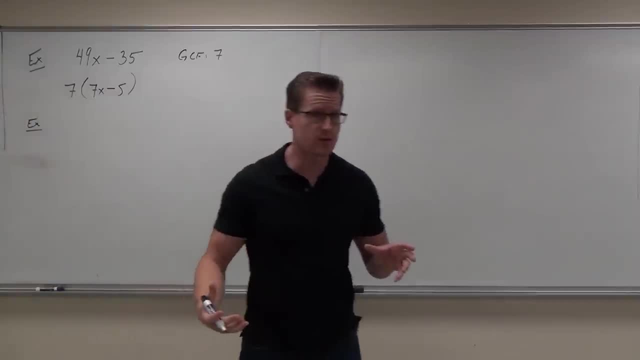 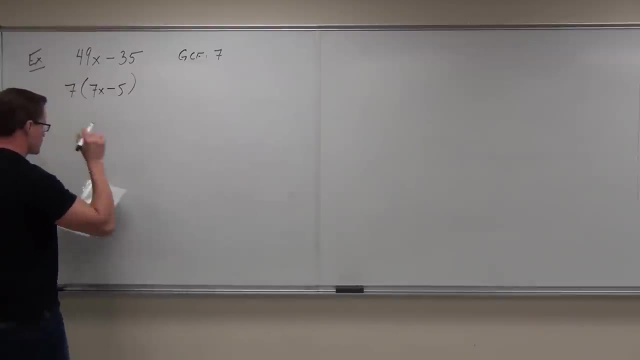 We're going to start ramping it up. This was probably the easiest one that we can do at this point. We're going to start talking about how variables play a part of this and then put numbers, variables together and see what all we can do. 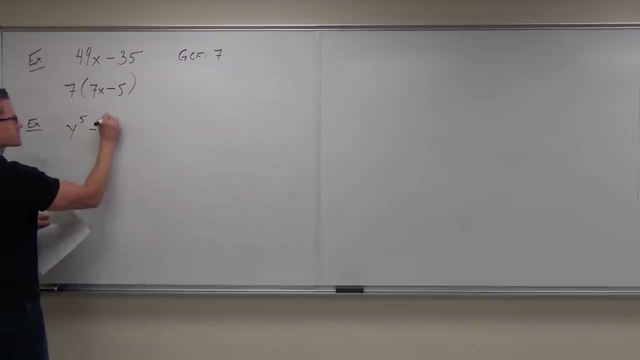 So next example: How about y to the 5th minus y to the 7th, y to the 5th minus y to the 7th? First thing, how many terms do we have? What do you think? Two: 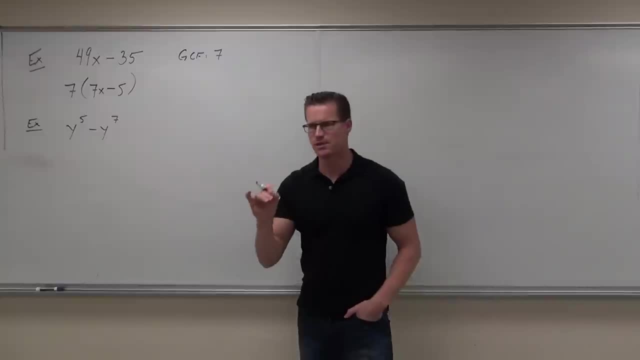 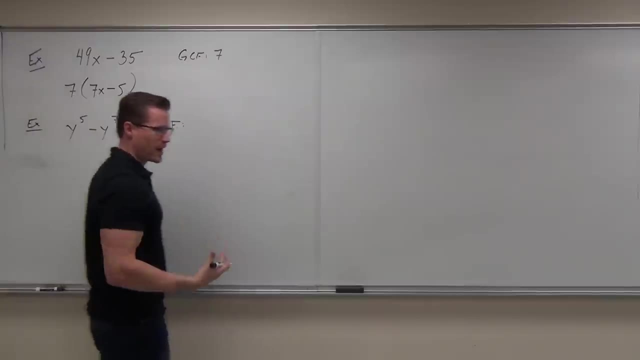 Perfect. What's the first step in factoring every single time? What is it? GCF- Let's look for the GCF And for now we're going to write it down. when you get more practice with this, you're. 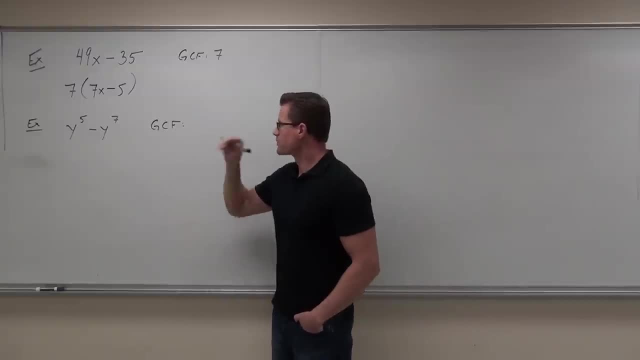 not going to do that, You're just going to go for it, You're just going to factor it. So we're looking for the GCF. Are there any numbers which go into those two terms? One, So, just one. Do we have to write down the one? 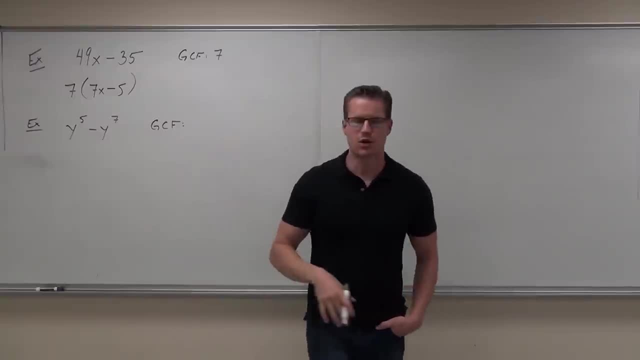 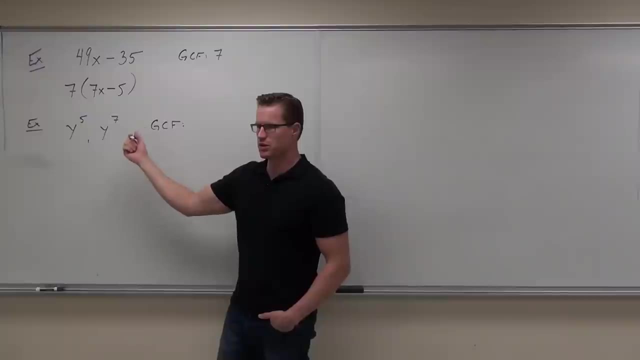 No, We can, but it's not going to help us. So next we look for any variables. Are there any variables which go into both of those terms? Remember, it's very much like doing this and saying, hey, what's the GCF of those two terms? 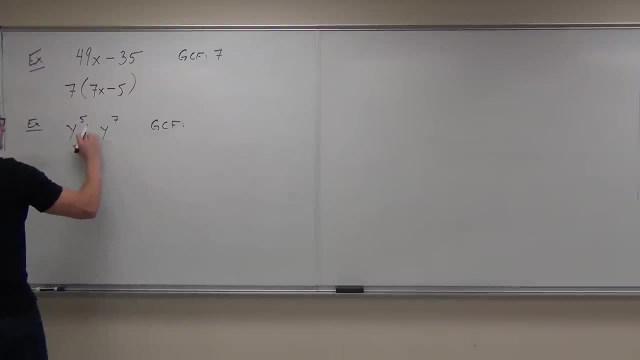 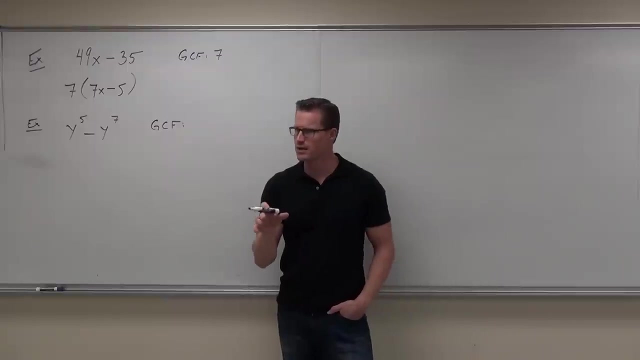 You're doing the same thing. it's just now we have a minus between it, But this idea does not change What is the GCF according to the y to the 5th and y to the 7th. Remember that what it is. it's the biggest power that both of these things have not. 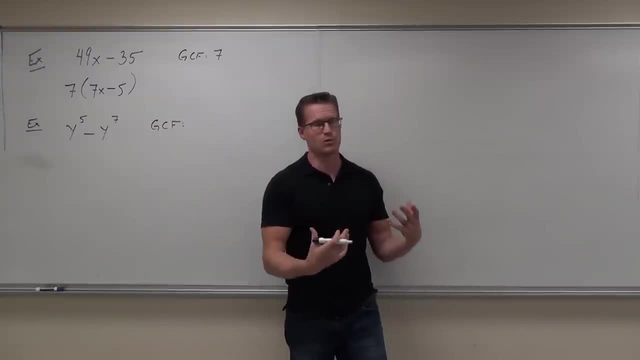 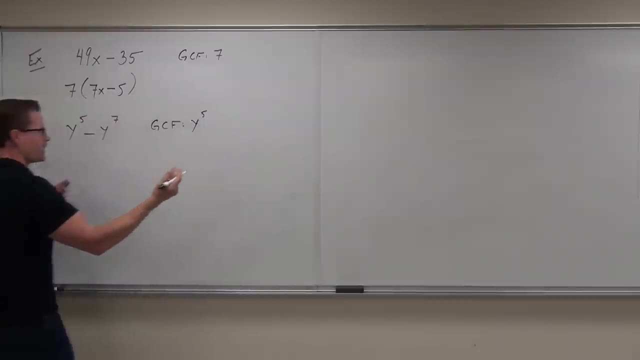 the biggest power, you see, But the biggest power that both of these terms contain. What is it? Y to the 5th, That's right. Feel all right with the GCF. Yeah, Hey, we're factoring. What do we do with that y to the 5th and where are we going to put that? 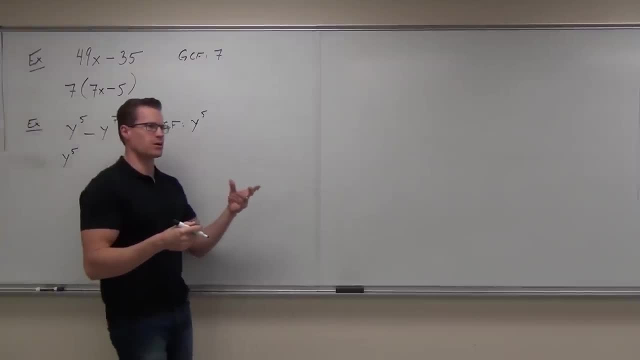 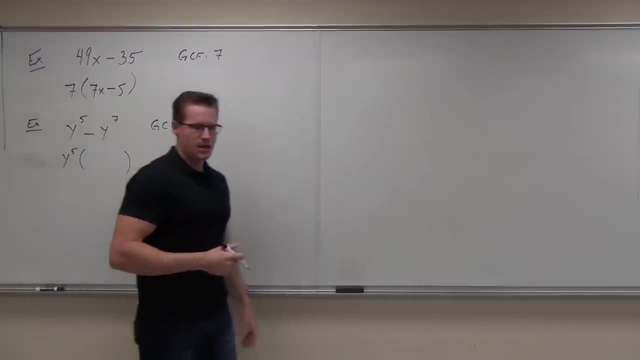 So we have y to the 5th and we know- wait a minute. factoring means that we're going the opposite distribution, So we're going to be creating some parentheses here. That always happens when you're factoring. Now we're just going to figure out what these two terms are going to be. 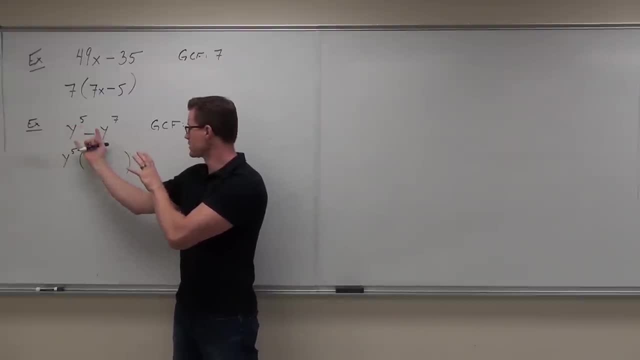 You still have the same number of terms, don't you? inside those parentheses, There's two here. There's going to be two terms here. You're just creating a factor, something that you can multiply by. that gives you back your original expression. 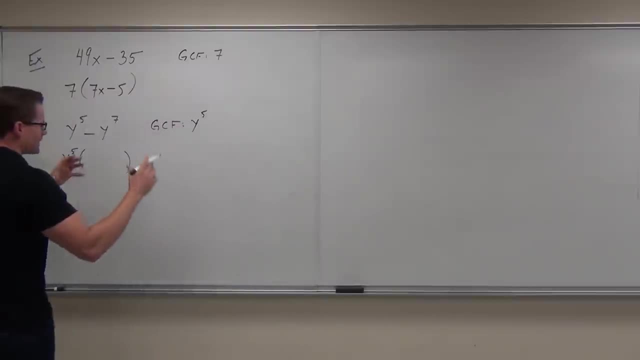 That's the idea. Now, if you're a little bit kind of- oh my gosh, I don't know how to divide with these exponents, here's a trick, not a trick, something that you can do to help you out. 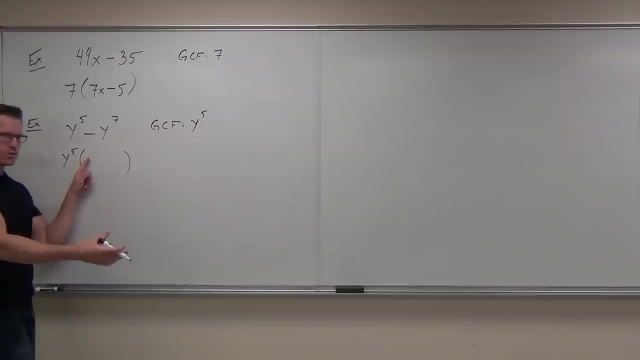 In order to find these- you guys all know these- you divide, right? Well, take your first term. Okay, Divide by your GCF, and whatever your answer is- by the way, this has to work, otherwise you picked the wrong GCF. 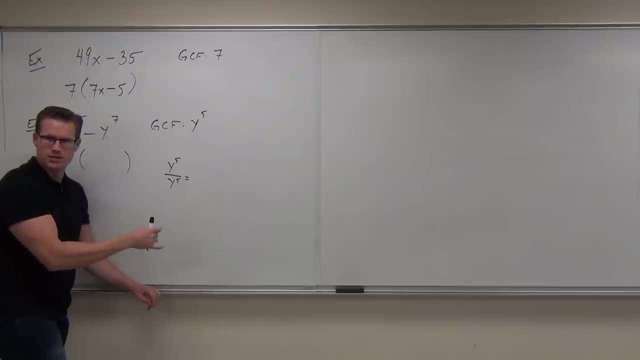 It must always divide, otherwise it's not a factor. Did you catch that? If you're trying to divide, you go wait a minute. it doesn't work. You picked the wrong thing, So go back and fix your GCF. 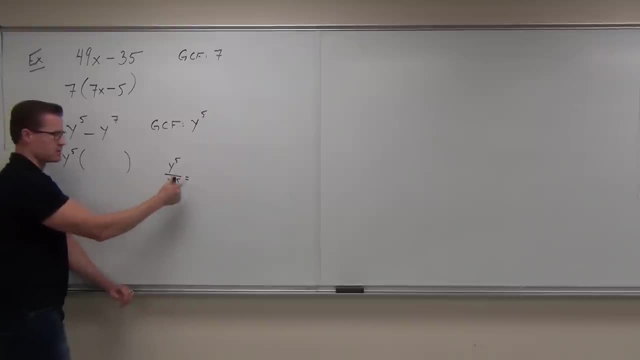 This will always work. How much is y to the 5th divided by y to the 5th? One That goes here? One. You can always do it off the side if it gets a little bit more advanced for you. Man, I can't do it in my head and write it out. 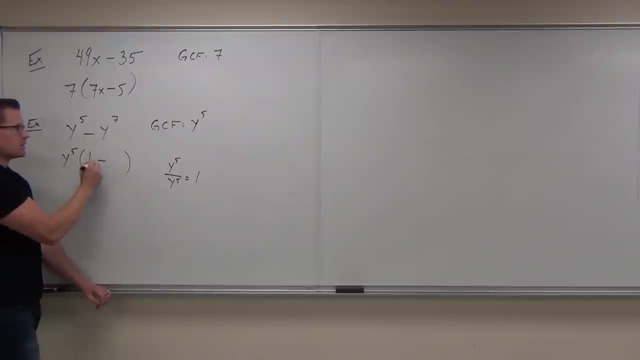 Not a big deal. I'm going to change What do you think? No, No, Okay. Next one, This one. So we wrote the first term divided by GCF, That's y to the 5th. divided by it just happened to be y to the 5th, it ends up being 1.. 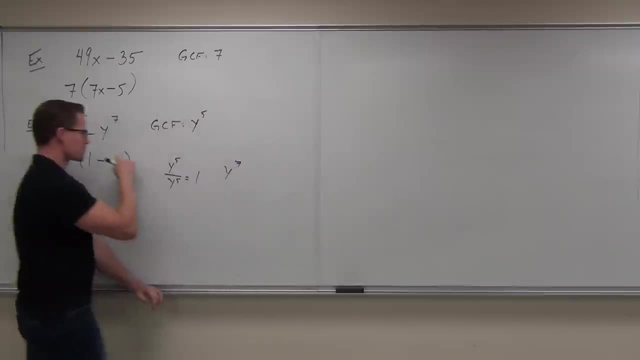 That's our first term. Now we're going to take y to the 7th. We already know that we're going to have a minus there, Divided by y to the wait. divided by what? The 5th Sure. 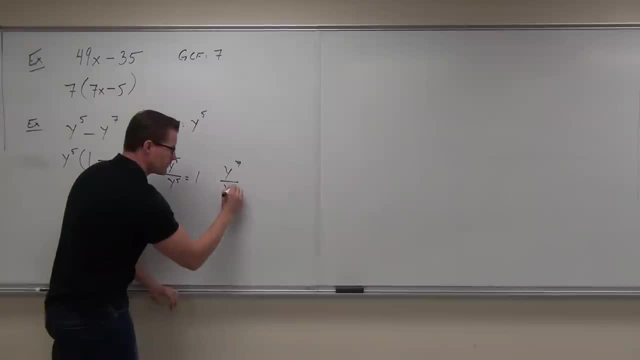 Second term, divided by GCF. you have them two places. Can you do y to the 7th divided by y to the 5th? Yeah, Y to the 7th. How do we do that? What do you do with those numbers there? 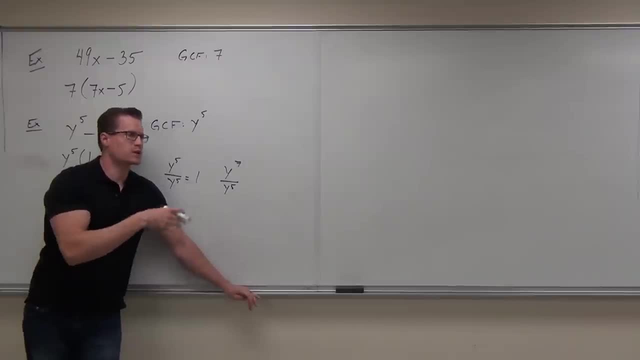 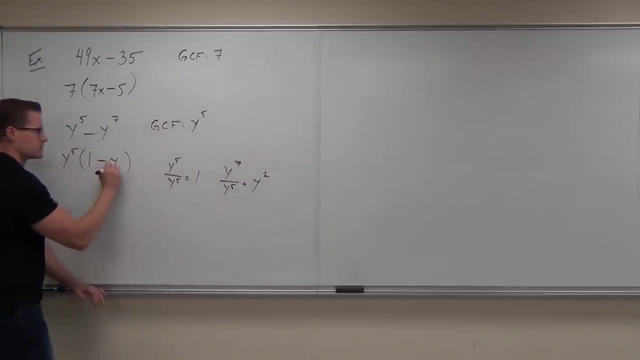 We know that when we're dividing common bases with exponents, we subtract those exponents, So we have y to the 2nd and that y to the 2nd goes there. Can you still check your work, even though you dealt only with variables here? 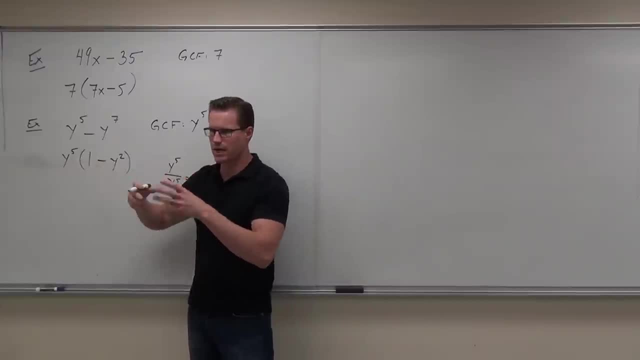 Yeah, Distribution is the opposite of factoring. So those things work hand in hand like division and multiplication. It is division and multiplication. So, if we checked it, y to the 5th times 1, y to the 5th and y to the 5th times 1.. 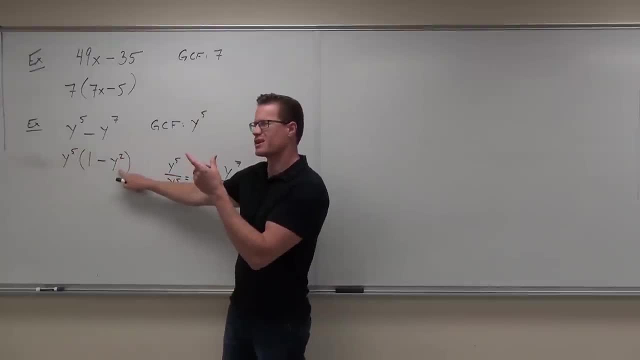 Remember, we have exponent rules. When I multiply common bases, I add those powers, So that would be y to the 7th, And we know we have it right Now. let's keep going just a little bit further. How about this? 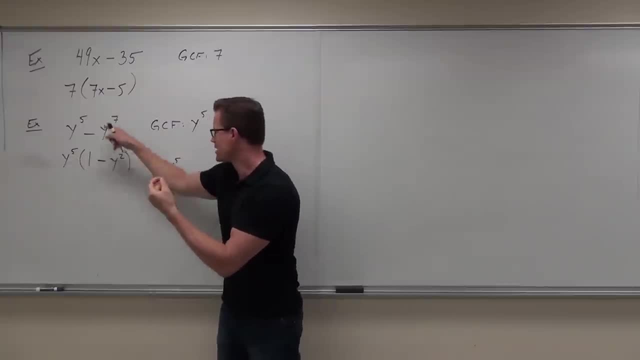 Is there anything that goes into both 1 and y squared? Kim, let's check for that. Is there anything that goes into both those things? 1. 1 does Anything bigger than 1? No, Are they relatively prime? 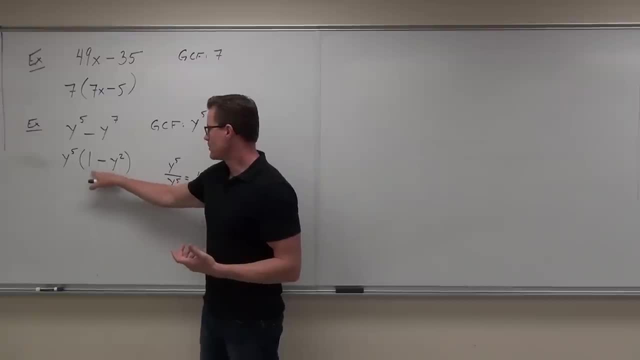 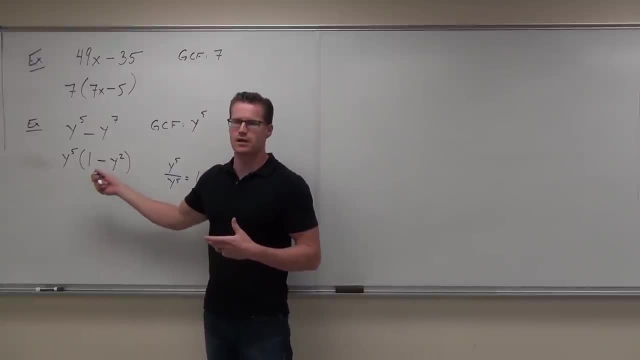 Do you feel okay with what we're talking about? Okay, Now, in the future, we will be talking about how we can go further on something like this. If you know this concept, if you've had this class before, or if it factory before which, 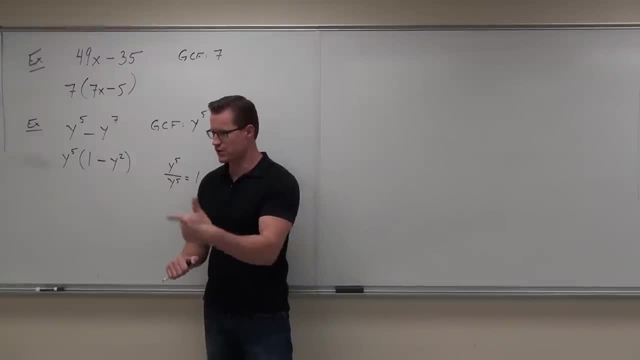 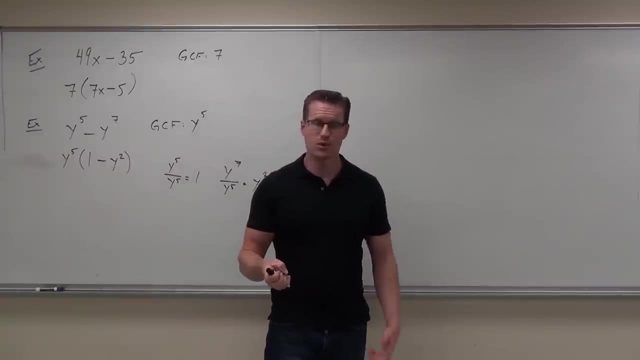 I think most of you have remember. it's kind of like a refresher for you. That's called the difference of squares And we're going to talk about it. Did you know that term, that difference of squares term? Yeah, 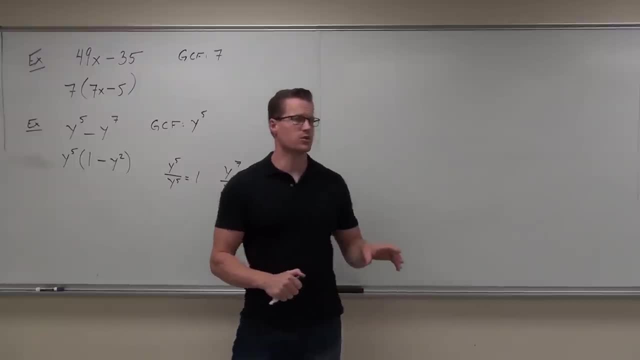 If you remember it, great. If not, we're going to cover it. Let's call it the difference of squares, and I'll show you what to do with that as we move forward. Okay, what I'd like you to do now. I'm just going to give you two examples. 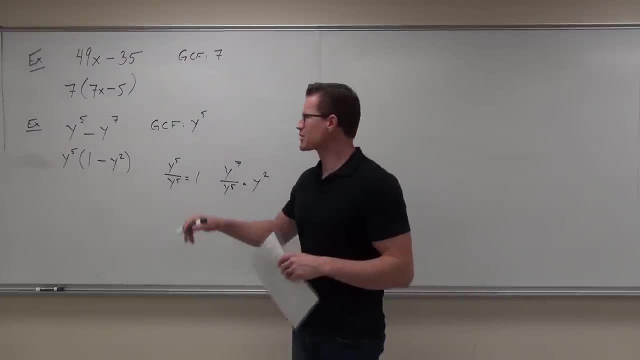 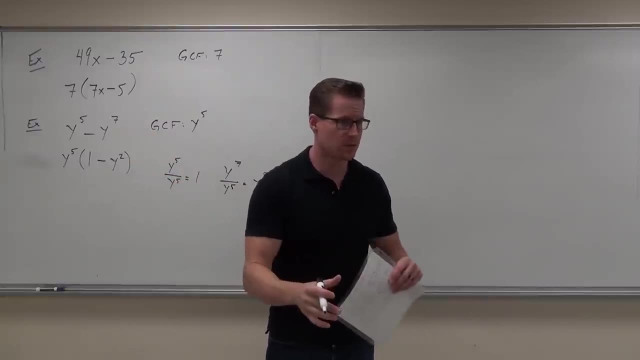 I want you to do them on your own, to make sure that you get this concept. When I do this, it's going to be really, really similar to the last two that I gave you. It's just so you can have that practice, so that I don't want you to completely phone. 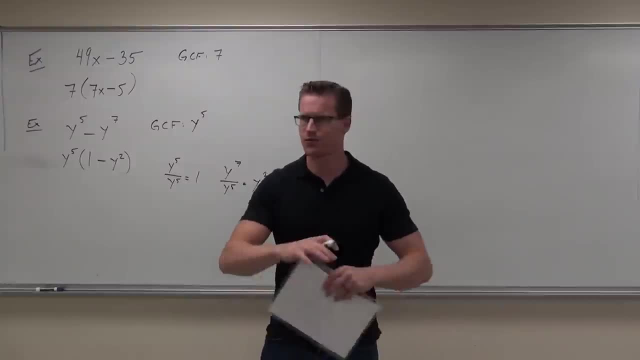 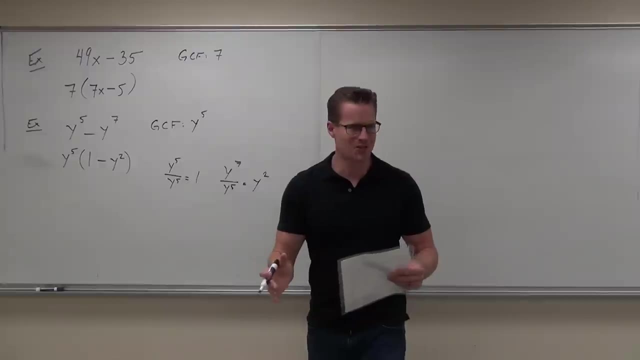 your notes. If you have to have your notes, okay, but try to do this fresh without having to go back, and that way you actually get it embedded in your head. You guys with me on this stuff? You're quiet today, Are you okay? 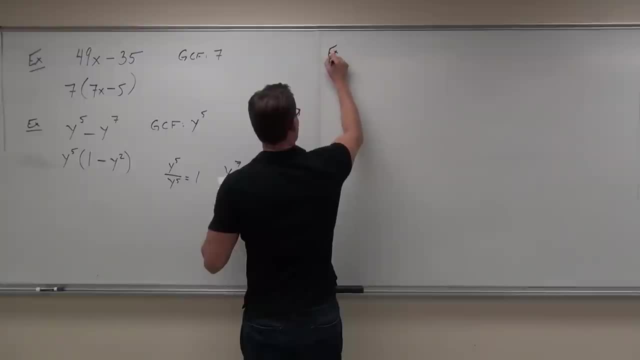 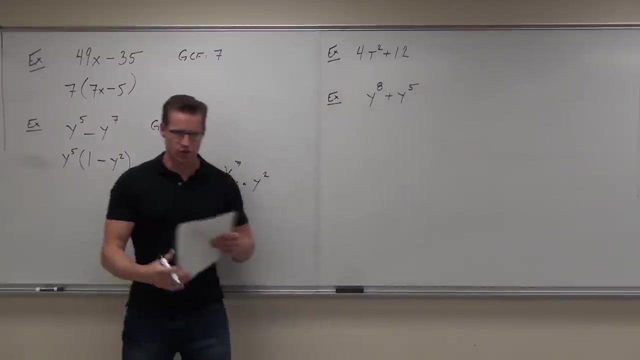 I'm excited. It might be that I'm extremely tired and running just purely off adrenaline, but whatever People on the video don't know this, but I had a baby in case, not me personally. Anyway, go ahead with these two. 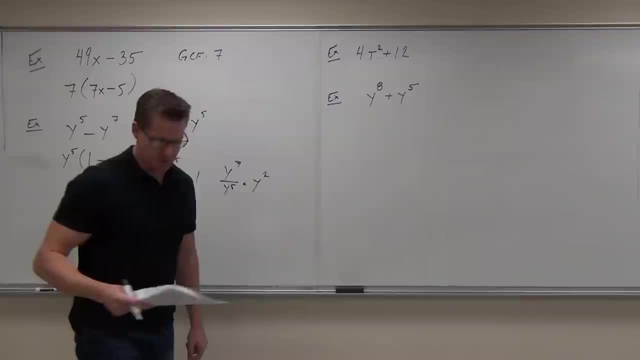 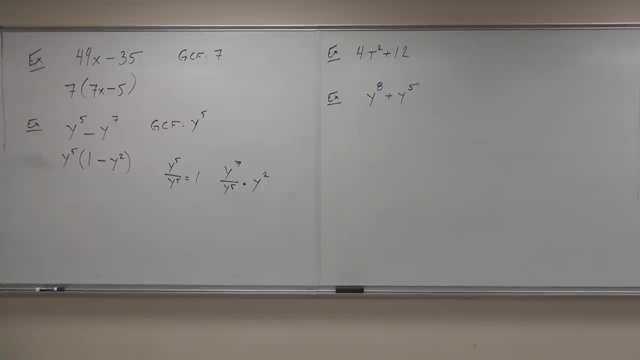 We're just working on factoring the GCF, so I want you to do that with these two. I love you. Say hello to my little girl, Hello baby, Hello Mary, Hello, You're wide awake. What's the matter? 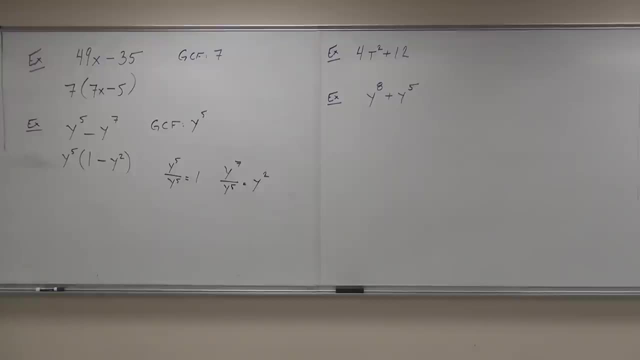 You're big, so you're a little bit bigger. Okay, You're a little bit bigger. Baby, I'm so glad you're not in an emergency room. She's a little bit bigger now, so you're going to have to go in and have this. 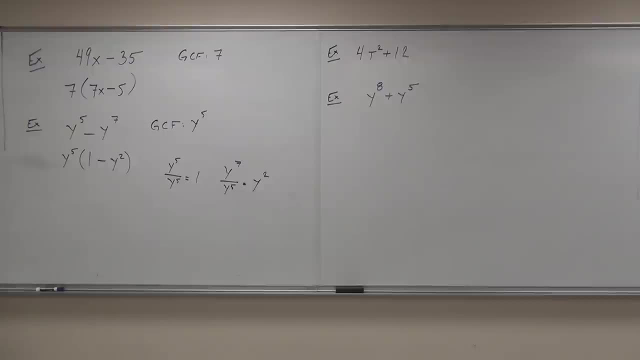 She's going to have to go on the floor. She's going to be a little emotional tomorrow. okay, Look at her face. She's going to be a little moody, Don't be ridiculous. She's going to be less emotional today. 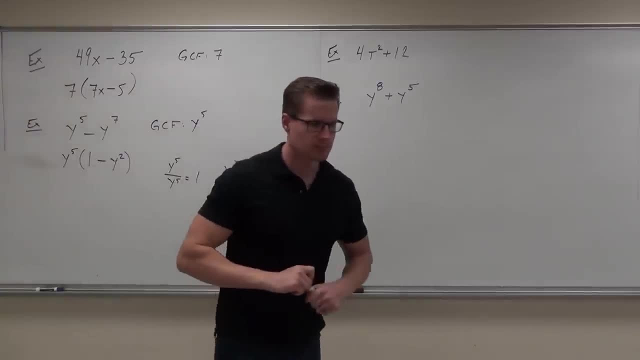 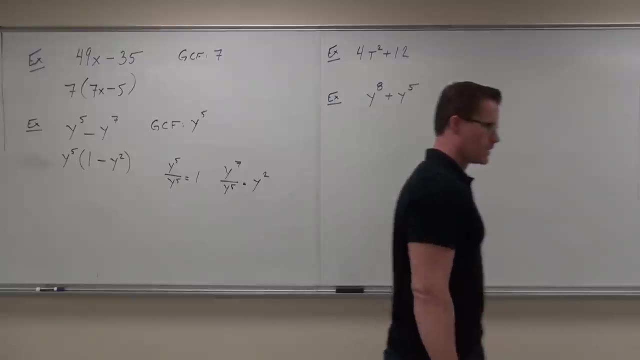 She's going to be very happy. Look at her face. Can you see the difference? The difference is she's a little bit more of a baby. So the idea is factoring is the opposite of distribution. instead of multiplying, we are dividing. 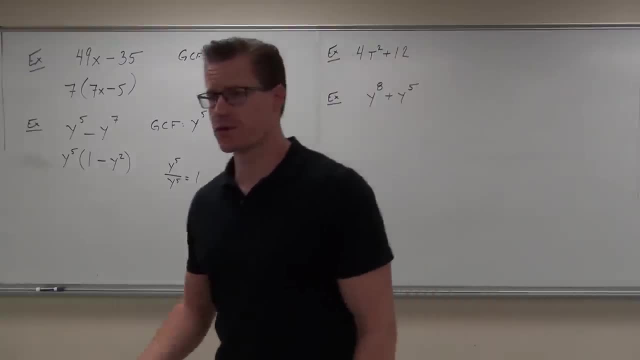 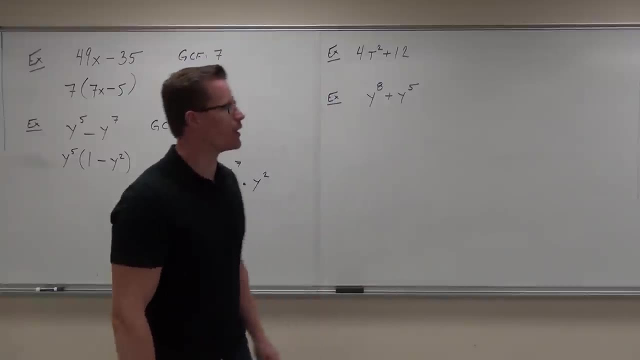 So the first thing we have to find is what will divide all of our terms. Remember, it's all of the terms here. In our case we only have two. in the next examples we're going to have three, four, so forth and so on. 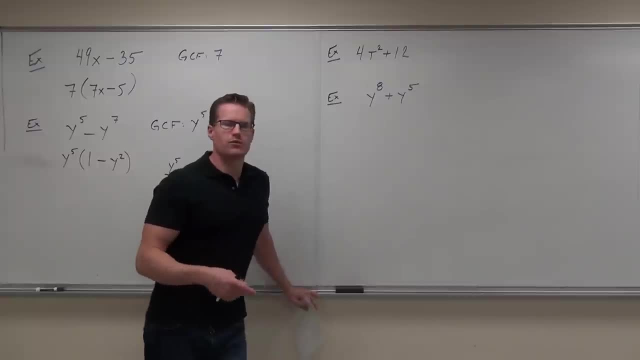 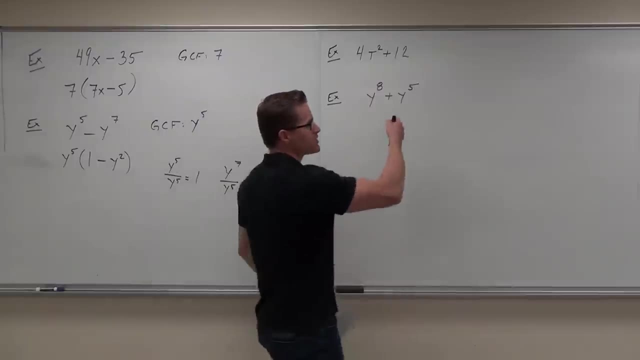 So for us, in the first example we're looking at 4t squared plus 12, we've got to find a number or a variable or both that will divide both of those terms. What number is that Four? So if you want to write GCF, great, if not, that's okay. 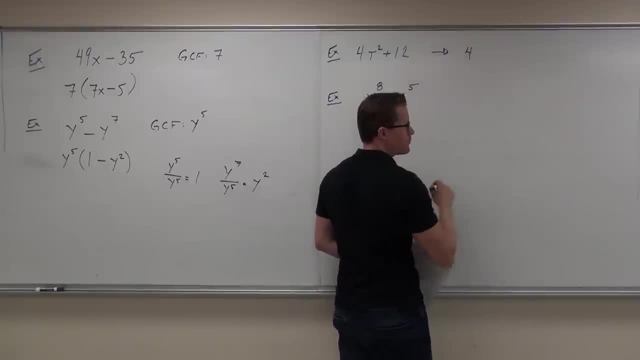 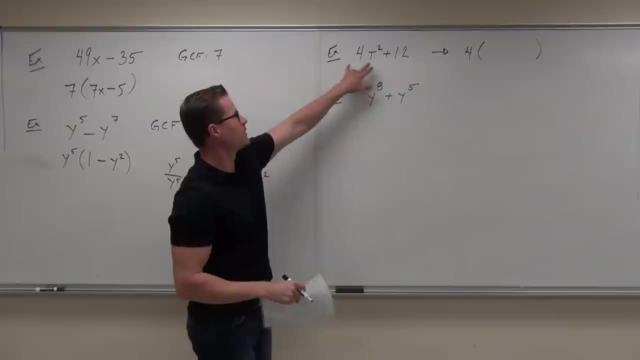 All you've got to do is write the GCF whatever you have in front of. some parenthesis factored means we're creating parenthesis and then start dividing What's 4t squared, first term divided by our GCF. 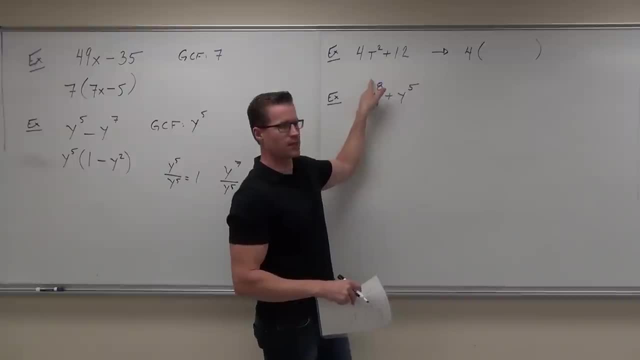 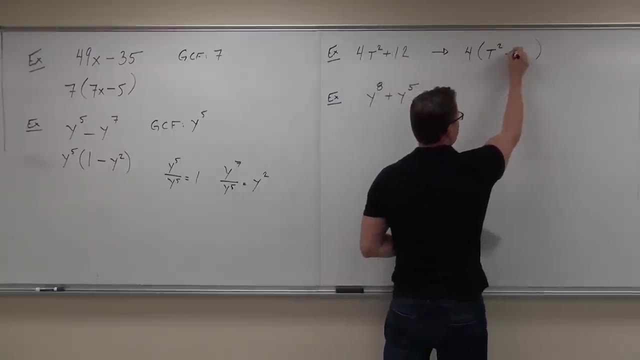 So 4t squared, divided by 4, you can even think of it like that. what is the answer to these questions? Let's see the first term inside of our parenthesis: Is the plus going to change? No, Okay, 12 divided by 4, our GCF. 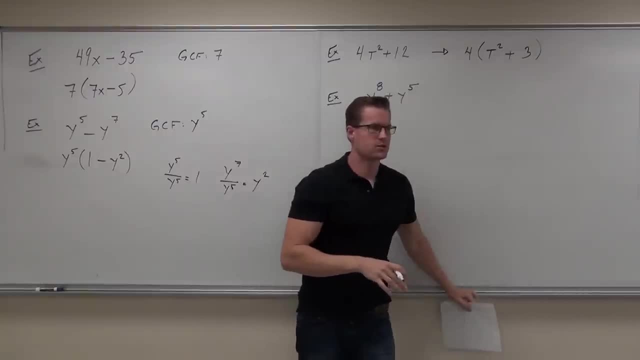 Have you double checked it to make sure that you're right? Don't go any further before you double check it. You've got to make sure. okay, I know it seems silly, I don't know. it's a pretty easy one. yeah, okay, it's easy. 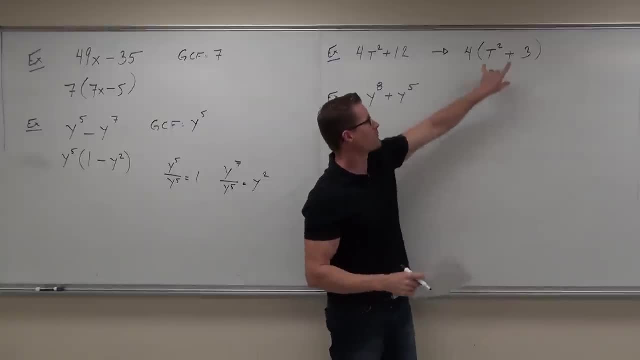 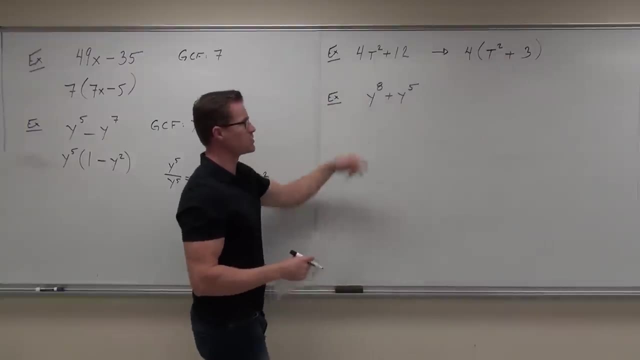 but later on, when they become more difficult, double check it. Can we go any further here? Is there a number or variable that goes into both those terms? No, Relatively. prime is a key word. we're good to go. we can double check the distribution. 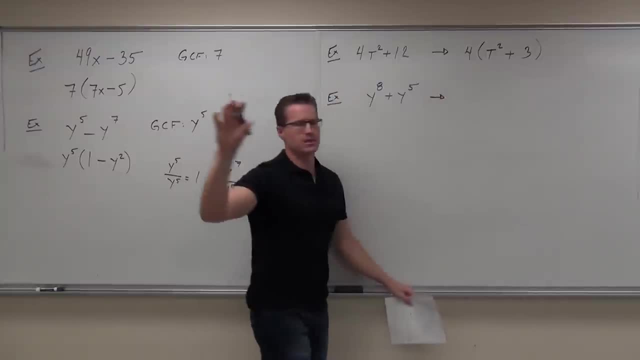 in our head Next up. Tell me the GCF. I just want the right side people, these are two terms. tell me the GCF with y to the 8th plus y to the 5th. what's the GCF there? 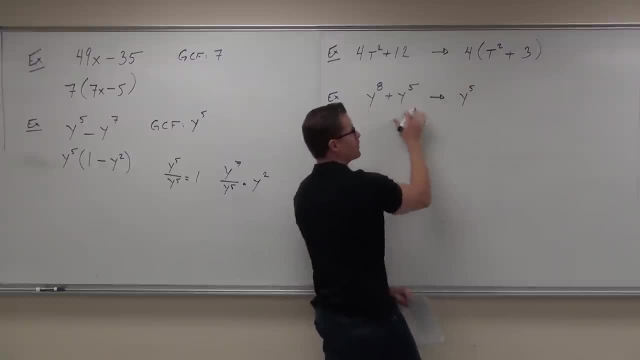 Y to the 21st. Cool, That's the largest power of y. that is common to both of them. Y to the 8th. it's too much for this guy. remember? did I give you the lunch analogy, Mm-hmm. 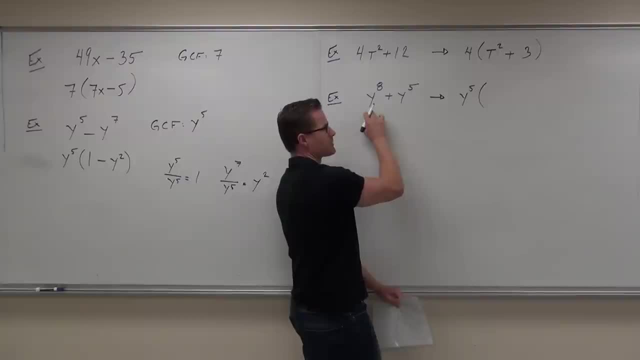 Going along, okay. Y to the 8th. if you need to write it down, maybe write it real softly under there: divide by y to the 5th. what's y to the 8th divided by y to the 5th? 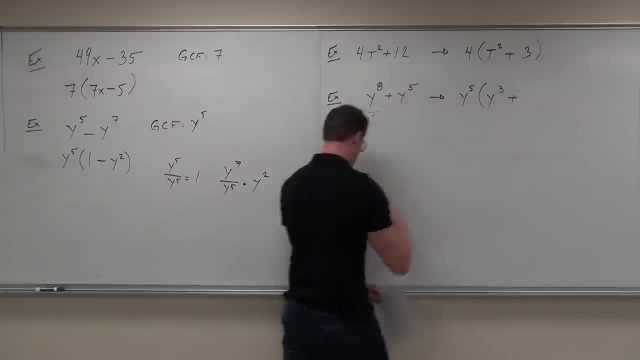 1. Plus, Plus, Plus. Okay, cool. And now y to the 5th. divided by y to the 5th, what is that? 1. Show of hands. if you got those two, That's great, that's fantastic. 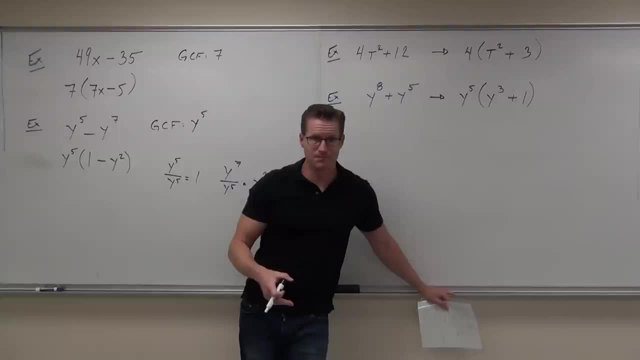 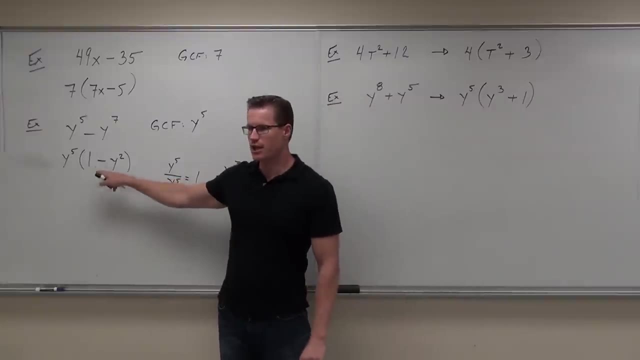 That's factoring the GCF. Are you ready to step it up just a little bit, Mm-hmm. By the way, in the previous examples- this one and this one- this is called a difference of cubes. I'm going to show you how to do that later. 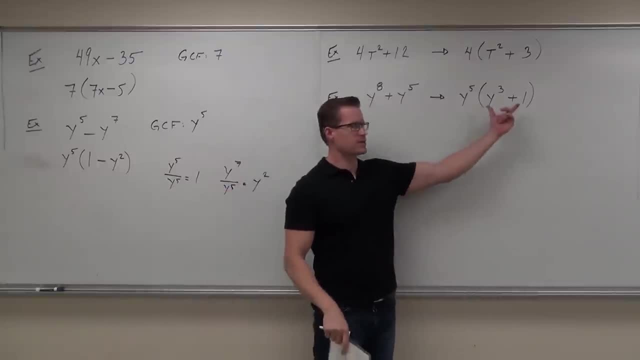 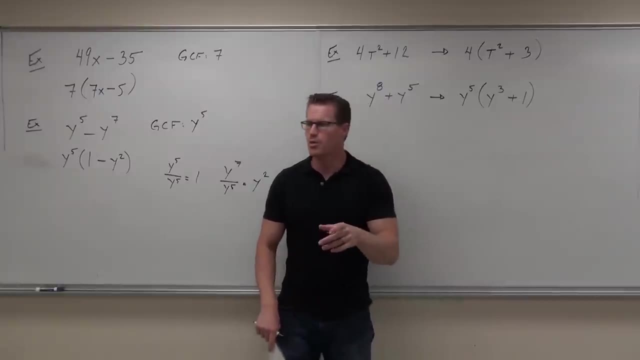 This right here is called, sorry, difference of squares. this right here is called a sum of cubes. We're going to talk about how to factor this. You can actually keep going on this problem Right now as far as the GCF you're done, but we can do other kind of brands of factoring. 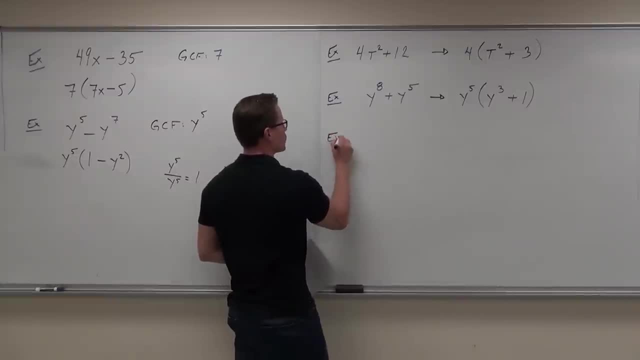 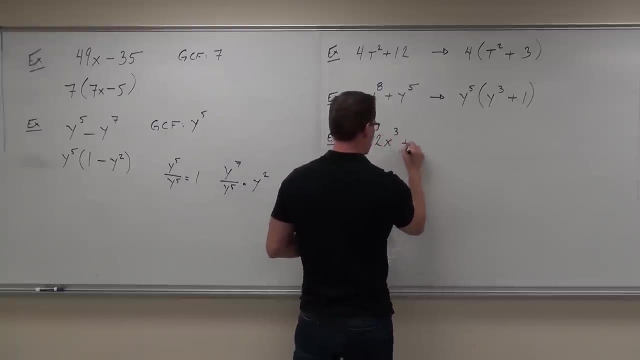 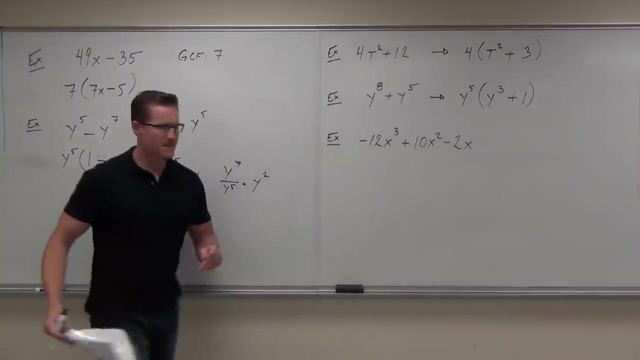 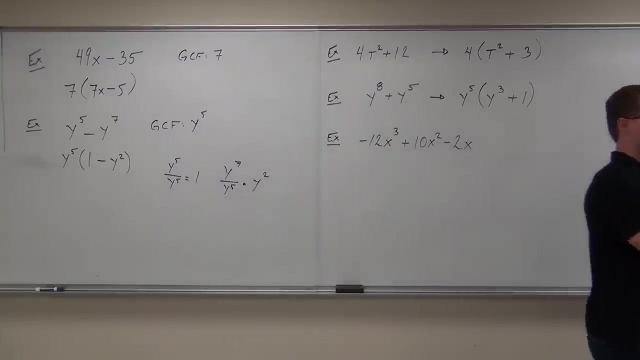 as we go through these problems. So let's start getting towards that. Oh dear, all right. So negative 12x to the 3rd, We get a plus 10x squared, minus 2x left side people. real quick, how many terms do you? 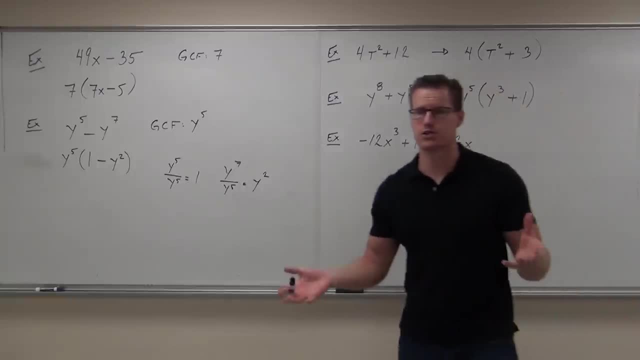 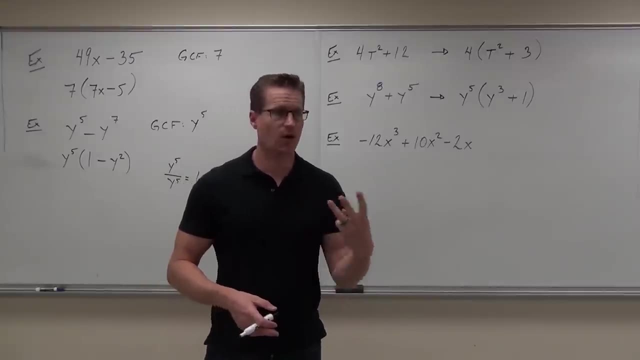 have Three. So if we're going to factor by the GCF, which is always our first step, we've got to have a GCF that goes into just two terms. right, Three terms, All three terms, Mm-hmm. 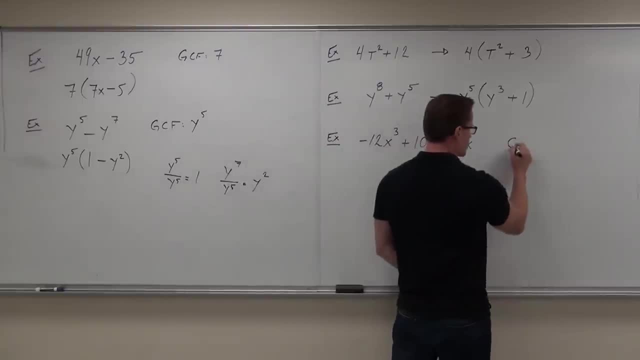 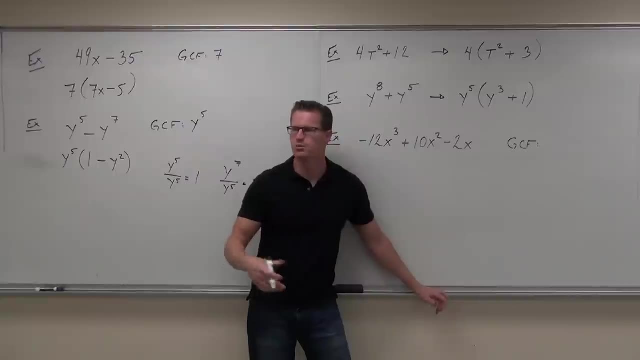 All three terms. So in our idea for finding a factor by the GCF, you've got to come up with something, some factor that goes into all the terms, not just one or two, but all three of them, four, if you have four, everything. 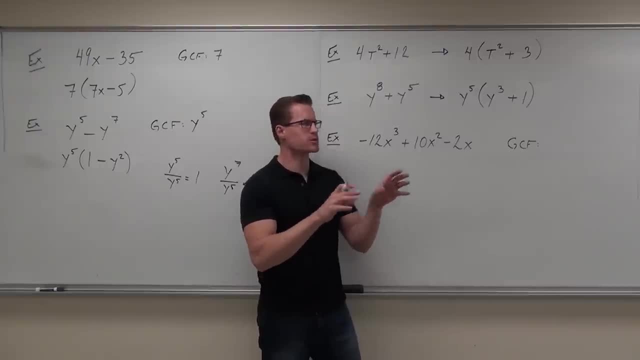 So let's look at the numbers first. Remember we can do numbers and variables separately. Let's look at the numbers. I've got negative 12,, I've got 10, and I've got a negative 2 for my coefficients. 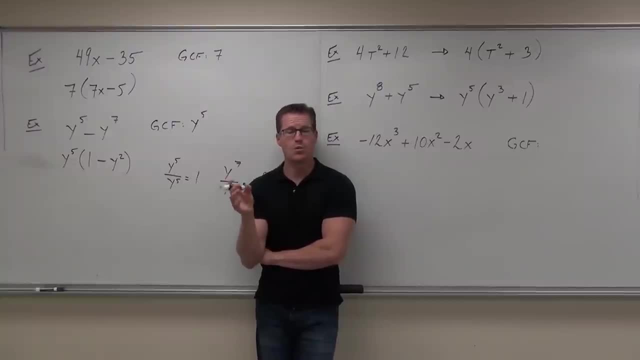 Can you tell me a number that goes into all three of those? Remember that it doesn't have to be negative or positive for it to have a factor, So negative 12 doesn't really matter. What number are you going to pick? Two: 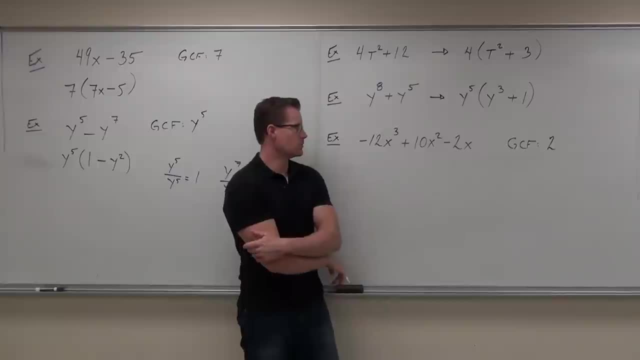 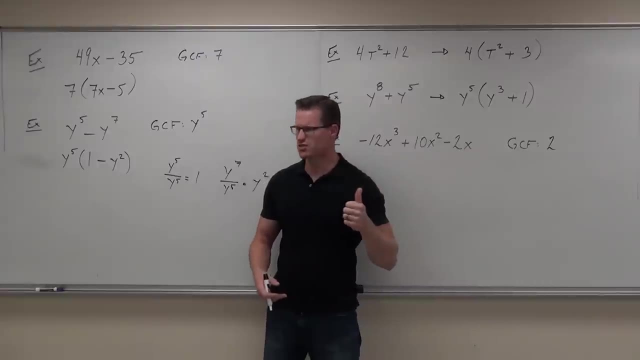 Two, Okay, Cool. Two goes into 12. And 10. 10. Mm-hmm, Two, Cool. That means that we can divide all three of these numbers by two. Is that true? Yes, That means we can factor by it. 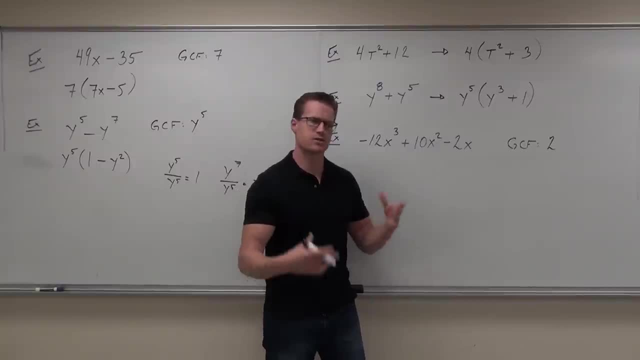 Is that the biggest number that goes into all three of them? Yes, Well, you want the biggest one. It's the greatest idea. Now we look for the variables. Remember, we do them separately. So I've got x cubed, I've got x squared and I've got x. 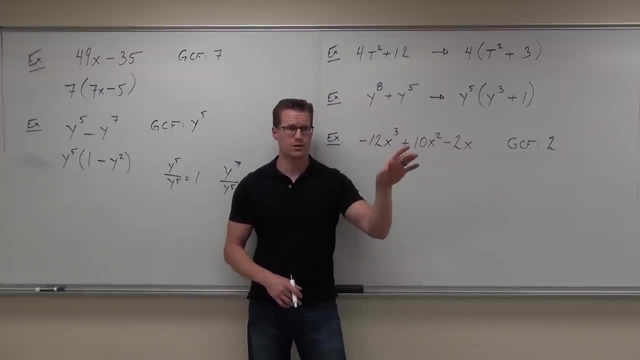 Can you give me a variable that goes to all three of those factors, all three of those terms? Yeah, x, And if we put that together, that right, there is our GCF. Okay, So in the next step, what am I going to do? 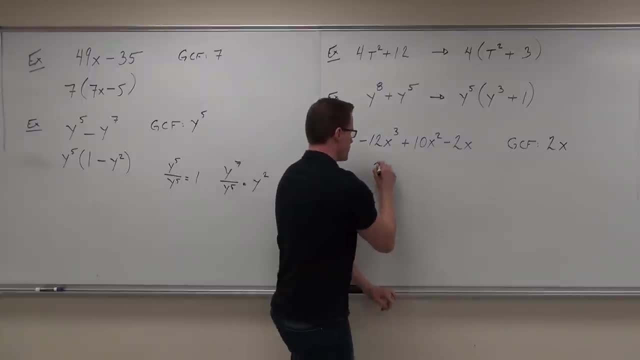 Put it outside the parentheses. Okay, So I've got my two x. I know factoring means parentheses. Quick question: How many terms are going to be inside the parentheses? Three, Does this get rid of terms? No, So if you have two terms, you're going to have two terms and a factor. 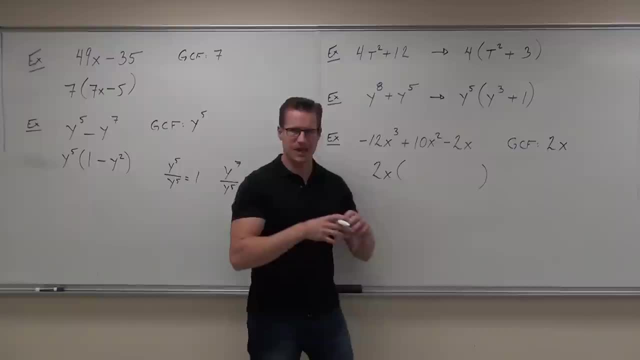 If you have three terms, you're going to have three terms and a factor. It's actually making it look a little bit bigger, isn't it? So inside there's going to be the same number of terms, But outside you're going to have this factor that you've divided out. 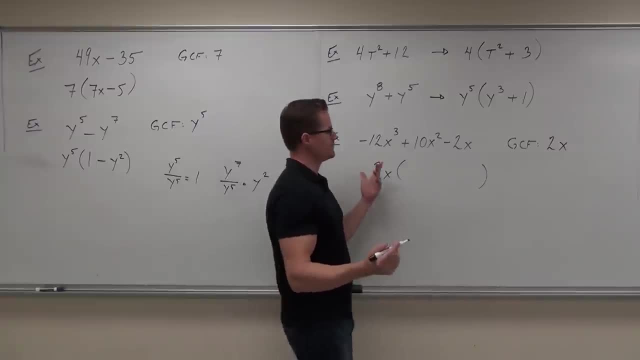 Now we start dividing. If you need to do this off to the side, do it. There's no sense in trying to do this in your head and getting it wrong. If you have trouble dividing this by this- and that's what factoring is- just write it. 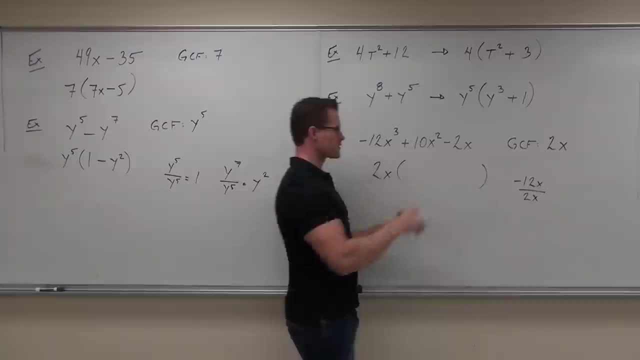 out there Negative 12x divided by 2x. That's fine, I don't mind seeing- well, I do mind that one- Why It's wrong. If you do that, then sure that's okay. How much is negative 12 divided by 2?? 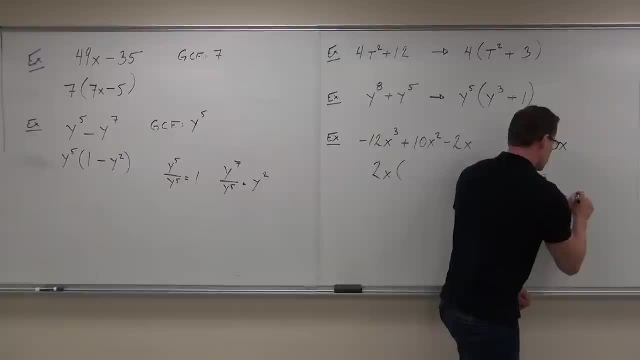 Negative 6x squared. Be careful, What is it? Negative 6x squared? Yeah, x cubed, divided by x. Remember this is x to the first. So if you subtract them, 3 minus 1 is x squared. 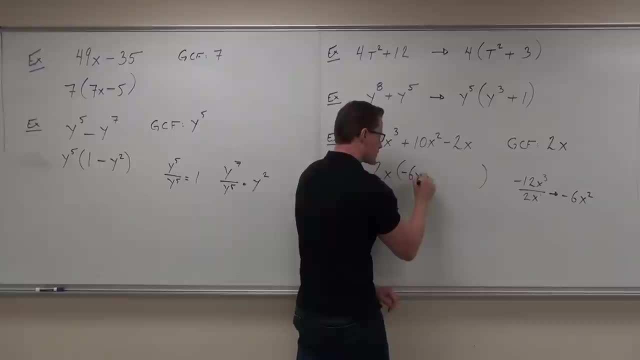 That is your very first term. If you want to write this off to the side, do it. If it helps, you do it. If it doesn't, if you can do this straight in your head, that's fine too. I don't care. 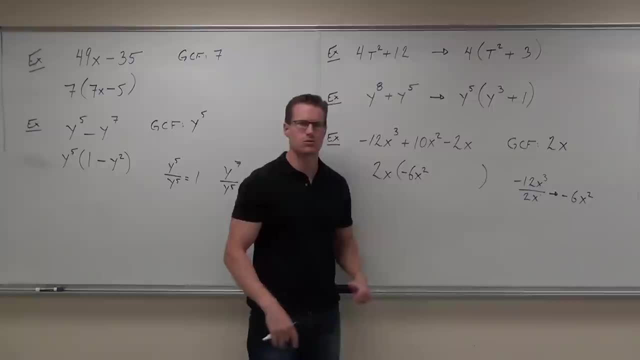 You need to know how you guys learn. So if you struggle with this now and always get the wrong answer, write it out. If not, if you're quick, it makes perfect sense. I can do it in my head. Cool, Do it in your head. 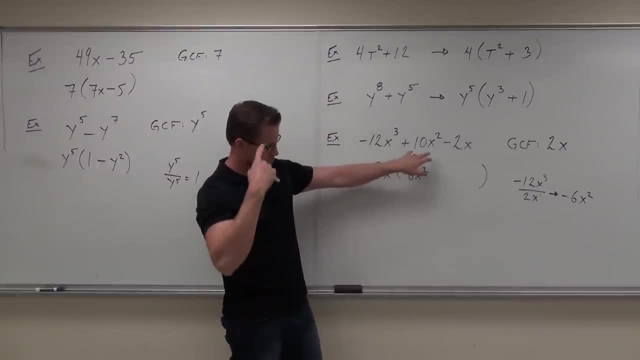 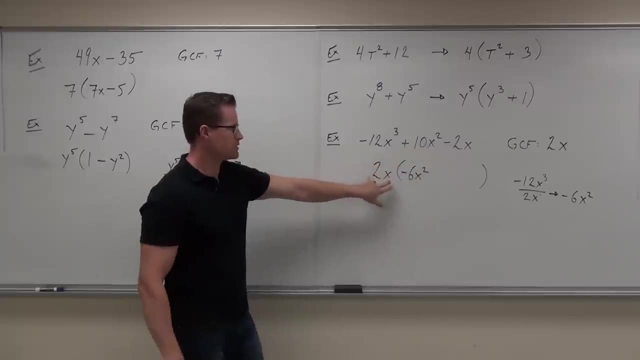 Let's do the next one. I'm going to do this one. just in our heads here, How much is 10x squared divided by- because, remember, we're factoring- divided by 2x? So 10 divided by 2 gives us: 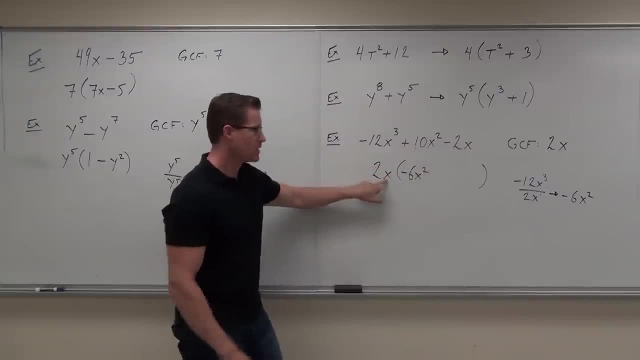 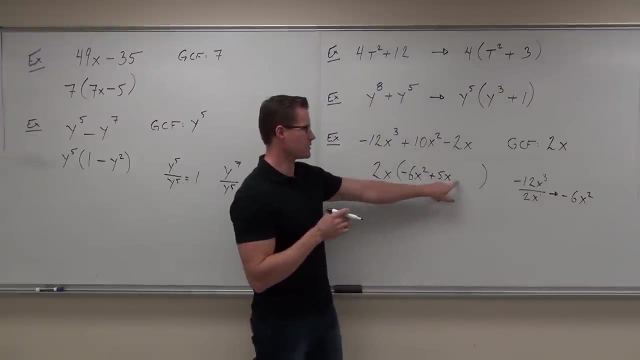 Minus And x squared divided by x gives us X Plus or minus Plus. Lastly, plus or minus here, Minus And then, oh yeah, that's a nice one. How much is that Minus? 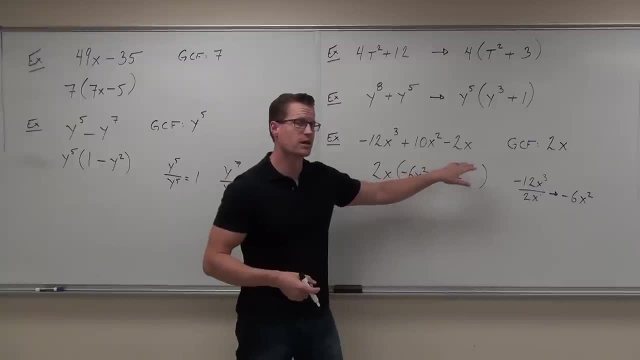 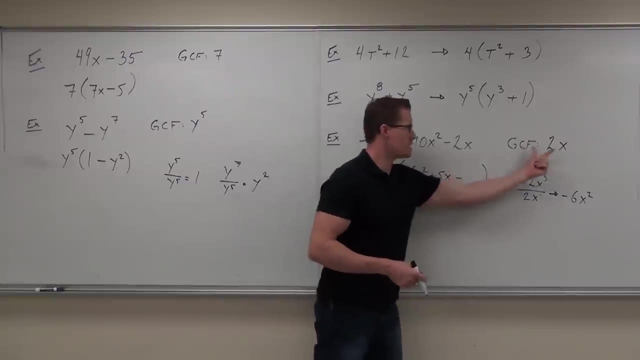 Minus 2x divided by 2x 1.. Notice how, when you're factoring, you don't get rid of terms. They can change to 1s, but that's the lowest that you can get right there. So when you have a GCF that matches up with one of your terms, you don't get 0. 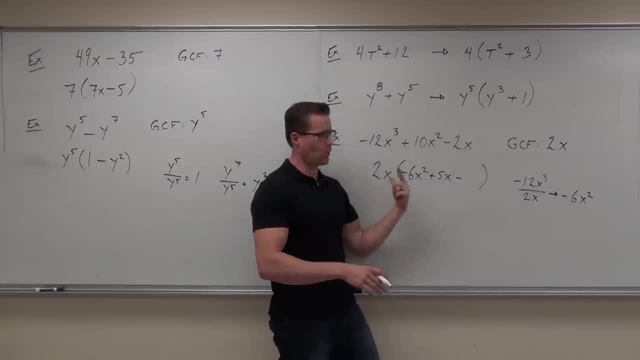 You get 1, because something divided by itself is always 1.. That's the idea. Show me if this feels all right with y'all. OK, Now can you check it? Yes, Should you check it? Yes, Should you check to see that these are all relatively prime. 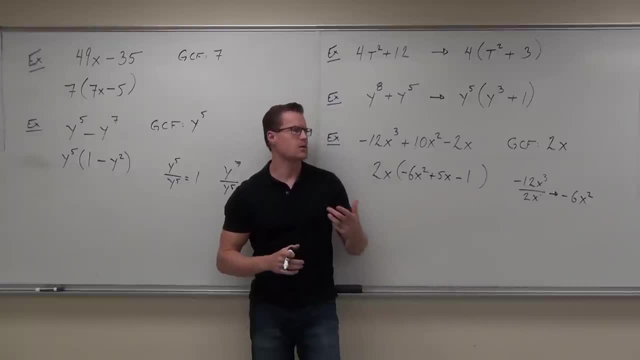 Yes, Don't go any further before that. Now I'd like to do something else. A lot of times in math it's really, really helpful to factor so that two things happen. One, that your polynomial- this is just a math expression- inside here, with more than. 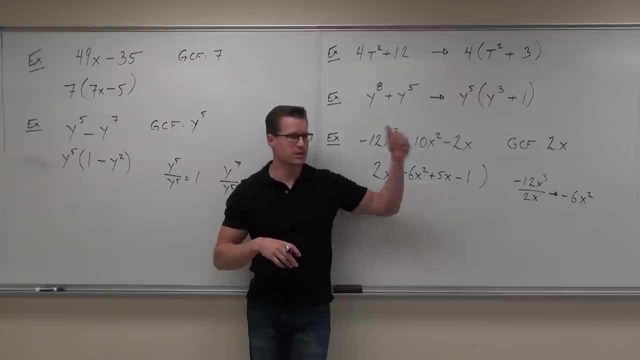 one term, that your polynomial is in order, And order means that it goes from largest to smallest exponent ending with a constant. So, for instance, this: out of order. See what I'm talking about: Mm-hmm, This is out of order. 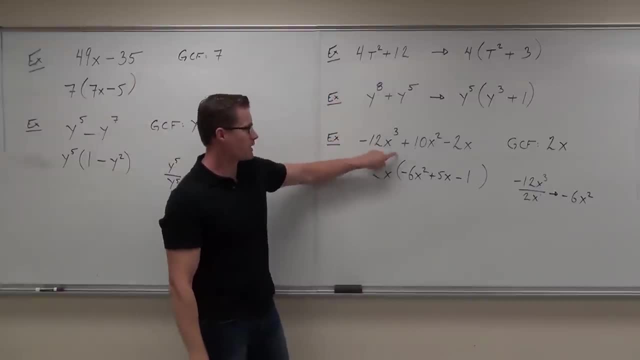 This is in order. This is in order in order. in order. Do you guys get it? This is in order. We factor so that that happens. We like to put things in order even before we factor, So here we probably would have done this a little different. 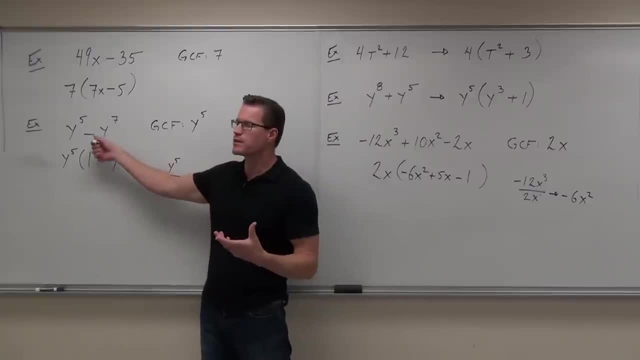 Second thing: we also like to factor so that the first term of the polynomial, that, is in order. I'll say that again, because some of you guys are zoning out already. Don't zone out, Zone out. You'll want to factor so that, firstly, it's in order. 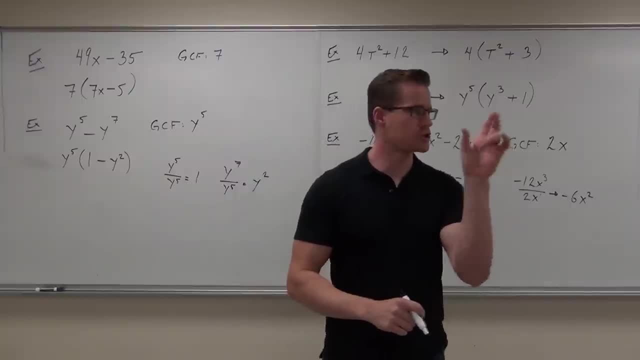 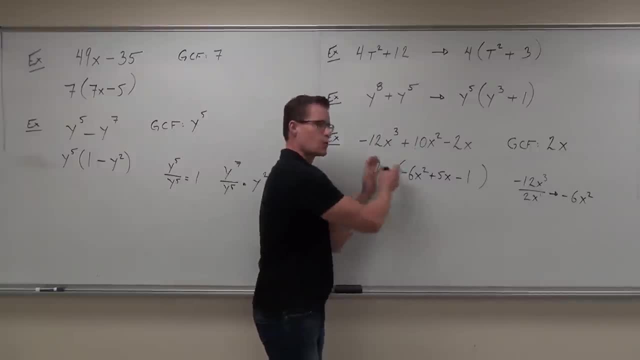 So you get it Mm-hmm. So that's positive. That helps a lot, because the next techniques we're going to do are dealing with these guys, How you factor this and it's really really hard if that is negative. 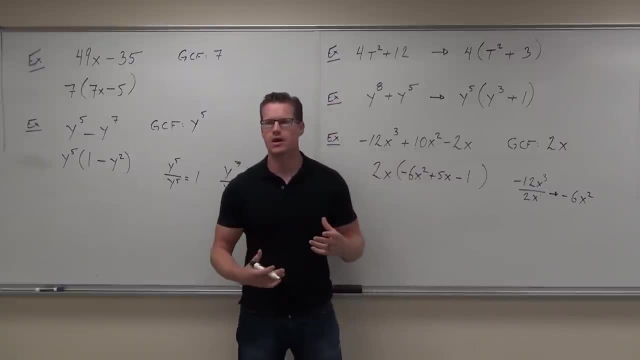 Does that make sense to you, Mm-hmm? So when you do this process, when you factor out your GCF, you could have one of two answers. One could be just like this: Two X, and this is perfectly fine as far as factoring the GCF. 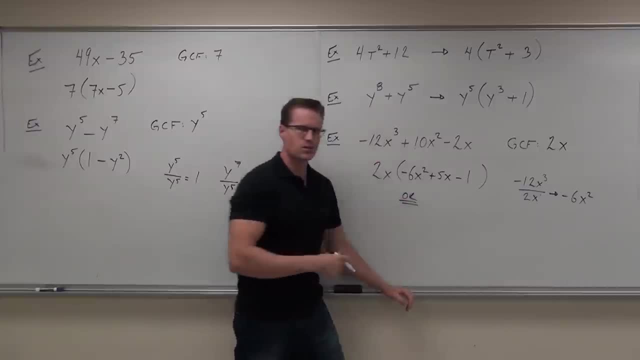 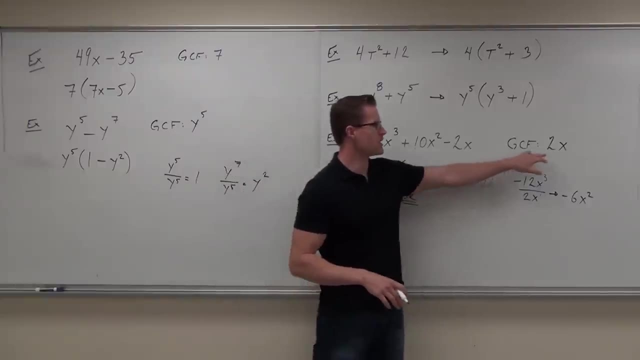 But there is an alternative, and this is the one that I'm going to prefer, because it makes the rest of our lives so much easier. lives easier, instead of going just with 2x. check this out. follow the logic. here Is this in order from largest to smallest as far as the exponents go: 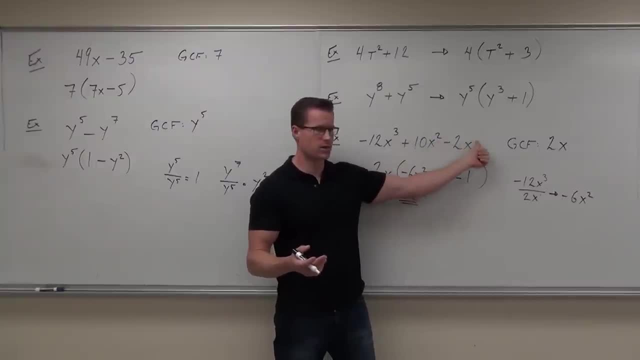 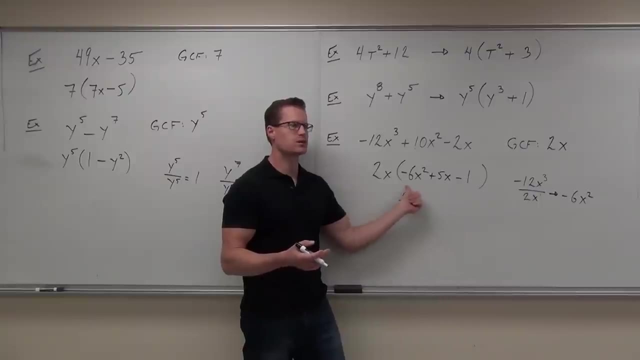 Yes, That's great. that's what we want. 3,, 2,, 1,. you with me? When I factored, I factored 2x. did I get a positive here? This is what I want, to be positive. 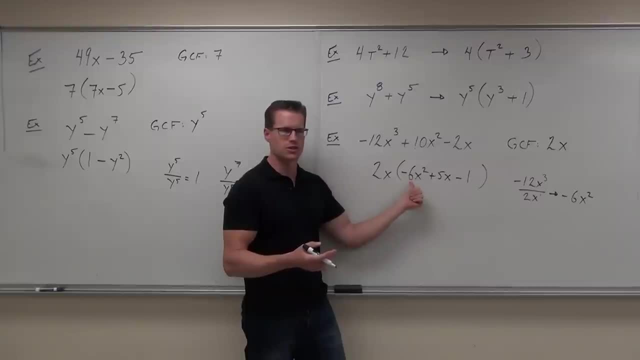 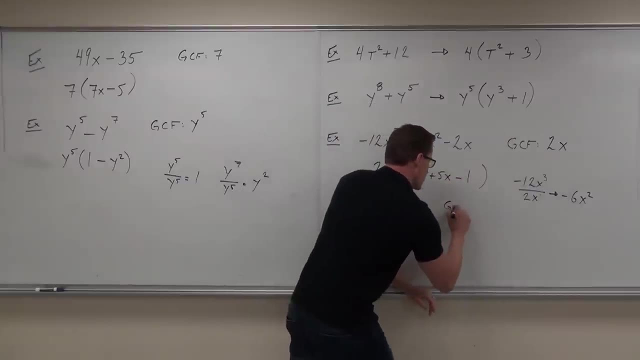 How can I change this to be positive? What would I have to do to my GCF? Multiply by a negative, Make it negative 2x. Okay, so instead of having the GCF of 2x, let's say I did a GCF of negative 2x. 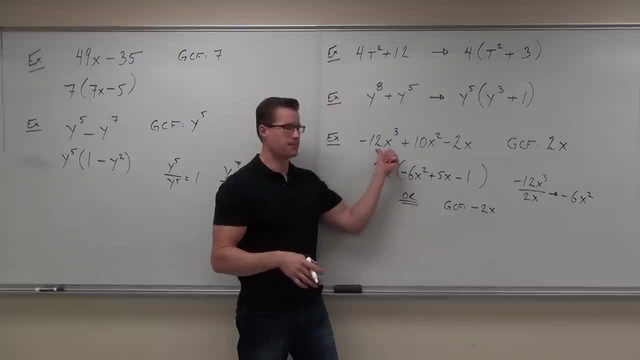 Is it possible? Yes, Will negative 2x still divide that Yeah, And that Yeah And that Yeah. What's going to happen to all three of my signs? They're going to change. That's the idea. So you have choice here, okay. 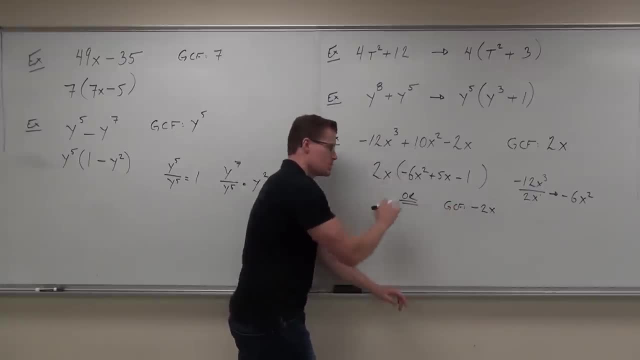 The both of these are going to be absolutely correct. but as far as continuing the process of factoring- it makes it a lot easier If you factor so that your first term becomes positive. the one thing you've got to worry about is that you don't mess up the rest of your signs. 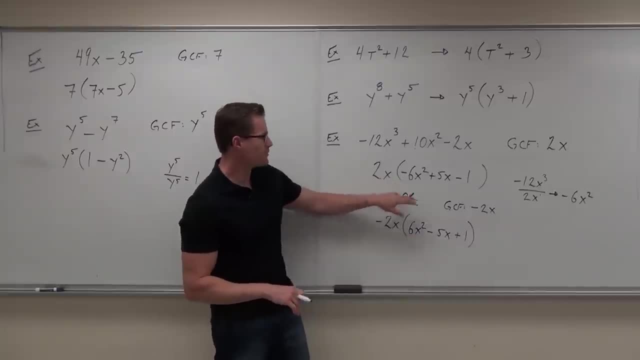 So I'm going to lead you through it one time, real quick, and then we're going to continue with another problem. If we factor out the negative 2x, tell me something. what's negative 12x to the third divided by negative 2x? 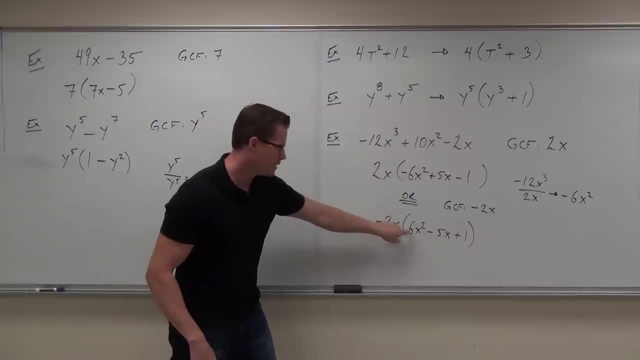 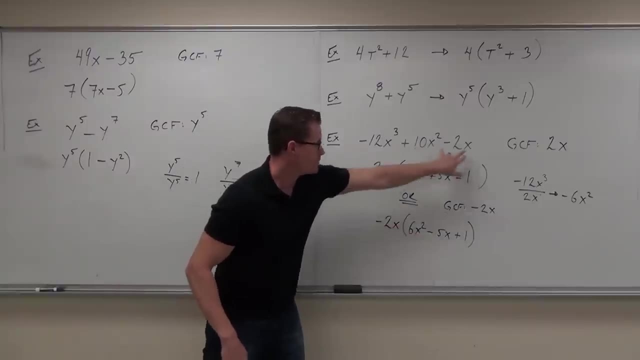 Remember, a negative divided by a negative is a A positive Bam. So we've got our subject squared: Positive 10x Positive divided by a negative is a Negative. 10x Negative: 10x Negative divided by a negative is a. 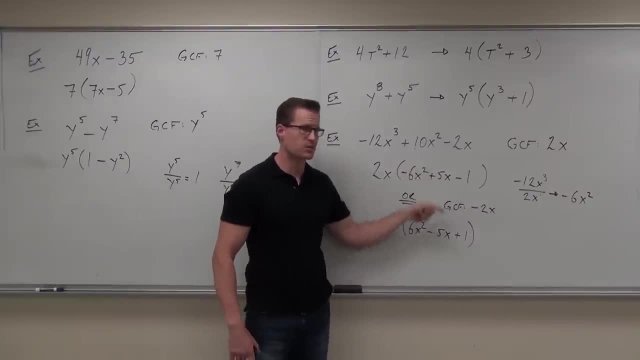 A positive. Are these the same? Yeah, No, Yeah, These are well. do they look the same? No, Do they represent the same thing? Yes, Yeah. Which one's going to be nicer for us? It kind of depends on the context of your problem. 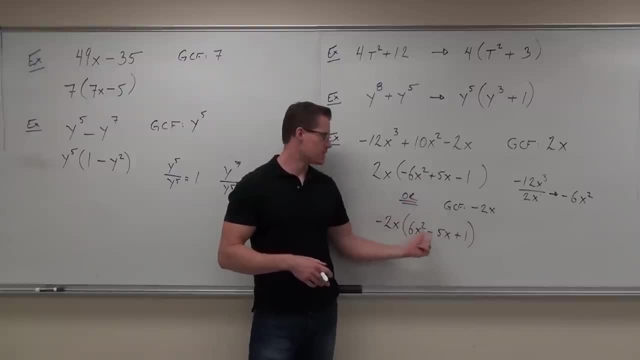 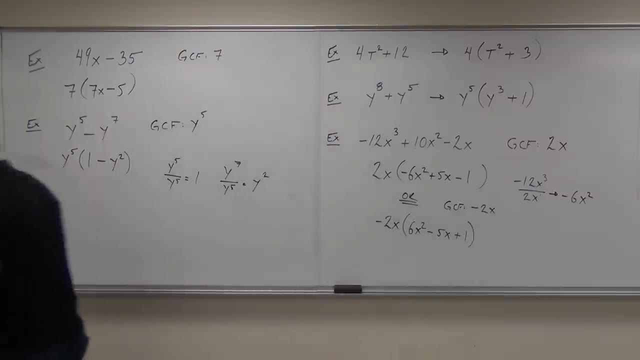 This, technically, is factoring out GCF, So is that one? This one would be easier to work on. after this, though, Show your hands if you understand the difference there. Okay, cool, Tell you what I want you to try. a couple of them on your. 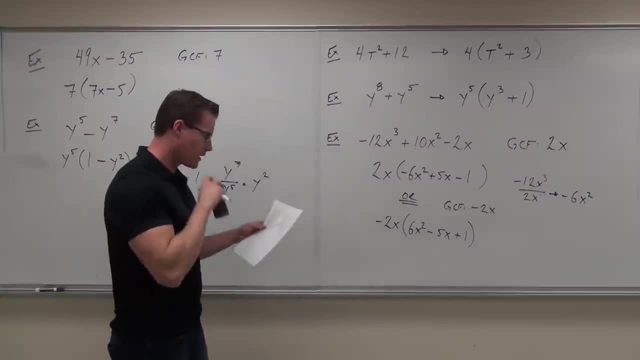 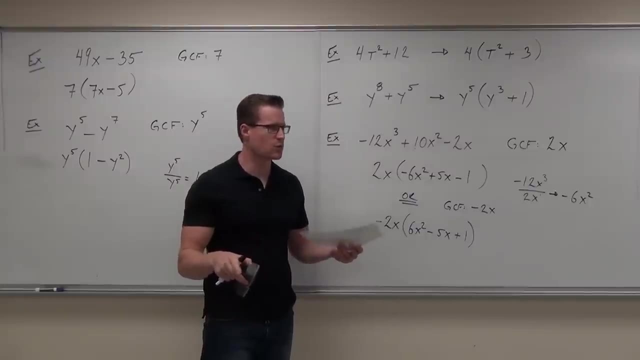 In fact, what I want out of you. I'm going to give you two of them that I know that you can do really well, And I'm going to give you one that's going to challenge you just maybe a little bit. See if you remember how to do this. 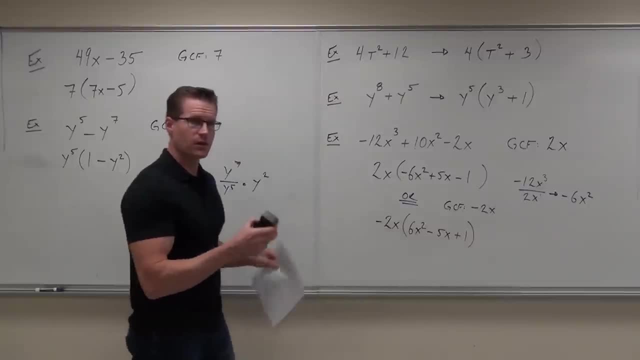 Are you guys ready for that? Yeah Question. You know how you said: like when you check and make sure everything's relatively prime, Yeah, What happens if it's not like, and it's still correct, If you have some terms like two or three terms that are not relatively prime. you did. 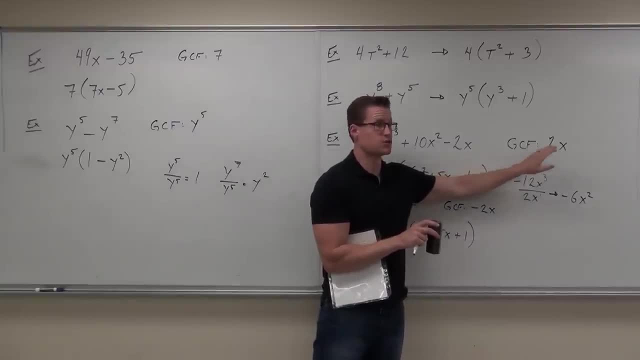 this wrong. If you do the GCF, not just the CF, the CF is common factor, right. If you do the greatest common factor, your terms will be relatively prime. They have to be, Otherwise you would have something else that would divide all those terms and that would 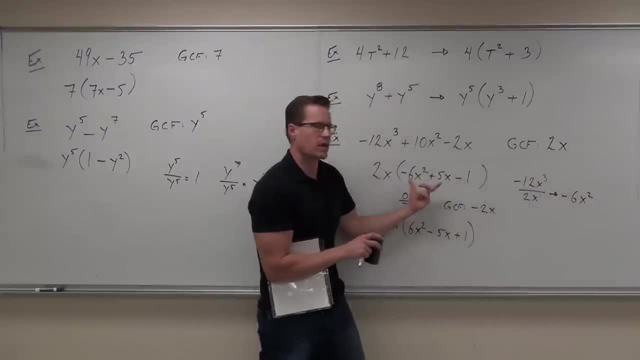 be part of your GCF. Does that make sense? Yeah, Which is why I'm always having you check. I don't want you to just factor out Y here, because if you factor out Y, these things are not relatively prime. But well, never mind then. 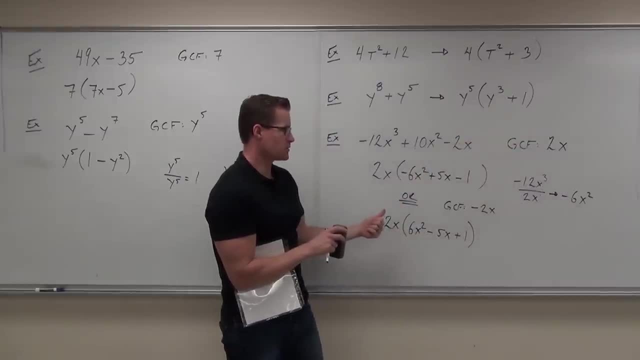 No, keep going, Because I was going to say six isn't really relative to prime. No, keep going, Because I was going to say six isn't really relative to prime. No, keep going. Okay, What is relatively prime? With what? 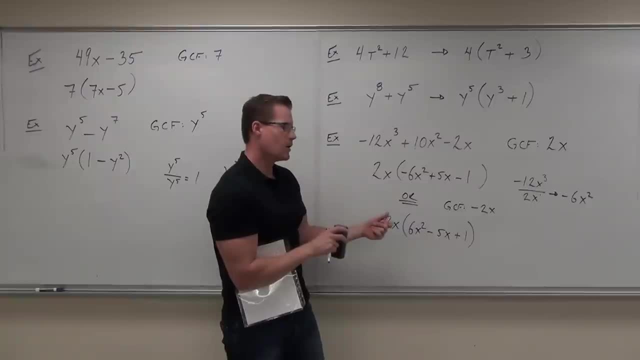 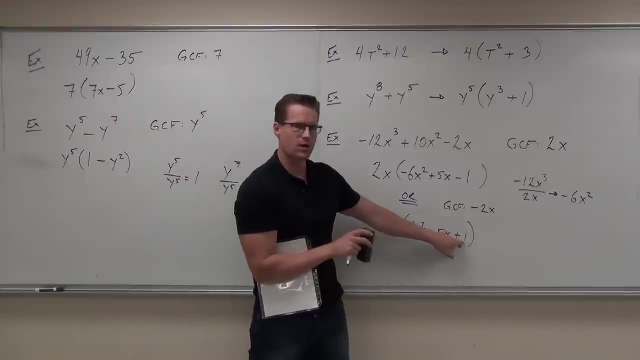 Because six can be divided by two and three. Okay, What relatively prime means is that when you look at this number and this number and this number, nothing divides all three of those numbers except for one. It's not just that the six. I mean, yeah, you're going to have some numbers that you 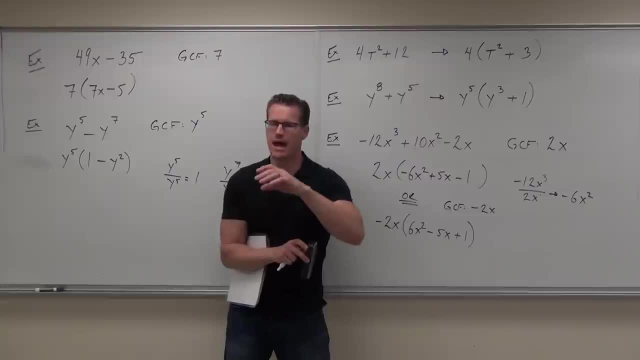 can factor the numbers individually, but what relatively prime means? as this number relates to a different number, only one divides it. That's what relatively prime means, Not that you can't decompose it as a composite number, That it's kind of a different thing. 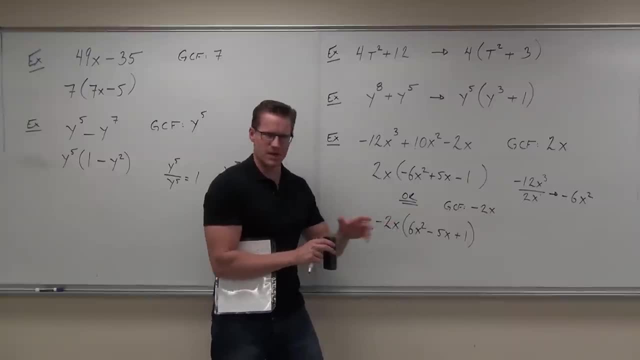 Am I making my point that those are a little bit different of an idea? So here's what I want from you. I want you to do the first two problems. I'm going to say that you're going to be just fine on these, because they're things like: 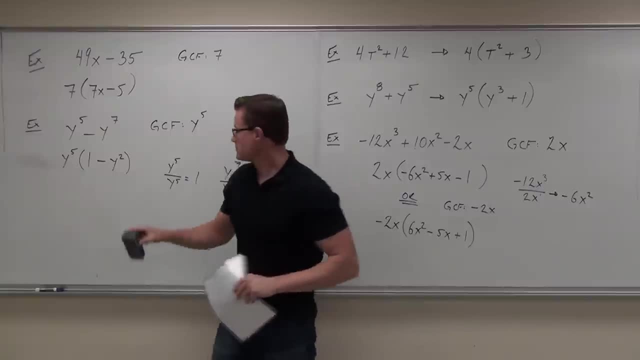 what we've done. The next, the last one that I'm going to give you a little bit challenging. I know you can all do it, but pay attention to what the actual GCF is. Are you guys ready for this Mm-hmm. 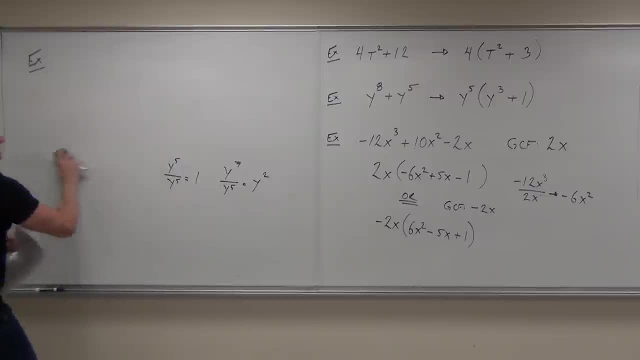 Okay, So the last one that I'm going to give you a little bit challenging. I know you can all do it, but pay attention to what the actual GCF is. Are you guys ready for this? Mm-hmm. 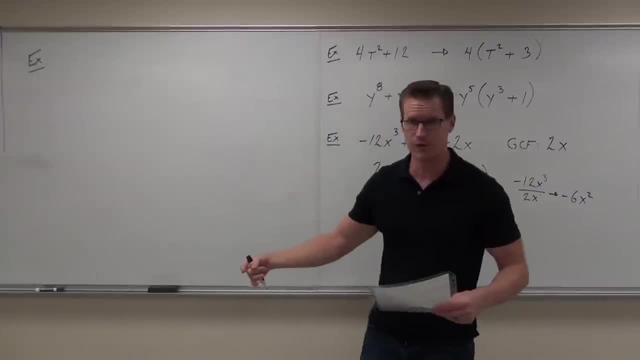 Okay. So first one: I want you to remember that the first two problems are going to be just fine on these, because they're things like what we've done. The next, the last one, that I'm going to give you a little bit challenging. 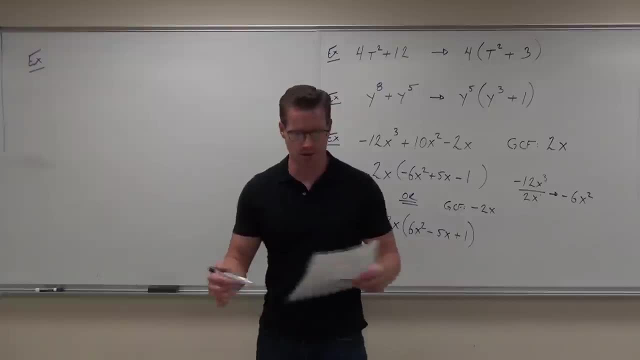 I know you can all do it, but pay attention to what the actual GCF is. Are you guys ready for this Mm-hmm? Okay, So first one. I want you to remember that the first two problems are going to be just fine on these. 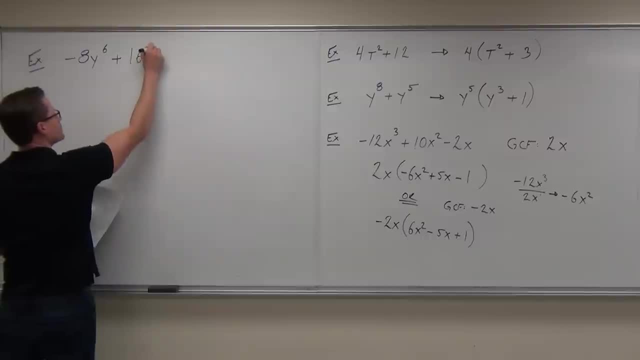 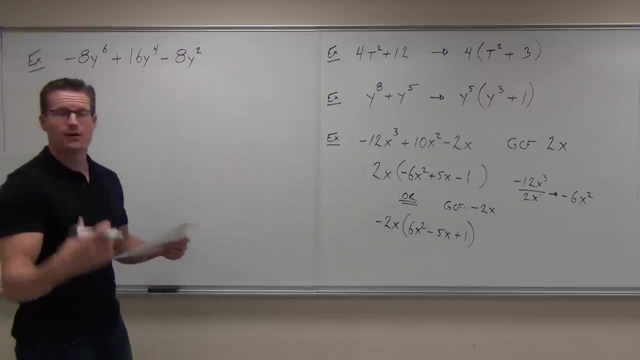 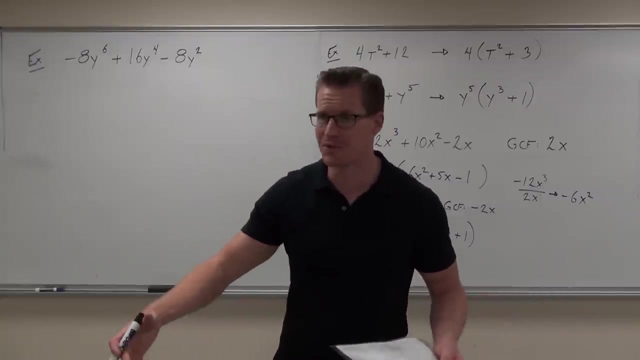 because they're things like what we've done. Am I making my point? Am I making my point correctly? To identify the GCF, this is up to you. you can use a positive or negative, I don't care. you know how I would probably do this problem. 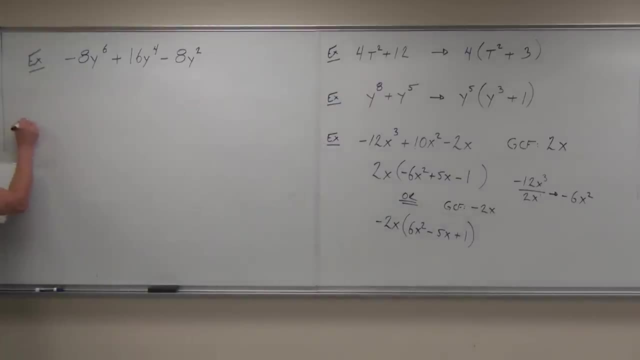 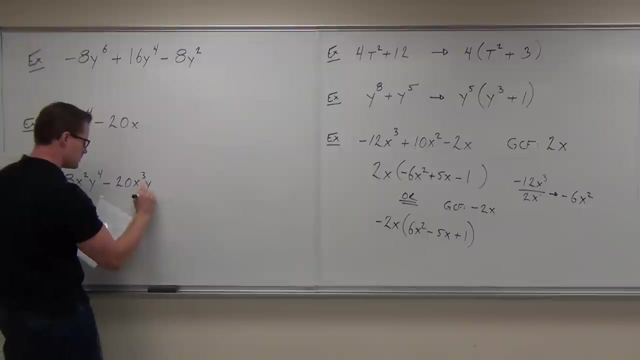 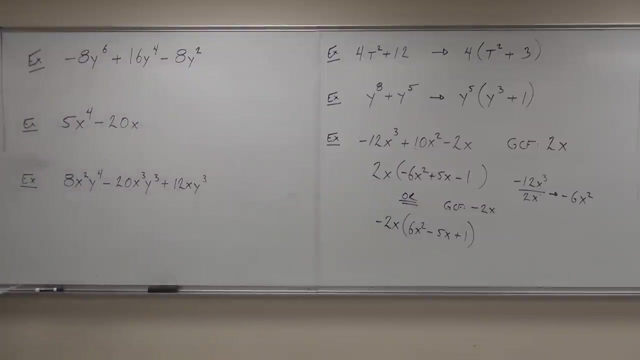 So pick the correct GCF and factor it, and then after that I want you to do this one. This is another one that I think you'll have no problem with. This last one may be a little bit challenging. I know you can do it. okay, there you go. 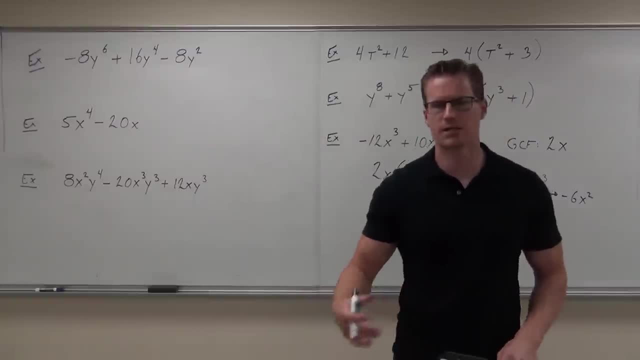 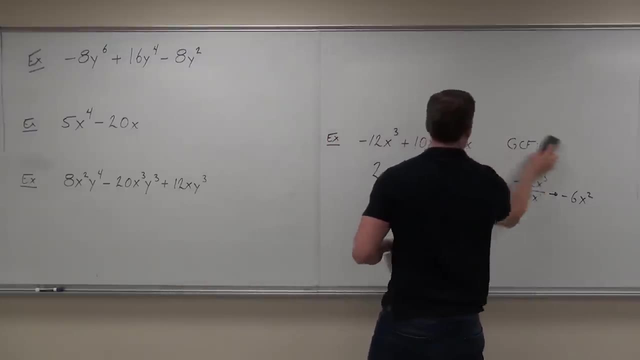 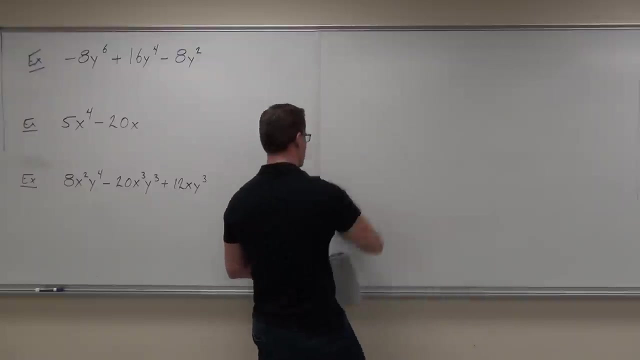 I'll be walking around in just a minute. if you need help on this, now is the time to ask. don't wait until it's too late. Also, keep in mind that if you want to really learn how to do something without relying 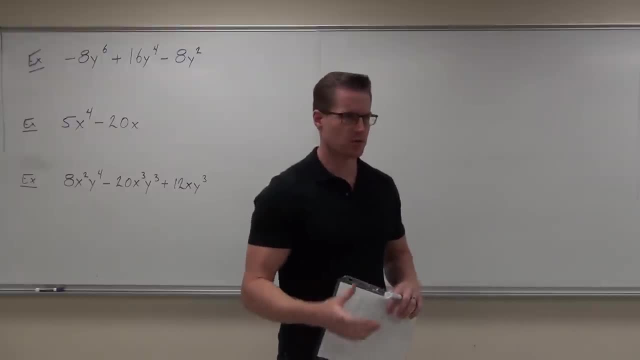 on something else as a crutch, try to do these without using your notes verbatim. okay, Try not to go. what's he doing? okay, now let me follow that step. If you have to at this point, do it okay, because I'd rather you get at least that down. 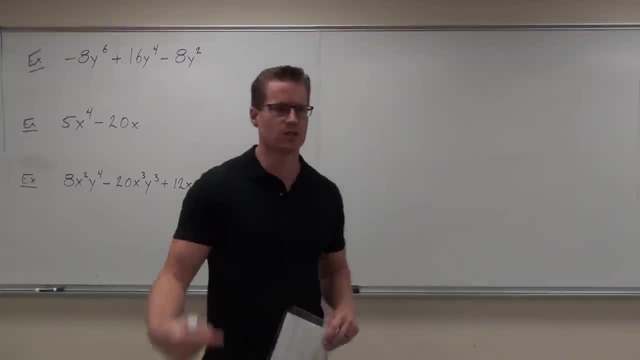 But if you can do it without your notes, that's better. That's what I want you to do. That's what I want you to do as you're doing your homework. Don't just always go back and forth between notes and do an example. that's lame, okay. 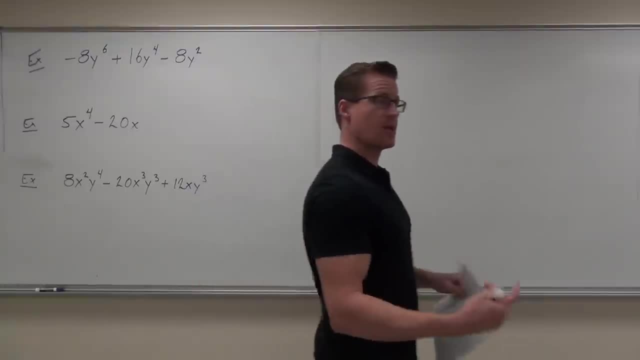 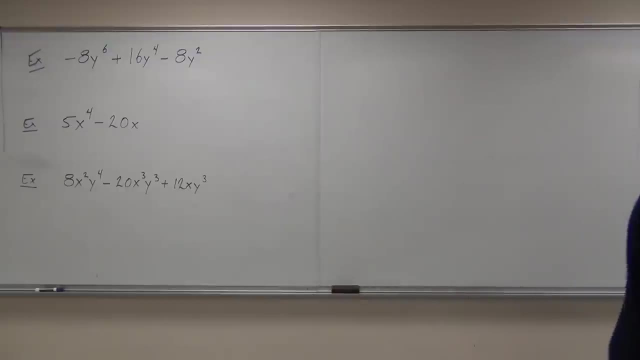 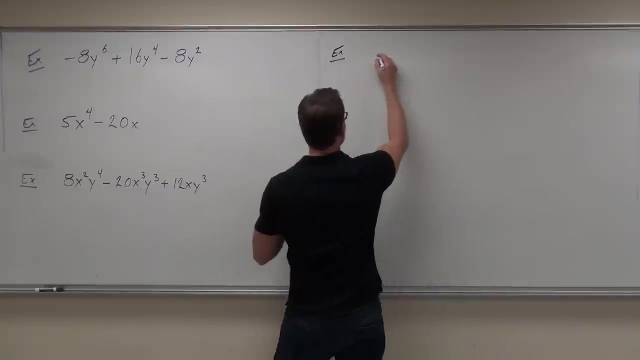 because when you get to a test, it's not going to be embedded in your head. So get to that point where you can do these problems without notes and you are going to be absolutely golden as far as factor and GCF. That's what I want you to do. 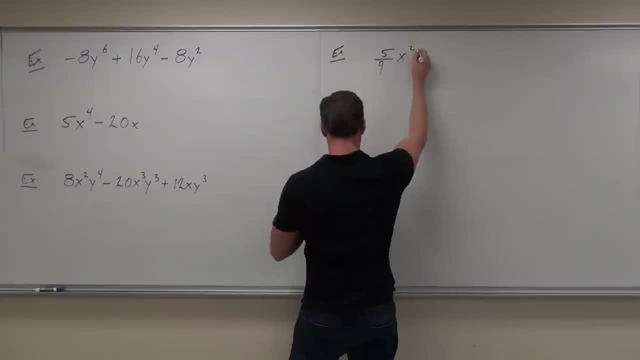 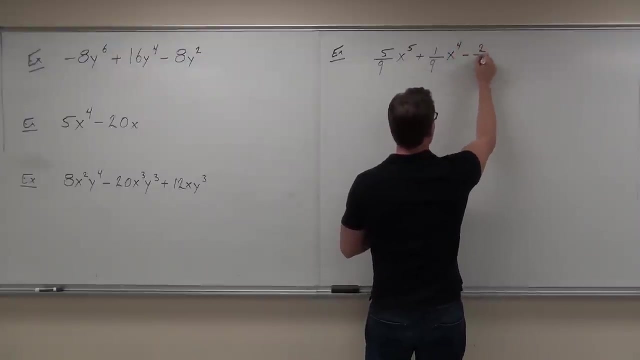 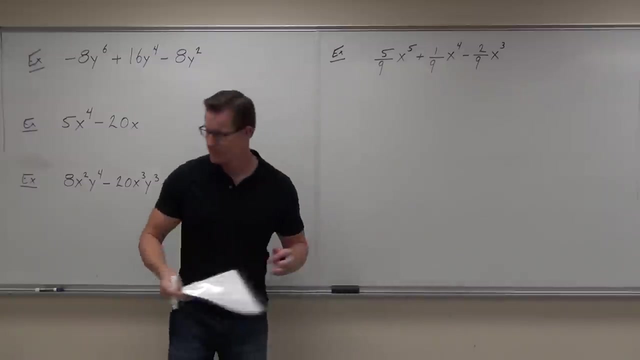 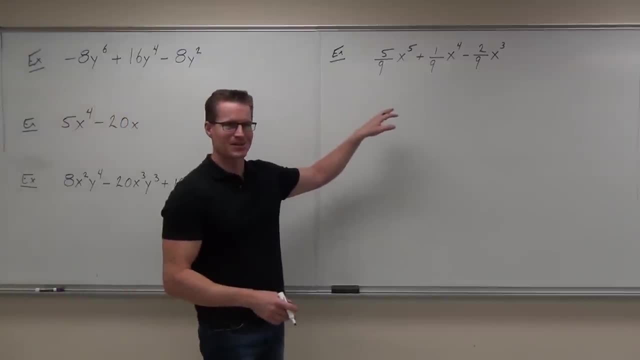 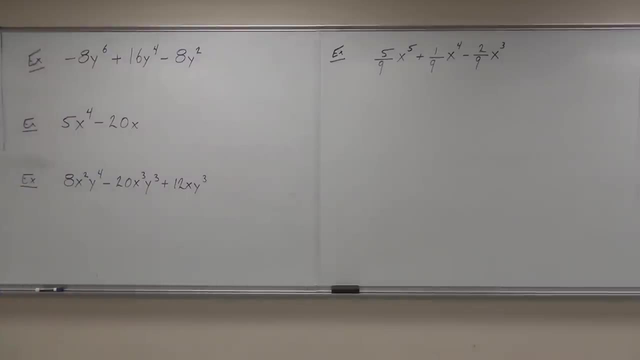 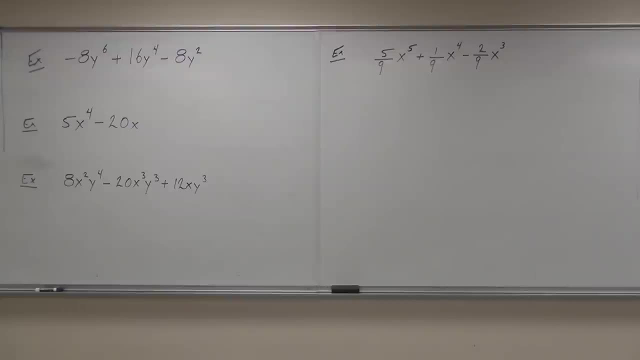 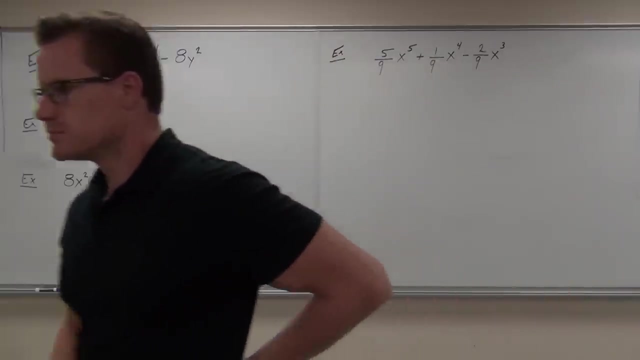 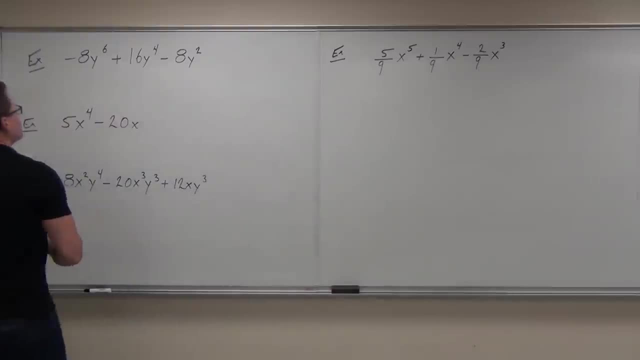 Okay, I'm going to start on the first two up here. So first one: Oh my gosh, Negative 8y to the 6th plus 16y to the 4th minus 8y squared. Can you give me a number which goes into all three of those terms? 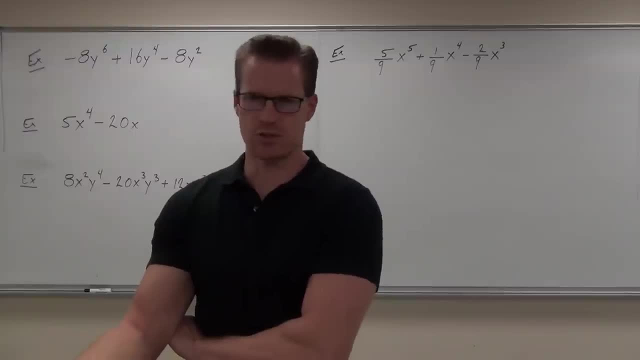 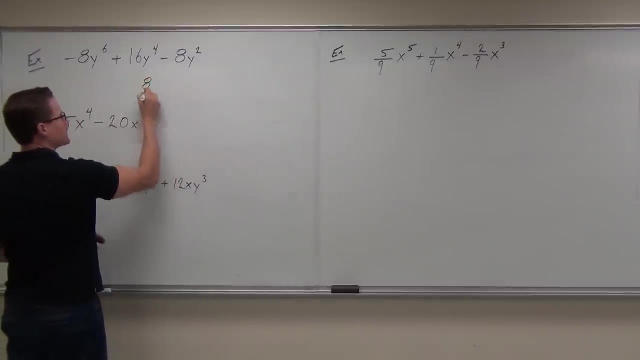 Eight does. Did you all get eight? We don't want to just have two, We don't want four, We want the largest. The grades come in factors, So for us we're going to factor out at least an eight. 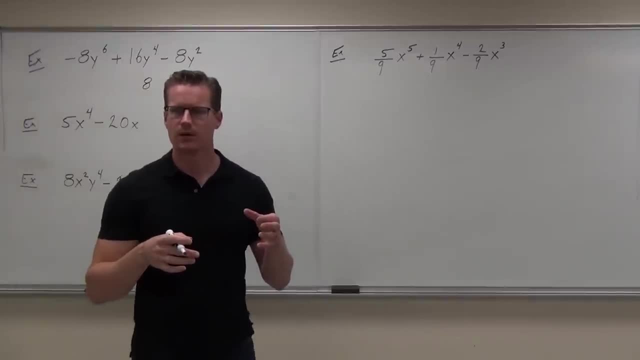 Now how about the variables? Are there any variables which are shared? Y to the 6th: Yeah, don't just get the numbers, We've got to have everything here. So numbers grade 8.. Variables: y to the 6th, y to the 4th, y squared. 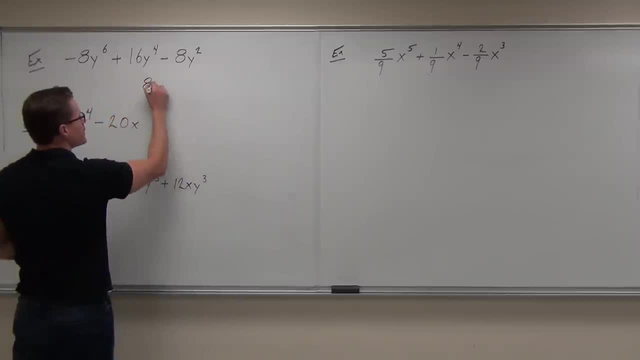 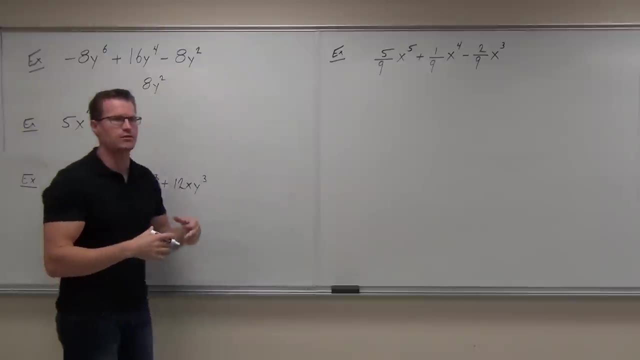 Well, the biggest one, the greatest one that goes into all of them, is y squared. y to the 4th is too much, because this guy doesn't have it. y to the 6th is way too much, because both of these guys don't have it. 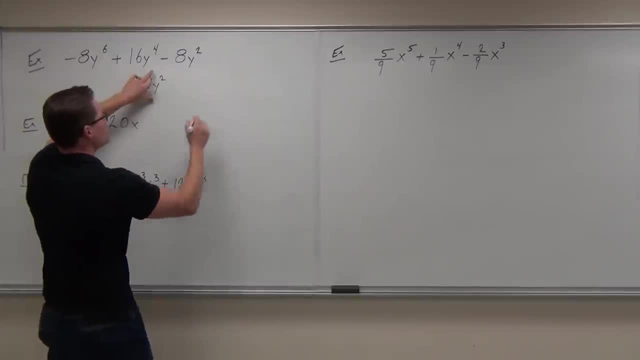 You wouldn't be able to divide by that. If you don't believe me, check this out. If you did 8y to the 6th as your GCF and started trying to divide these things, is that going to work? 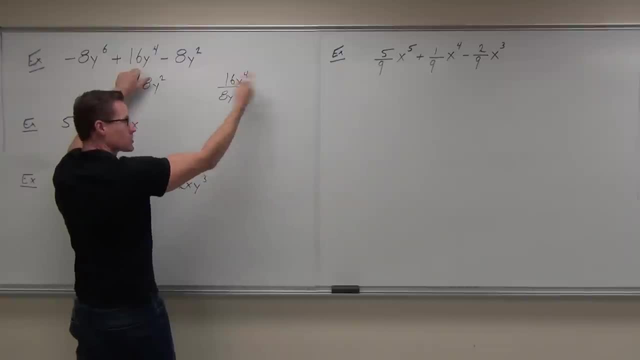 That's too small for that to work. That means that when you start factoring like I showed you those steps before- you come to an impasse, and that's not a good thing. We don't want negative exponents and polynomials right now. 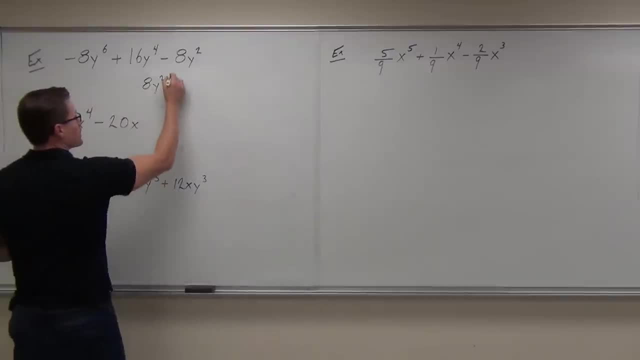 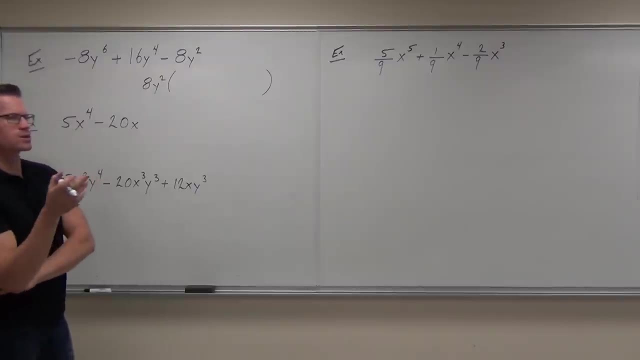 Okay, that's really awkward. So we've got 8y squared and then we have how many terms are going to be inside. You know what? There's one thing I want to talk about right now Is this: in order. 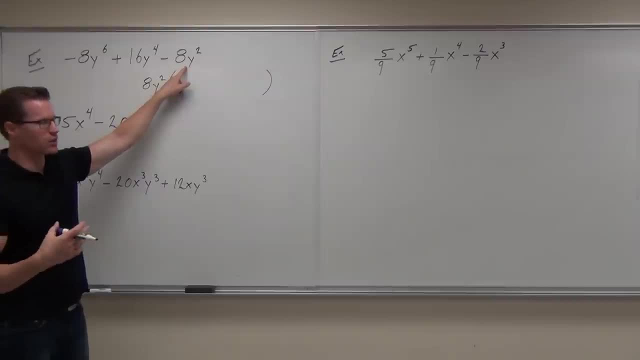 Okay, So might I choose something just a little bit different than them? The 8's perfect, the y squared's perfect, but I might choose something a little different. What might I do instead? Yeah, I might do that. And the reason is: what is the reason again? 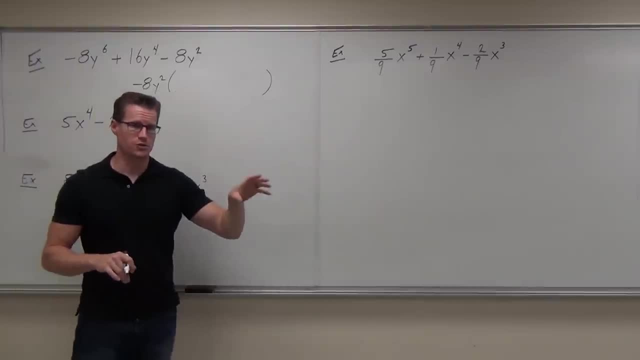 Yeah, if this is positive, that helps us a lot for future factoring and for solving things, And so, typically, is it a must right now? No, The must for you to understand is where in the world that 8 comes from. 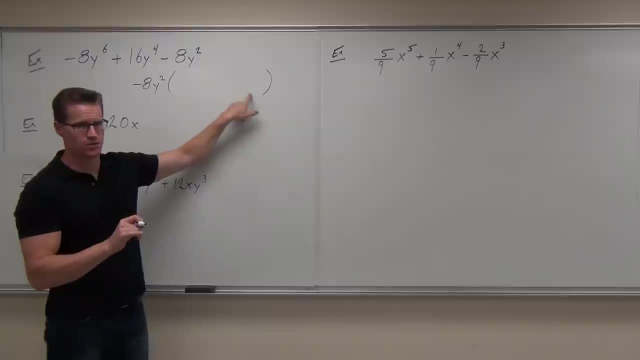 where in the world that y squared comes from and how to use it to get these three terms. That's what you have to understand. In the future, we're going to be doing this because it's going to be really time-saving. It's going to be really useful for us. 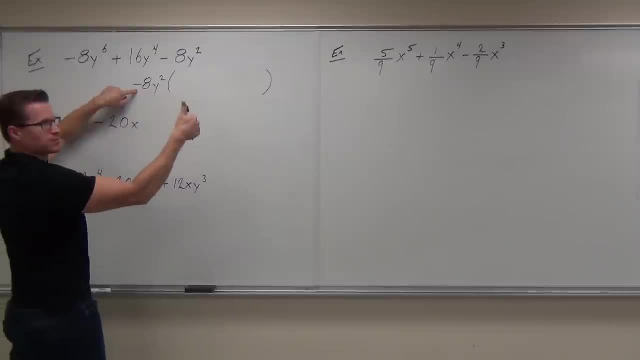 So this is what you have to have. If you get this right now, that's great. If you get that, well, we're going to pick the negative, because I want that- my first term here- to be positive, So we're going to do that one. 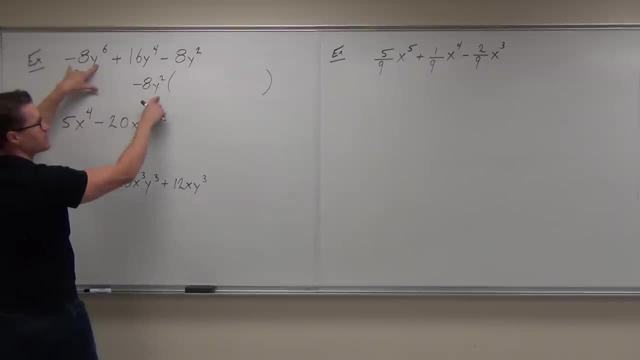 How much is negative? 8y to the 6 divided by negative, 8y squared. Remember, a negative divided by a negative is a 8. divided by 8 is Cool, we can do it that way. How about y? 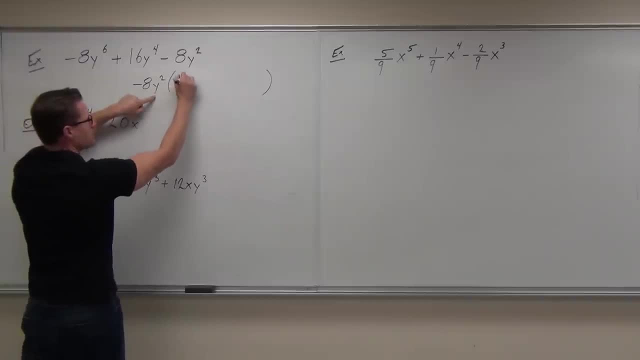 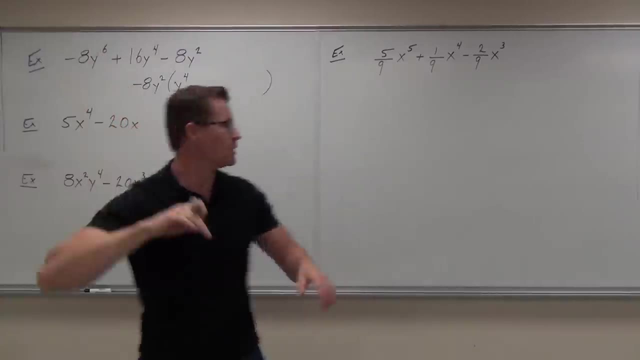 Y to the 6 divided by y squared Y to the 4.. Your first term should be y to the 4.. For how many people is it y to the 4?? Did you get that? Can you double check it? Add these, because we're multiplying common basis. 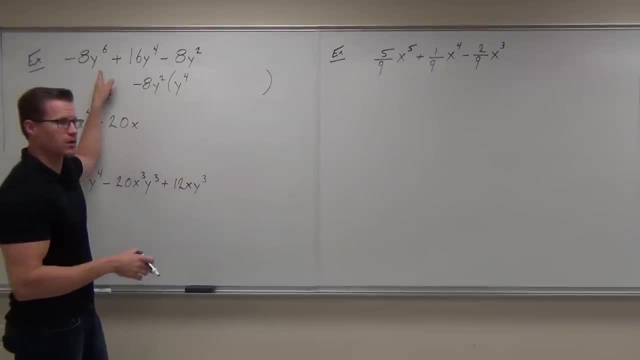 That's y to the 6, negative 8y squared. Hey, yeah, we got exactly the same thing. Next up, should this be a plus or a minus? Minus Why? Because you're pulled out of negative, Positive by negative. 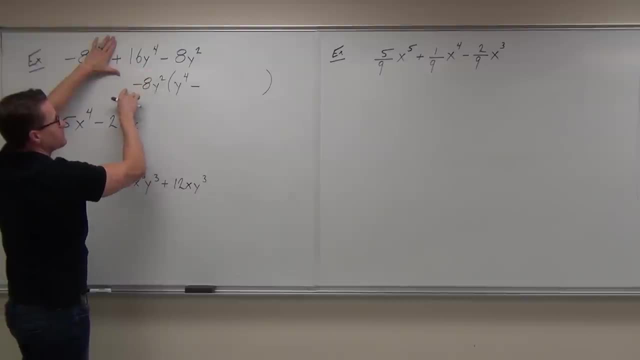 So remember, We divide term by term: 16y to the 4th divided by negative, 8y squared. Positive divided by a negative is a negative. That's why we have the minus. How much is 16 divided by 8?? 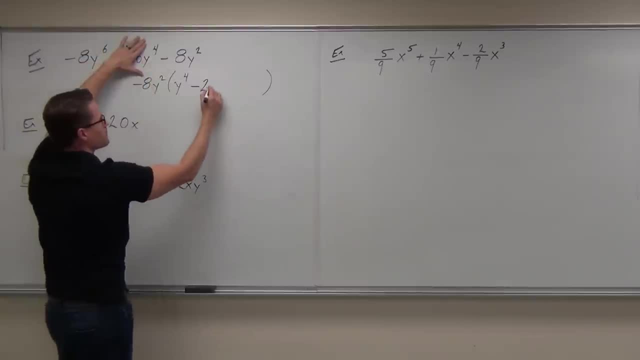 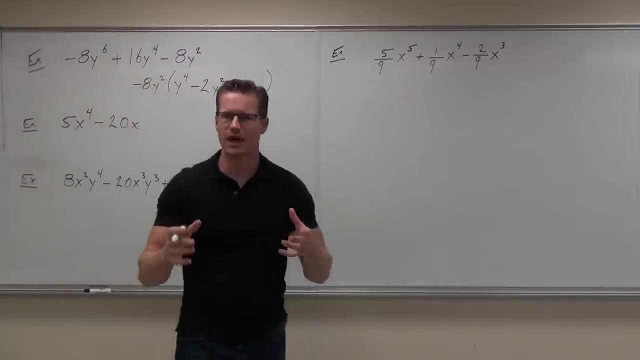 2. How much is y to the 4th divided by y squared? When we divide common basis, we subtract the exponents. If you have trouble doing that in your head, that is not a problem, write it out, Do not just say man, Mr Leonard doesn't in his head. 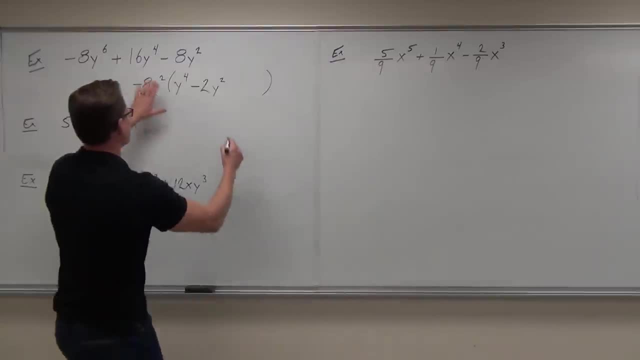 so I have to. That's not true. If you have trouble with this, all you've got to do is just take this 16y to the 4th negative 8y squared and then get your negative 2y squared. 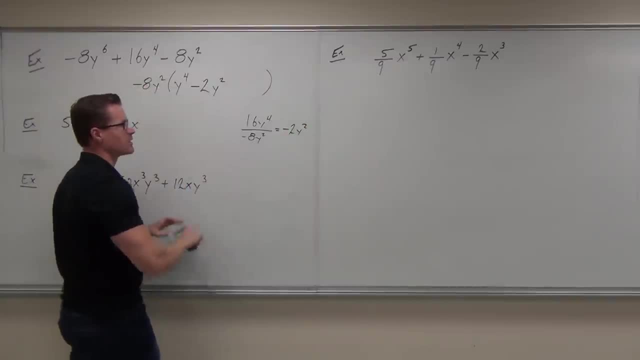 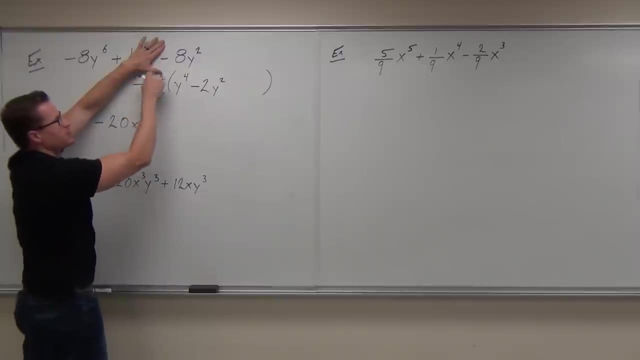 That's where we're getting that Okay. So please do not make the mistake of thinking all this stuff hasn't been in your head. That's not true. Next up, we're going to do negative 8y squared divided by how much is a negative divided by a negative? 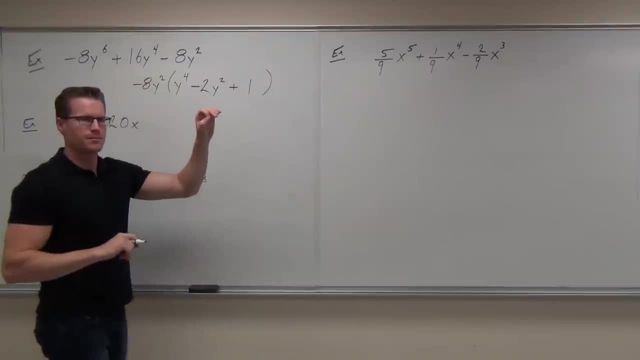 8y squared divided by 8y squared. Are these relatively prime? Yes, They have to, because that's a 1. There's nothing else that's going to go into that, So you're automatically done. You would double check that by distributing. 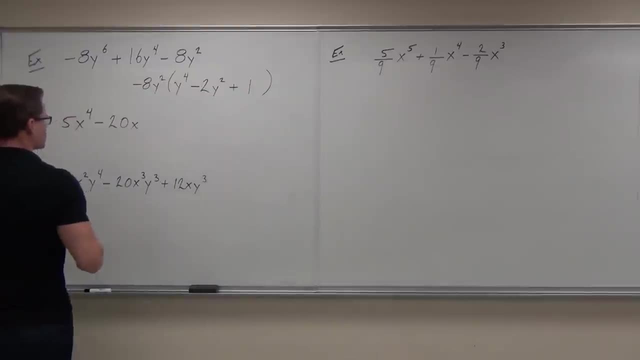 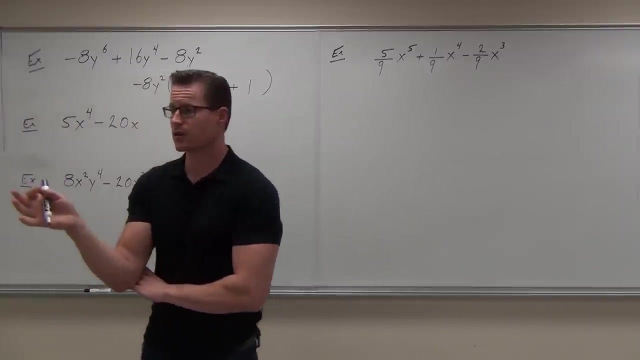 but I'm sure you've already done that. Next one: Oh, let's find our GCF here. We, how many terms do we got Two. What goes in? what number goes into both of those terms? what do you think? 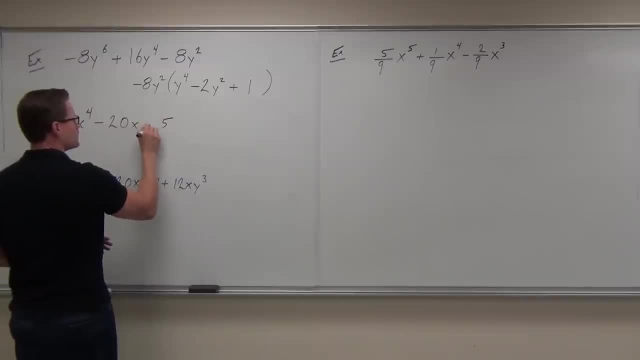 Five. We're going to write the five. Cool. What variable goes into both of those terms? X, That's your GCF. Yes, That means that we're going to create some parentheses because we're factoring. Let's divide. 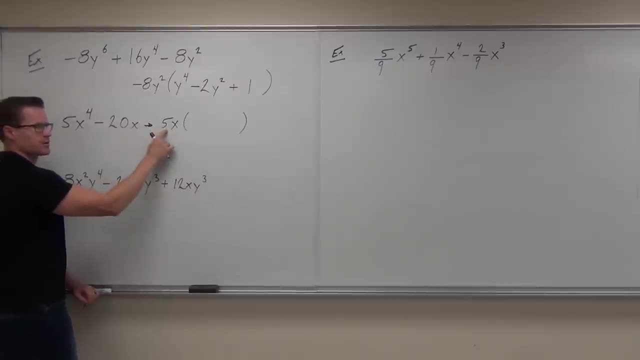 5x to the 4th divided by 5,. how much is 5 divided by 5?? 1. You're going to write the 1? Yes, No, No, It's there. How much is x to the 4th divided by x? 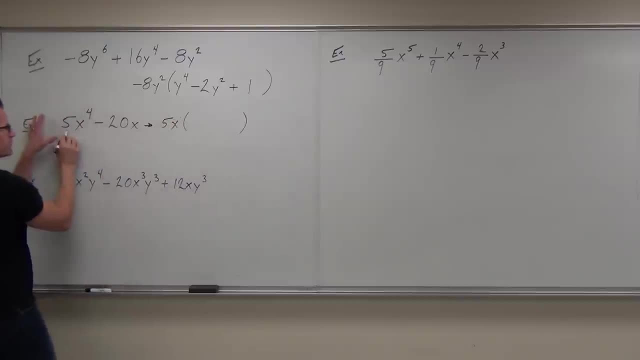 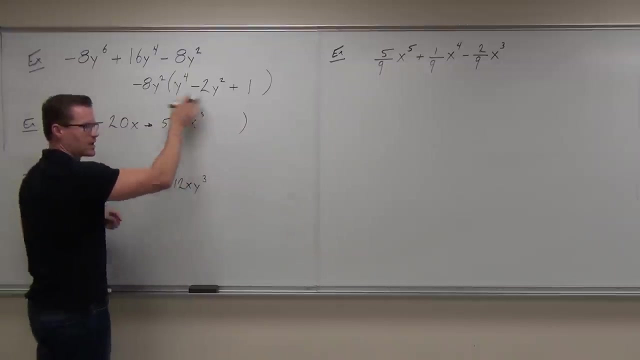 2. Remember this is x to the 1st right. So when I divide by 5x to the 1st, that's 1,, that's x to the 3rd, and that way our exponents are going to add up. if I were to distribute. 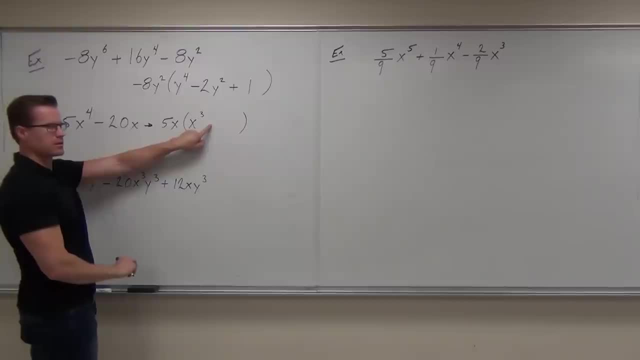 Okay. lastly, am I going to have a plus or a minus here? Minus, Can someone out there explain to me why in this case I factored out the negative, but in this case I didn't? Why? Because if you had created a negative on the first variable, 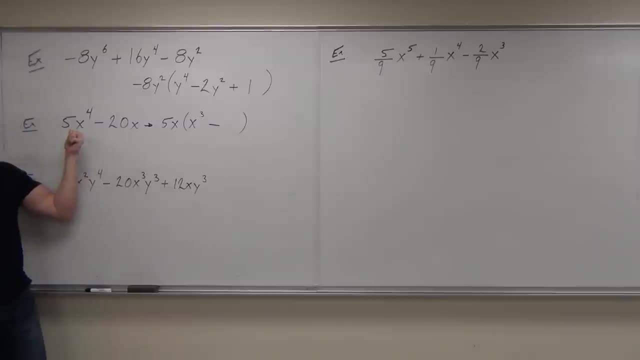 if you factored out a negative, Yeah, that's exactly right. If I were to do that and to make this divided by a negative, my first term would be negative. I don't want that. This is already ordered. That's perfect. 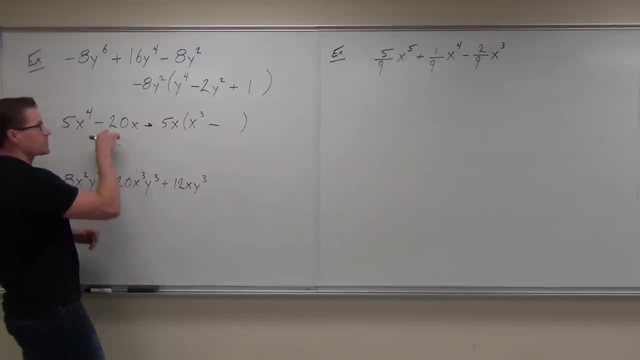 We like that, So factor out a positive. you're good to go Now. 20x divided by- let's do this If you just want to write it right underneath: Second term: divided by GCF. 20 divided by 5.. 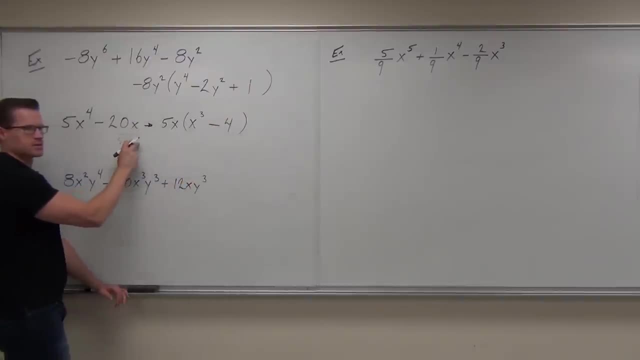 How about x divided by 5?? How about x divided by x? Well, that would be 4 times 1.. 4 times 1 is 4.. We're just going to leave it as that. 4.. Shobhanan, did you get both of those correct? 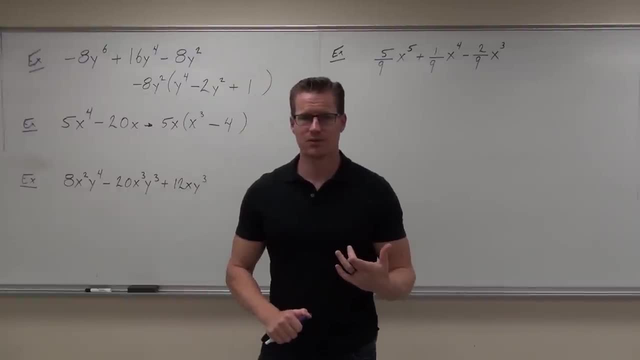 Did you? Are there any questions at all before we do the next one: Did you do the next one? It's a little weird, right? There's so much going on. Is it super hard? No, Not, if you understand the GCF. 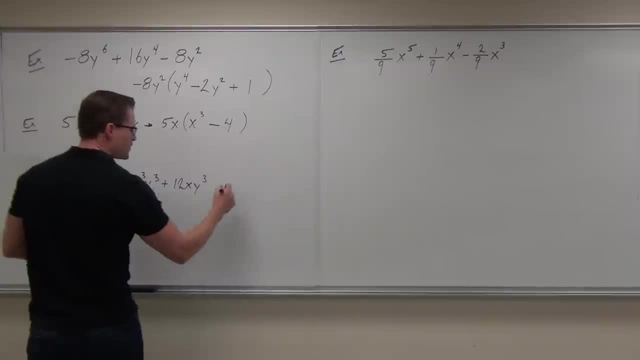 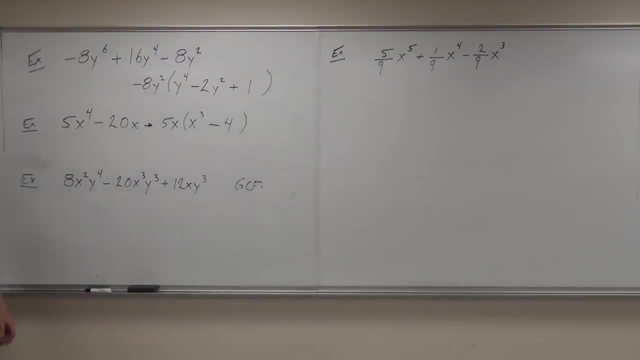 It's all the same, You just got to be careful. So let's look at the GCF. I'm going to write this one out, That way we don't lose it. Man, this is a little bit more complicated. So first thing, let's look for what do we do first? 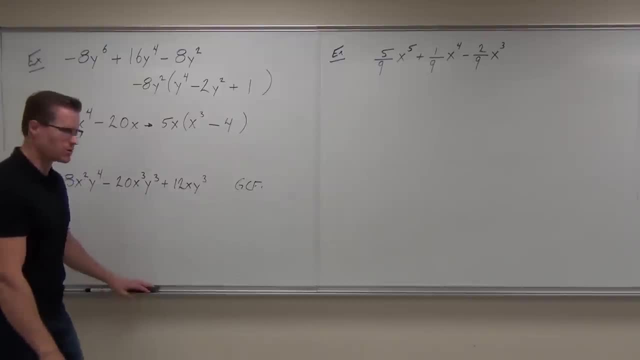 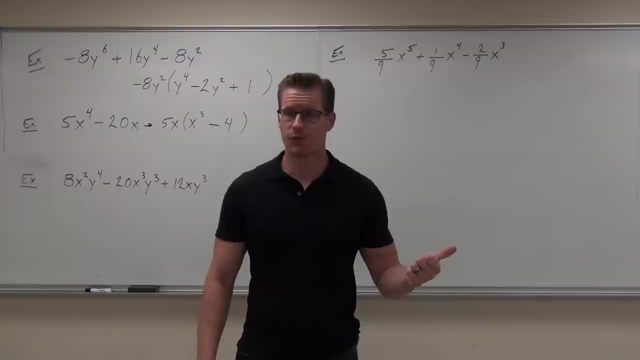 GCF- I know it's GCF, Numbers, Numbers. We've got 8, we've got 20, we've got 12.. GCF: true, false is 2? No 4.. True, Okay, 8?. 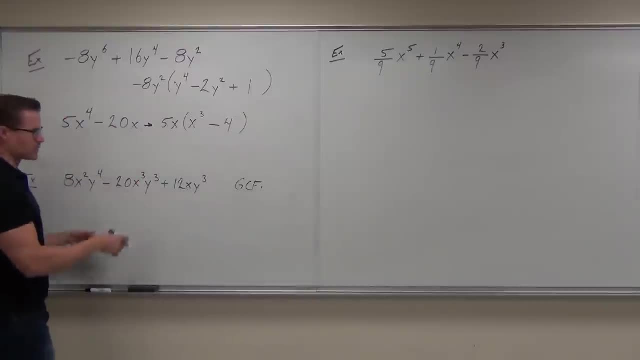 No, Why not 8?? Either 1 going or 12. Or 20. But yeah for sure. So 4 is going to be our GCF as far as the numbers are concerned. Now do we have to do all the variables at once? 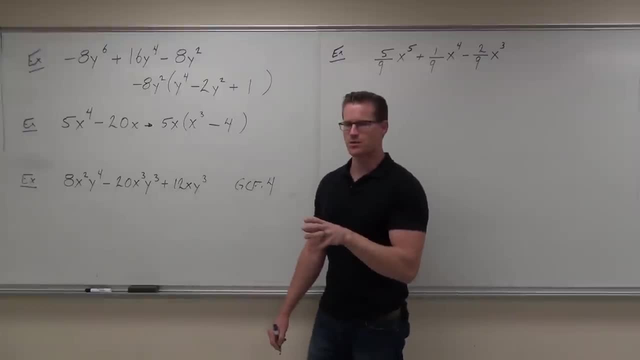 No, You can if you're really good at it. That's cool. Let's do the x's first. So I have x squared. I get x to the 3rd. I get x. What's my GCF for my x's? 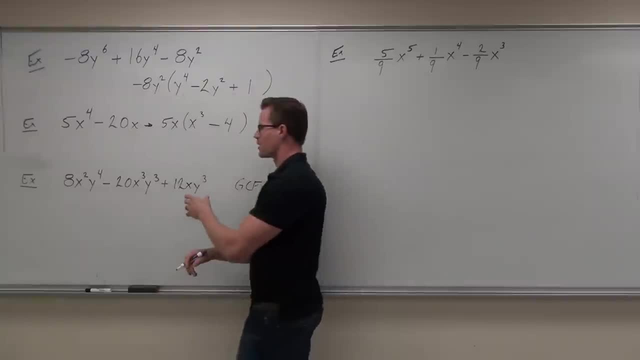 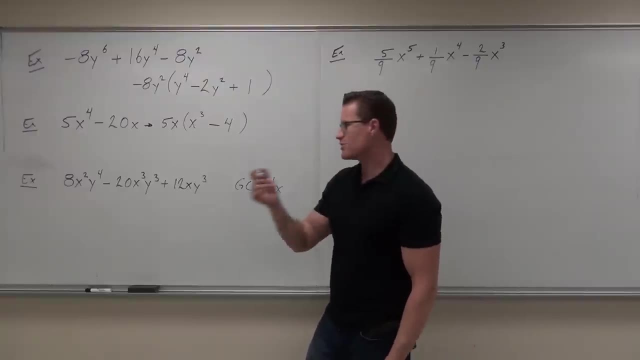 X, X. That's the largest power of x that all three of these terms have in common. How about the y's? What are the y's? Y to the 3rd, Yeah, I can't use 1 to the 4th. 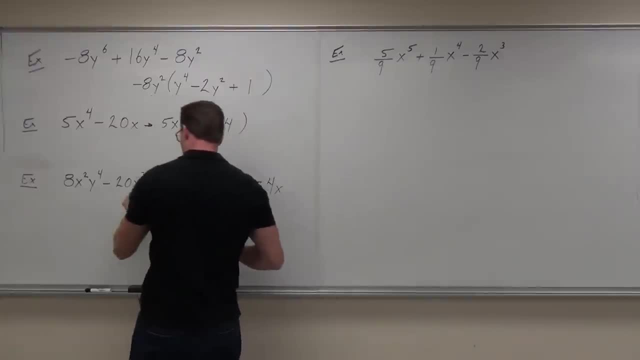 These guys don't have enough to go to lunch. So y to the 3rd: that works here. That works here. That works there. Were you able to find your GCF of 4xy to the 3rd. All I'm going to do is divide it. 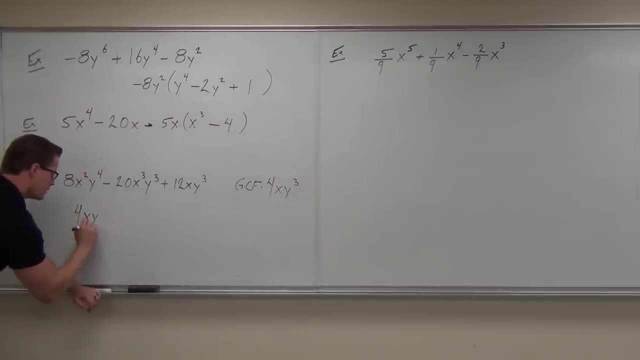 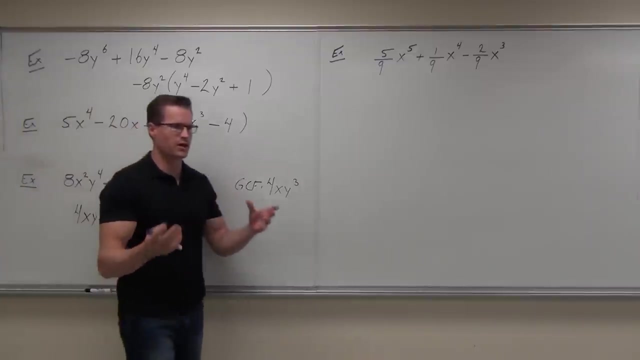 So our GCF goes in front. We create some parentheses, We have 1,, 2, 3 terms. We're going to end up with 1,, 2, 3 terms. Right now it's this type of a problem because we have all these variables flying around. 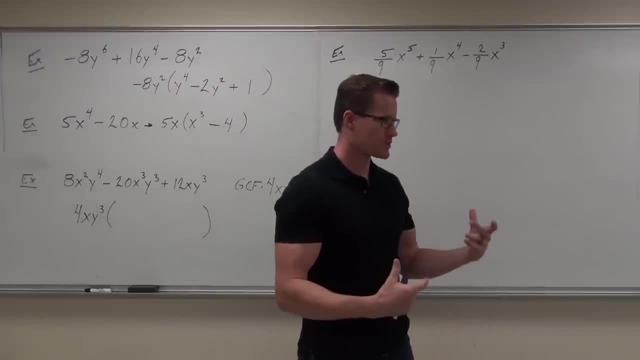 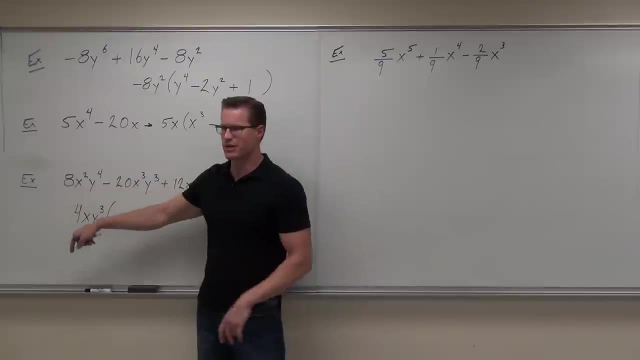 We really don't need it specifically in order as far as x numbers go, because it's not a right now, it's not that type of polynomial that we do that with. So if this is the case, if the first term is positive, just factor out a positive. 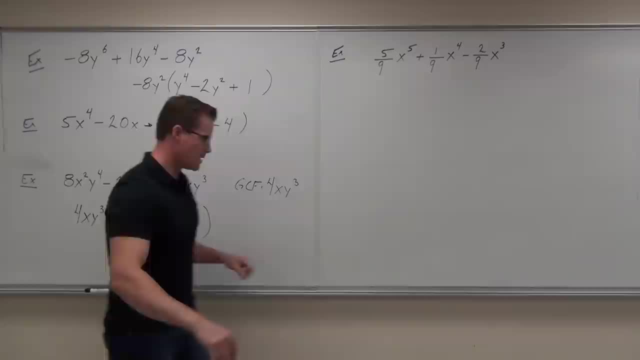 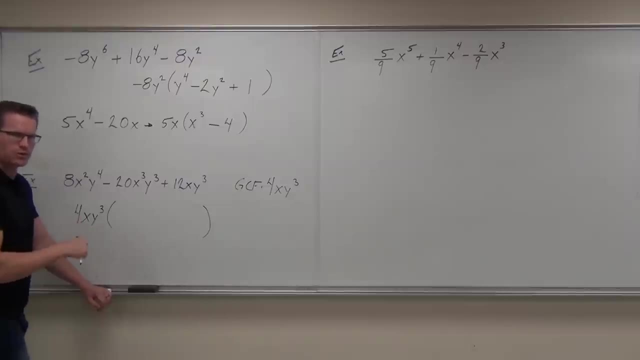 That's basically the idea. You guys with me on that one. So we're going to go ahead and do that. What might be a good idea here Should, if you struggle with this, would you try to do this in your head if you struggle with it? 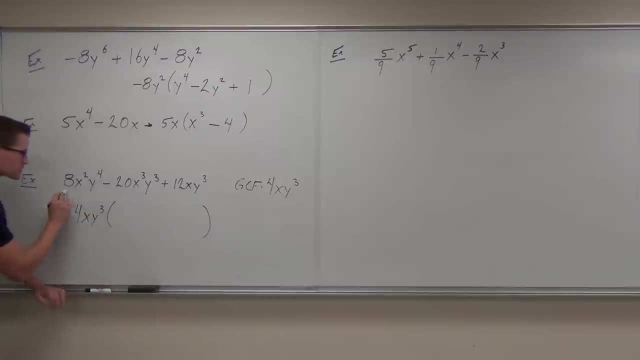 No, No, You'd probably write it out, okay, Or you can even do this: Do the 4xy to the 3rd. If that helps, you can put it in all three spots. That's cool too. How much is 8 divided by 4?? 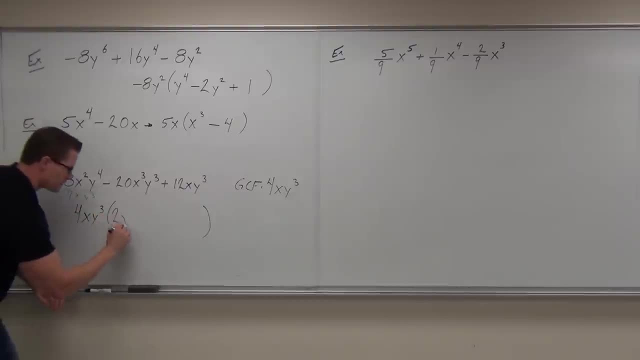 2. 2. How much is x squared divided by x, x, x. How much is y to the 4th divided by y to the 3rd? 1. 1. Cool, We subtract exponents every single time when we're dividing by common basis. 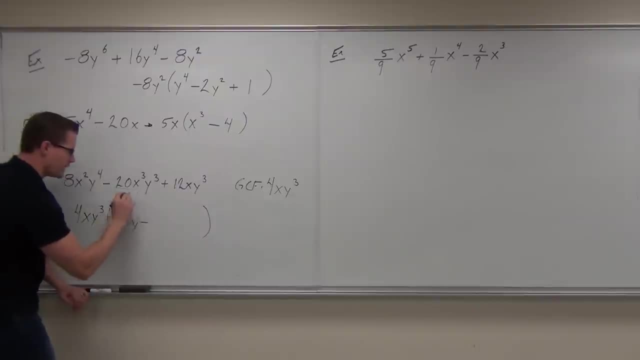 Next up plus or minus Minus. Remember that we're dividing by always the same GCF. You cannot change that. 20 divided by 4? 5.. x to the 3rd divided by x: x to the 3rd. 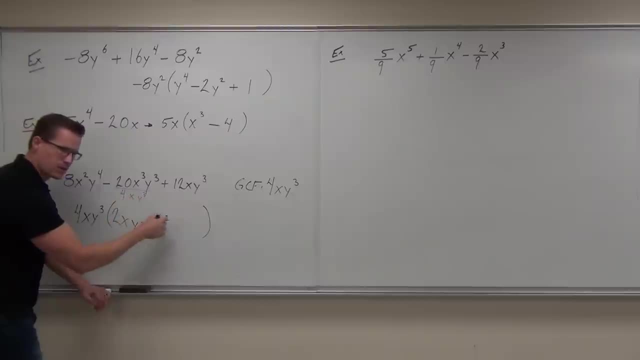 And lastly, y to the 3rd divided by y to the 3rd: 1.. 1. Do I have to write anything here? No, No, Okay, cool, Now we're going to go ahead and do that. 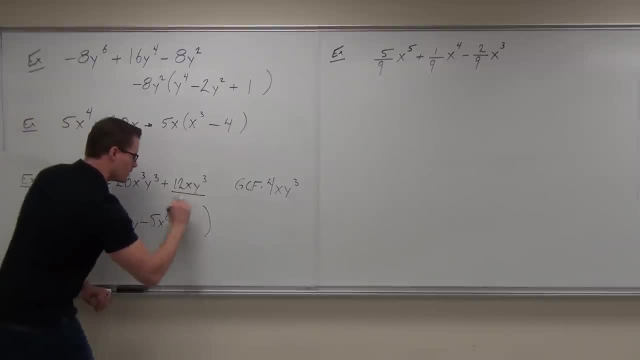 Okay, Now I'm stuck 4 x, y to the 3rd, 12 divided by 4? 3.. So I'm going to have that plus 3.. Well, the rest of it's kind of nice. 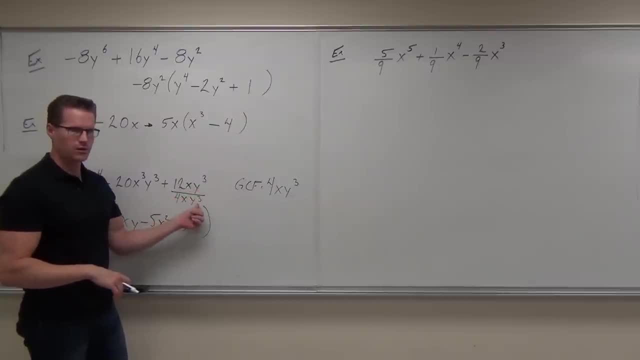 x divided by x: 1. y to the 3rd. divided by what? to the 3rd? 1. Cool, We just have that 3, and you can certainly double check that by distribution. What I want to know is how to explain up to this point, how to use the GCF for factoring. 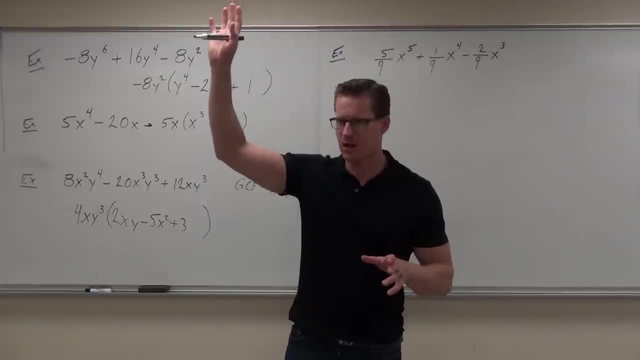 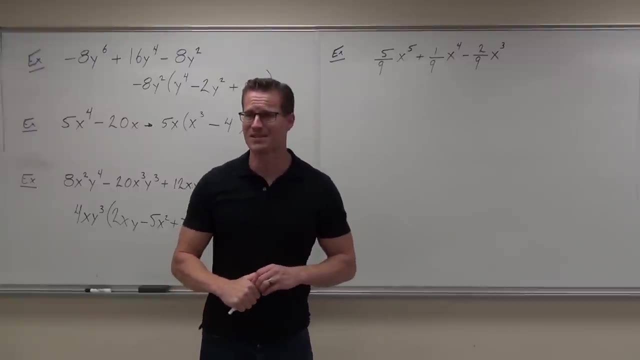 well enough for you. Raise your hand if I have it. Feel okay about it, Okay, Okay Now y'all love fractions, right? Oh, fractions are horrible because they make things more difficult. So one thing that happens is when you're factoring a lot of times. 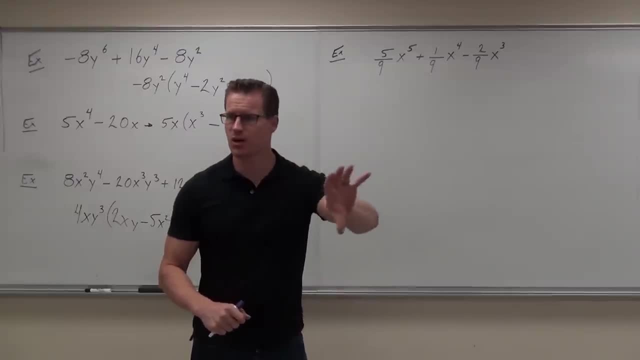 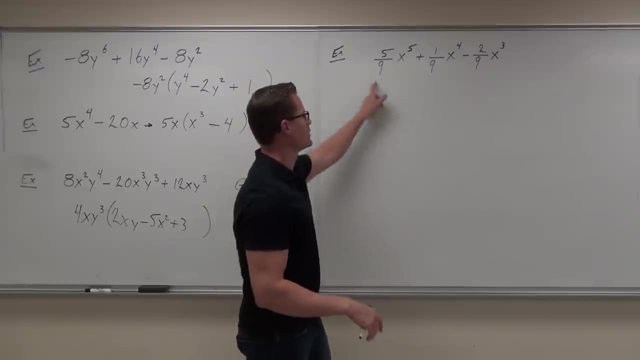 it's really nice to factor out the fractions because that makes the rest of your problem, inside your parentheses, easier. So when I've given you a really easy example to illustrate this, It is harder if these are different numbers because you have 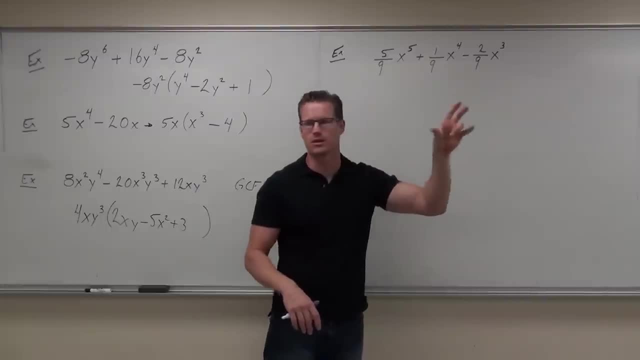 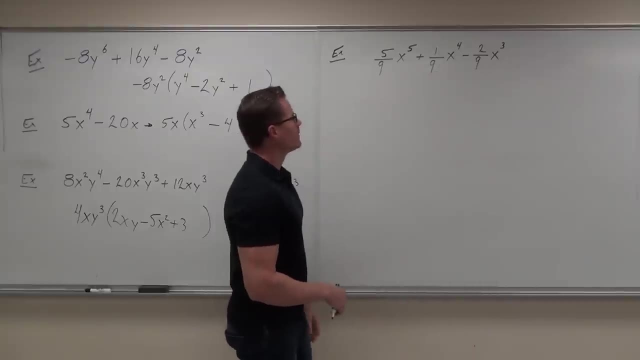 to factor basically a little bit differently and I'll show you one of those a little bit later. but for right now, if you have the same denominator, like in this case 9,, look up here. Are there any numbers which go into 5, and 1, and 2?? 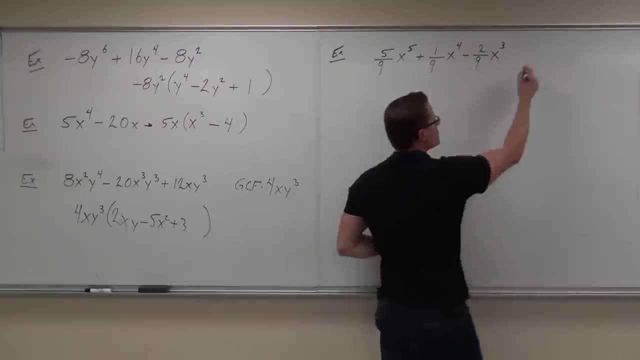 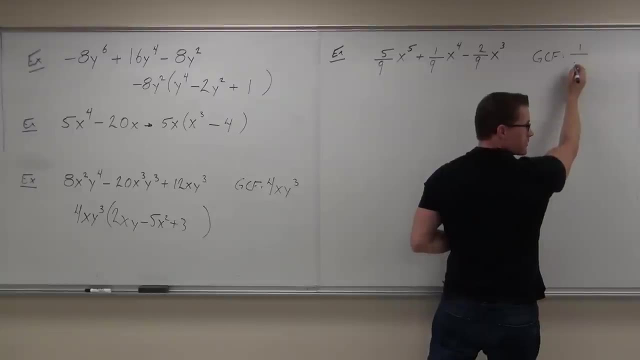 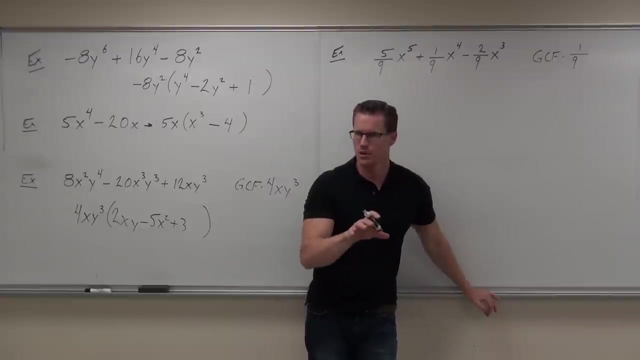 1. Besides 1. So our GCF- here you said 1, right, 1 goes in all three. 1. Factor out that common denominator. Do that, It'll make the inside of your Parentheses much, much nicer looking. 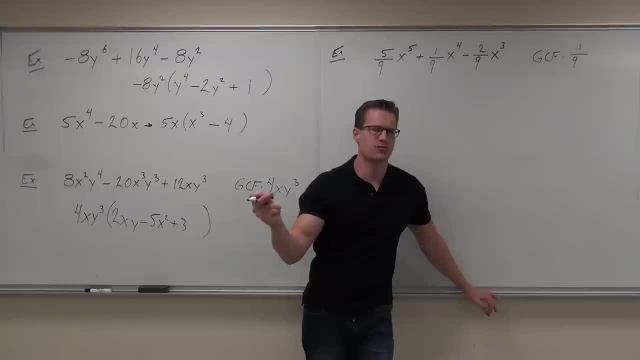 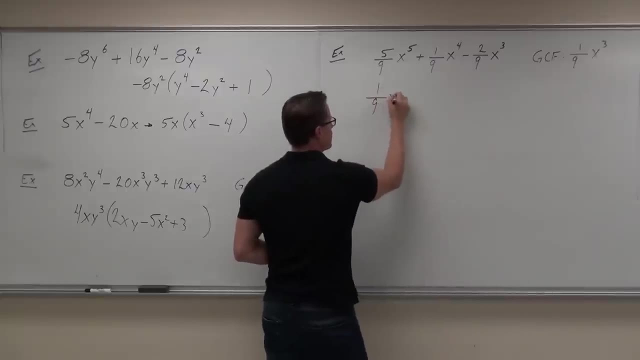 Now the variable should be easy for us, Real quick. what's the GCF for variables If we factor that the 1, 9th, X to the 3rd? I'm going to do it really fast for you guys. 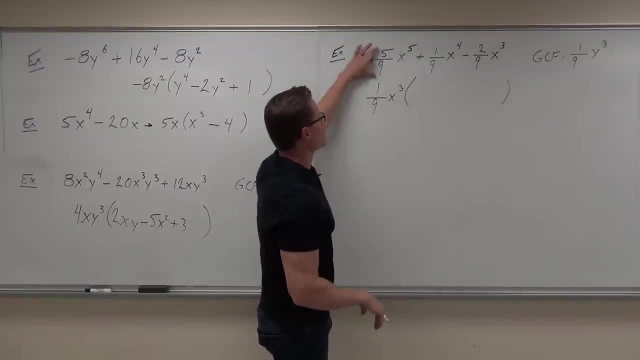 because I believe that you have this kind of down. If I factor out the 1 9th, yeah, you could do 5 9ths divided by 1 9th. It looks kind of awful to be honest with you, but remember. 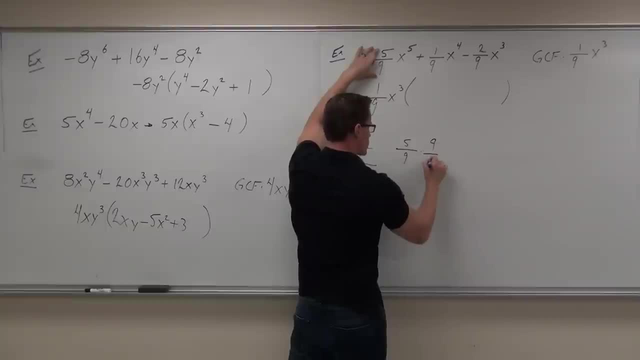 that all that's really good is that you can do that. So what's really going to happen in this case is you're going to be multiplied by the reciprocal of that fraction. Your 9s are going to be gone. So when you factor out the 1 9th, it's really the 9 that's disappearing. 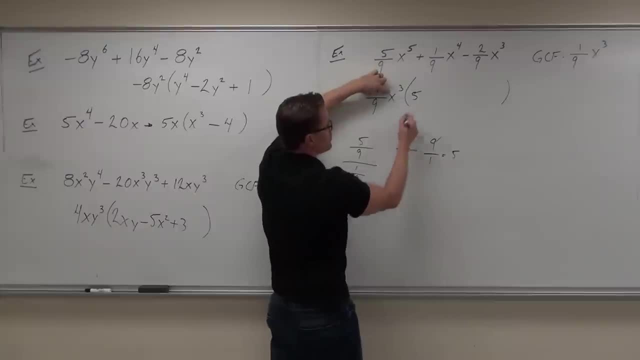 You're going to have the 5: X to the 5th over X to the 3rd. Remember you subtract when you divide common basis, That's X squared. We're not taking any signs away. We're going to have the same signs. 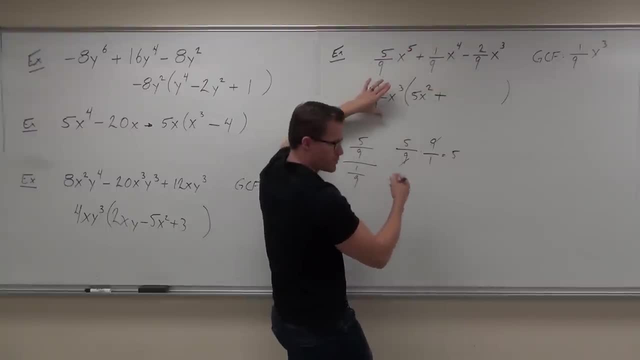 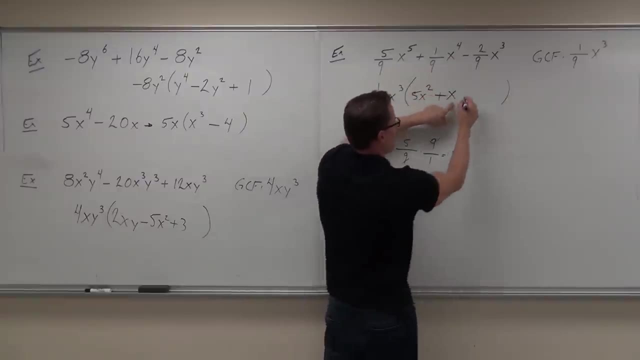 1- 9th. when I factor out 1 9th, well that's 1. We'd have X, because X to the 4th over X to the 3rd gives us. And lastly, that's a minus. 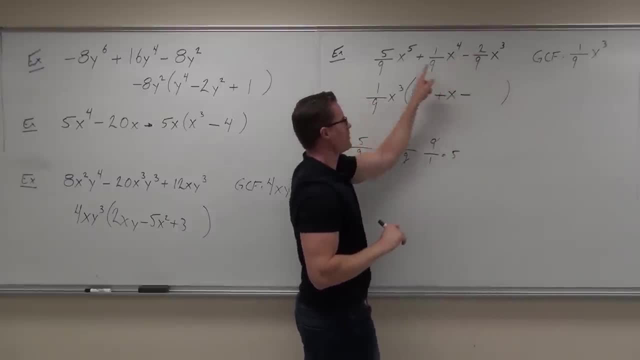 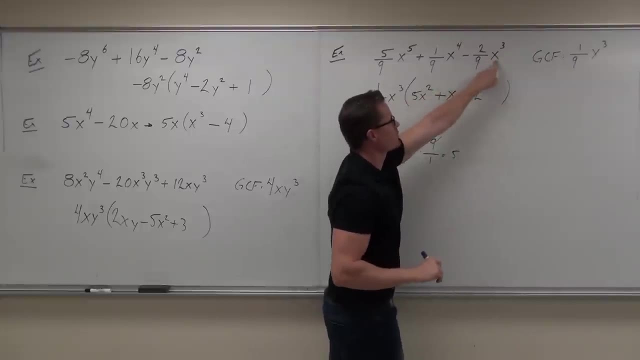 This is a minus 2 9ths divided by 1 9th. All it's going to do is remove the 9th part of that. We're going to have 2.. And then we have X to the 3rd divided by X to the 3rd. 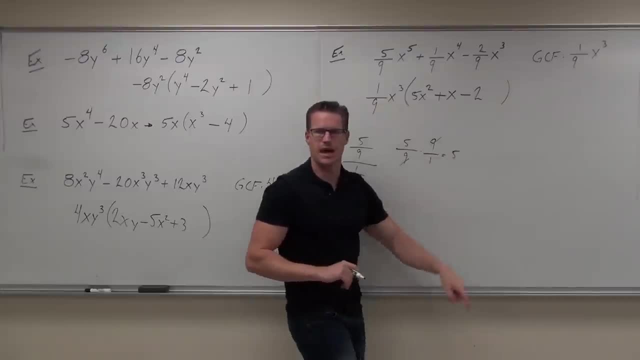 That's going to be. oh man, I lost half of you, didn't I, Goodness gracious? X to the 3rd divided by X to the 3rd is 1.. It's 1.. Hopefully that's real. 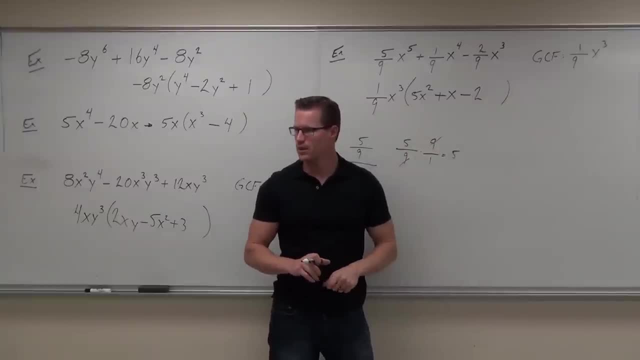 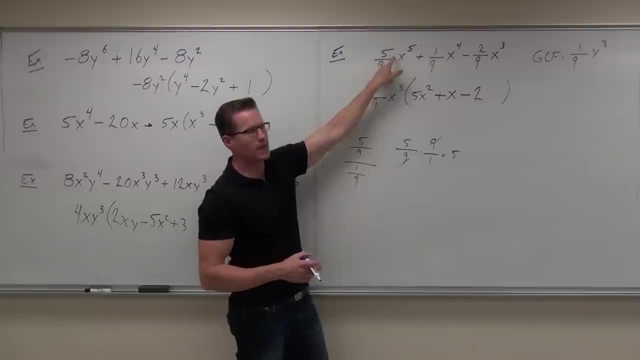 1.. 1 times 2, we got 2.. Are we okay with those ones, The 2?? If I'm basically what I'm doing, I'm removing the 1- 9th from each, I'm getting rid of the fraction. 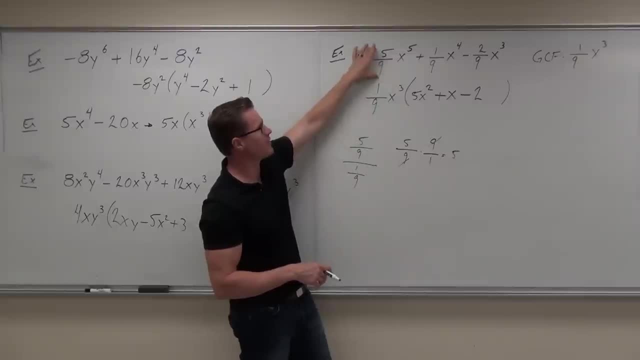 So if I remove the 1- 9th, take away this idea of having the fraction 1- 9th, I get 5.. Take away the idea of having the fraction 1- 9th and dividing that out, I get 1.. 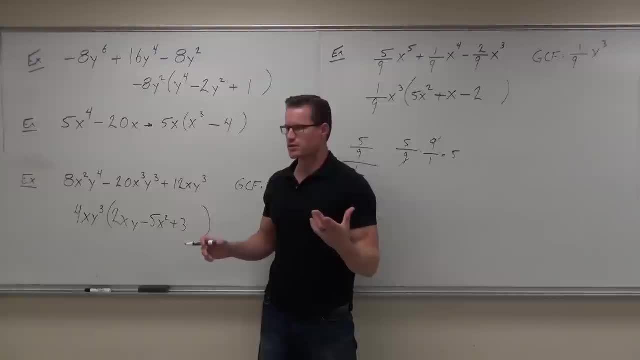 Take away the 1- 9th, I get 2.. Basically, just the numerators, That's all we have. 5, 1, 2.. Hey, 5, 1, 2.. That's the idea. 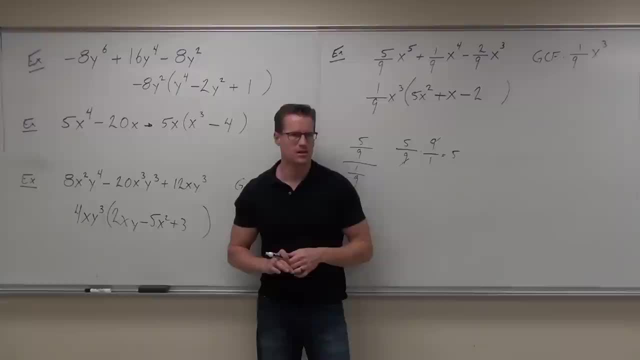 Does that make sense to you? I know it's a quick one, Quick little trick, but it's kind of nice Question. Couldn't you also multiply H1 by 9, and then it would cancel out the bottom denominator here? No, you can't. 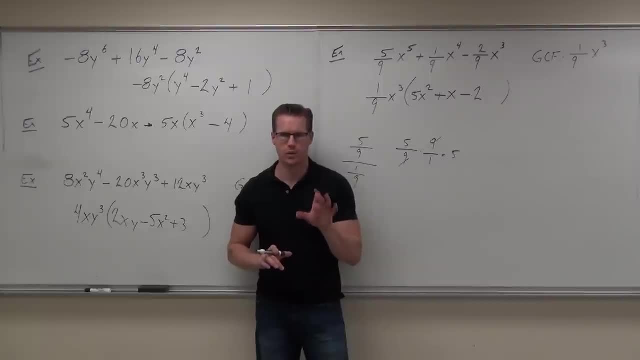 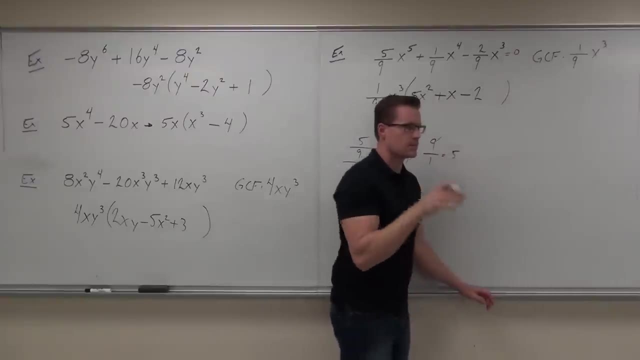 The only time you can ever, ever, ever multiply by a number that's not 1 is if you have an equation. If this were equal to 0, if it's an equation, you can do almost anything you want to, As long as you do it to. 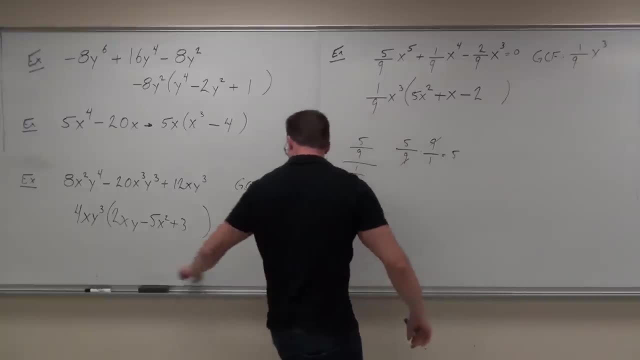 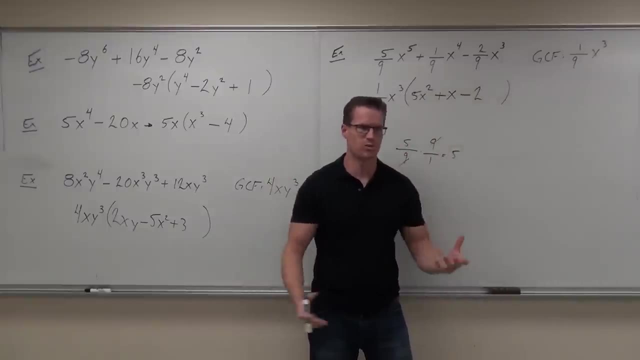 Both sides, Both sides. Oh wait a minute. If I don't, If I don't have an equation, I don't have the idea of both sides. Does that make sense? Which means you can't just multiply whatever you want to. 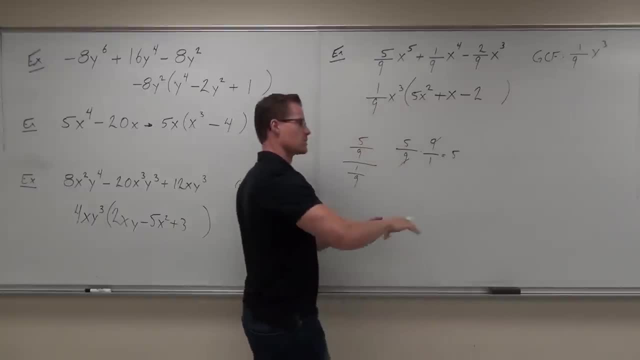 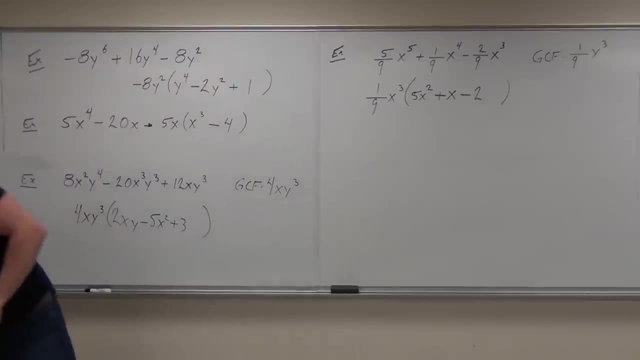 It would be awesome, But you can't do that. It's a good question, You're on the right track, but you're a little bit thinking of equations rather than expressions. Thanks for bringing that up, though Can we move on a little bit? 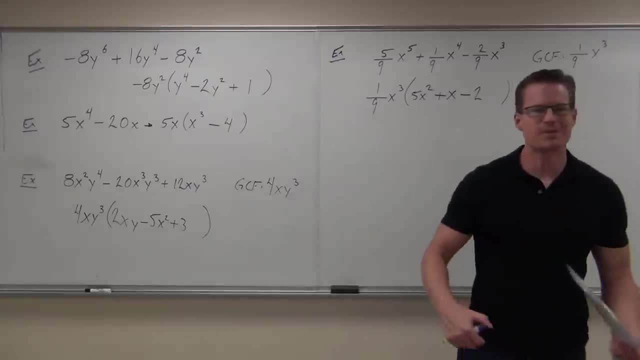 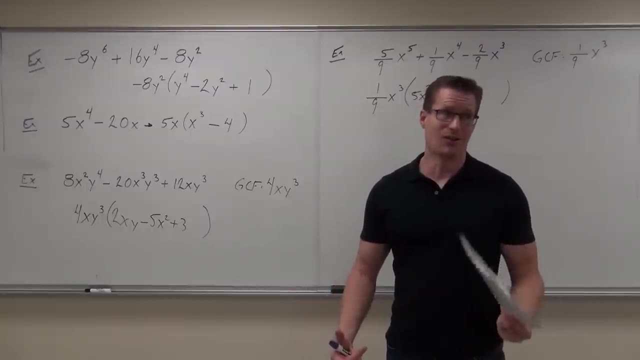 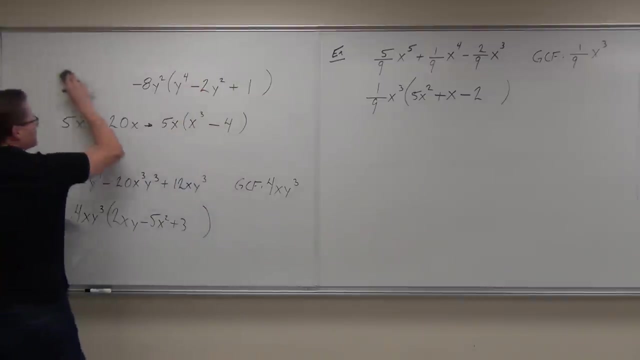 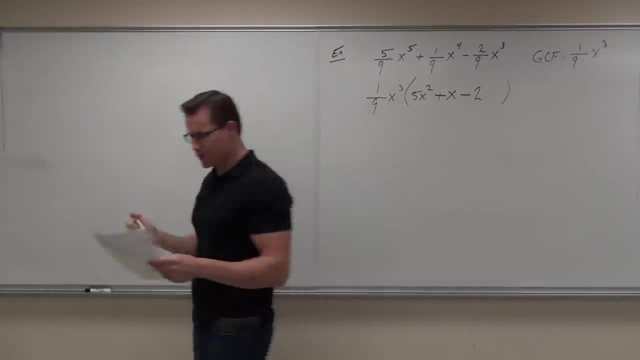 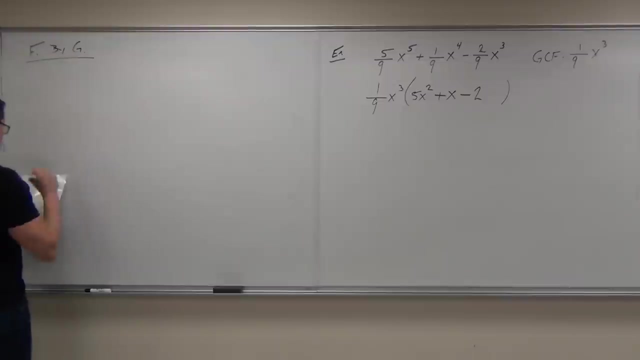 So I'm going to introduce vector by grouping with this one example. If you had this so factoring by grouping, Let me pretend for a second that I couldn't combine those. I know right now that 8x plus 7x is 15x. 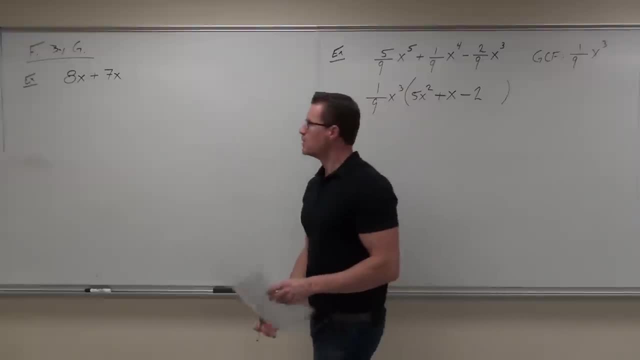 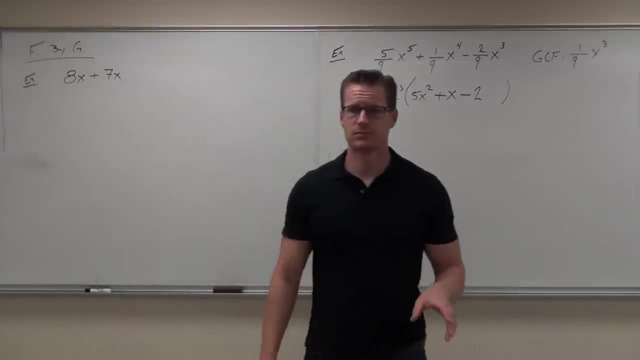 We know that, yes, Not 15x squared or something silly like that, but 15x. Now let's say that what I want to do instead of combine these was: I wanted to factor it. Could I factor it? Let's try this again. 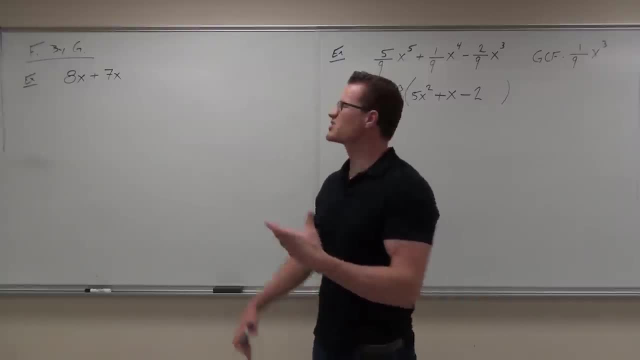 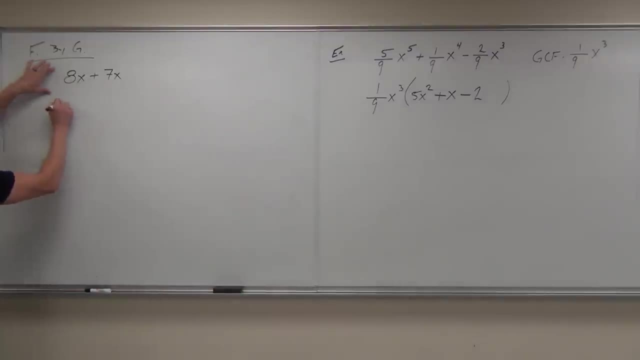 Could I factor it? Are you with me? Yeah, What goes into? but what's the GCF of 8x and 7x? So if I were to, If I were to factor this, I'd write the x here, correct. 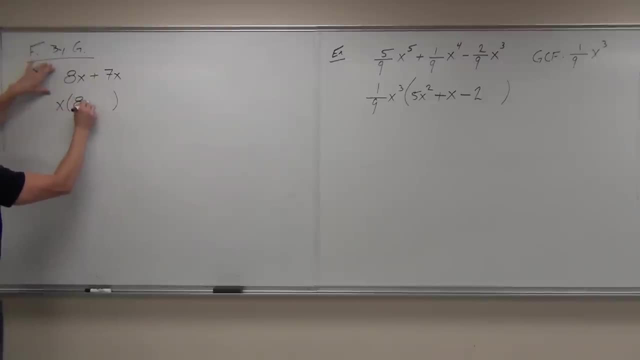 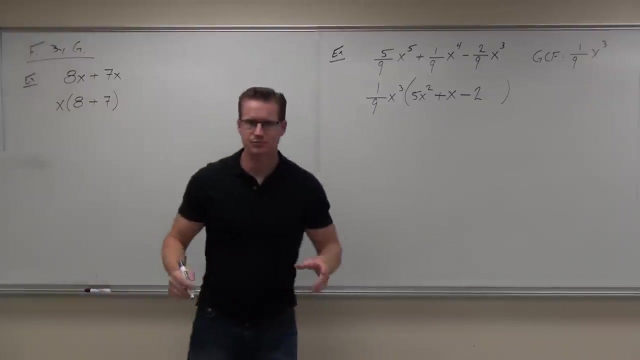 And then, inside parentheses, I would have 8 plus 7.. You all still with me? Now let me show you something about this. How many x's do you have here? How many x's do you have here? Why did these two x's become one x? 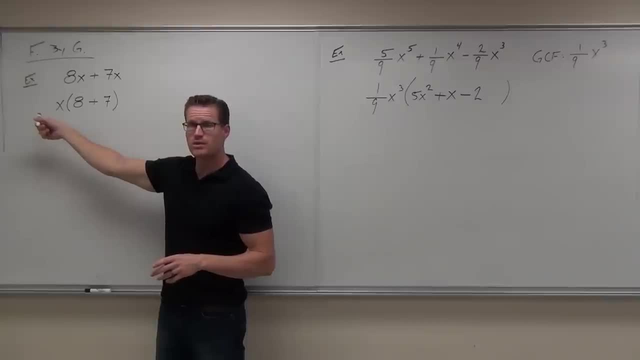 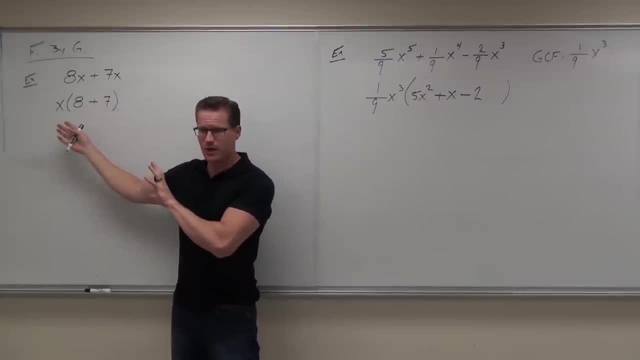 Creating these two x's again. This idea right here, if you understand that factor by grouping is easy, I swear easy. okay, What happens is you have two x's here, you have one x here because we're factoring and dividing both those terms. 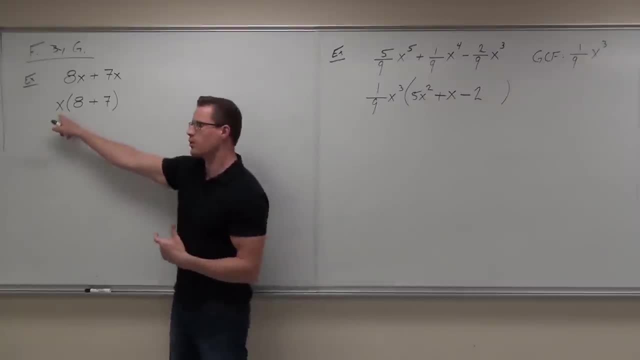 by that one single factor. It makes it look like there's only one x. But if you were to distribute it it would go to both those terms, giving us back those two x's. Quick head nod if you're okay with the idea. 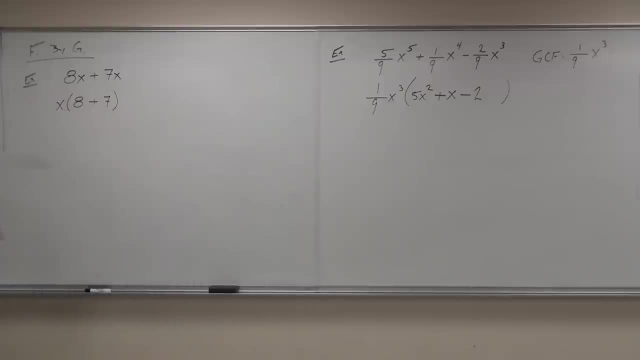 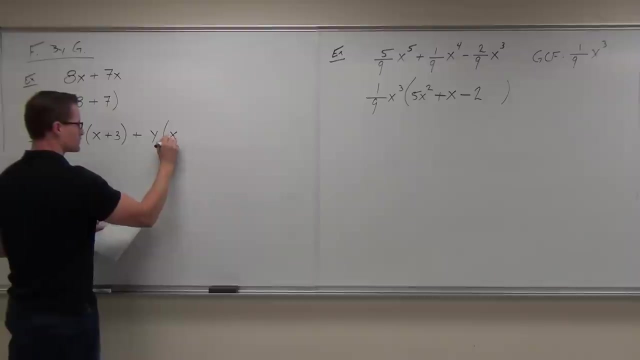 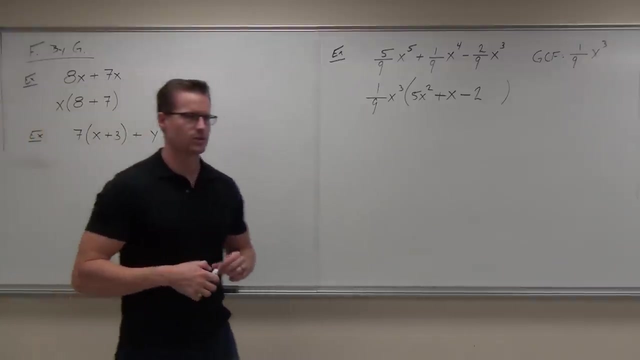 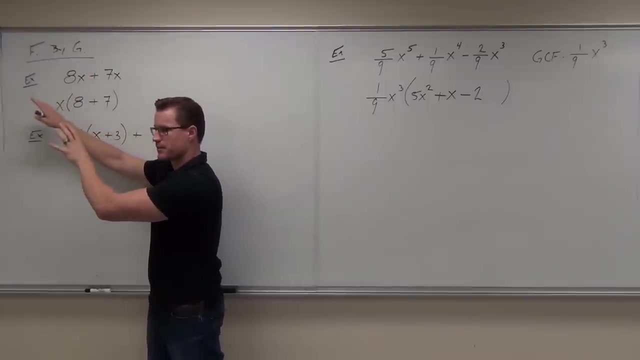 All right, That's how factor grouping, factor by grouping, works. So let me show you. So let me take this and run with it a little bit. So again, these two x's become one x, because when we factor from both terms to undo that we would distribute to both terms. 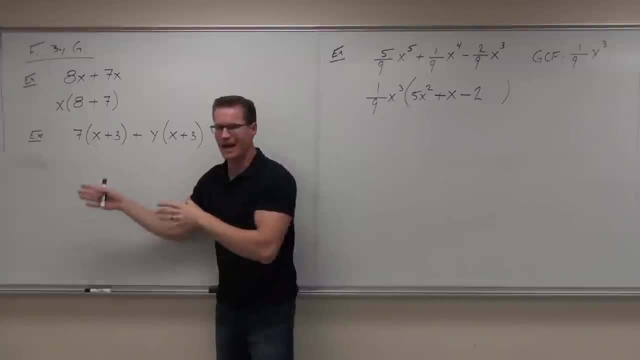 So you get those two x's back again. Now, if we look down here, yeah, it looks a lot more complicated, right, because there's lots of stuff going on, But I want you to recognize what we're doing. You're with me. 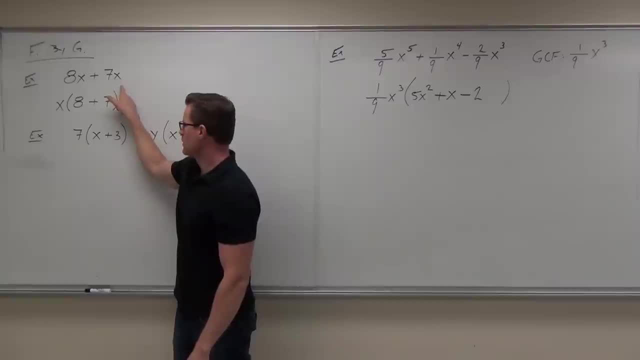 Recognize what we're doing. How many terms do you have here? Two? How many terms do you have here? Look, you have two. This is one term and this is one term. Yeah, they're really big fat terms. 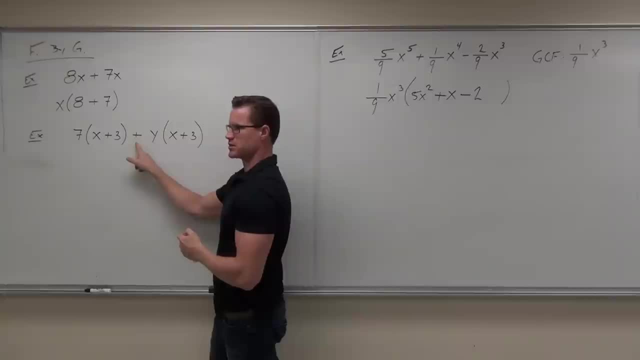 But notice how it's this and this that's separated by the plus. Do you get it? Mm-hmm? What that means is that this is one term, and this is one term. What it also means is that someone's already gone ahead. 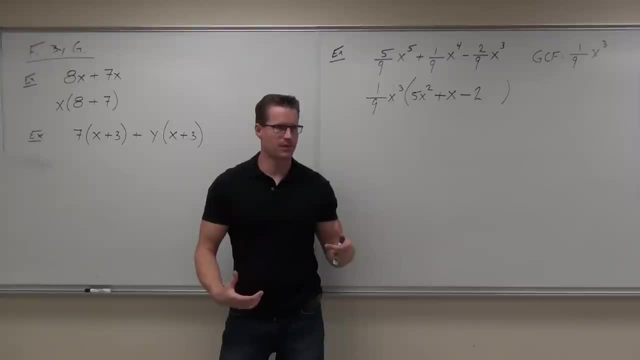 and done the work for you and actually factored it. Have I lost you? Some of you guys are zoning out. still, I don't want to lose you. If you look at this, that's multiplication. yeah, We all know that. 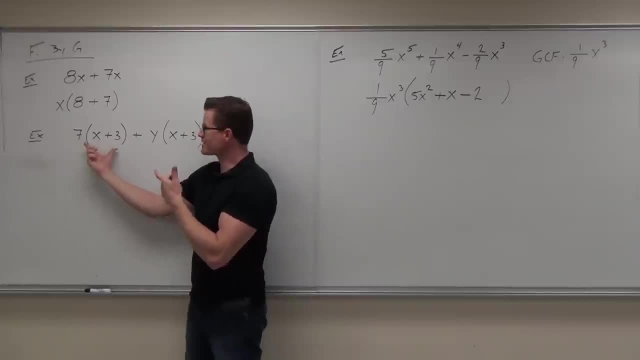 Don't distribute this. Someone's already done the work. That's a factor of 7.. That's a factor of x plus 3.. That whole thing is considered a factor here. Here that's a factor of y. That's a factor of x plus 3.. 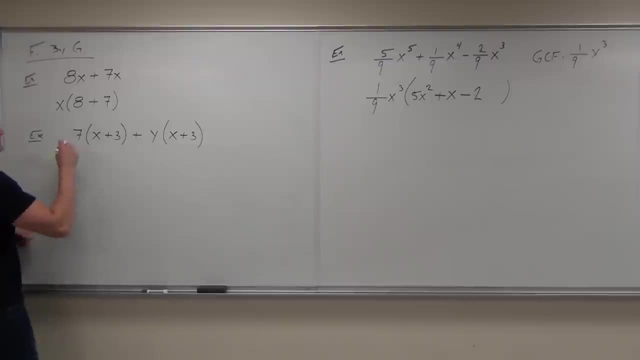 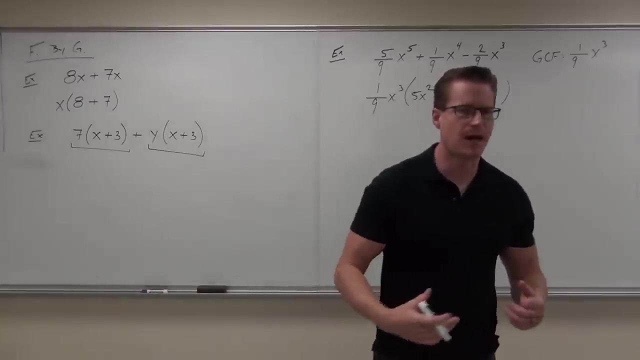 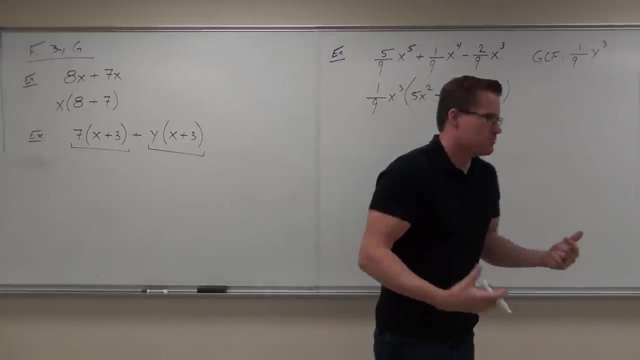 So when we're looking at this, we're basically looking here and here and asking: do these things have a factor in common? A factor is a piece of a math puzzle, a piece of a term, basically A piece of a term that's being multiplied by another number. 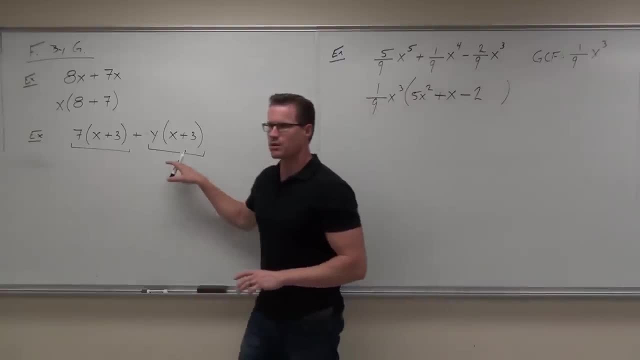 variable, whatever another factor, Do they have a factor in common? Yeah, Now check this out. This x plus 3 acts exactly the same as this x does. The x went out front, didn't it? Are you listening? 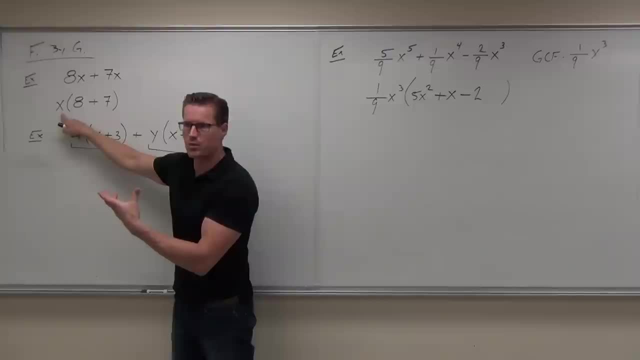 Mm-hmm, The x we did went out front and we're factoring, We're creating even more parentheses. So when I take this x, I go: okay, lookit, that's a factor, isn't it? It's being multiplied. 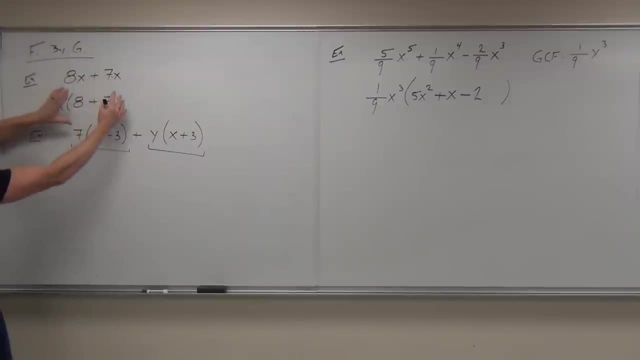 That's a factor, isn't it? It's being multiplied. I take that x, I put it out front, create parentheses. This now, here is my factor. that isn't common, It's the greatest common factor. Take that common factor and put it out front. 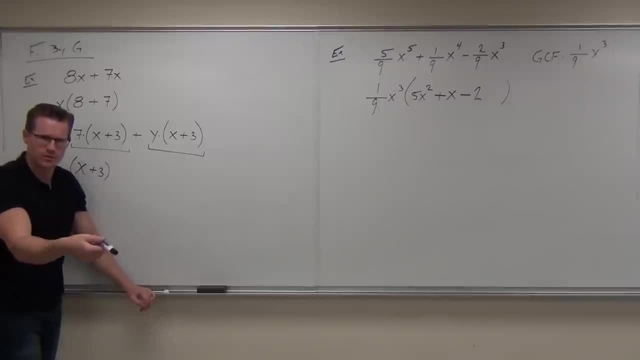 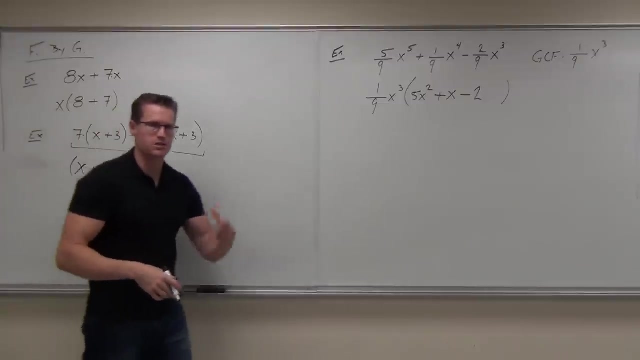 Now wait a minute. Does factoring destroy parentheses or create parentheses? Create parentheses. I already had one set. I need to create another set. Factoring always creates parentheses. So if I factor this, now check out what happened. Look at the. are you guys seeing the similarity? 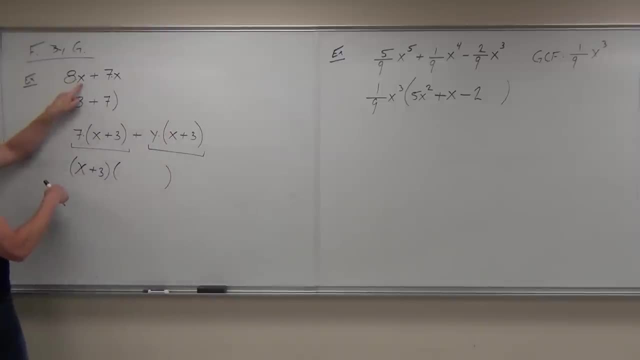 between these two problems at drill? I'm sure, hopefully you would. If I factor out the x, the only thing that's remaining is that 8, do you get it? Yeah, If I factor out the x, the only thing that's remaining is that 7.. 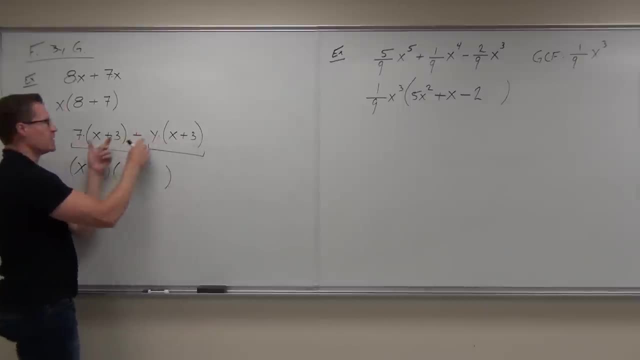 If I factor out my x plus 3,, that's the factor they have in common- what's remaining? if I factor out, divide out the x plus 3,, that's 7,. is going to be there, You with me. 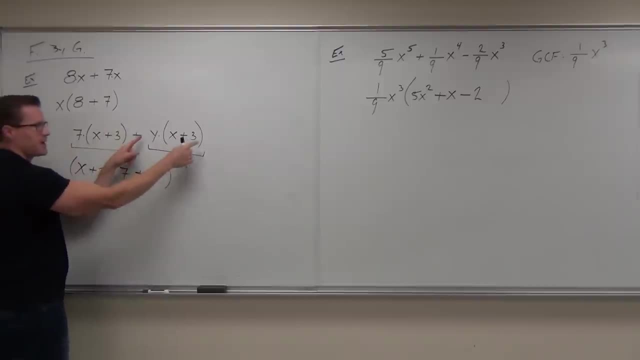 Plus plus. hey, plus plus, plus, plus. If I factor out the x plus 3, the greatest common factor, factor it out what's going to be there? Y, Because I asked you A little math humor, I know. 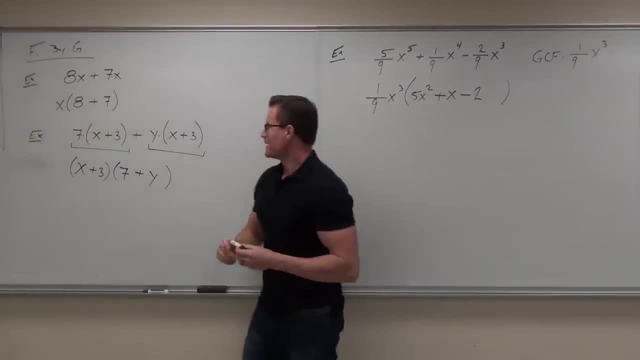 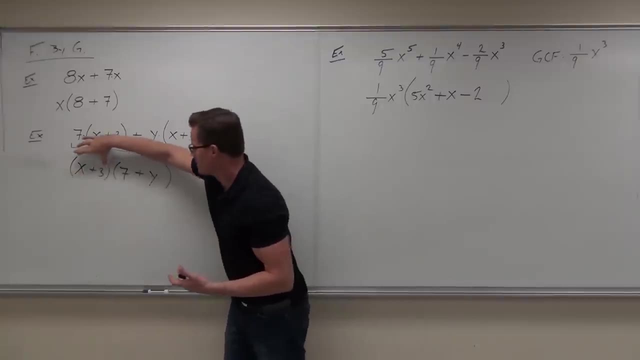 I'm such a dork. Anyway, can you see that if you were to distribute this, if you get the same thing, check it out, x plus 3, it's weird to see, but if you took x plus 3 and distribute it, 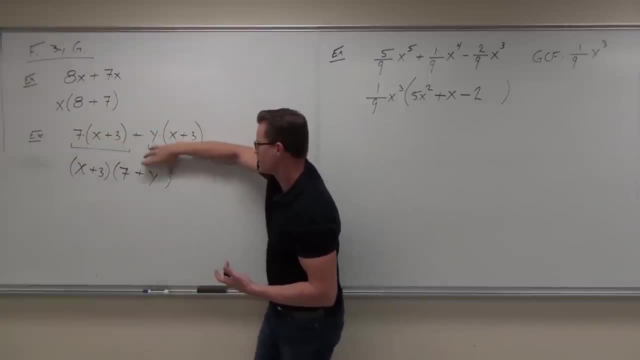 you'd have 7 times x plus 3.. If you took x plus 3 and distribute it, you'd have y times x plus 3.. Show your fans, if you feel okay with that, What I really want to get across. do you understand why there are? 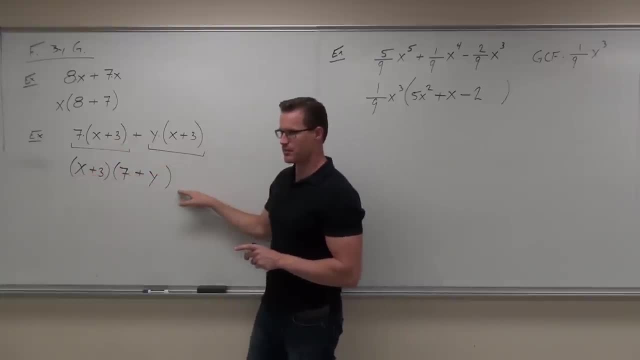 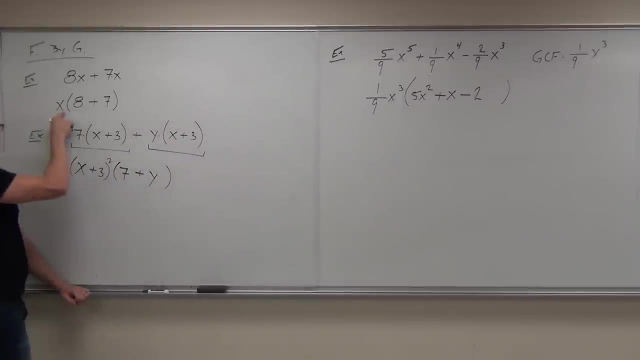 two x plus 3's here and only one x plus 3 here. That's what I want you to get. Do you understand why it's not squared? Is that x squared? No, No, 2x is 1x. 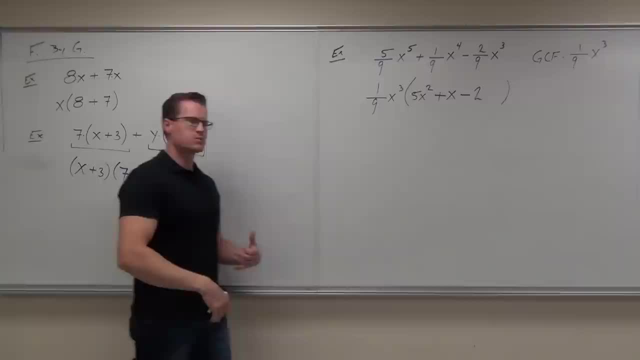 2x is 1x, 2x is 1x, 2x plus 3 is 1x plus 3.. You're factoring it, which means if you distribute it, it's going to go to both terms. 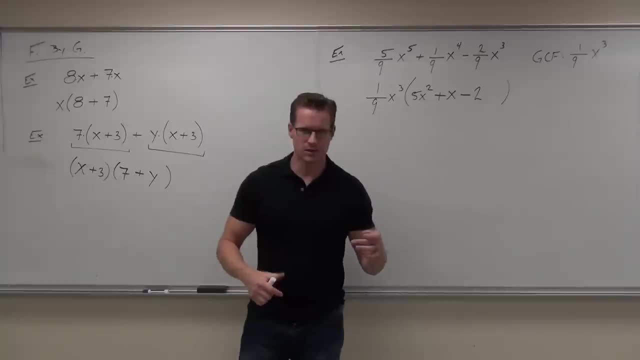 You can see it twice again. If I've explained that well enough, give me a quick head nod if you understand that concept. We're going to practice a lot more, trust me, but I want to make sure that the concept is right. 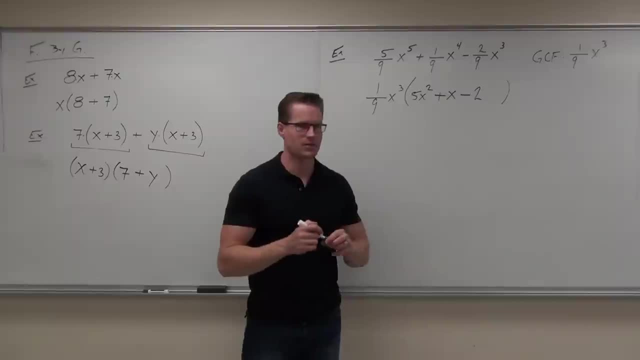 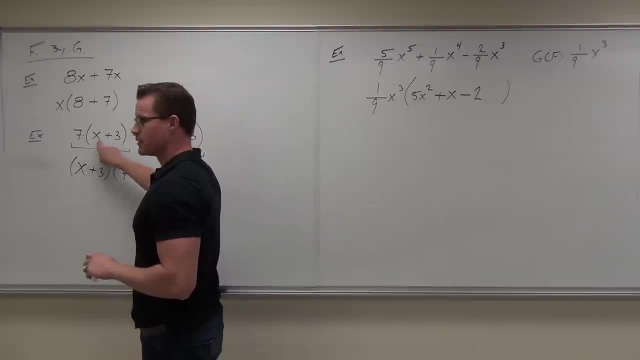 That way you understand this further. You had a question. Oh, I thought I saw a hand go up. Sorry, If it was x squared, it changed the problem. If what was x squared? If it was x squared Here, Yeah, 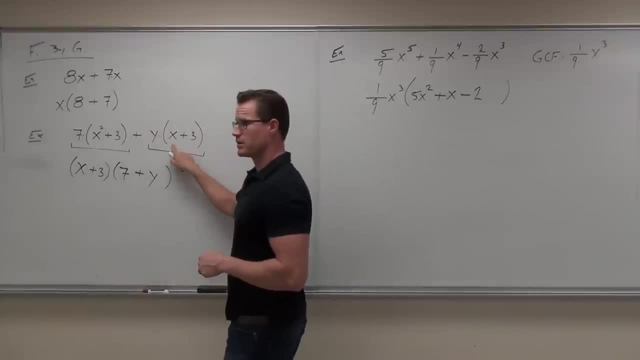 If this were x squared and this were not x squared, you couldn't do it. If this were x squared and this were x squared, it would be no different. That would be x squared. All I'm trying to tell you is these two things have 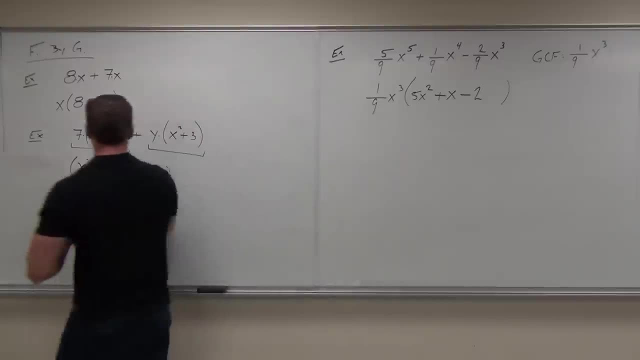 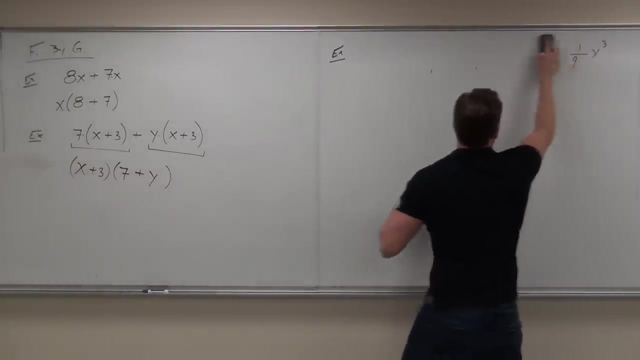 to be identical. That's all you have to know. If these are the same, you're good to go. If they're not the same, you've got problems. You've got problems anyway. Okay, Tell you what? why don't we try a few more? 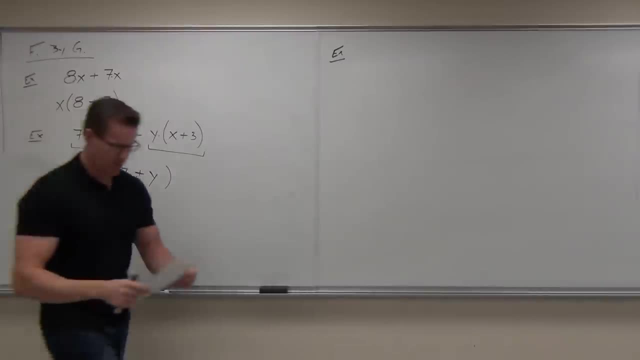 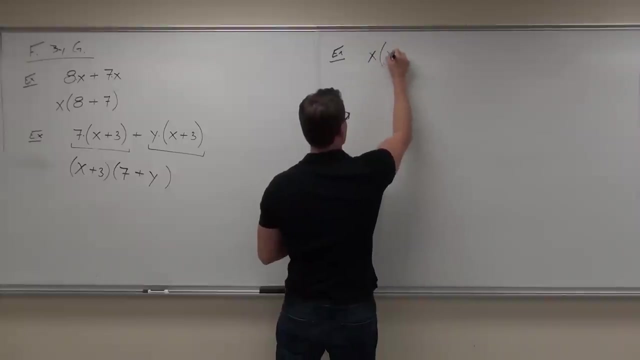 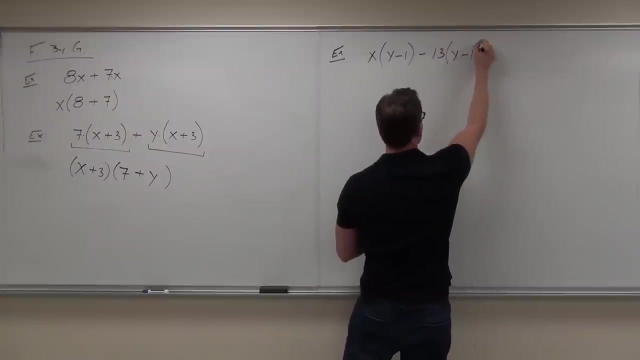 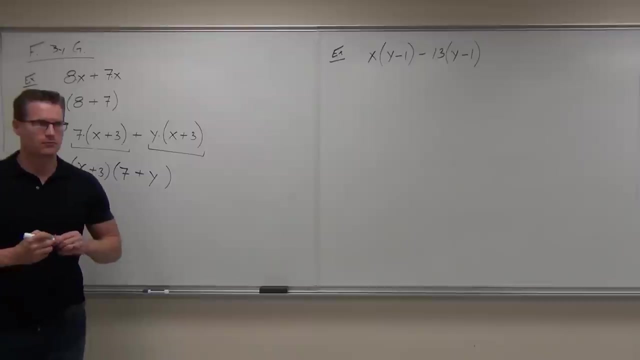 so you all get the hang of this. In fact, I'm going to have you do one right now, just on your own. I'm going to kind of lead you through this, but you're going to do all the work here. The first thing I want you to look for: how many terms do I have? 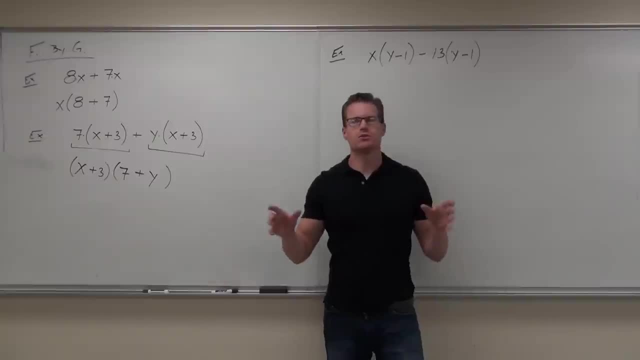 Two Big terms. Yeah, they're really big terms. Do those two terms have any factors? Remember, factors have to be contained in parentheses. Do they have any factors in common? Yes, What factors? Y minus 1.. Okay, So write that y minus 1 in front. 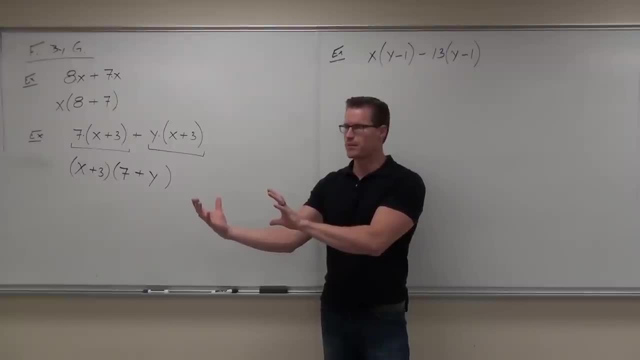 Did you get it? How many y minus 1's should you have right now? One, Because you're factoring, It's coming out of both. Next you're going to factor. it always creates parentheses. always Create another set of parentheses. 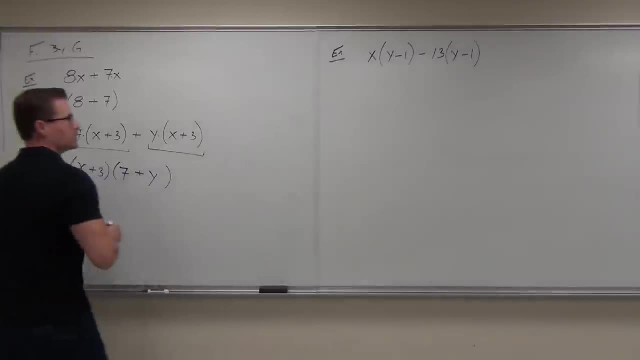 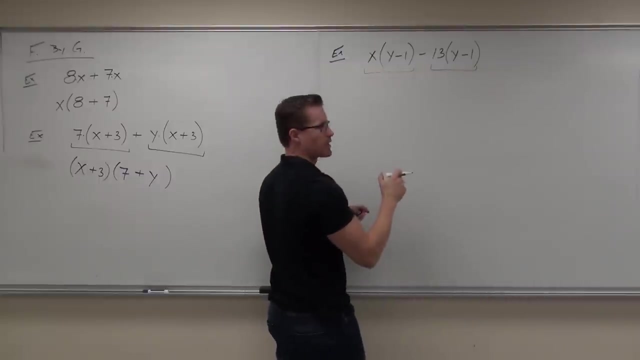 Did you do that already? Yes, Yes, So you say two terms: 1, 2.. Anything in common? Yeah, common factor is what we're looking for. Common factors have to be in parentheses or be multiplied. So y minus 1 is the common factor. 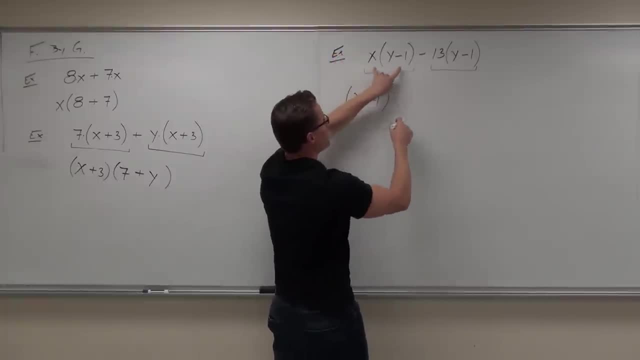 That's what we did before. right Wrote the GCF first. Now, if I divide by y minus 1, you can do it here. If I divide by y minus 1, well, those would go away. You would get simply x. 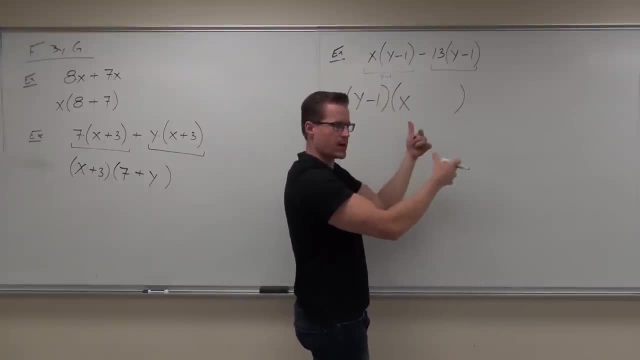 Why? Well, because you're factoring, You're dividing out that y minus 1.. It's going from both terms. That's great Cool: 13y minus 1 divided by y minus 1.. What's going to happen? 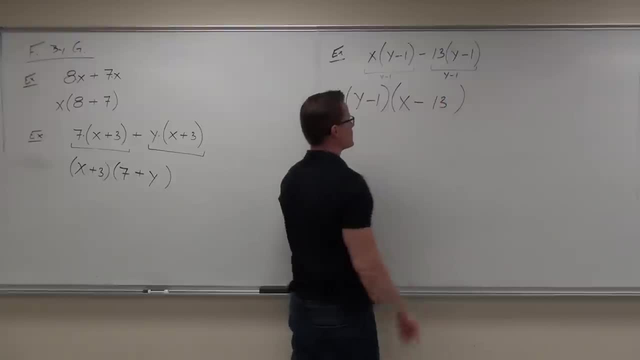 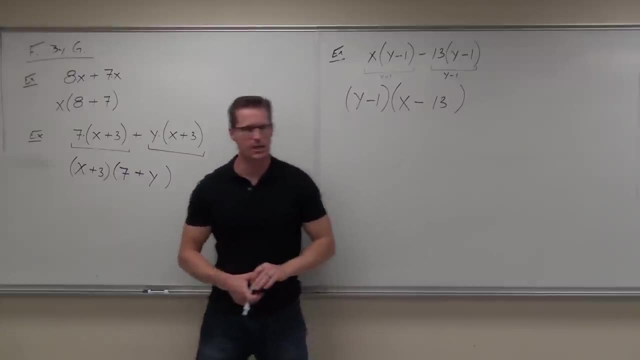 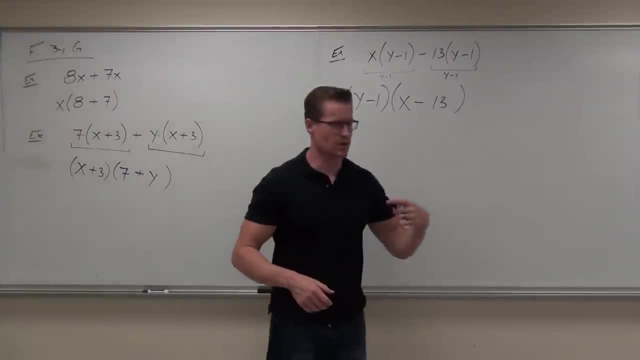 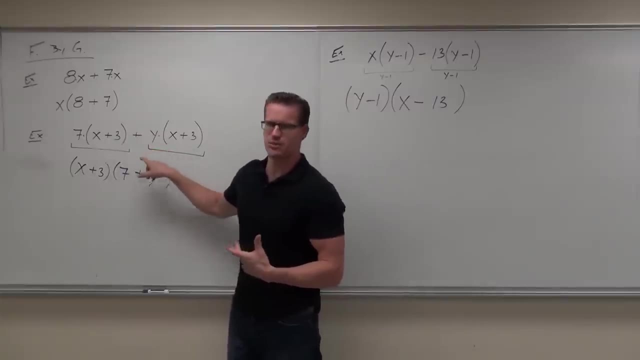 We're going to go back to the last one. All right, We're going to end there. Next time we're going to start on a little bit more advanced concepts. I'm going to give you ones that don't automatically look like this, because this right now is really simplified, okay. 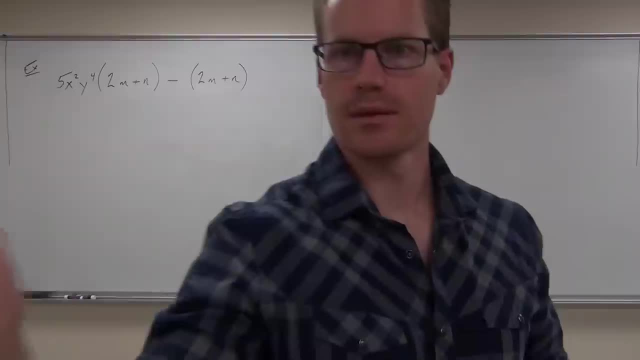 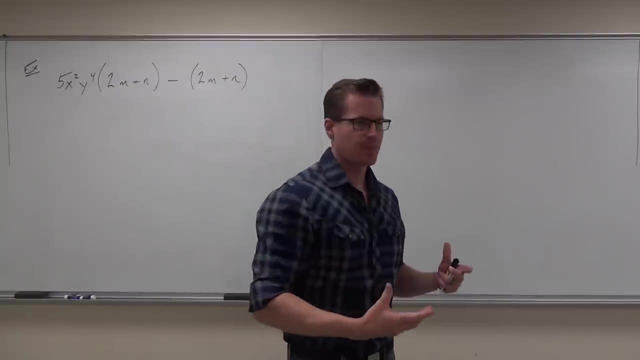 We're going to start figuring out how to do that. All right, So we're going to continue our journey through factoring, and what we were discovering was that when we have a GCF- the greatest common factor, it doesn't necessarily mean 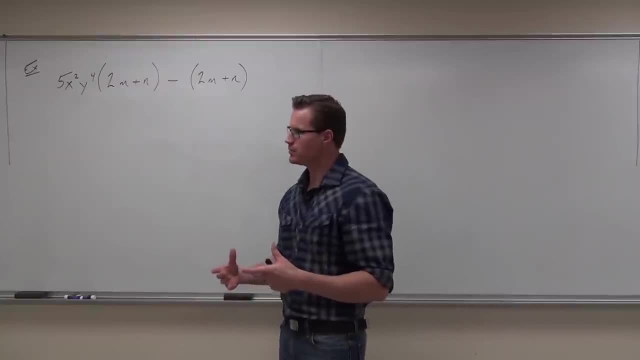 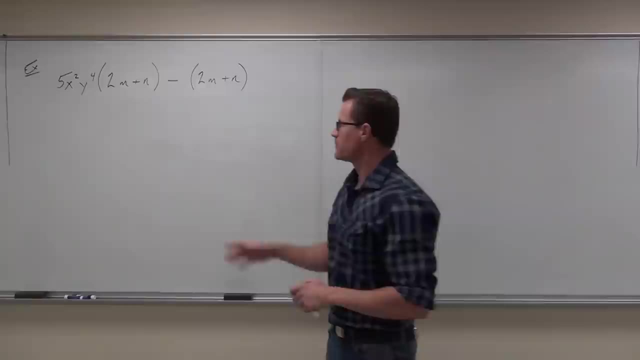 that it's just one number or one variable. It could be an entire factor in parentheses. It could be an entire factor in parentheses. It could be an entire factor in parentheses. And that's what this factoring by grouping does for us. It says: you know what, even if you have something like this: 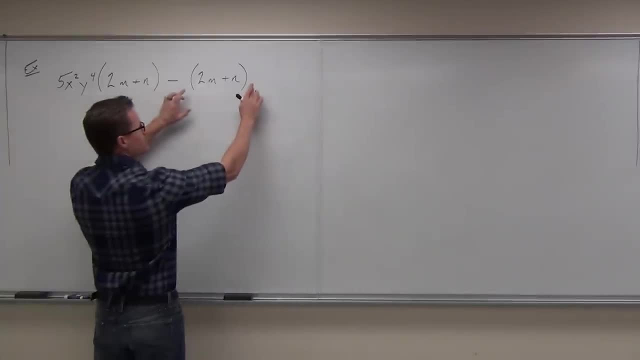 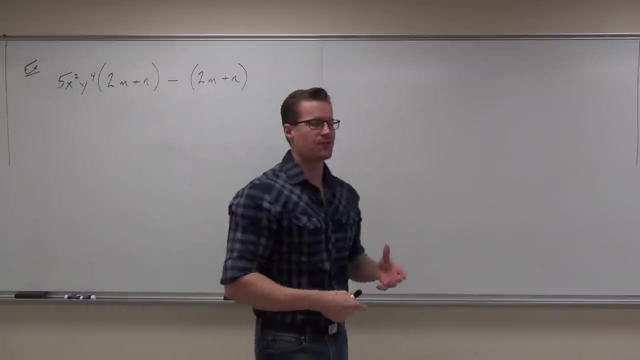 where this is one large term and this is another term separated by that minus. even if you have these two terms, we're still looking for factors, and factors are really anything that's grouped together that's being multiplied by the remaining part of that term. 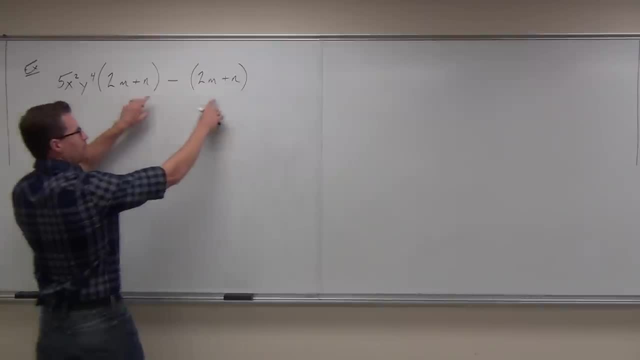 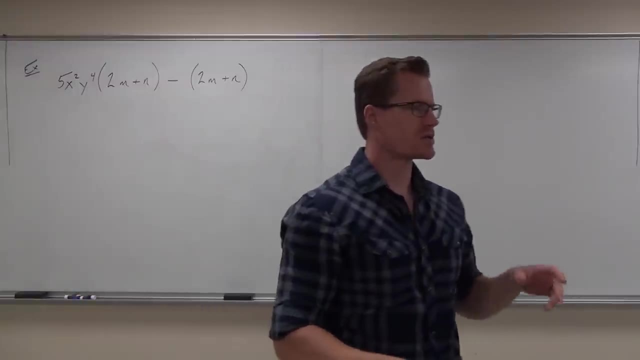 So for instance, this right here, that's a factor and that's a factor of these one, two large terms And factoring by grouping. I know this is the last time but it's kind of a refresher. factoring by grouping says we: 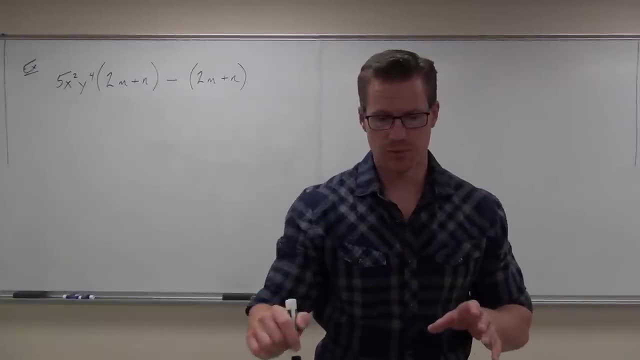 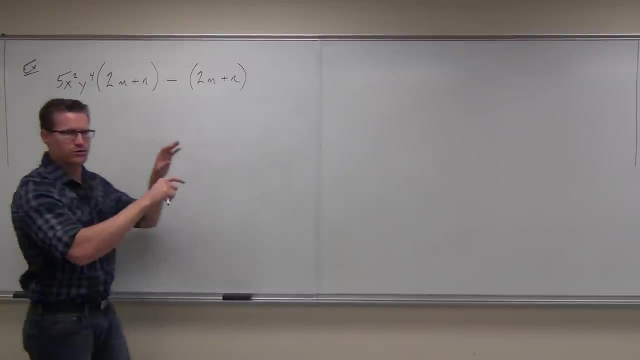 can factor. as long as those two things are exactly the same. Watch your foot, please. As long as those two terms are factors- are exactly the same. What that means is that we can remember what factor does right. Factoring is the opposite of distribution. 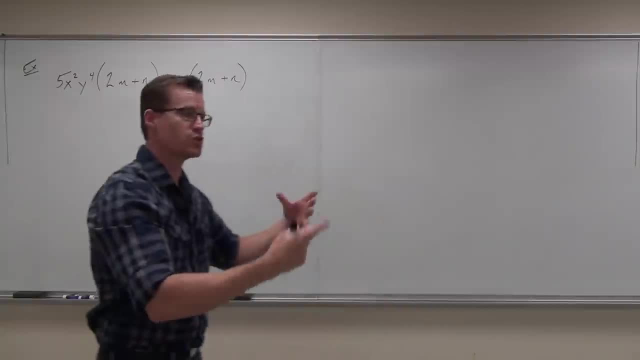 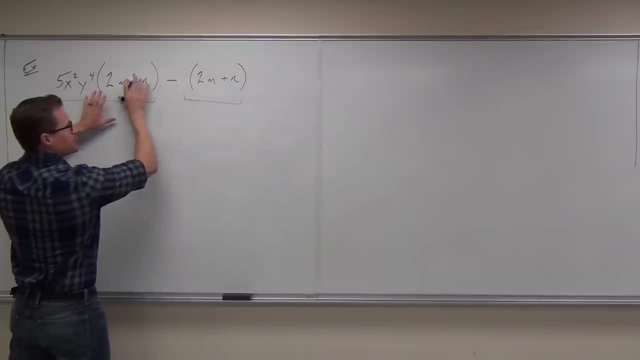 So where distribution destroys parentheses, factoring creates parentheses, a new set of parentheses. What the factoring says is out of these two terms: if they have a common factor, the greatest common factor, we write that common factor out front, just like we normally would. 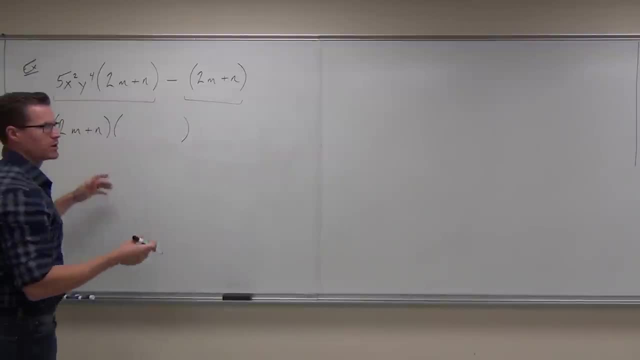 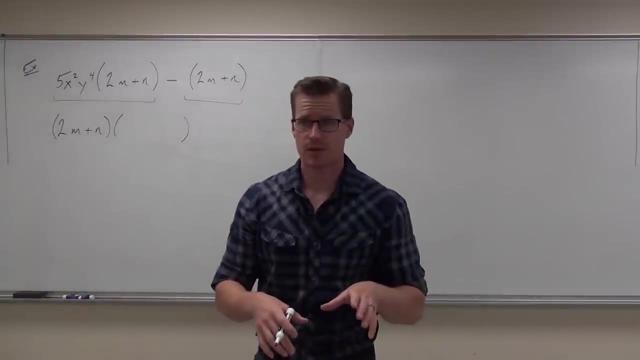 We create a new set of parentheses, just like we normally would, and then we find the remaining two terms by dividing. Remember that does factoring ever get rid of terms. So if you start with two, you're going to end with two inside of your parentheses. 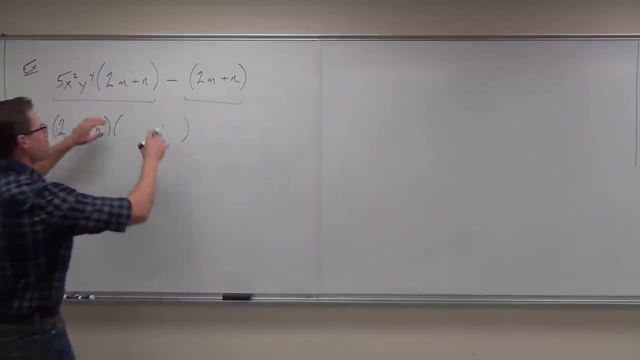 You might just have a new factor out front. So here, if I factor away my 2m minus n, remember you can even show that if you wanted to divide by 2, sorry, 2m plus n If you want to divide by that. 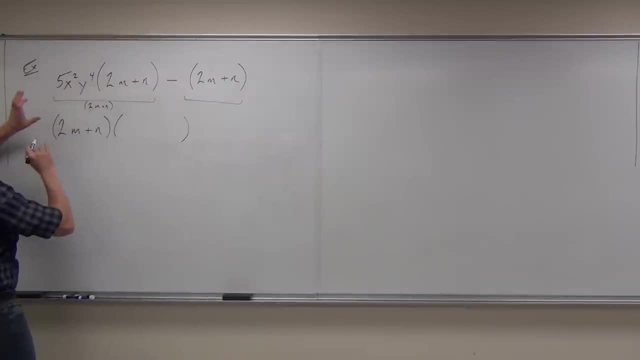 those are gone. what's remaining from that big term? 5x squared minus 1.. So from this term we get the 5x squared 1 to the 4th Quick hit now, if you're okay with that so far. 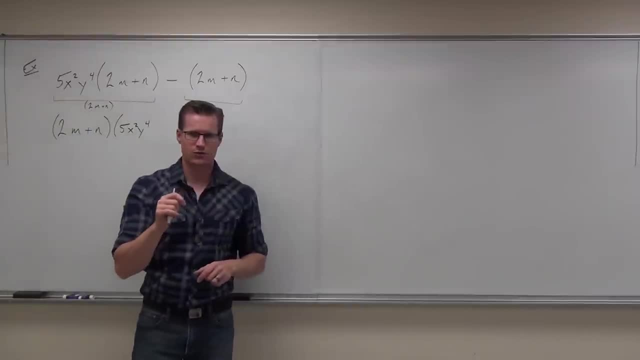 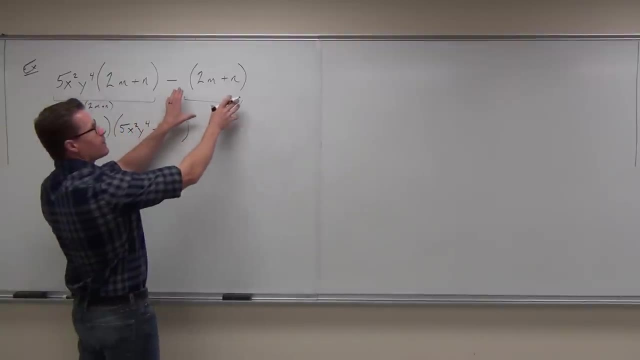 Is that sign going to change? When does that sign change? if we do what? If we factor out of it? So here's, so it'll be minus. We do the same thing here. Now, wait a minute, If, when I factor this and I take this thing away. 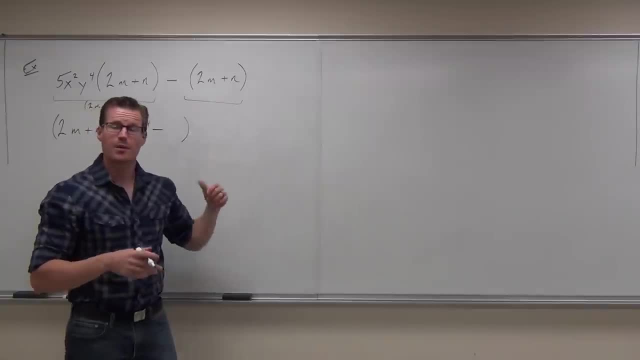 it's going to be minus 1.. So what's going to happen? So so, so to speak, Does that become a zero? No, Now remember, the smallest thing we can ever get is what One? Yeah, And because that's because we're dividing. 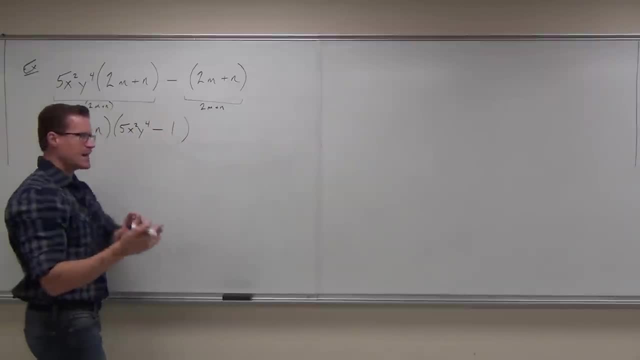 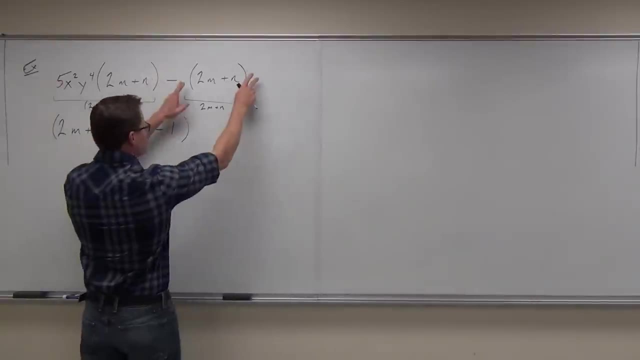 So if we divide this out- that's what factor it is- we're actually going to get a one. We never eliminate terms. You're always going to have the same number of terms inside the parentheses as what you started with. We start with one, two big terms. 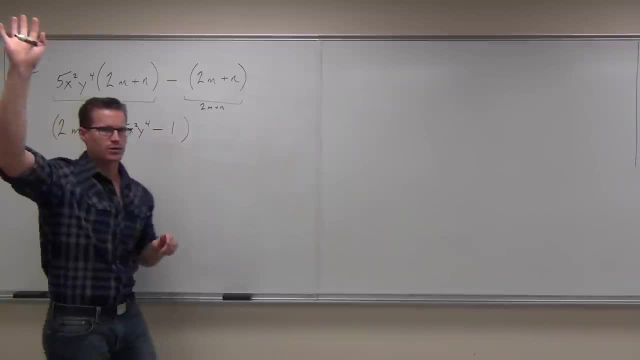 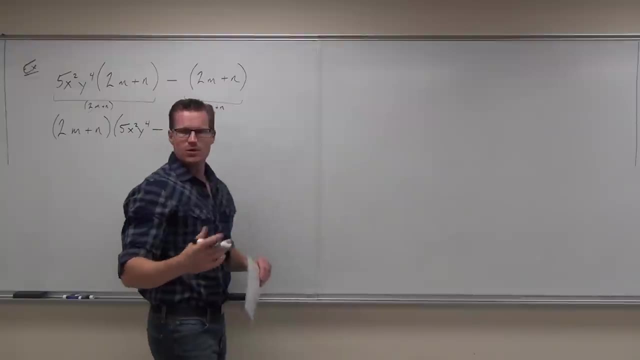 We end with two terms inside the parentheses: Show your hands if you feel okay with that. so far Good. So just a little refresher to get us rolling today. And now I'd like you to try one just on your own. really similar idea. really similar idea. 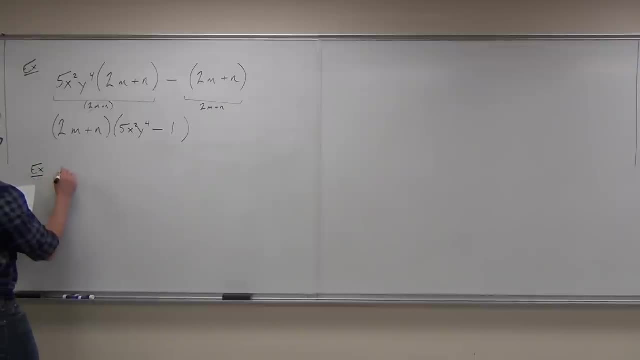 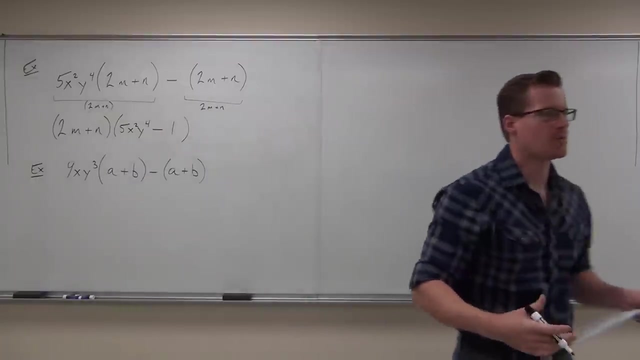 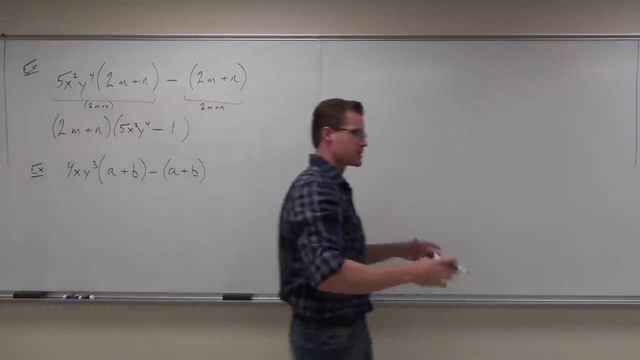 but just with this. Okay, go for it. So I want you to, I want you to verify how many terms are there. first, Just look at the number of terms that you have. Remember. terms are those big pieces separated by pluses and or minuses. 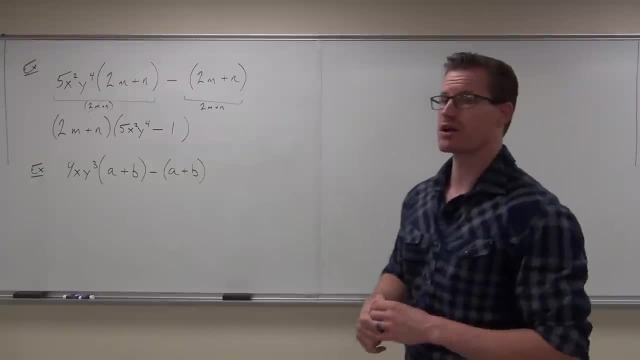 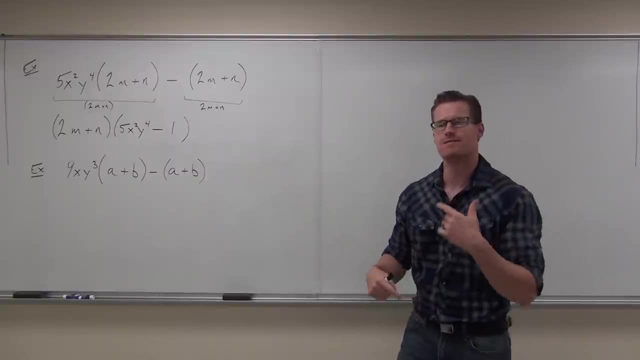 Then what I want you to look for inside those terms. do they share a common factor? If they do factor that, factor out, So put that in front around parentheses, create a new set of parentheses and then divide to figure out what those new terms are going to be. 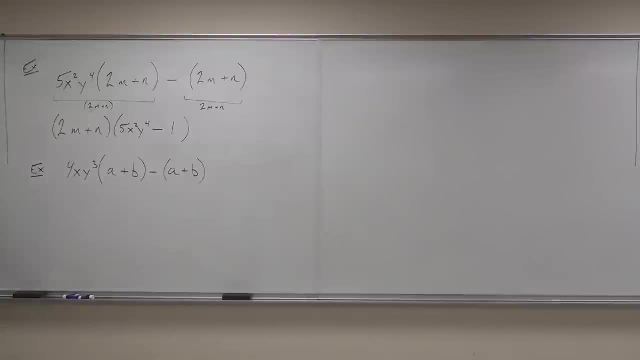 Okay, so let's go for it. How many terms do we have here? Two, Yeah, two big terms are separated by that minus sign. Do we have a common factor? Yes, What is the common factor? A plus B, That's right. 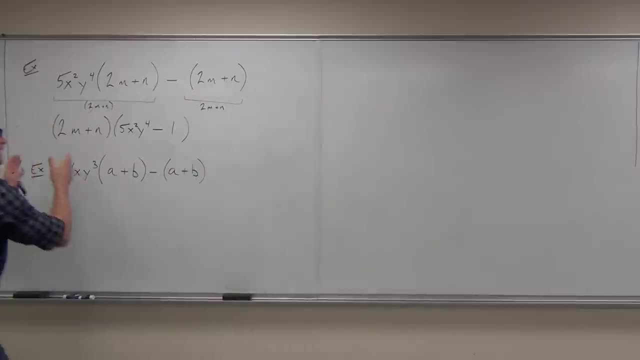 It's all contained in the parentheses. That's what we'd have to have happen. Otherwise we would have several terms here if those parentheses weren't there. Here, factor, factor- in these two terms We write out our common factor first. 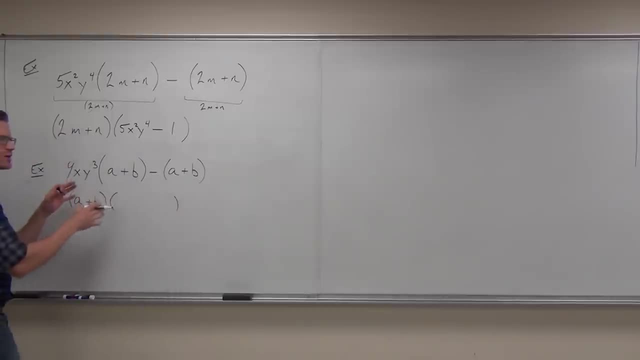 Then we create a new set of parentheses, Because we're factoring. we write out our common factor first. And if we were to divide this away, what happens when we divide out the A plus B? What do we get left, Minus 1.. 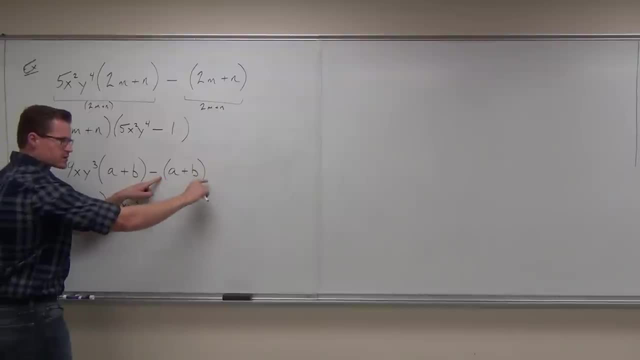 Minus doesn't change. What do we get here again? 1. Yep, we're dividing this. So A plus B, divided by A plus B, gives us our 1, and we're done. Show of hands if you got that one by yourself. 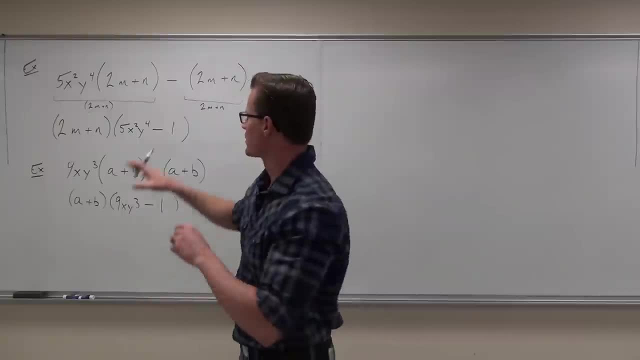 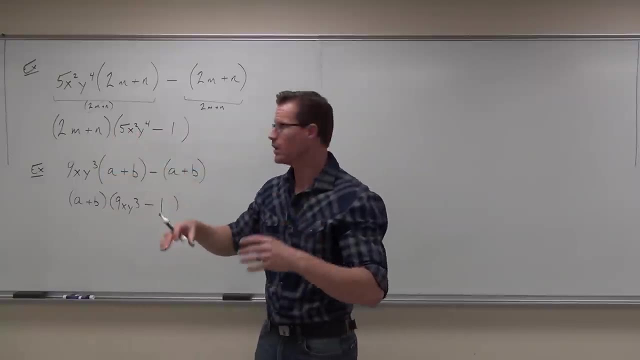 That's really good. Now we're going to make the jump Right here. this has basically been kind of done for you. The first step has been done for you. You don't know it yet because we haven't talked about factor by grouping in its whole. 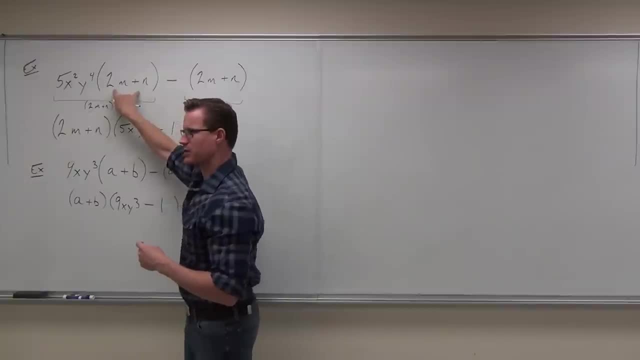 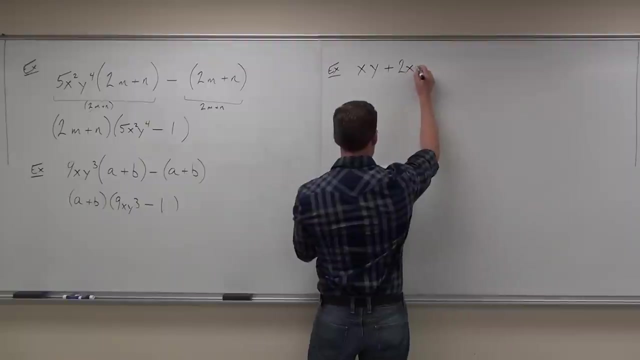 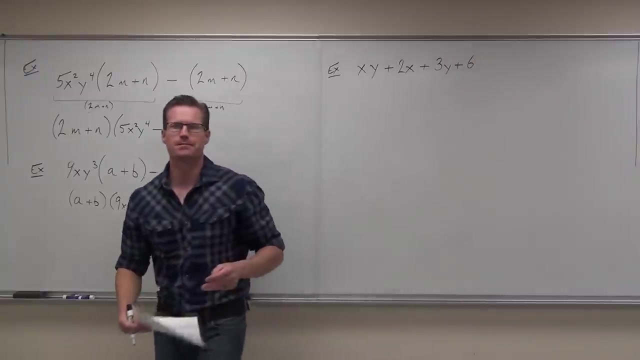 But here Someone's factored this, so you have that factor here and that factor here. What I'm talking about are examples that look like the following. Let's look at that example together. The first thing I want you to notice is the number of terms that we have. 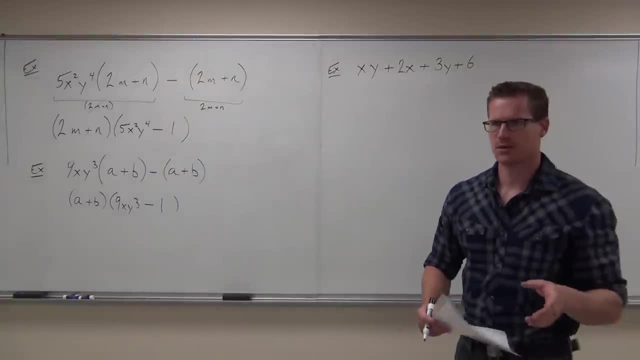 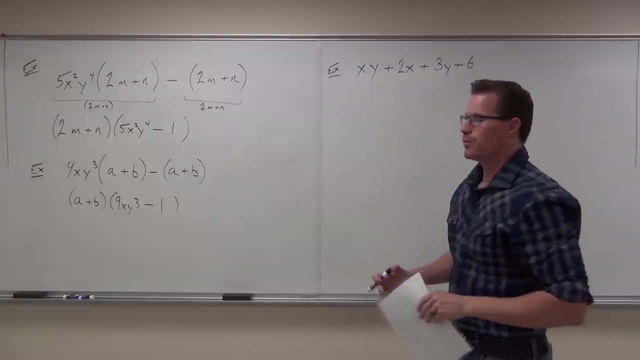 How many terms do we have? What do we have here? Four, Yeah, there's four terms. That's different than before. right Over here we had two terms, Here we got four terms. Now I don't want you to ever miss this ever. 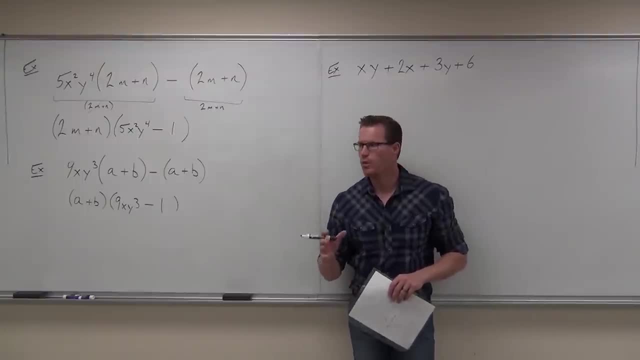 First thing you do whenever you're factoring: you always, always look for a GCF. if there is one, Always. I don't care what you're doing, You always look for. that Is that clear. No matter what other factoring I teach you about, always look for the GCF. 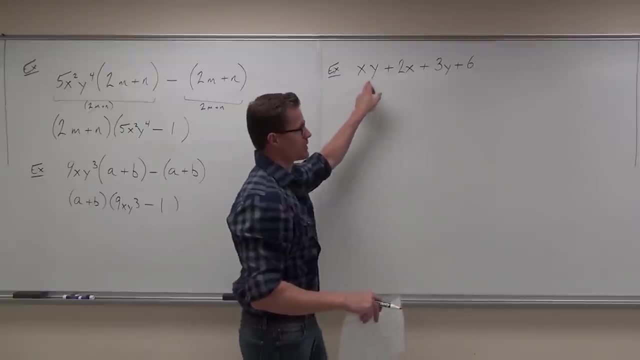 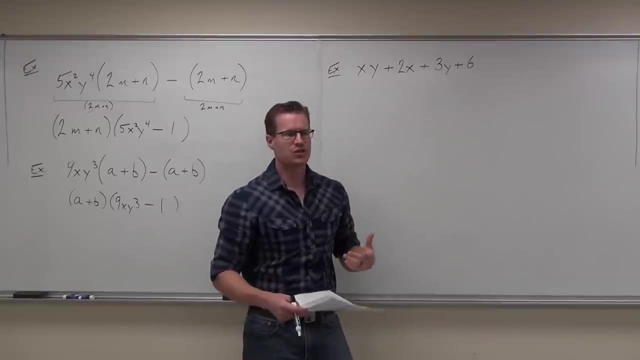 So we're going to look for it. Does this have a GCF? Remember, you've got to consider all four of these terms. Does it have a GCF? No, No, But that's what we check for first. Now, if it had a GCF, great, you'd factor it out. 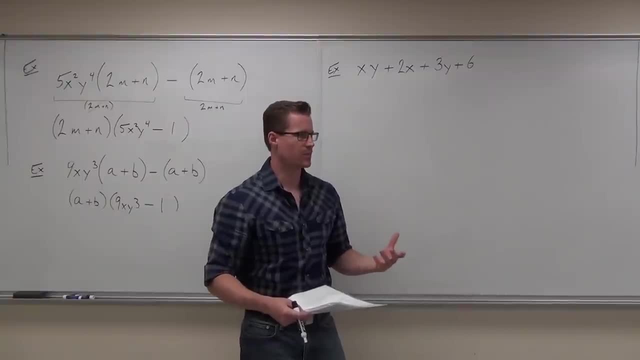 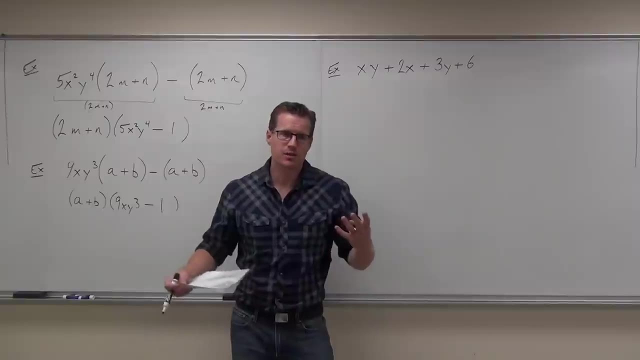 If it doesn't, we've got to consider something else, something else to do In this class. if there's four terms and you're asked to factor, practically the only thing we can do with that is try to factor by grouping. So here's how you factor by grouping. 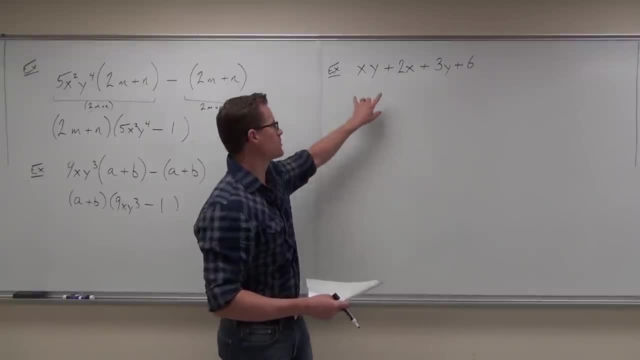 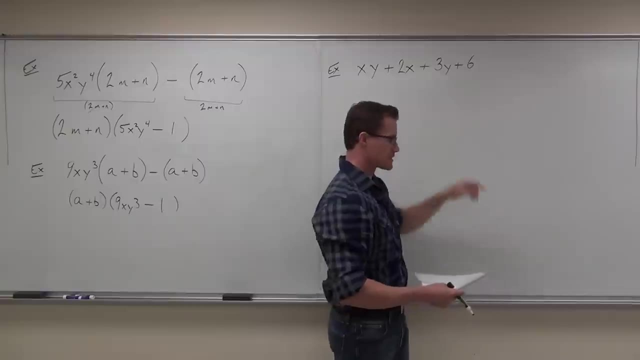 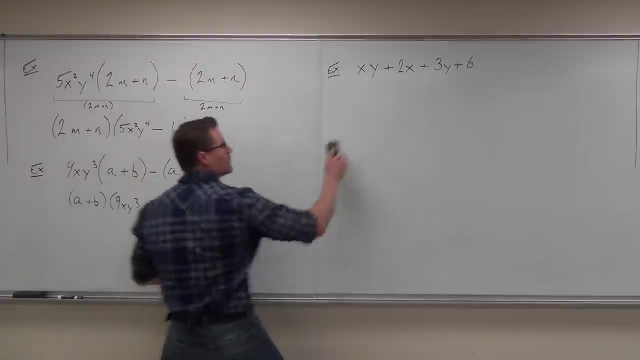 You organize these terms so that the first two terms have a common factor and the last two terms have a common factor. What that means is that sometimes- I'll show you this right now- If these things, what was that? a 2x and a 3y? is that what I gave you? 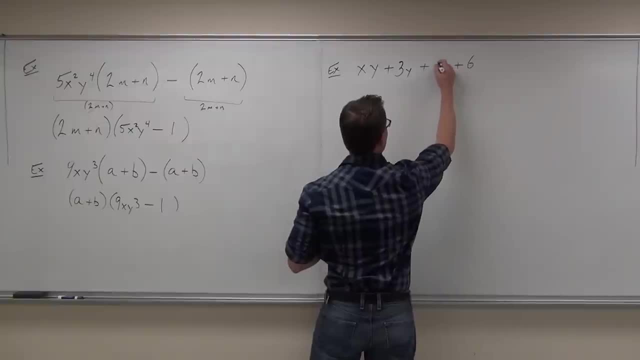 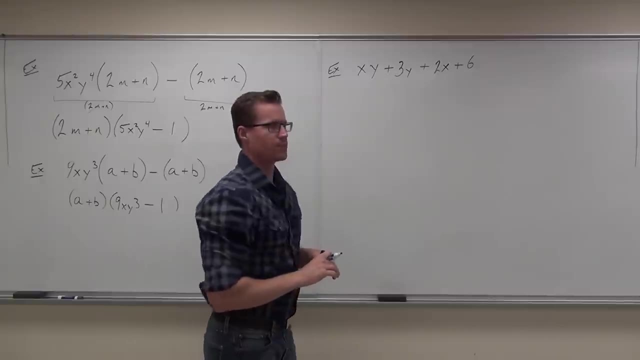 Yeah, If these things. are you sure it was a 2x? That was right. Yes, If these things are out of order, sometimes it won't make a difference, and sometimes it will make a difference. You might have to rearrange them. 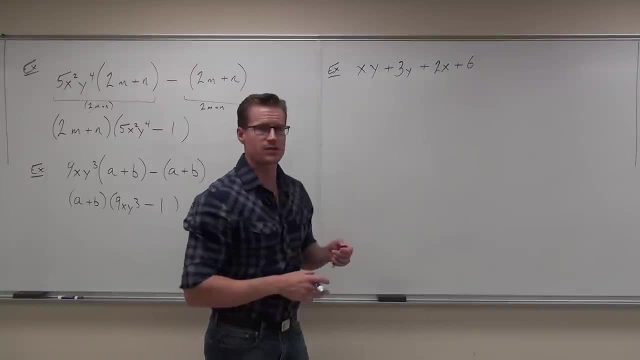 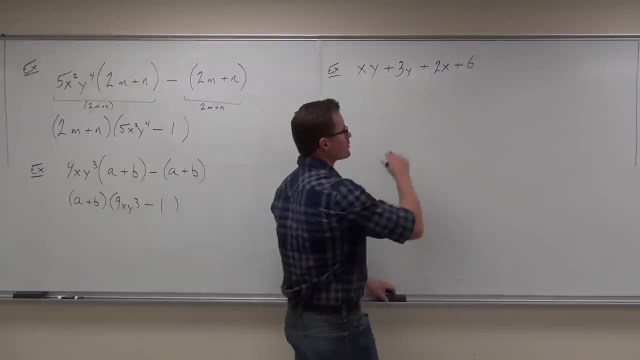 In this case it doesn't make a difference. In some cases it will make a difference. You would have to arrange them certain ways. Does that make sense to you? So for us, either way, you do. in this case, we're going to group these. 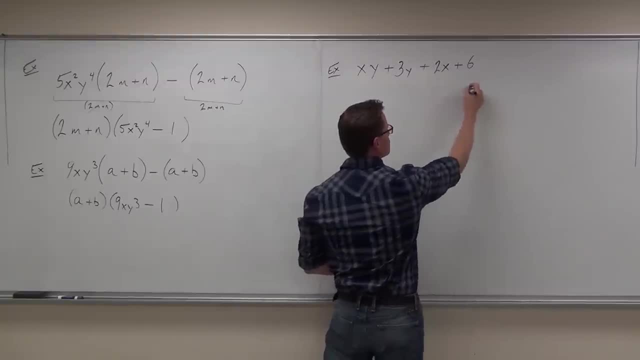 so that the first two terms have a common factor and the last two terms have a common factor. Which way did you guys write it down? This way or the last way? The last one, The last one, The last way, Okay, And then a 2x right. 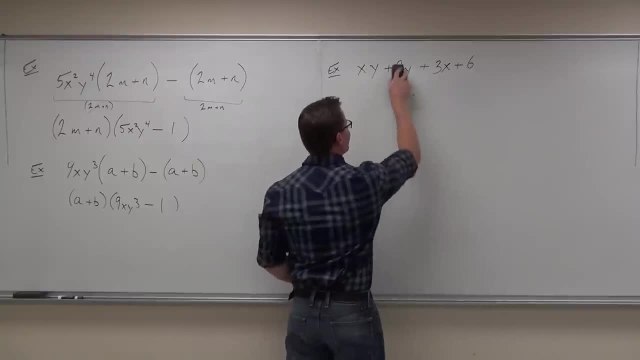 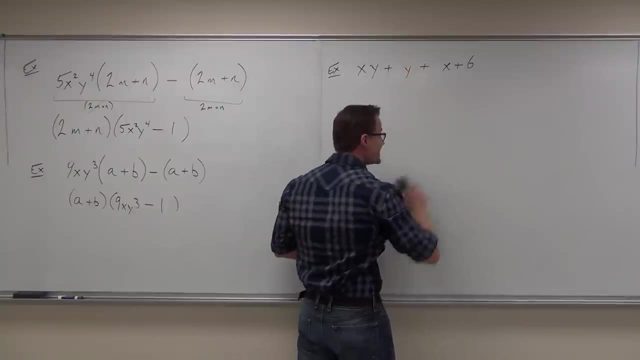 2x, 2x, 2x, 2y, 2x, 2y, 2y, 2x, 2y, 2y, 2x, 2y, 2x plus a minus 3y. 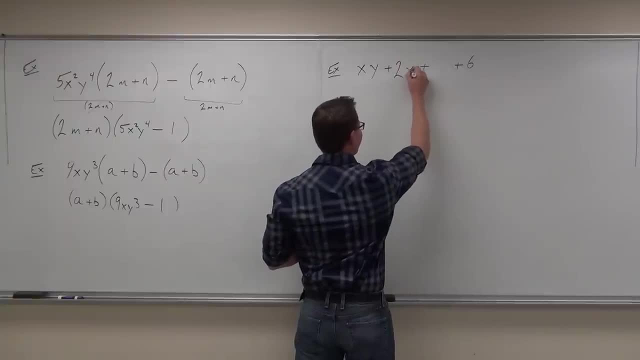 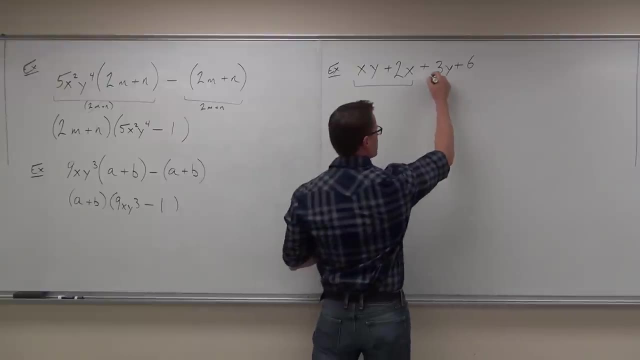 2x, 2y, 2x, 2y, 3y, 3y. Oh good, Okay, Good, So they're grouped either way. I just wanted to mention that sometimes you might have to look at organizing them in a certain pattern. 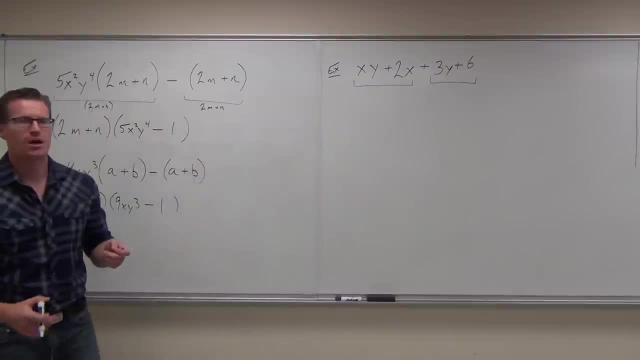 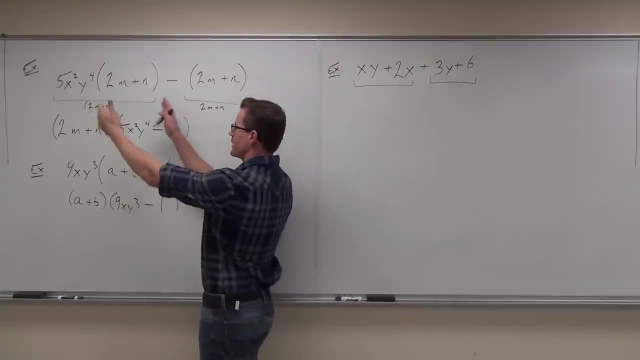 Group: the first two terms and the last two terms. what you're doing is you're trying to go from our four terms, like this, to our two large terms, like these, examples where you have a common factor. That's the idea. If it doesn't work, the first: 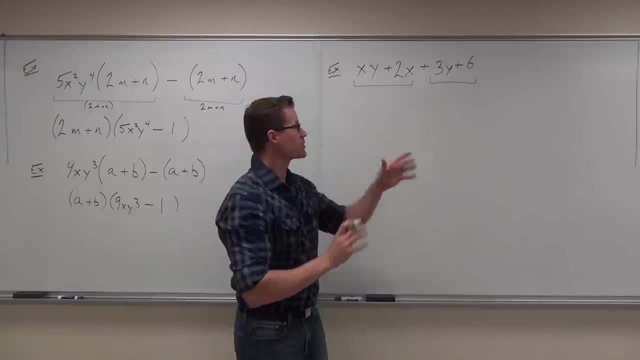 time, reorganize your terms and maybe it'll work a second time. So for us, look at our first two terms. Is there a greatest common factor here, The x? Now I'm going to start going a little quicker on our factor, because we talked so much about it, okay. So here, yeah, if we factor out, 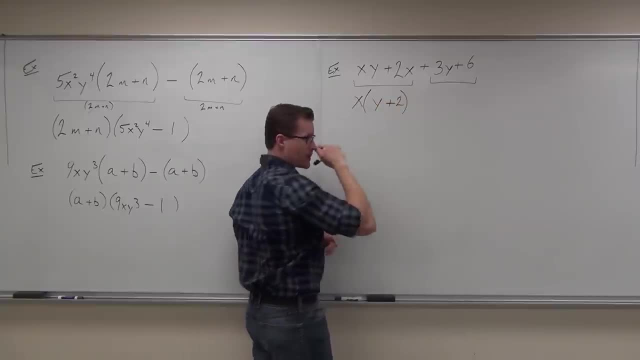 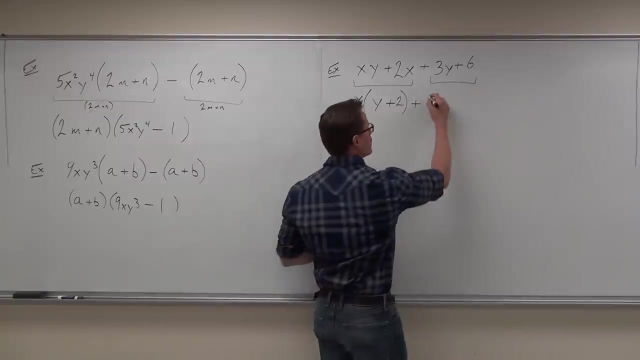 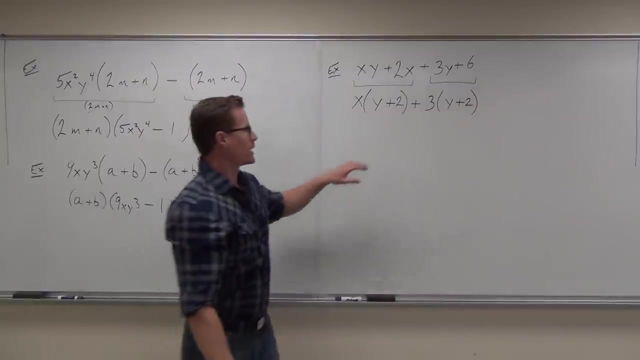 the x, we have y plus 2.. Can you verify that for me? Yeah, You sure. Okay, Plus sign, plus sign. It's not going to change. Now, does these two terms have a common factor? Three? Factor out the three, we get y plus 2.. If it's factorable, it will work out so that these two 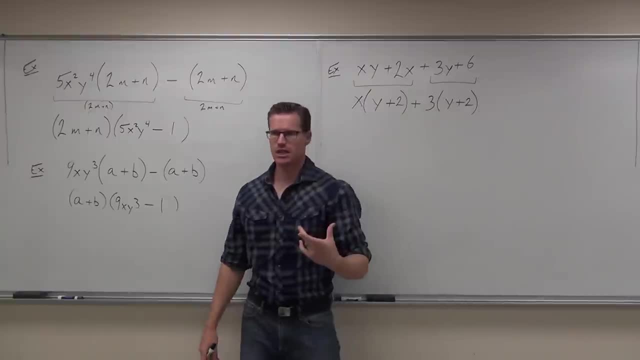 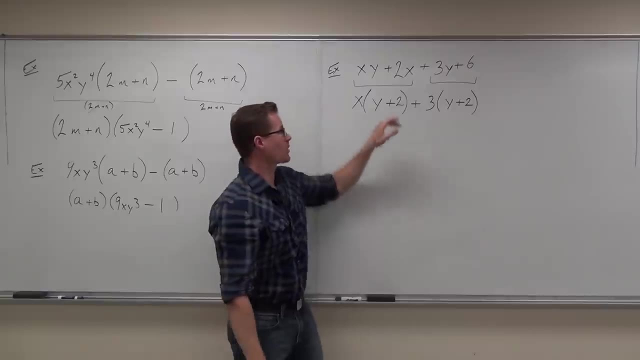 factors are exactly the same. If that happens, then you continue, If it doesn't, you try to reorganize your terms or it's not factorable, Quick hit note if you're okay with that. What I want to know is: are you okay getting the x factored out and getting the three factor? 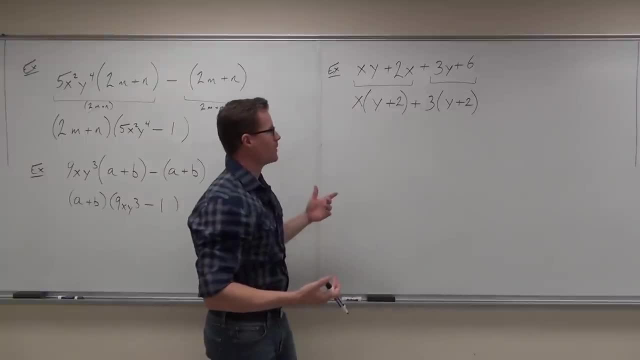 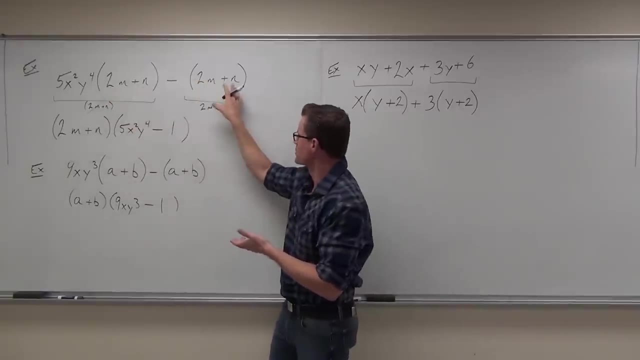 out Show of hands, if you are. Okay, very good. Now, well, wait a minute. That looks exactly like what we did over here, doesn't it? It's exactly the same thing. Here's one big term, another big. 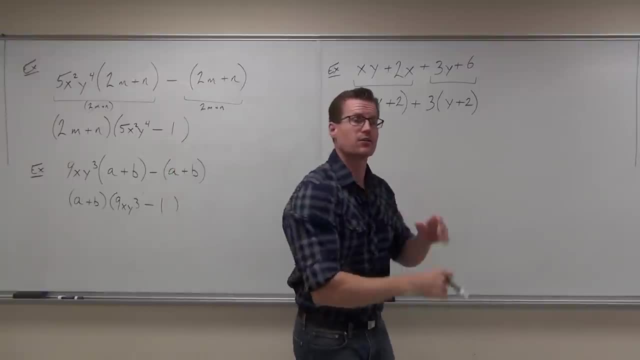 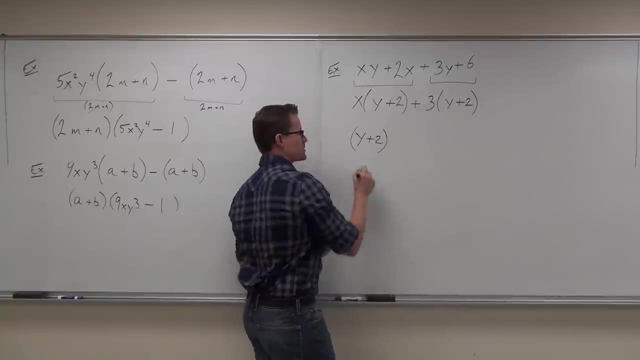 term. We had a common factor. We're just going to divide out or factor that out. What happens to my y plus 2?? What do I do with it? Yep, So we have y plus 2.. I have parentheses. What happens to? 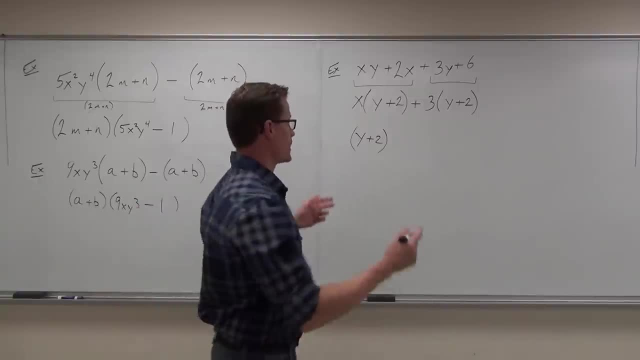 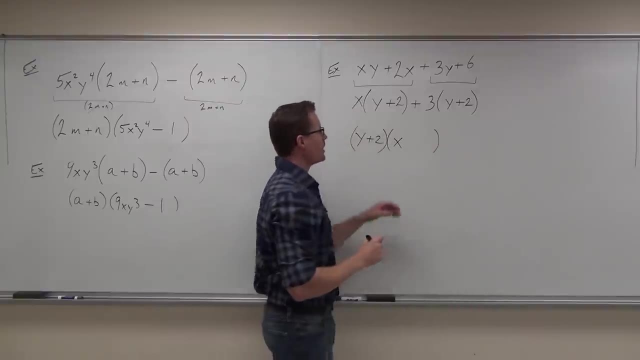 my y plus 2?. What's the next step that I'm going to do? Just write x plus 3.. Okay, factoring creates a new set of parentheses, So create another set of parentheses If I factor away the y plus 2,. 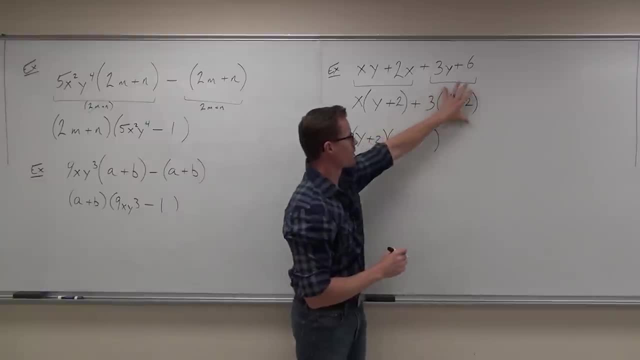 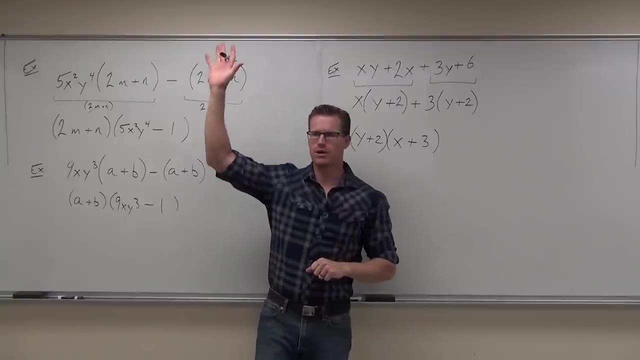 I can divide it. If I factor away the y plus 2,, I'm getting x. If I factor away the y plus 2, I'm getting plus and 3.. I want to show of hands if you feel okay with that one Now. could you check? 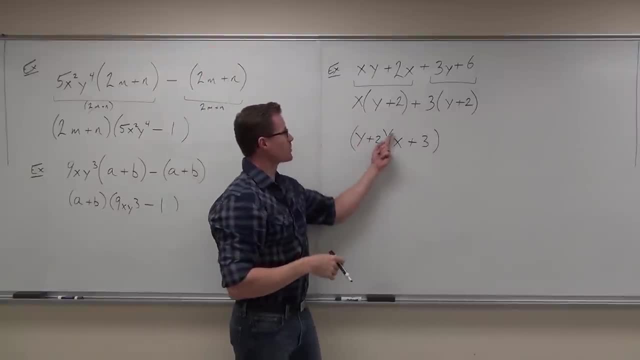 your work. Yes, sir, If you distribute this. here's your y times x, or x times x, x times y is the same thing. Here's your 3y by FOIL. Here's your 2x, right there. Here's your. 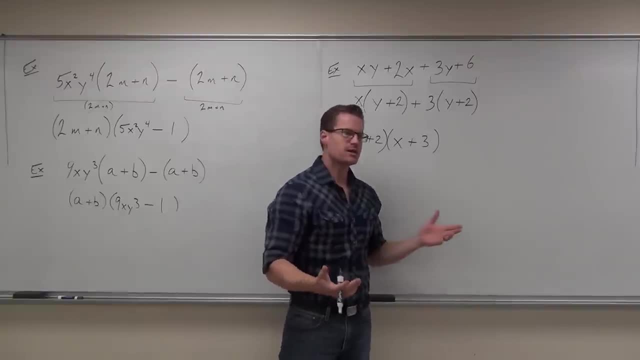 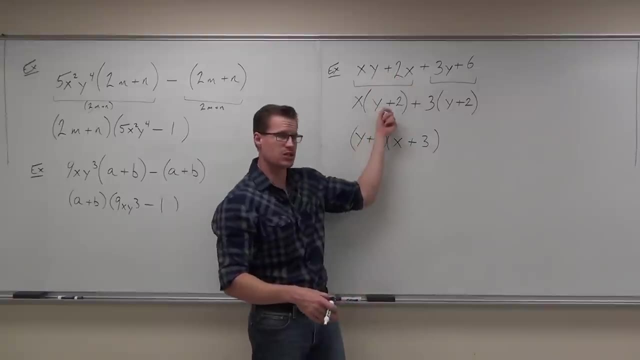 plus 6.. It has to work if you've done it right. That's the idea behind factoring by grouping. Basically, we've done this like baby steps. at a time I showed you how to factor a GCF. I showed you how to factor with these awkward-looking factors. Now we're just putting that idea together. 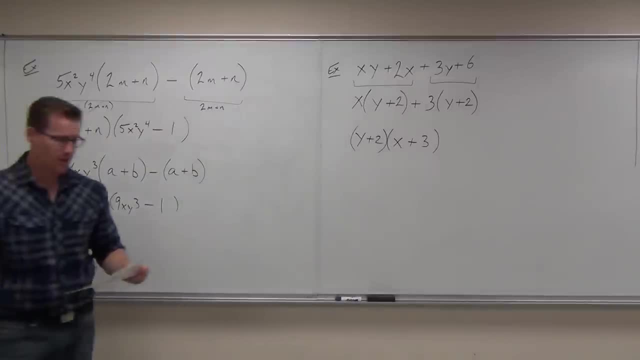 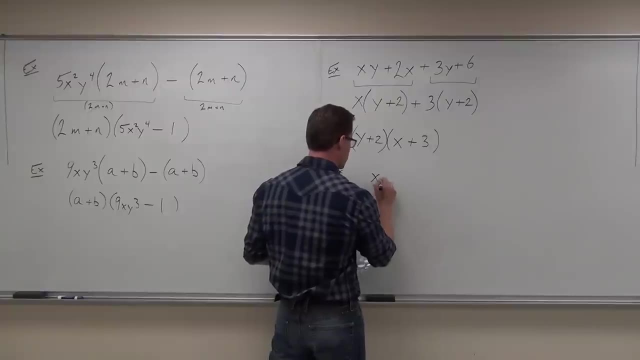 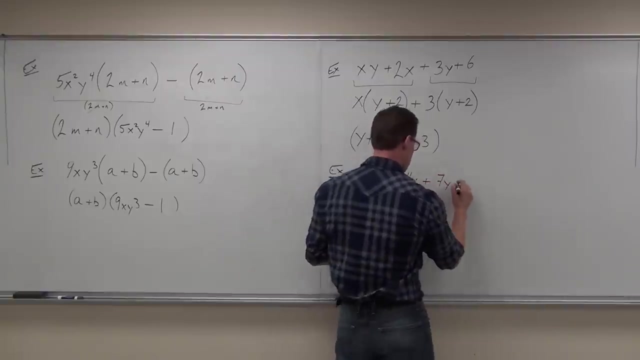 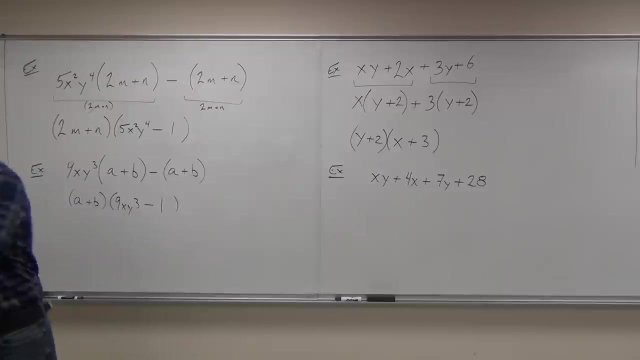 Let's try a few more examples to really get this solidified, and then we're going to move on. So for right now, I want you to try one on your own. I want you to look at this. Here's the thought process for going through these. The first thing: 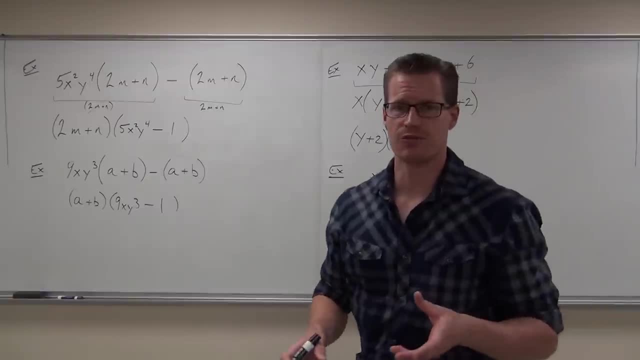 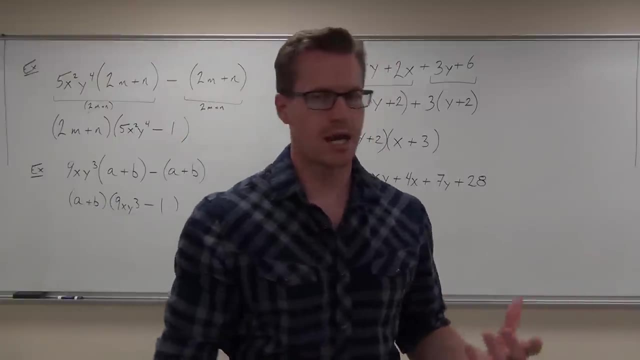 you do. you look at all your terms and you see if you have a GCF, because if you do you need to factor that out first. So factor a GCF if you have one for all the terms If you don't have a GCF. 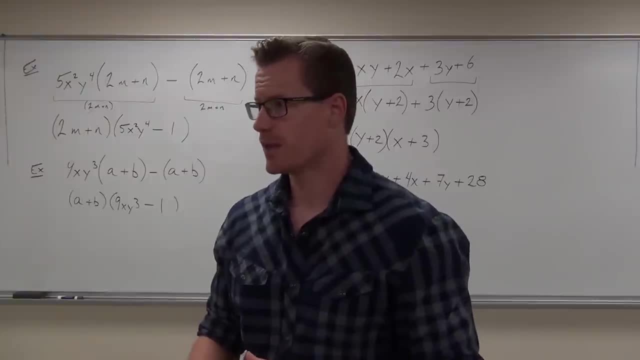 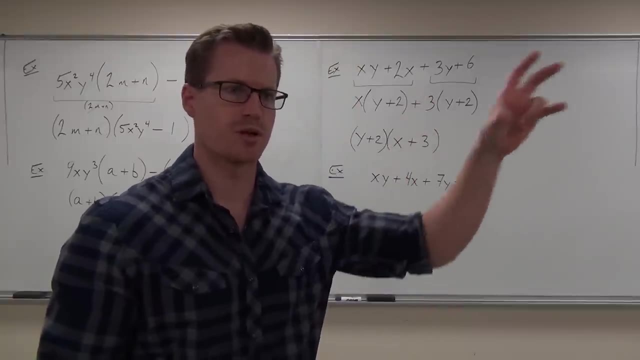 look at the number of terms that you have. If you have four terms, the only thing that we can really do here is factor by grouping. So you're grouping the first two, factoring it, Grouping the last two, factoring it, And then you're looking for that common factor. So go ahead and try to do. 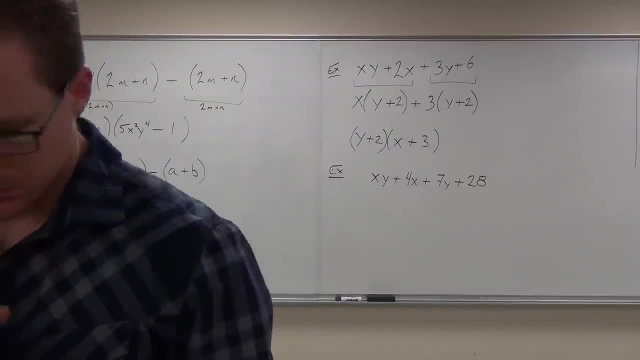 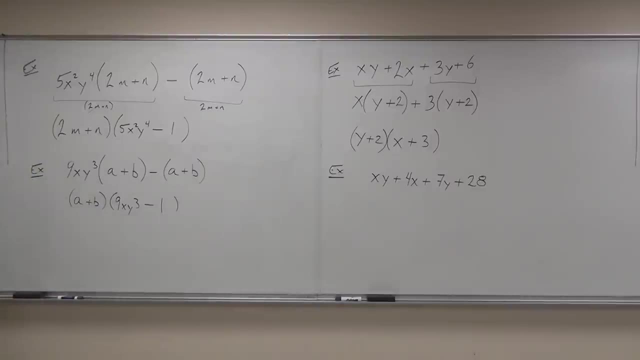 that problem for me, if you would Okay. So first thing, left side people: does this have a GCF for all four terms? What do you think? No, Yes, Yes. What goes into all four of them? Oh no, not for all four of them. 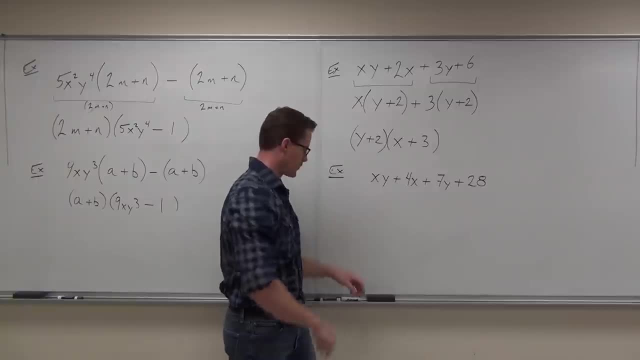 Okay, So that's the first thing we check for is for all four of them. does it have a GCF? Because you've got to do that first. If it doesn't, then we start looking at other options. Does that make sense to you? 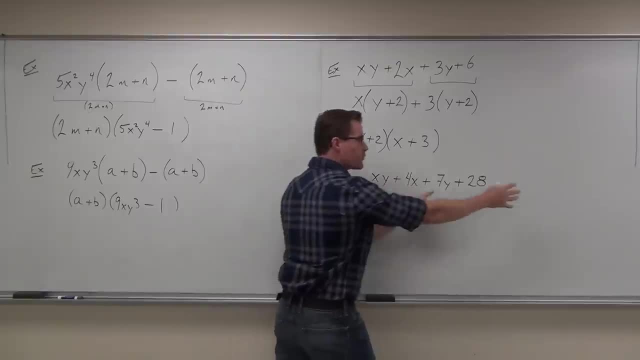 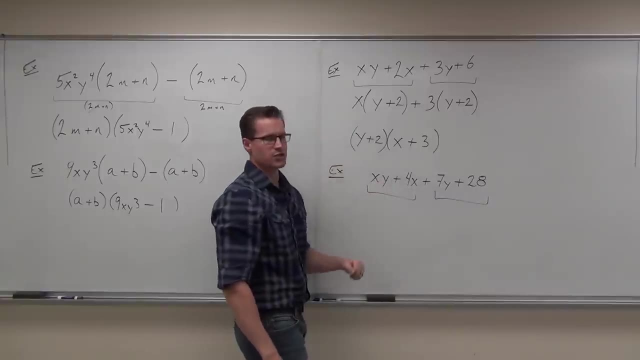 Mm-hmm. If it doesn't have a GCF, it's really important to look for all four of them at once, And then, if it doesn't have one, then we start breaking this up. Does the first two terms have a GCF there? 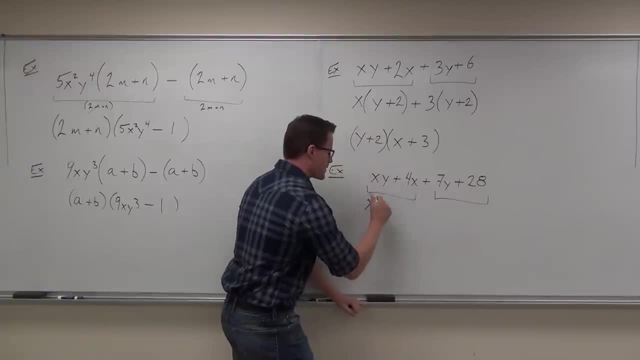 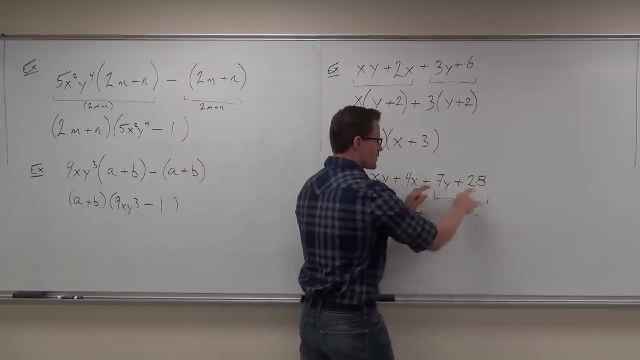 Yes, What is it? X? If we factor out the X, we divide it away, we get Y. Remember, factoring creates parentheses. Divide out the X, we get 4.. Good to go, Keep the plus Here. we have another factor that these two 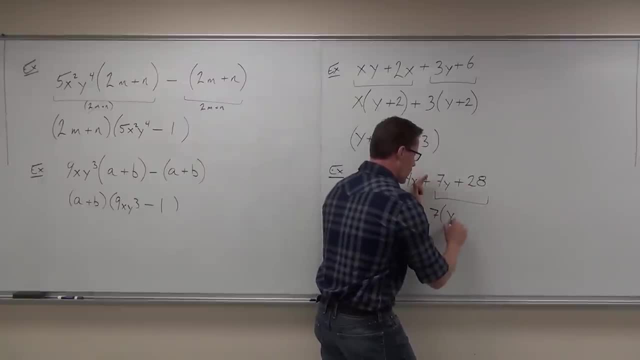 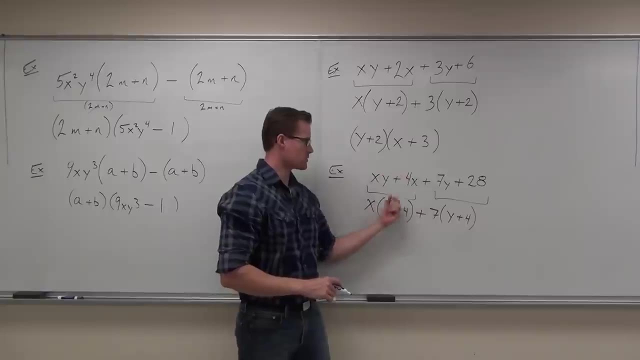 have in common, We have a 7. And if we factor that out, we get a Y plus 4.. We can double check our work if we wanted to, But that's the only way to do it. That's the only way to factor these two terms, and the only way to factor these two terms. 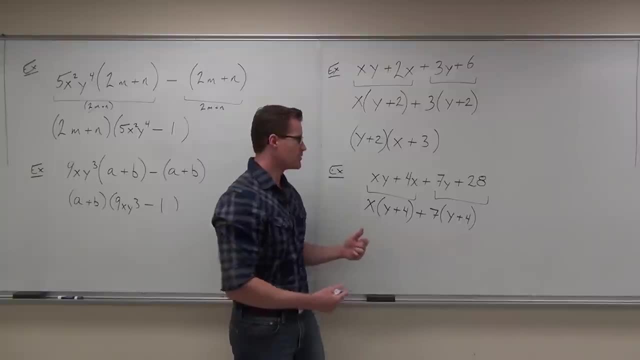 Quick head nod if you got that far on your own. At this point this is really nice. Now we've changed four terms into two big terms And then we continue. We look for a common factor within those two terms. So it's kind of doing like these two finding common factors and then another two terms finding common. 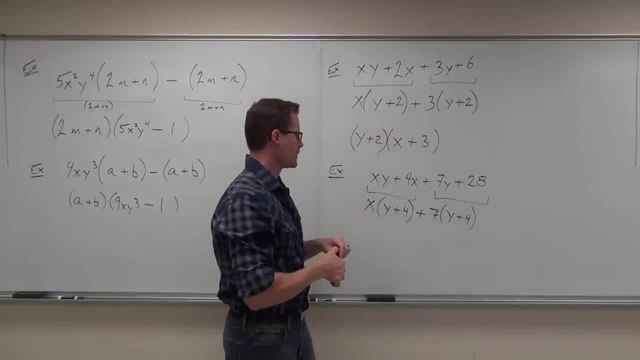 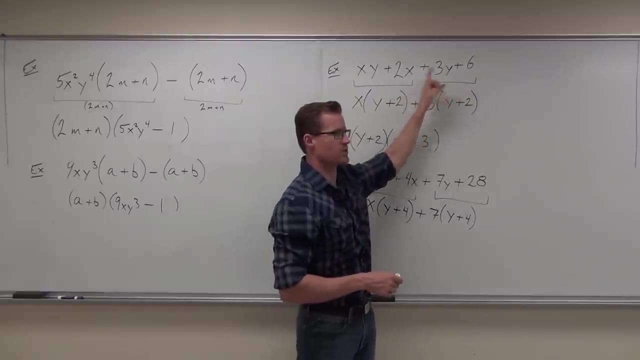 factors Question. There's two ways to do it. If you do the XY plus 7Y, it does the same thing. It does the same thing. That's right. Sometimes that's going to work. So you can see that 2 times 3 equals 6.. So no matter what way I have this organized, 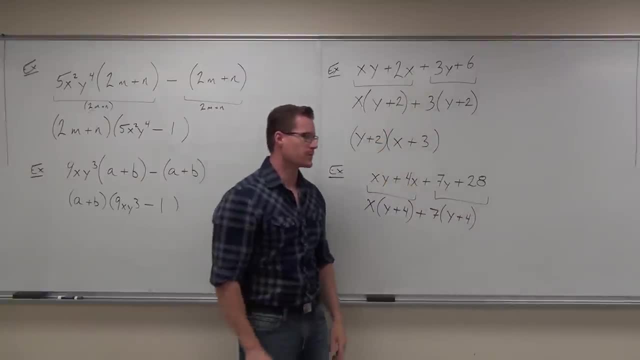 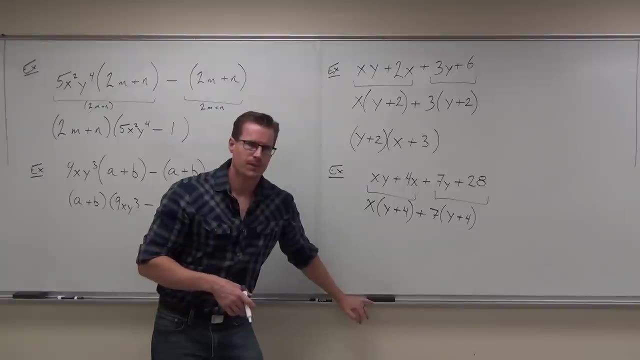 4 times 7 gives you 28.. It's going to work for you. Sometimes it won't. So if we continue to factor, can we continue to factor? Yes, How do you know? Because it has common factors. What if this was different than that? Would you be able to continue? 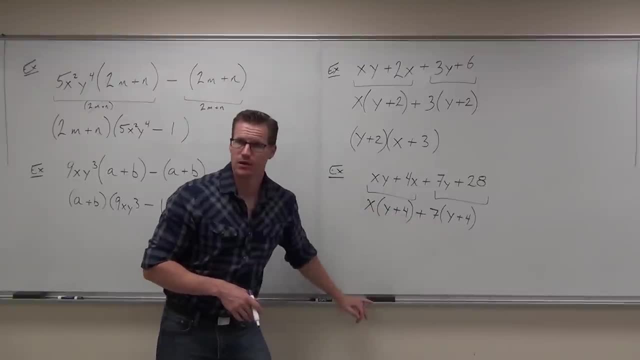 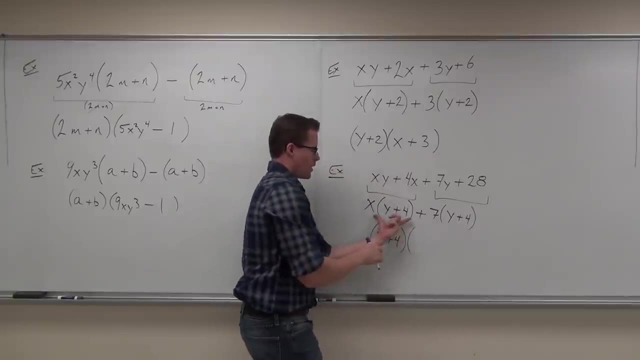 No. So if that's a plus and that's a minus, would you be able to do it? No, That's a problem. So here we factor out the Y plus 4.. If we factor out the Y plus 4 from this large term, what's remaining? 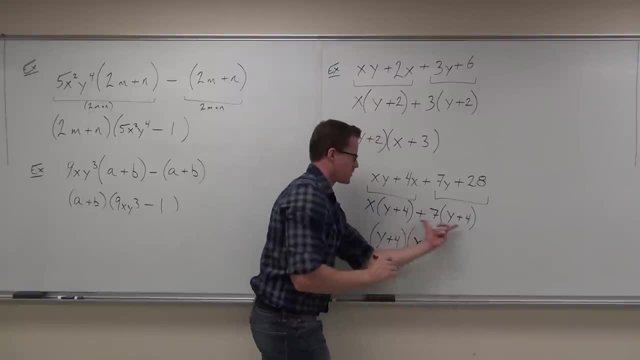 Plus 7.. If we factor out the Y plus 4 from this large term, what's remaining? Plus 7.. Good, I like how you said: the plus 7.. That's correct. Could you check your work? Yes, I'm not going to do it, but you just FOIL that out. It's got to be exactly the same. 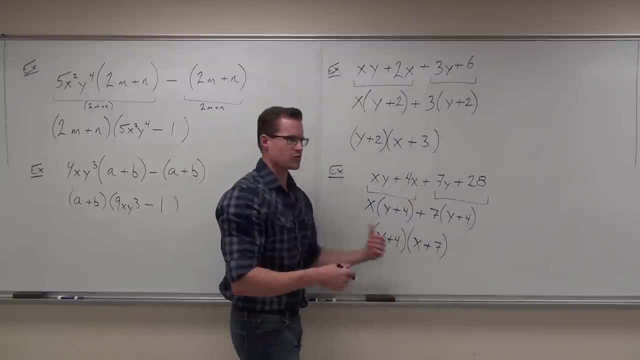 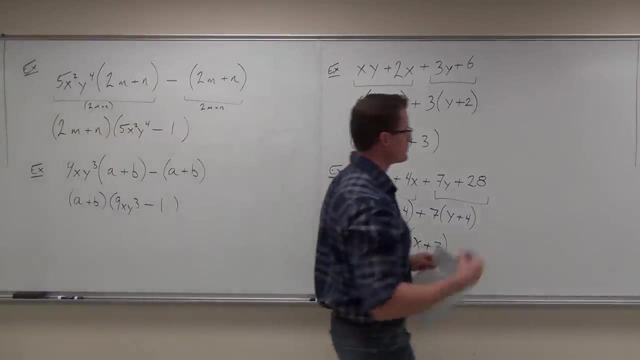 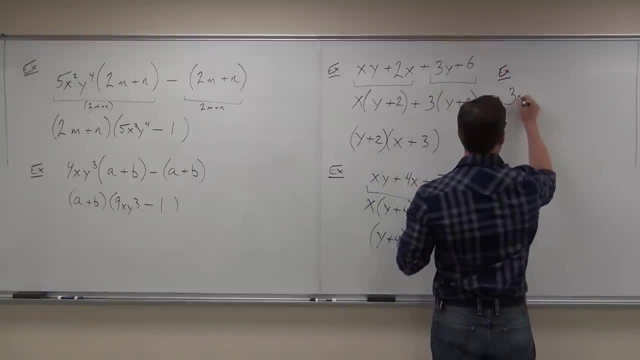 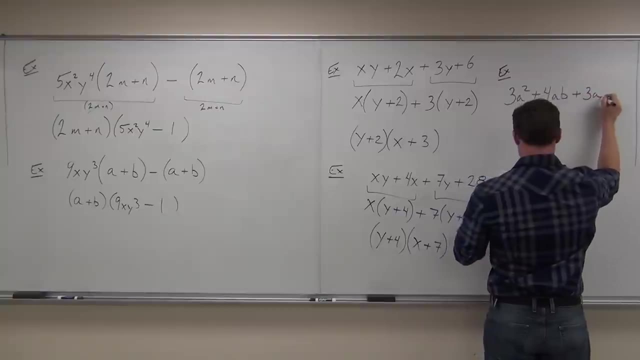 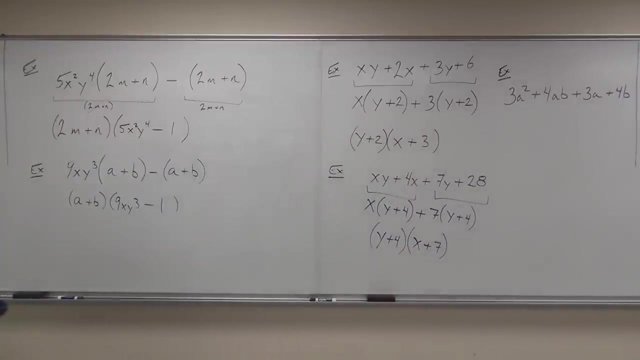 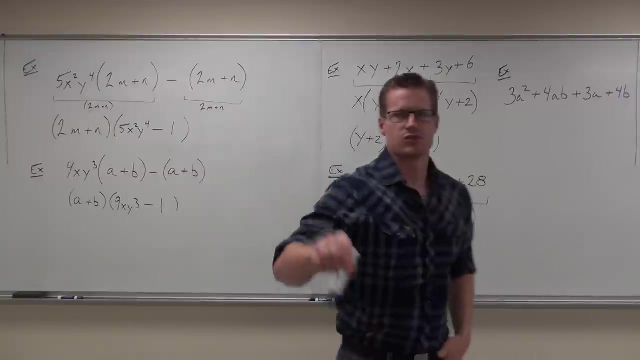 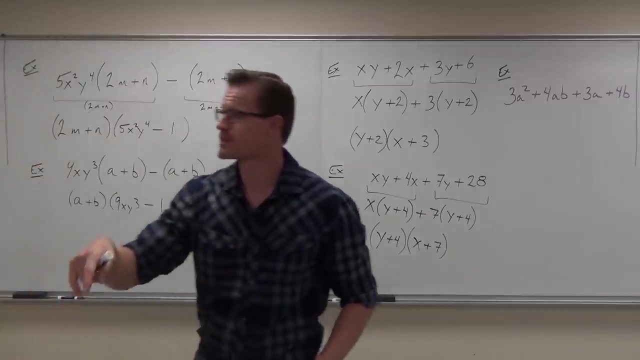 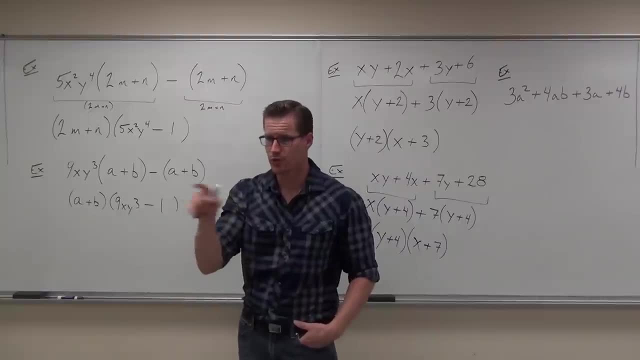 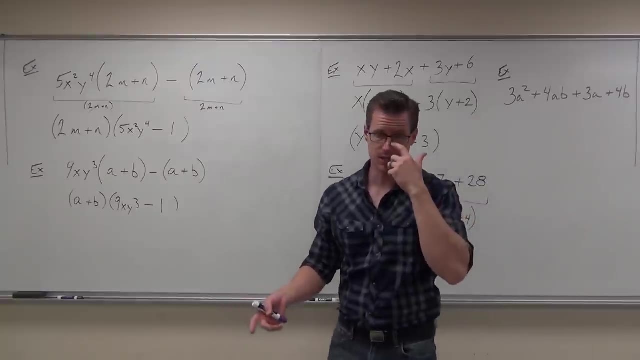 And in all four terms, is there a greatest common factor besides 1? for all those four terms, Anything go into all four of them besides 1.. Okay, Four first, but no, not in this case. So now that we have these four terms, 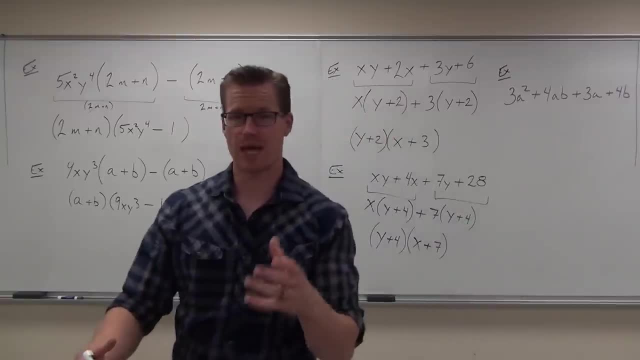 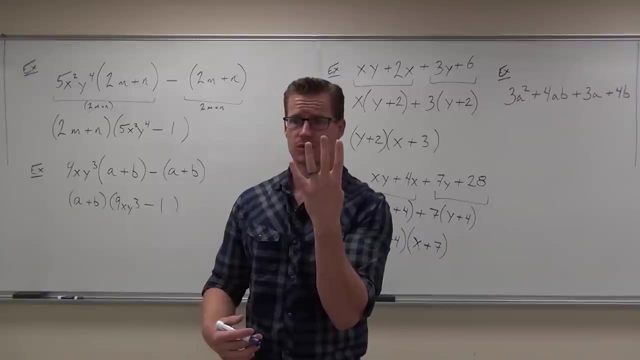 what's the next logical step? If we don't have a GCF, what should we be trying? if we have four terms, What should we try? Can you combine those? Are they like terms? Okay, no, So I'm trying to factor here. 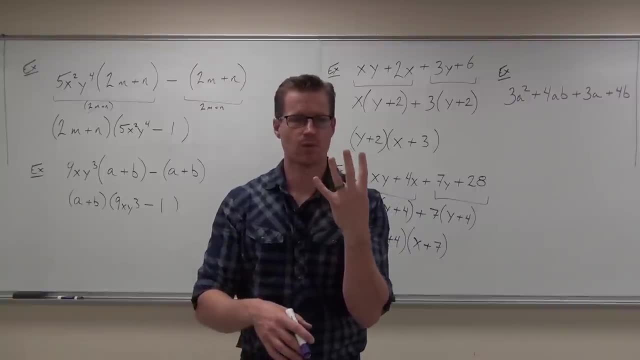 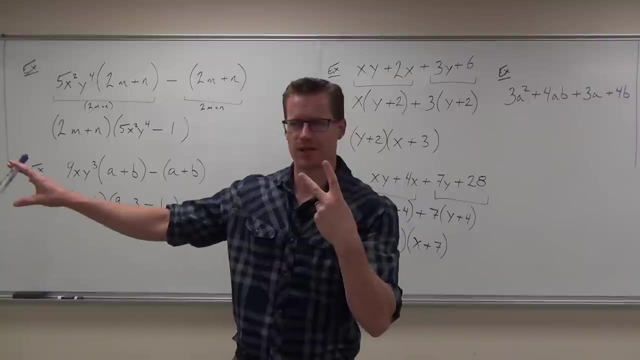 If I don't have a greatest common factor and I have four terms, the only thing we can do in this class is factor by grouping. So two terms, GCF, or some very specific types of factor. I'm going to tell you later. 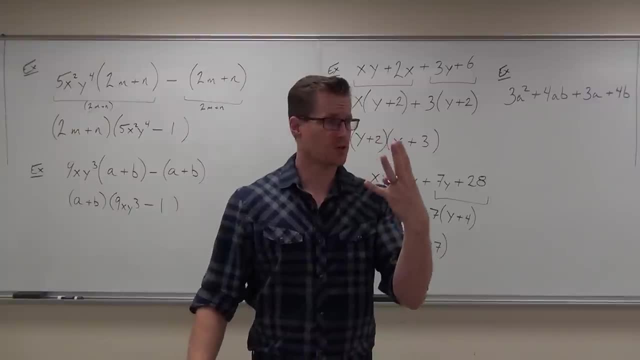 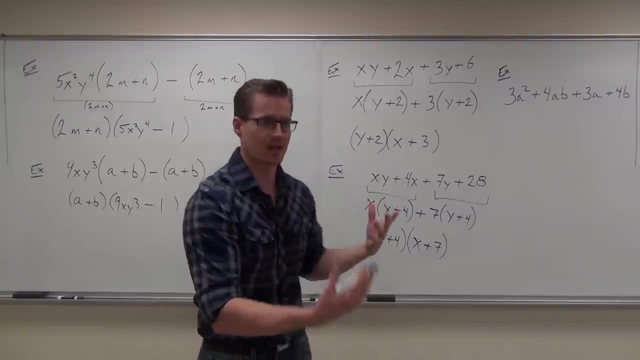 Three terms. we'll talk about that in maybe about 10 minutes. Okay, Four terms: GCF, but then grouping. It's all about factor by grouping, Because if you don't have the GCF, the only thing that we can do is factor by grouping. 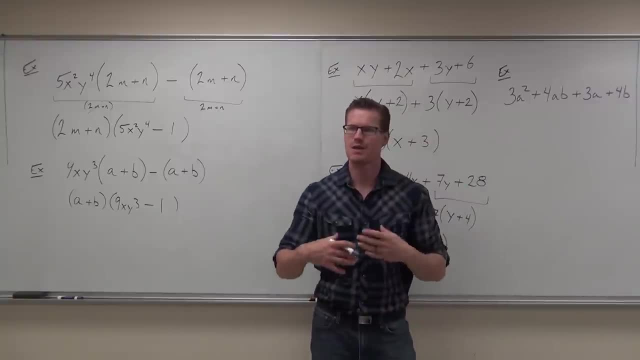 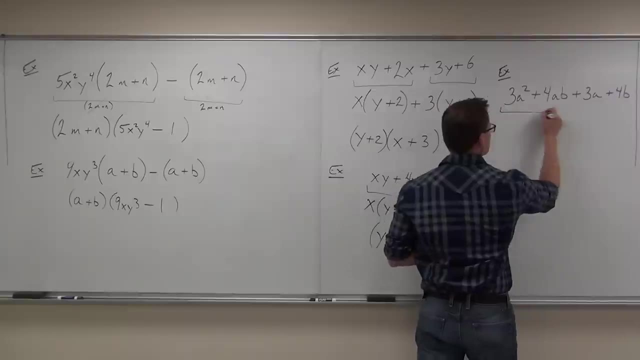 So I'm going to ask you one more time, With four terms: what's the only type of factoring that we do in this class? Factor by grouping, Grouping, Yep, we'll want you to try grouping. So we're going to group the first two. 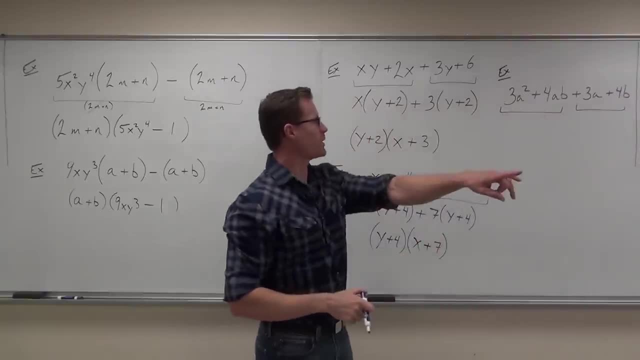 and we're going to do the next two And we're going to group the last two. Hey, tell me something, left-sided people. What goes into both 3a squared and 4ab? What's the GCF there? A? 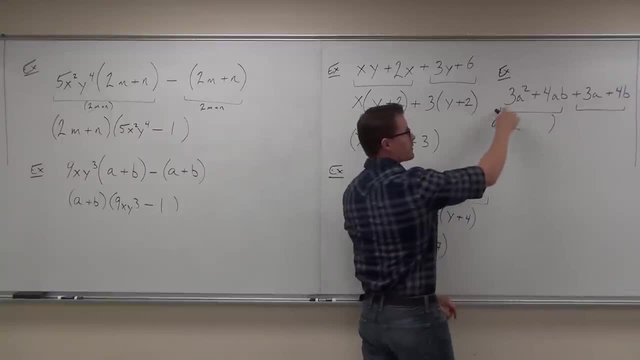 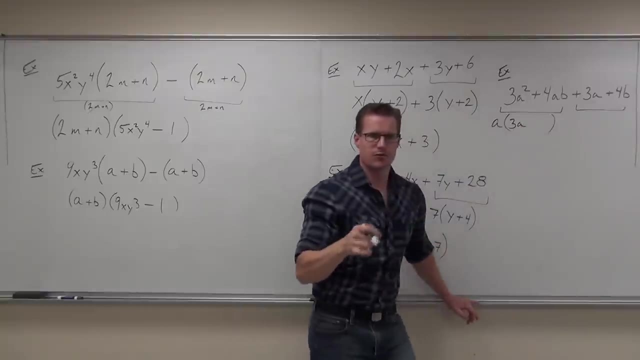 A, you're right. And when we factor that out, 3a squared, when I divide out 1a, what do I get? 3a, 3a plus 4b? Remember, I know I'm going faster right now. 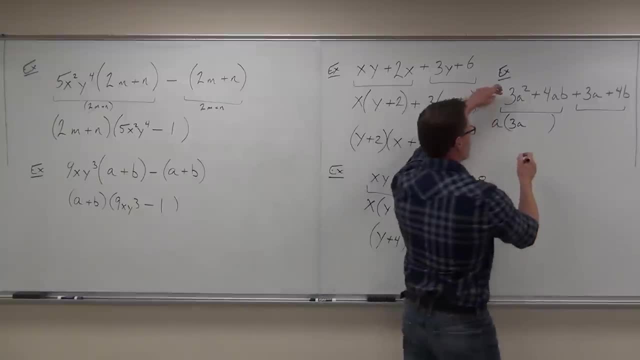 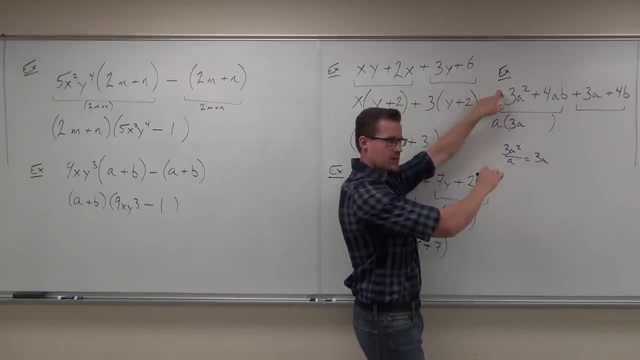 You can always write this out. Don't be afraid to do this and say: oh, he's factoring out the a. So 3a squared divided by a gives him 3a. That's how we're getting that. Do you remember that from last time? 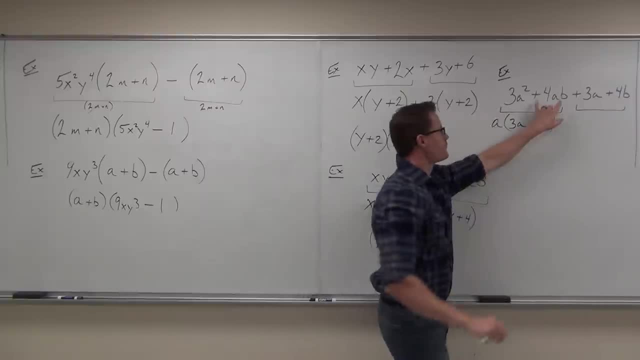 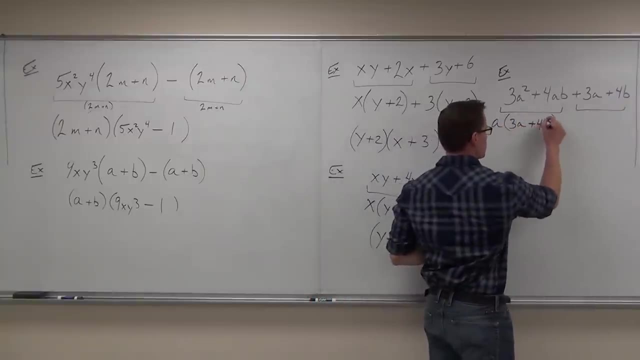 So don't be afraid to write that out. Okay, let's continue. How about 4ab? when I divide out that a, What do I get? 4b? And I'm going to get a plus between there. Quick head nod if you're okay with that one. 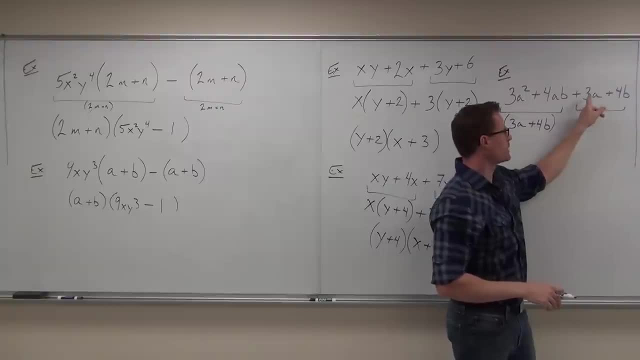 Now, this is a little weird, though. Wait a minute Over here We have 3a plus 4b. 3a plus 4b. What goes into both 3a and 4b? One Nothing. 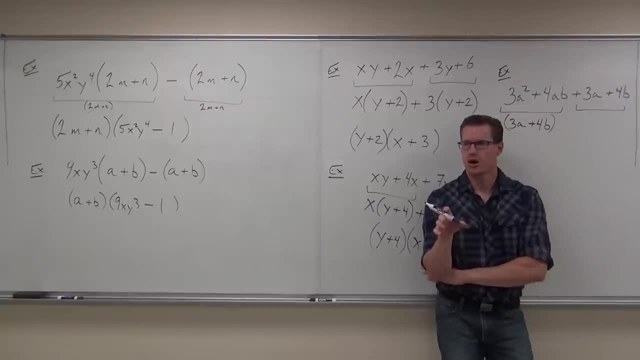 Nothing besides One One. If you have two terms which are automatically relatively primed- Remember that word Mm-hmm- We're using it a little loosely because we have variables here, but the idea is the same- Where these two terms have only the factor 1, when that's the case, write down the 1.. 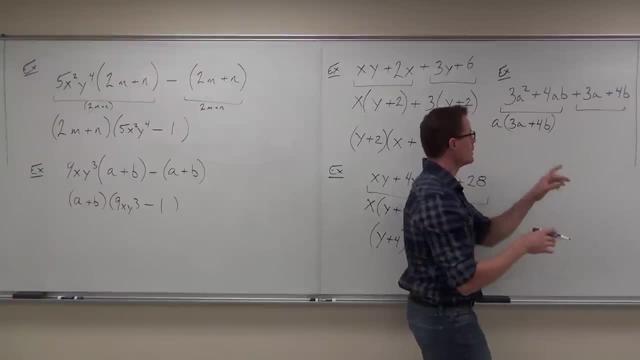 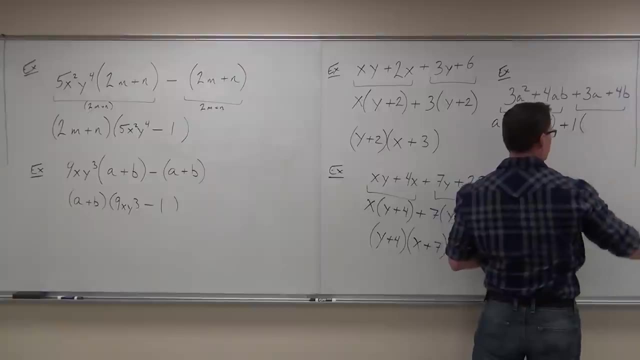 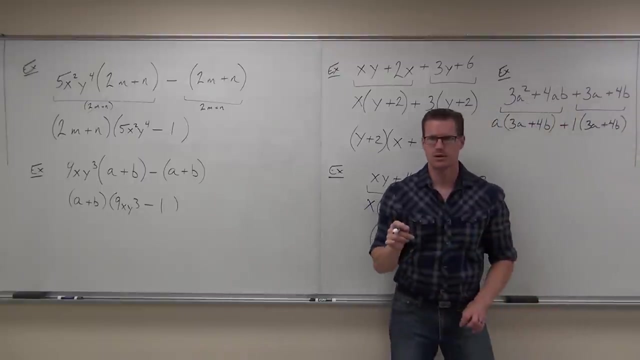 Force it to factor by 1.. I promise it will help you a little bit. So if we write down the 1 and factor this, we still have 3a plus 4b. I want you to verify that. I want you to verify that formula. that's still the same. 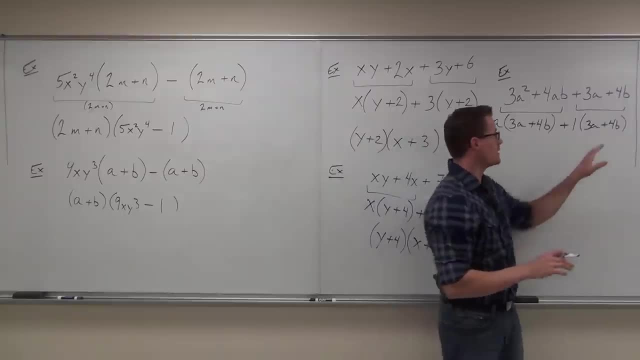 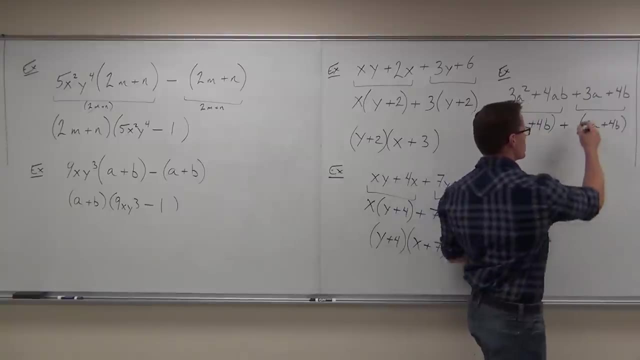 Is that okay with you? Mm-hmm, For some of you, if you don't like the 1, that's fine. If it does not factor, you can also just put parentheses around it, just like that. The reason why we do the 1 is because sometimes people struggle with this. 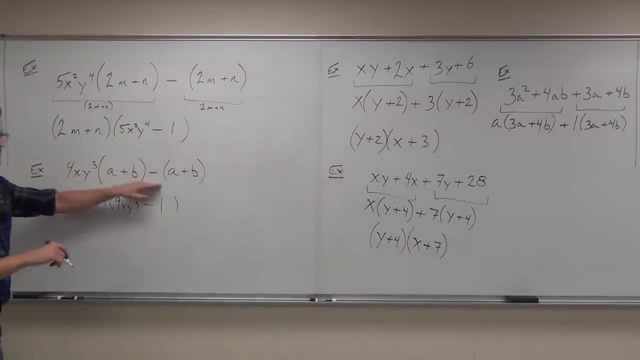 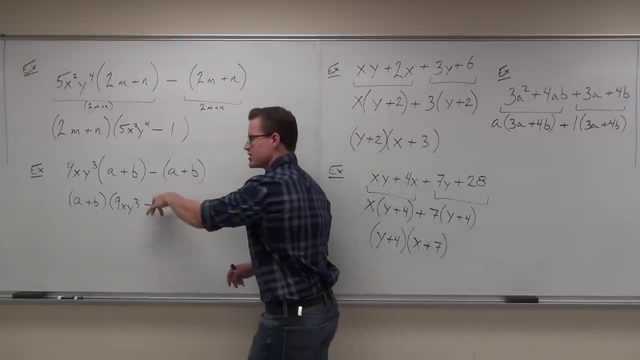 If you notice this, that problem is exactly the same as this problem, except instead of a minus you get a plus. Do you guys see what I'm talking about? So some people struggle that well, why doesn't that just disappear? 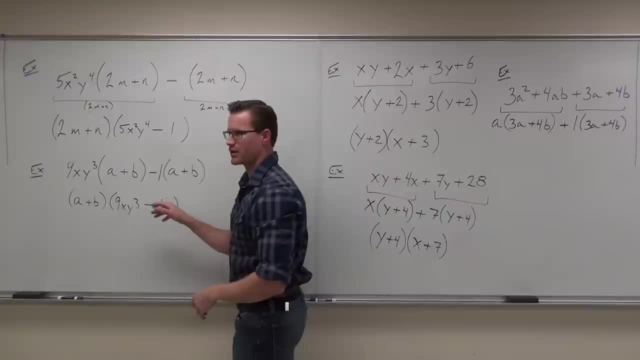 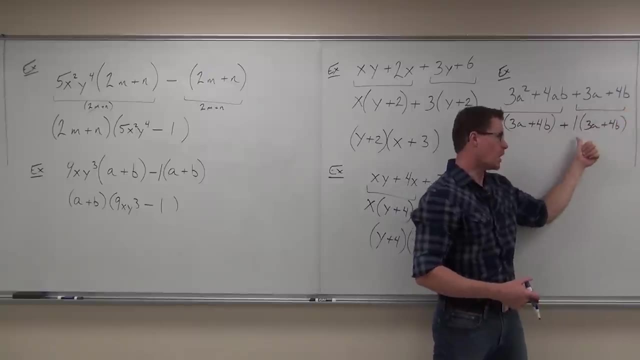 Why is that a 1?? Well, you can always put a 1 out front. So if you divide by this, you automatically get 1.. For some people, this really helps to say: the only thing that divides into these is 1.. 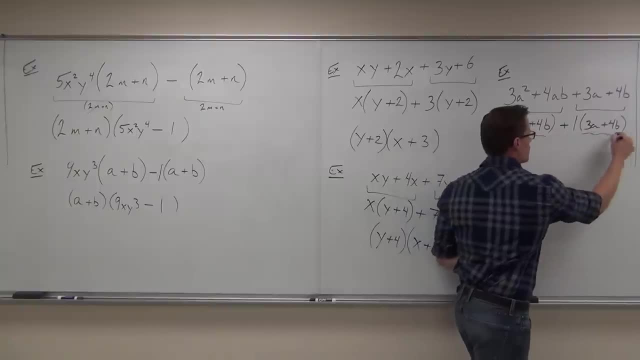 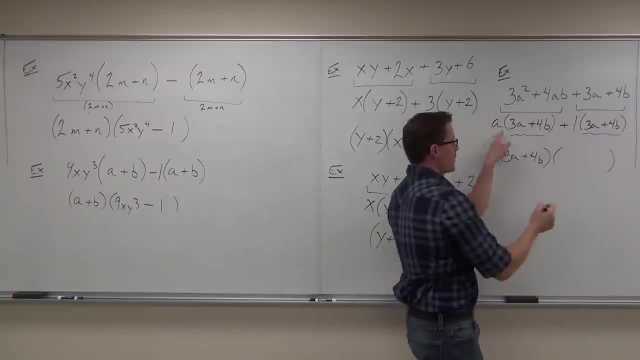 That way, when I factor out my greatest common factor here and here, we don't forget that we create parentheses- and we'll have an a and we'll have that. 1. A quick show of hands, if you feel okay with that one. 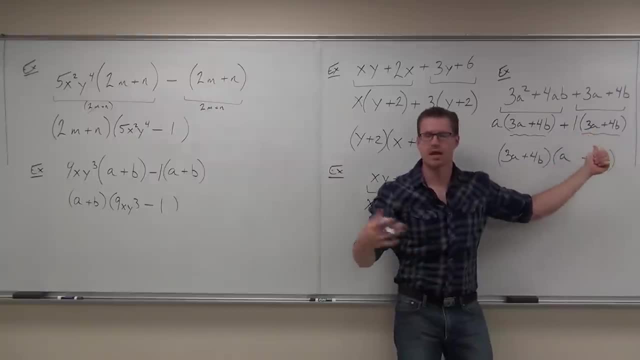 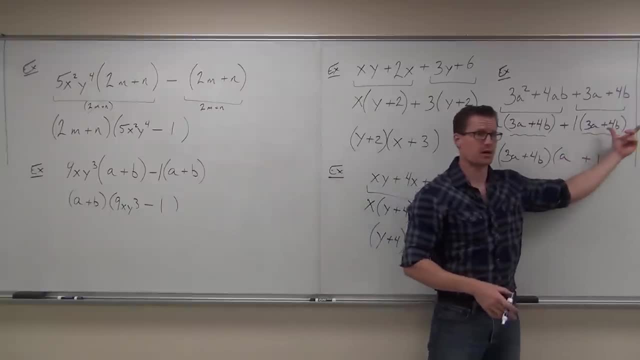 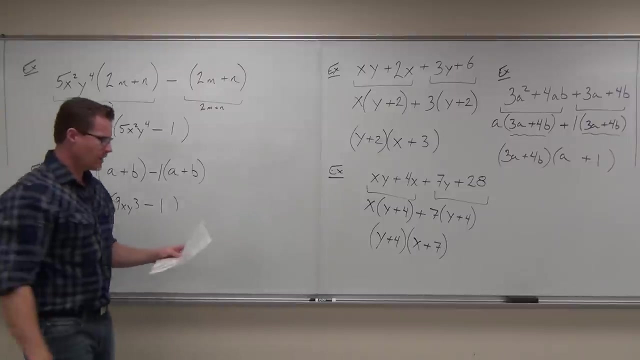 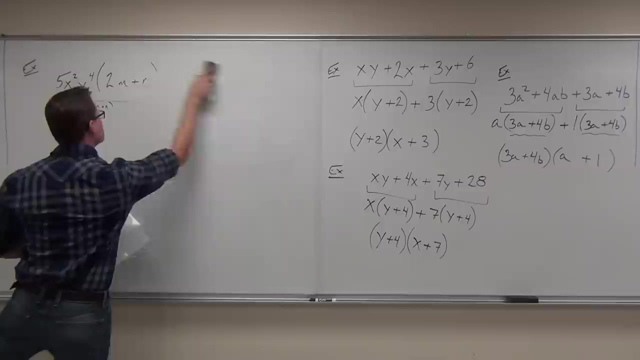 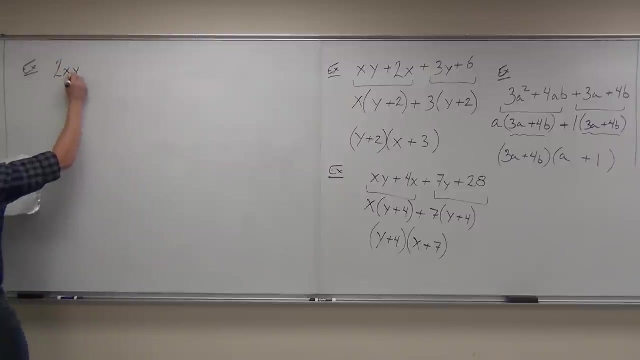 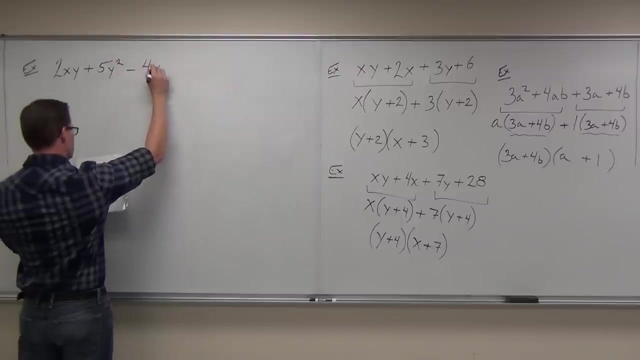 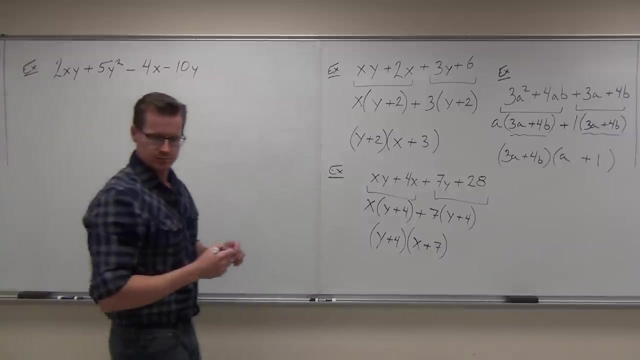 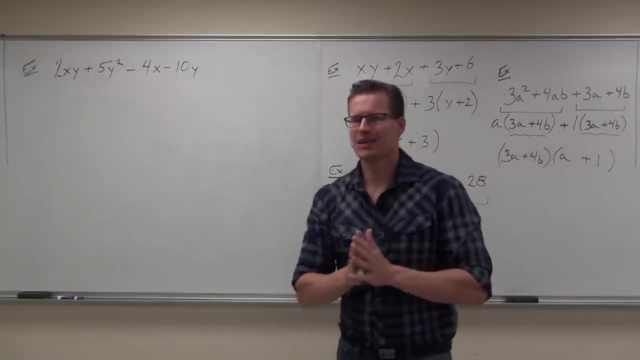 It's fine. It's fine, Okay. 10 and 5. 7. Okay, you know what? I'd like you guys to help me with this one? I want you to tell me what I I know how to do this stuff. I want to make sure you know. 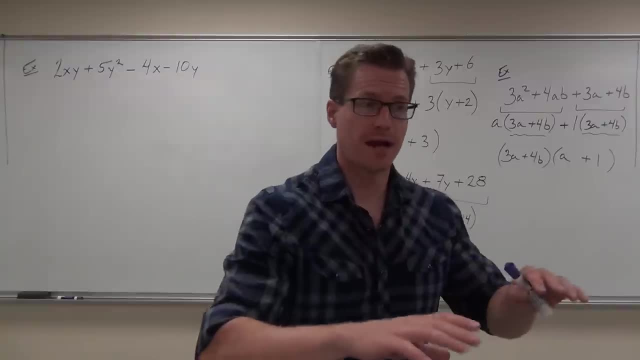 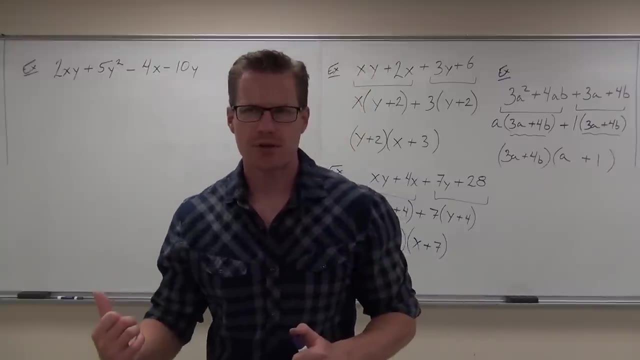 how to do it. So tell me what my first step should be When I factor, no matter what, all the time with factoring I'm always checking for what first. Very good, And how many terms does this have? Is there a GCF besides one that goes into all four of these terms? 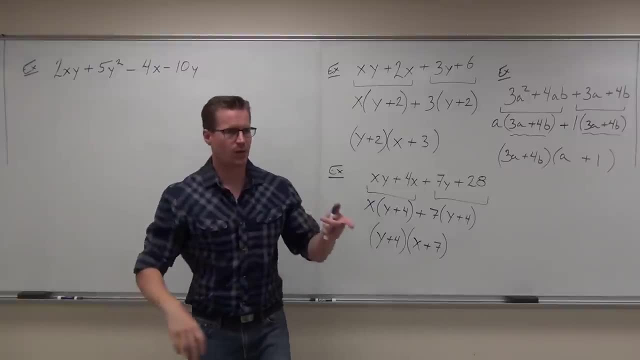 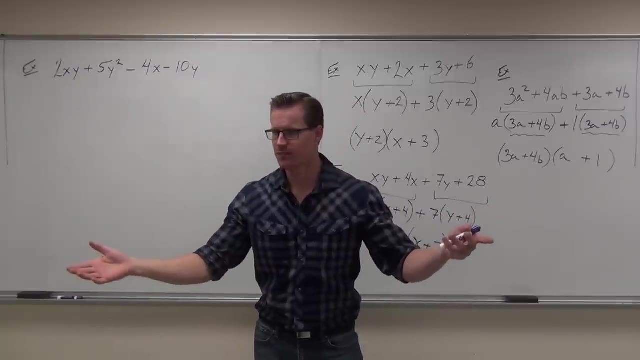 No, Okay, but we check first. Never ignore that. Now we have four terms. Okay, hey, if there's no GCF in four terms and you can't combine them, what do we use to factor it Grouping? 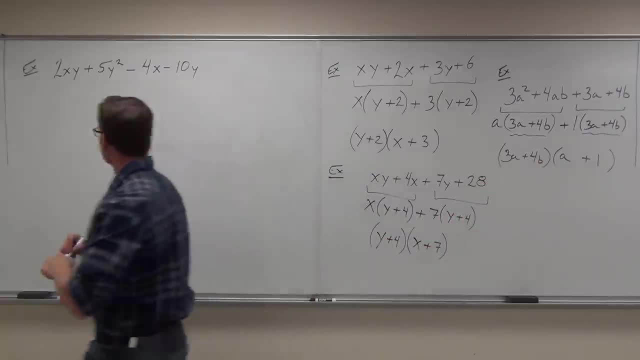 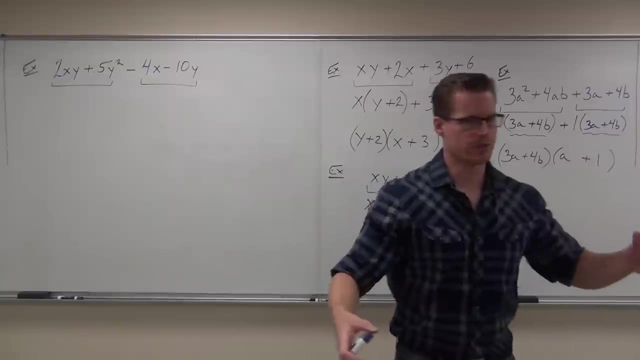 Grouping. That's right, Let's group them. So, after I've grouped the first two, we group the last two. Okay, we're on a roll. Now what do we do After I've grouped the first two and the last two? what's my next step? 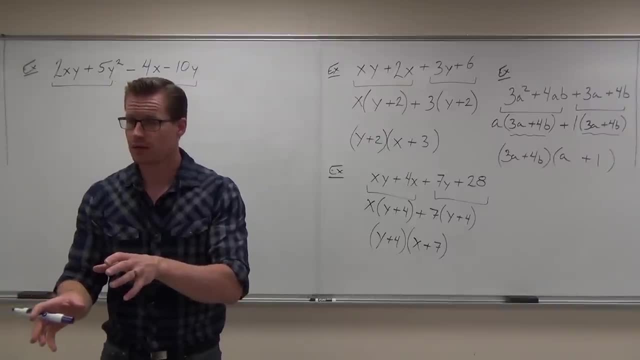 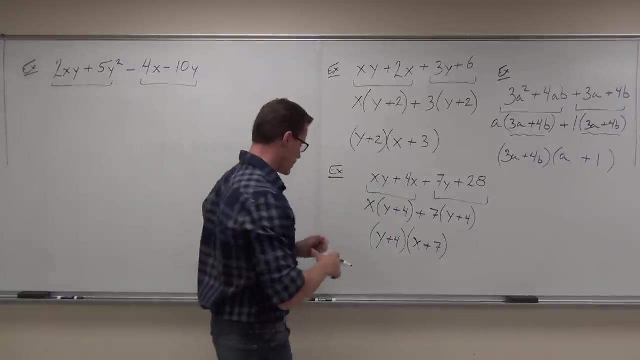 Factor, Factor what Each? Okay, so we're going to look at the first two terms and see if we can find a GCF just with those two terms, and then the last two terms and do the same exact thing. So, first two terms. can you find me something that goes into just these two terms? 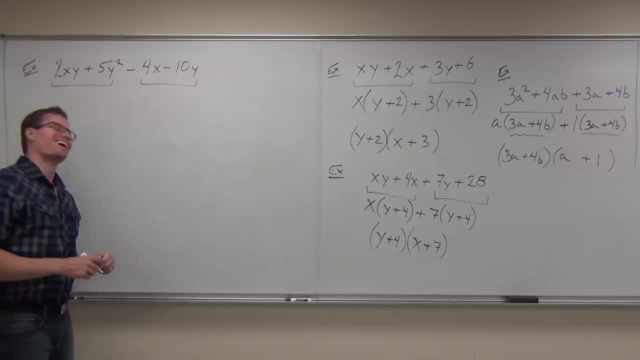 Why? Because I asked you Why. Oh, I used that joke already, didn't I? Yeah, Dang it. Oh, I'm unoriginal. now, Factoring creates parentheses. What's remaining when I factor? Remember: factoring just means divide. 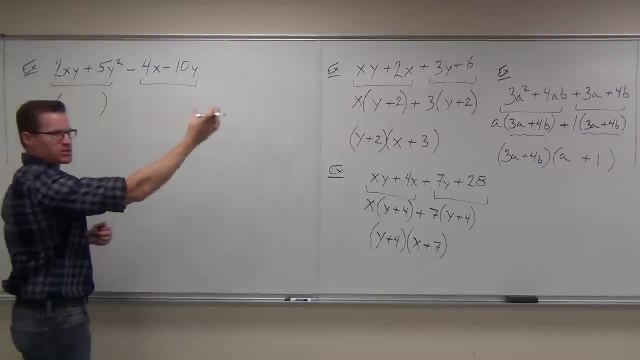 Okay, we're just dividing Two x plus five Two x. Okay, I like the two x. What's the rest of it? Five y, Five y. Very good, If I factor out or divide one y from this y squared, I get one y left over. 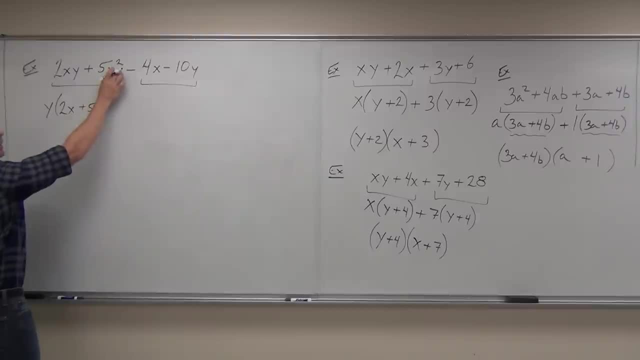 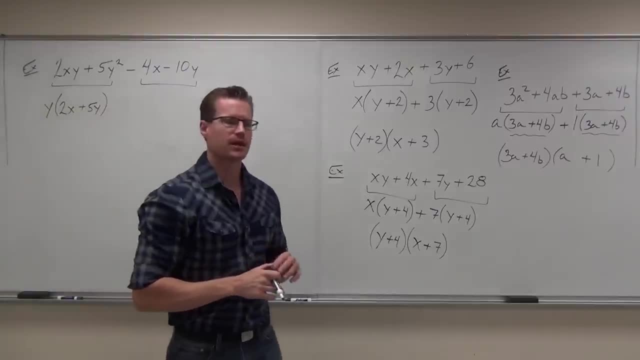 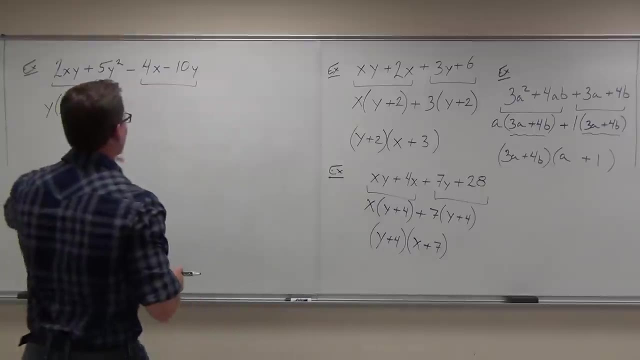 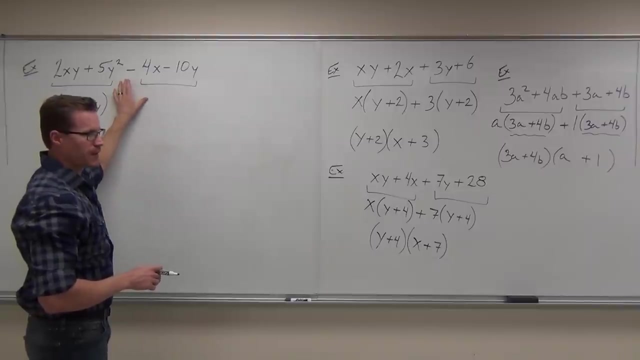 It's all about making mistakes. It's all about making mistakes. Let's talk about negatives. Whenever you have a minus, that is separating your two groupings, it's factored by a grouping. whenever you have a minus, what this is going to do, it's going to force you to factor out. 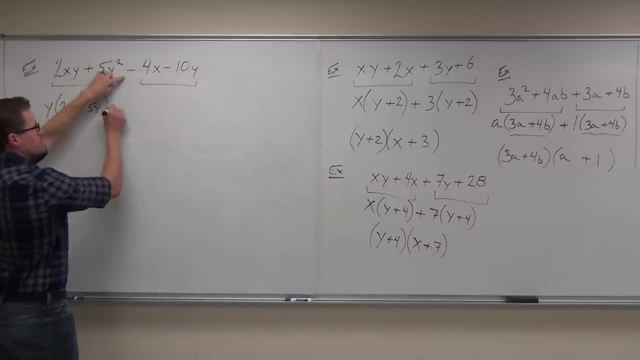 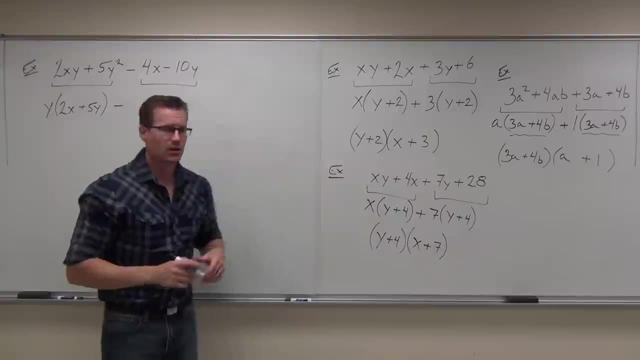 a negative. You have no other choice. So what that means: you write down the minus because it's a minus. You can't change that. What number goes into both four x and minus, or ten? four x and ten y? 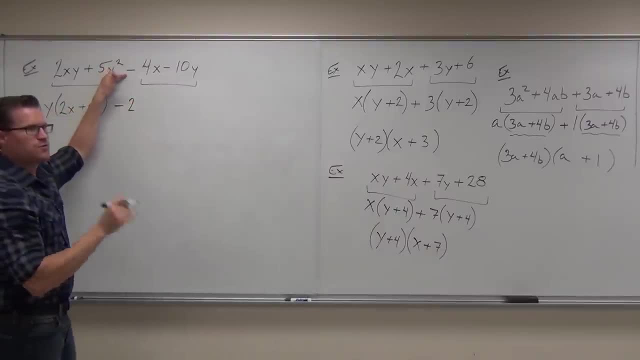 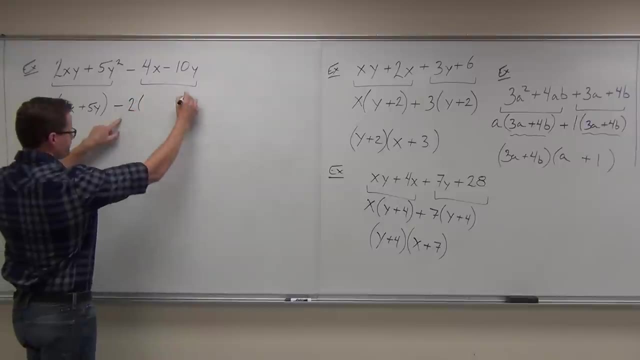 Two, Two. So because that's a minus, it is going to force you to factor out not just two, but negative two. What that's going to do? it's going to change your signs. So do you guys see what I'm talking about? the negative two up there? 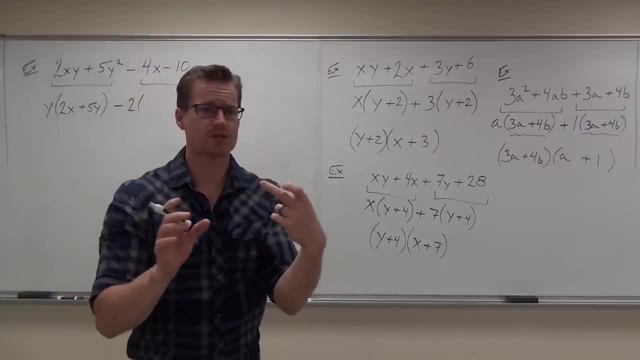 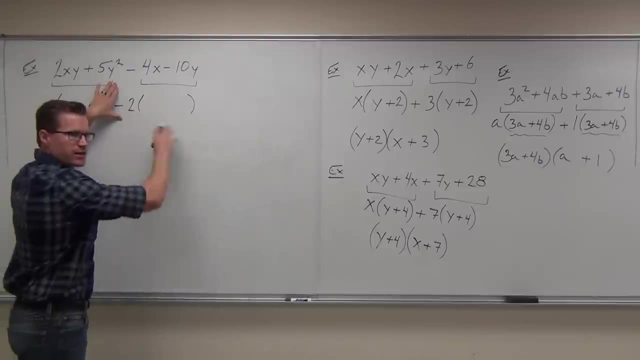 We always know that numbers go with the sign right in front of them. So right here, when we're factoring out two- not really We're factoring out negative two because of that minus. So when you do this, when you find out your terms, please don't just divide by two. 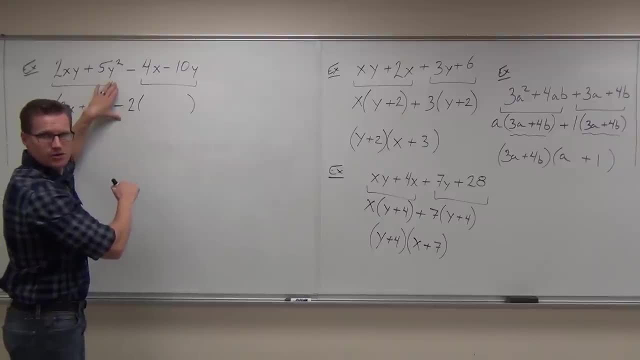 You need to divide by. if that's a negative, divide by negative two. I don't know if you understood it, Okay, so let's do it. What's negative? four x. Remember we always go with the sign in front. 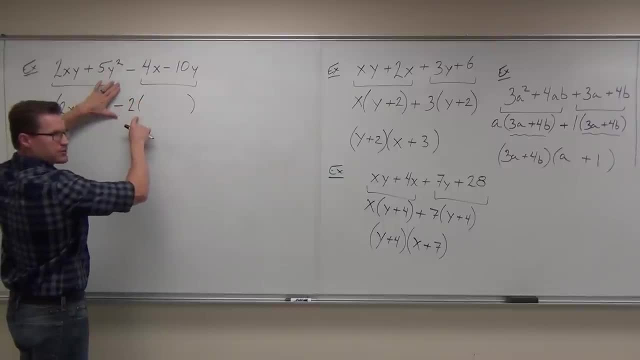 What's negative four x divided by negative? two, Two x. Positive two x, isn't it Okay? What's negative ten y divided by negative two, Five, Five y. Aha, Do you know what? I'll bet you know. 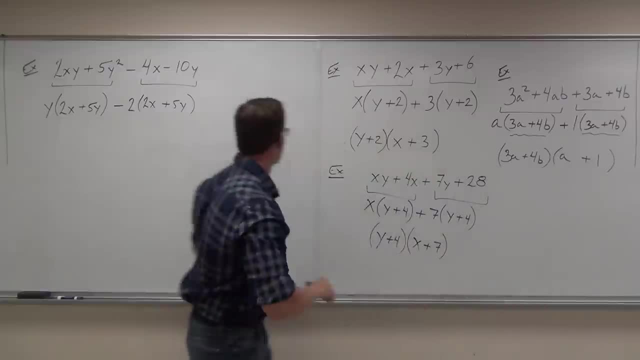 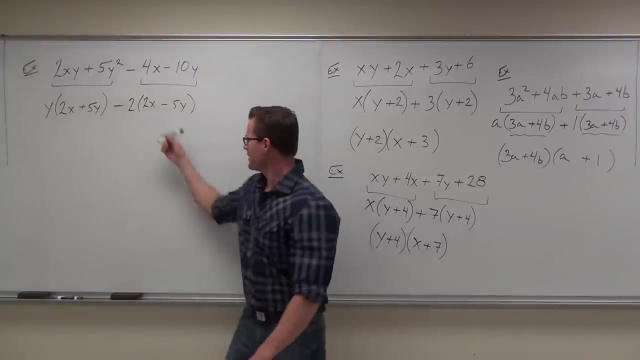 I'll bet you know what most people are going to do here. if they're going to make a mistake, What's going to be there? Yes, Mr Leonard's method. don't work with crap man. That's why I like this. 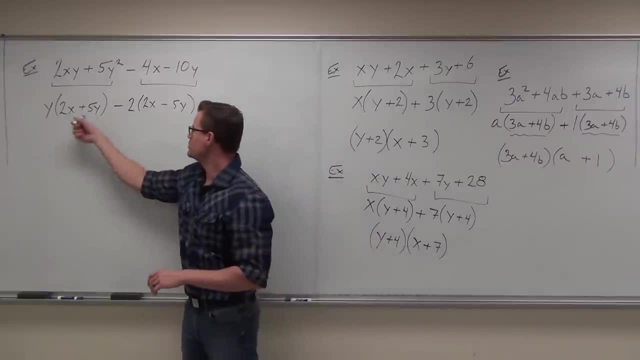 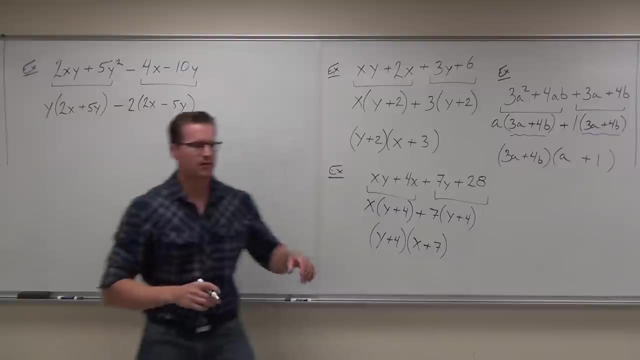 Because it's going to be different. If you mess up that negative, can you continue with this problem? right now? That's a problem, So it's really imperative that you understand that. if there's a minus right here separating your two groupings, it is forcing you to factor out a negative. 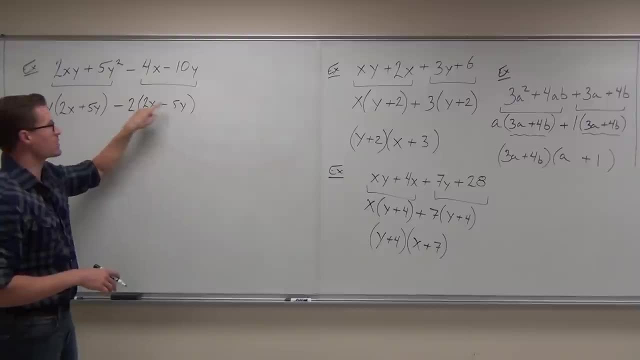 All that you need to recognize is: hey, minus, both these signs are going to change. That'll be positive. That sign will change Plus, Just like that, And what that's going to do is make this at least doable for you. 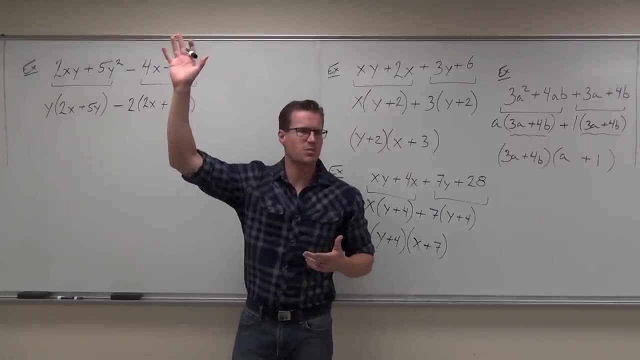 Show of hands if you understand the idea there. It might take some practice to get used to the idea. But if you mess up that negative, can you continue with this problem? right now That's a problem. So you get used to the idea that minus means factor out a negative every time. 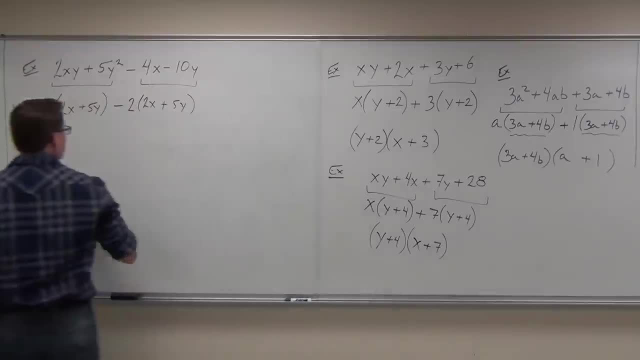 Plus. Don't worry about it, Just factor out the positive, It's all good. So now that we have this- oh man, we got one big term, We got two big terms. Do you see a common factor in there? 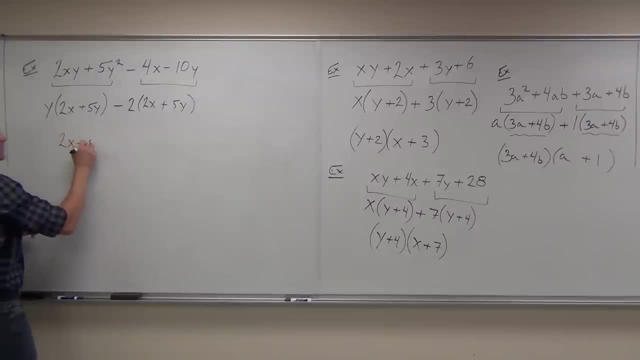 Yes, Let's write our common factor first. If we remove that common factor by division, ie we're factoring. If we remove it, we have a y, If we remove it, we have a minus 2. And we're completely factoring. 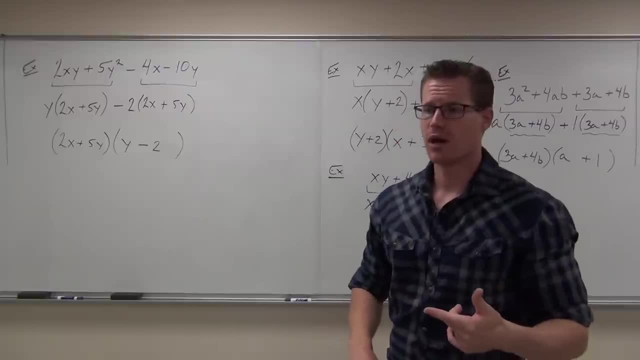 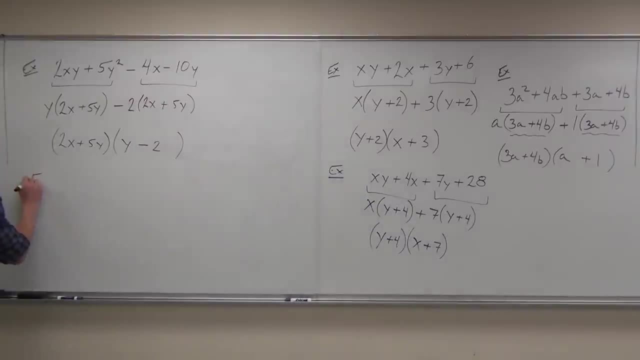 And that's nice. Well, I'd like you to do it now. I'm going to have you try two of them. OK, I'll be walking around. If you need help, now would be the time to ask, So let's put one right here. 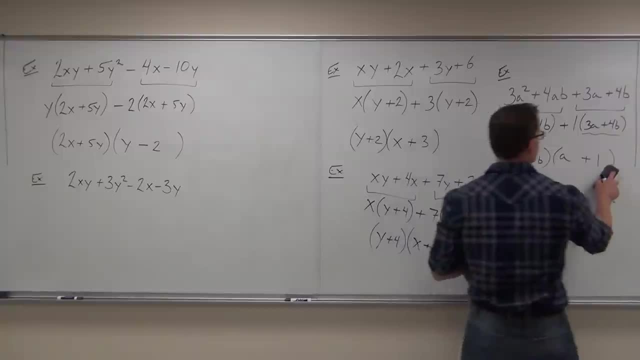 So we're looking at the total number of terms and figuring out if we have a GCF, If we do awesome, Factor it. If we don't have that, then we count the negative. That's fine, Then we count the number of terms. 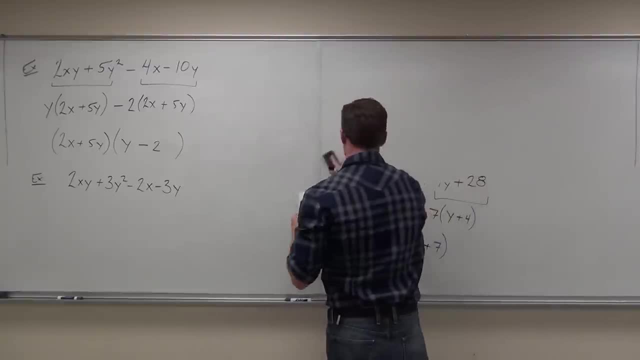 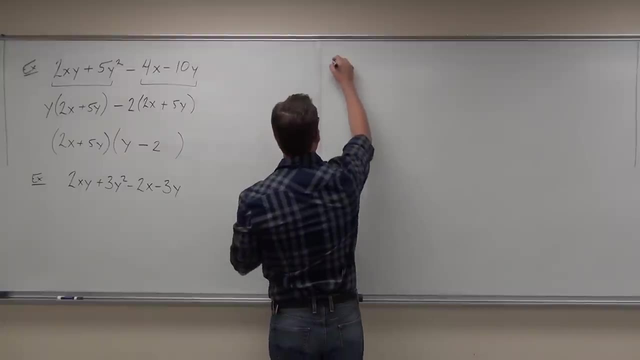 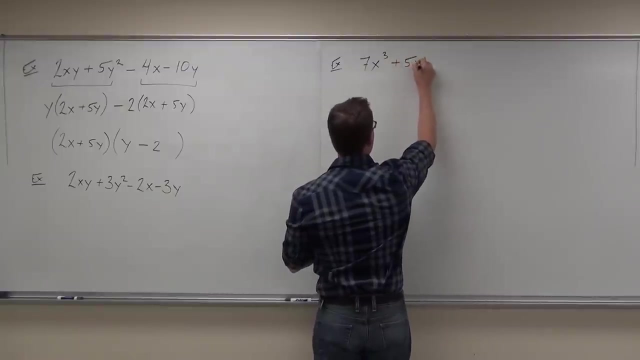 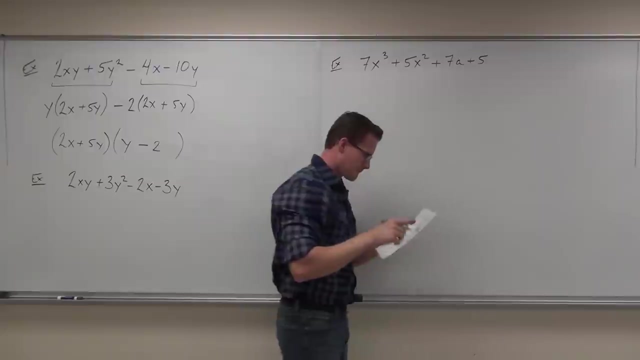 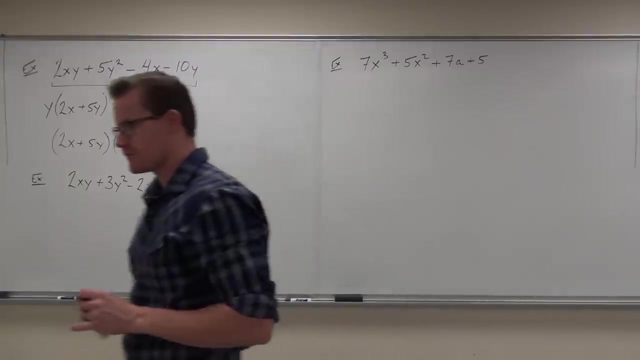 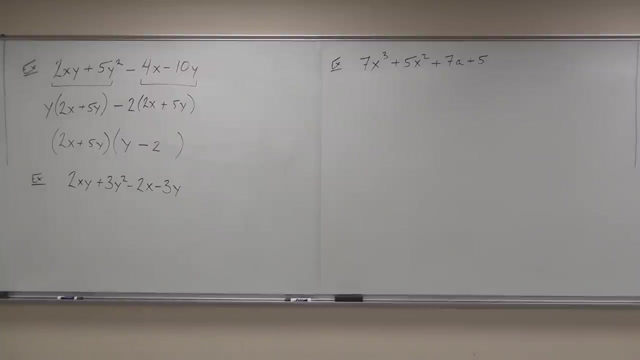 And if there's four of them, we have to factor by grouping right now. Thank you, Thank you. I think I made a mistake on that one. I think so too. What you guys can't figure that out, Come on. 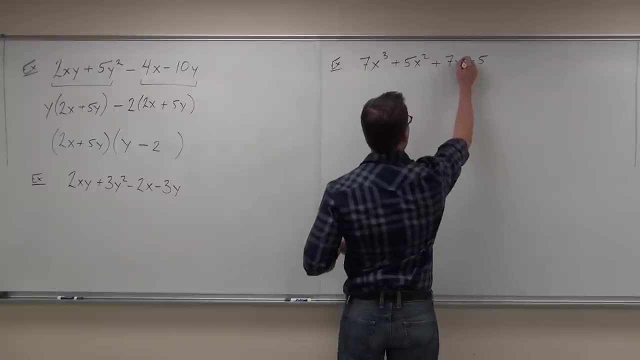 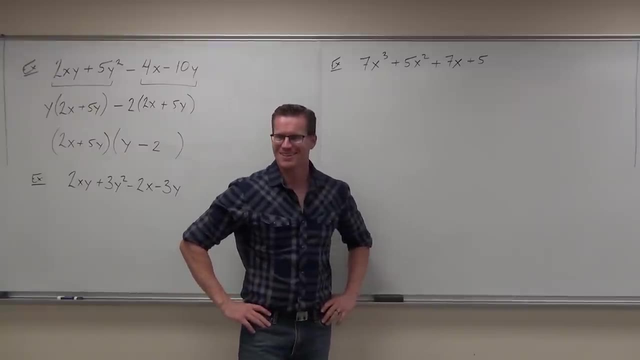 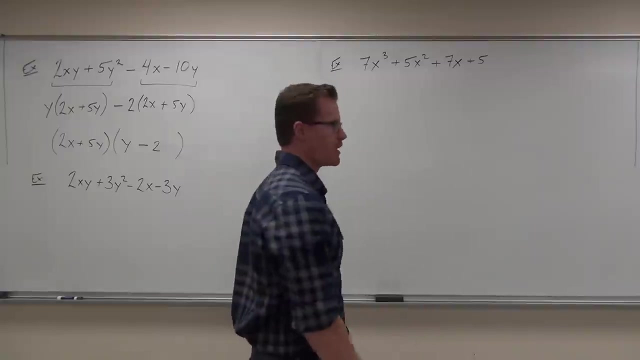 It's going to be easier. That's next right. All right, I mean, I tested you, You passed, Congratulations. If you had done that problem, then you wouldn't be able to go any further, right? In fact, you might have failed. so it's good that we see that. 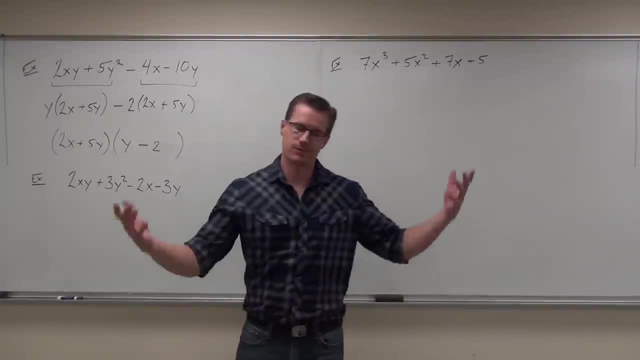 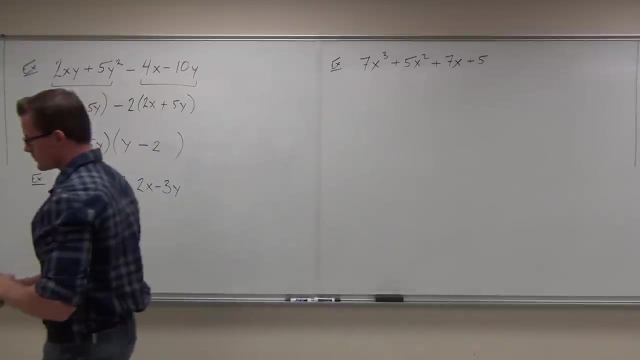 But you try, You try with four terms, And if that happens you go. Well, I just can't factor it. That can happen too. Okay, so I'm assuming that, since you're working on that one, that you guys finished up this one. Is that true? 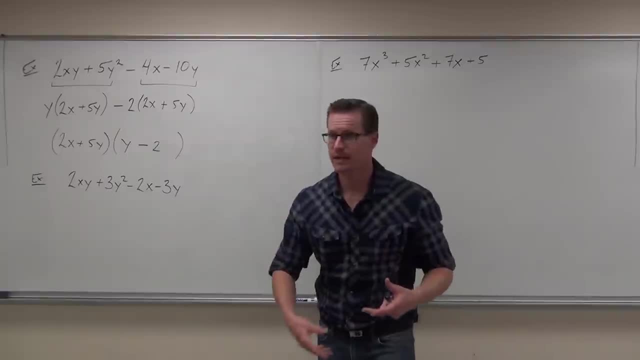 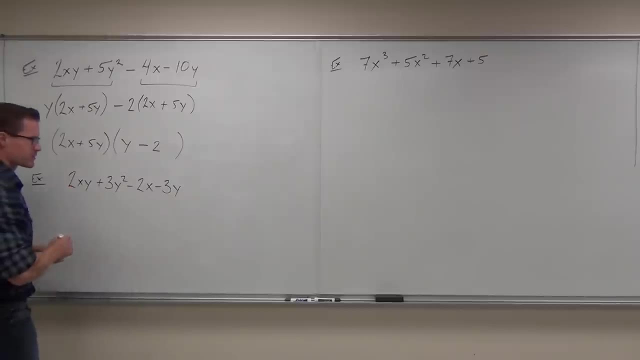 Yep, Okay, I'm going to go through it a little bit quickly, since we should have this idea pretty much down at this point. So we look for greatest common factor. They go: Oh, x is here, y is here. Nothing for all three of them. 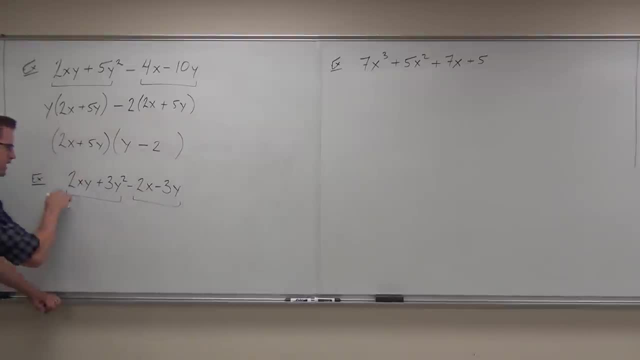 So I'm going to factor by grouping, because I have four terms. I look here I see a factor of y, That's the GCF for these two terms. Factor means create parentheses, It means divide out that greatest common factor. So we've got our 2x, We've got our plus 3y. 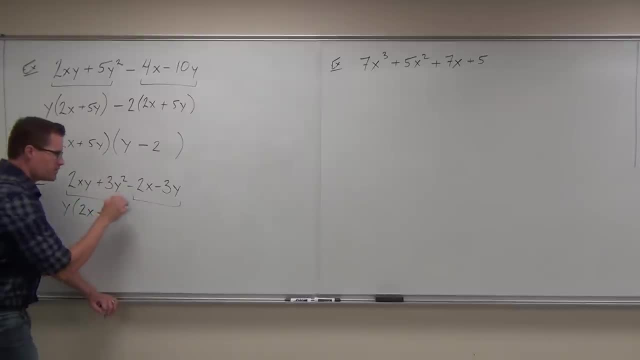 We never lose a term. We always have the same number of terms here. That minus is going to force me to factor out a negative something. Now, the only number that goes into both these two terms is what One? That's right. 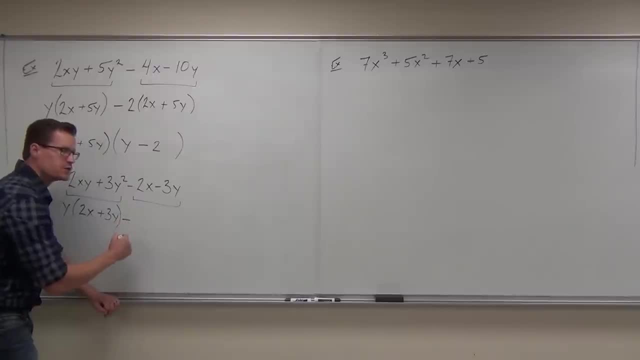 I can put the one if I want to. I don't have to put the one, But what I do have to do is somehow make parentheses. Now, if you're going to factor out negative one, basically I like putting the one because it reminds me. 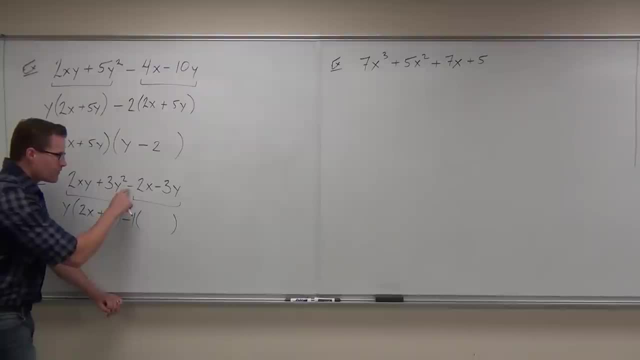 that I'm going to have something down here, not just nothing. So if I factor out the negative one, all that's going to do is change this sign to a positive 2x and change this sign to a plus 3y, And you can verify that really quick. 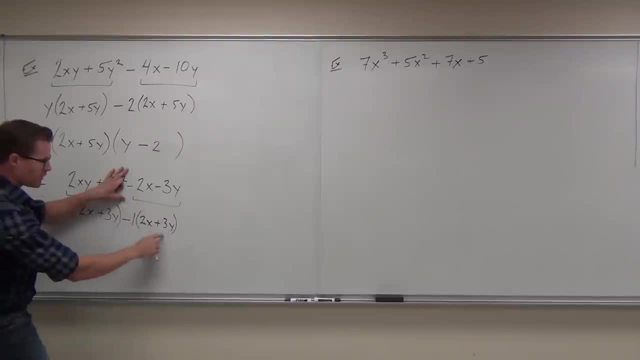 If I take my negative one and multiply negative 2x, negative one and multiply minus 3y, So we know we have it right Now we look at a two large terms, a common factor. We write our common factor first. 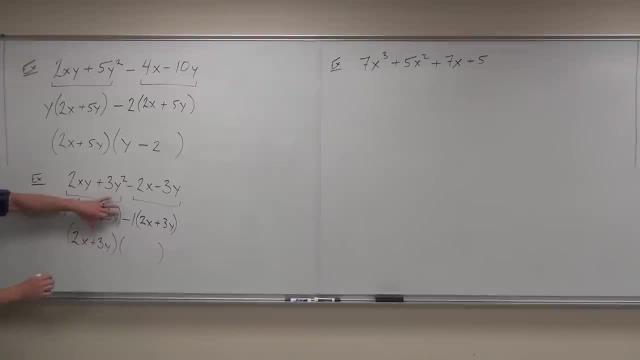 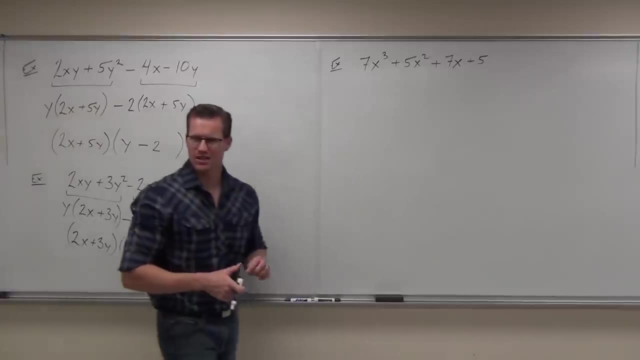 We create some parentheses. If we remove by division, factor it. If we factor this out, we have a y from that term. If we factor this out, we have a minus 1, and that's the correct factorization. Did you guys get that one? 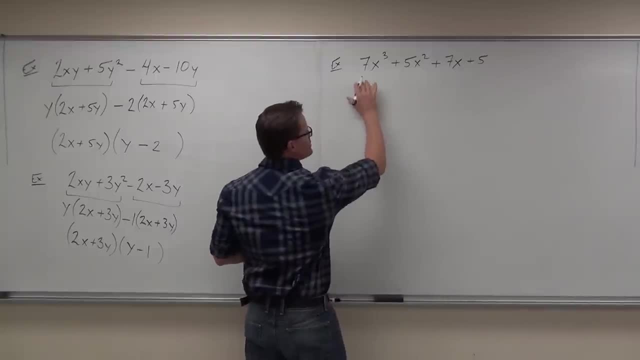 Same thing happens over here. It's just a little bit different because we haven't seen this larger variable here. No GCF, but we do have a larger greatest common factor than we normally have. What goes into both those terms? Square? You've got to factor out the x squared. 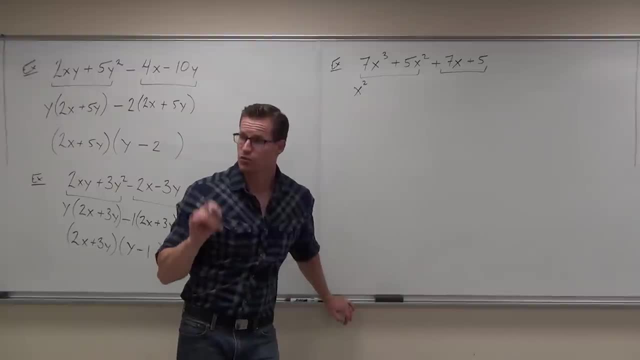 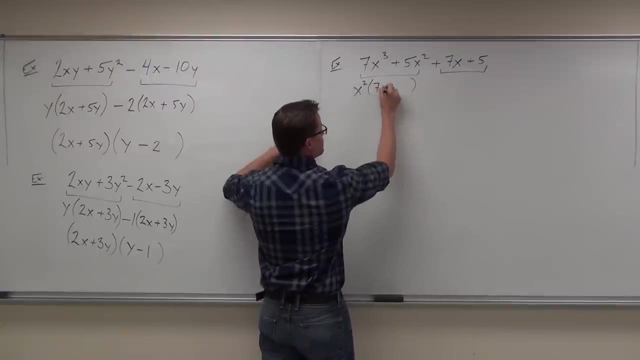 You have to do the greatest common factor, Not just x, but you have to do the greatest common factor. It's important for you guys to see that. So if we factor out that x squared, we actually get a 7x by division. x cubed, divided by x squared is x. 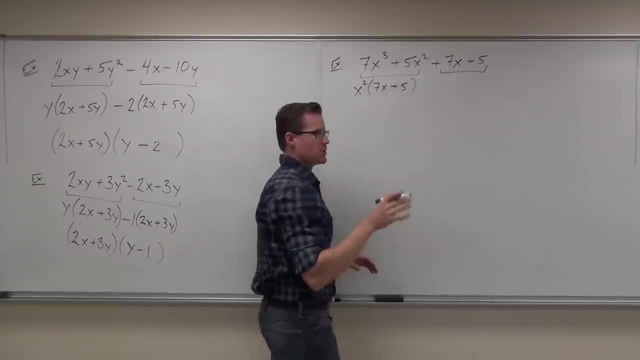 plus 5x squared, divided by x squared, is 5.. If you don't do that, it's going to look like these things are different. Okay, You've got to have the GCF Now. next one: This is one of those cases where only one goes into 7x and 5.. 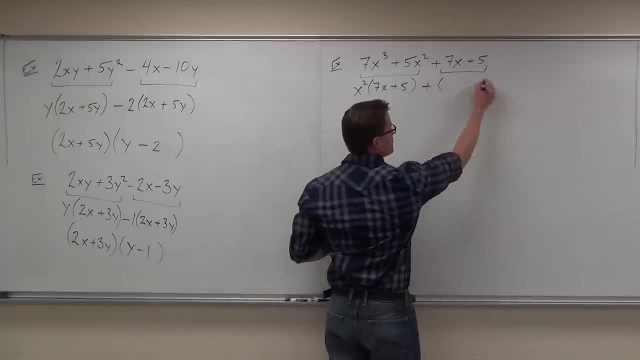 So at this point you can put plus and just put parentheses there, 7x plus 5, if you want to, Because only one goes into it. If that looks fine, you can put plus. If that looks fine to you, do that. 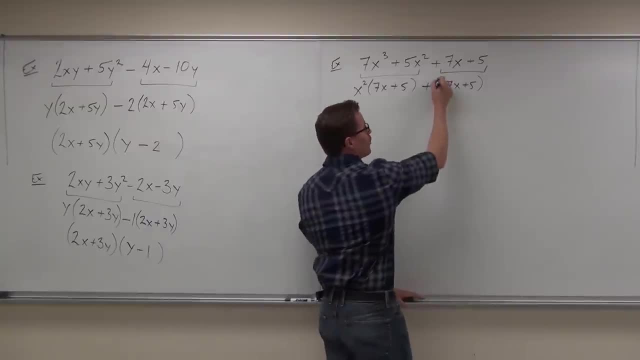 If you think, if you want to do like I do, if you go, well, I want the 1 there. that way, when I factor this, it reminds me that I have an x squared, oh, and I have a plus 1,. 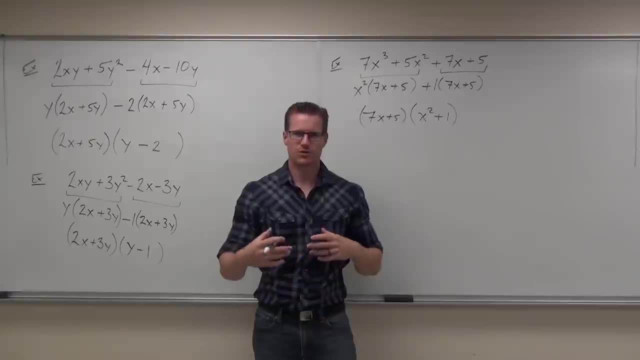 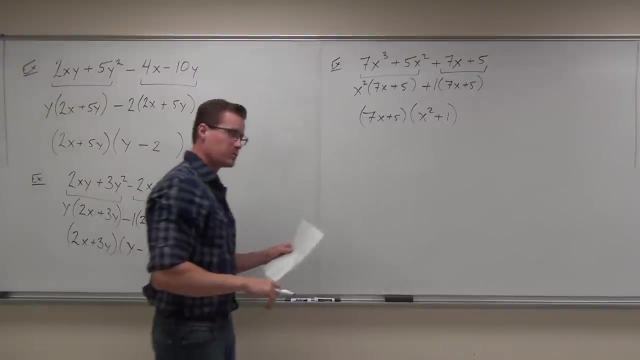 and I don't lose any of those factors. Have I explained this well enough for you all to understand it? Okay, cool, I'm going to give you two cases where this might throw you for a loop a little bit if you're not really careful. 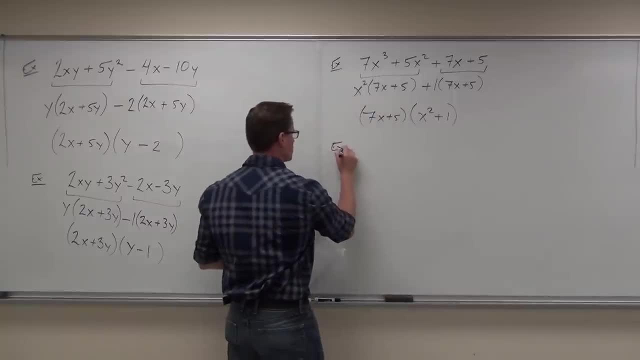 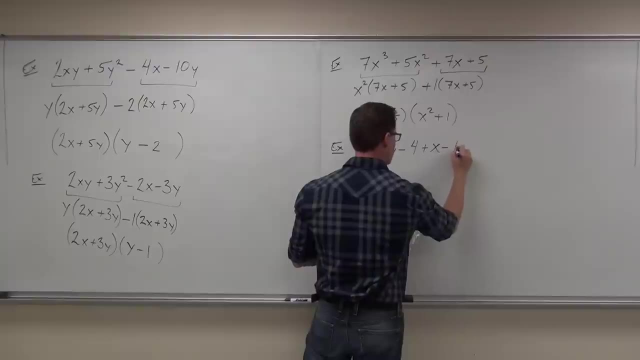 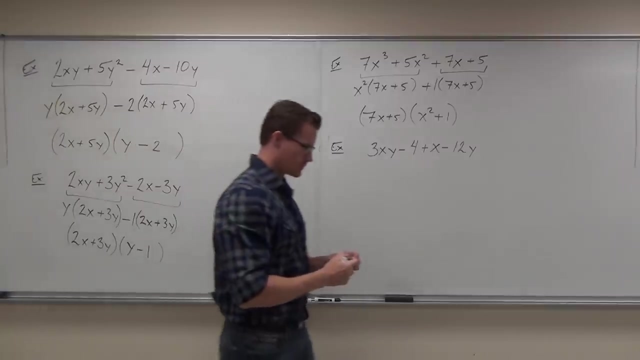 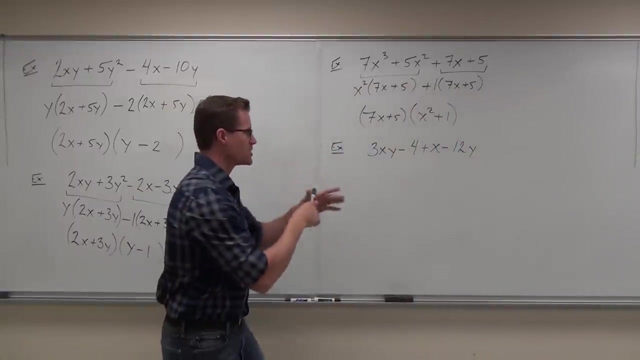 I'll show you how to deal with those. Okay, So first one. Okay, Real quick, though real quick. So how many terms? Four: Is there a GCF on these four terms? No, No, because some have x's and some have y's. some of them. 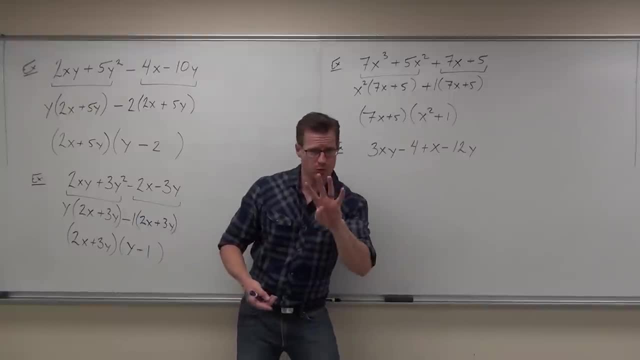 but nothing goes into all four of those terms. So if we have four terms and I'm asking you to factor, what do we need to use? Okay, So check this out. If we group this, what goes in these two terms? 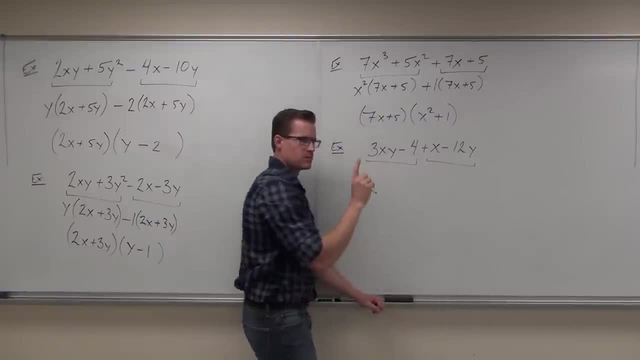 One: What goes in these two terms? One: Do you understand that if I factor out one from both sets of those terms, it's not going to do anything? Yeah, Yeah. So this is one of those cases where one way doesn't work but another way might. 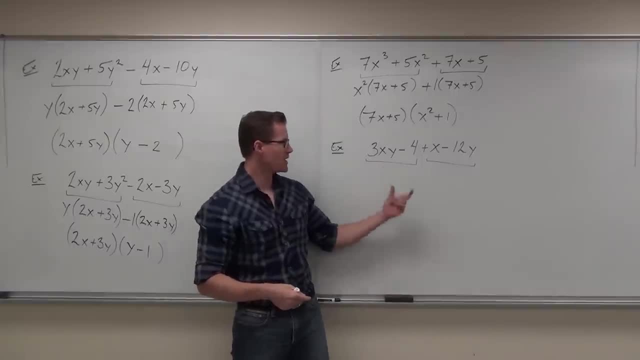 So if you run across this, you go: well, wait a minute, there's four terms. Nothing goes into those. Nothing goes into those two terms besides one. Nothing goes into those two terms besides one. This is one of those times where you'd want. 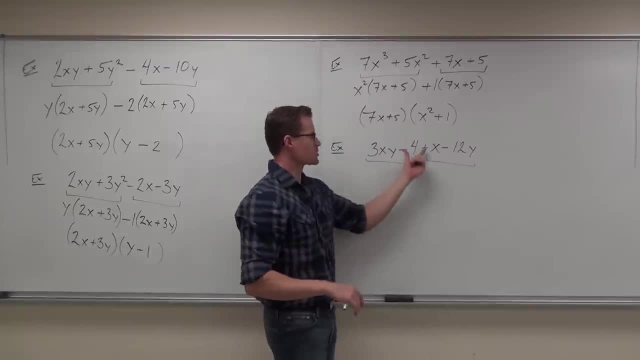 to try to reorganize it. So usually, usually it's just a matter of flipping those two inside terms. Sometimes it's a little more complicated, but usually it's just just remember this. Please remember this: Your terms have to go with the signs in front of them. 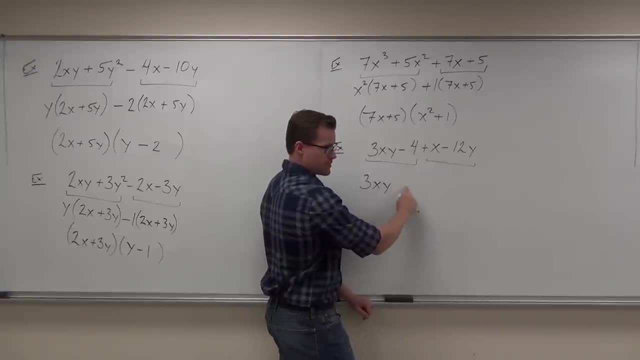 So if I'm going to interchange this, is it minus x or plus x, Minus x And then minus four and then minus, And then minus four and then minus x and then minus 12y, And by interchanging them sometimes we match. 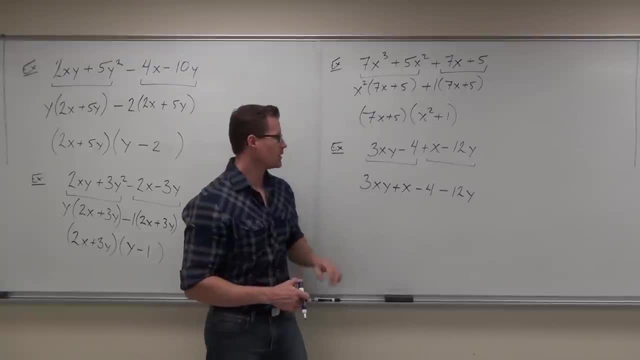 up factors better. I didn't see that. probably Do you see that nothing factors here And nothing factors here, right? Okay, If we interchange the terms: x goes here minus four goes here. sometimes we're going to cheat, not cheat. 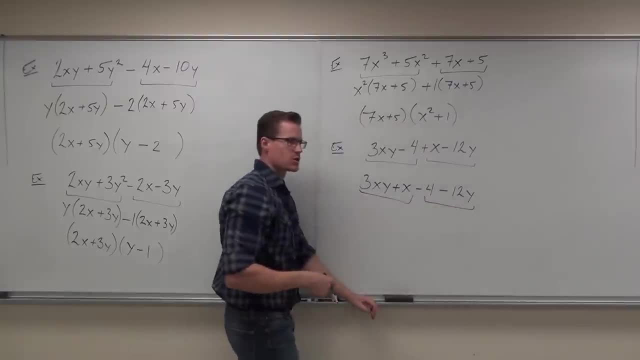 use this to our advantage, and then we get some terms that do have common factors. So let's look at it again. Do these two terms have a common factor? No, And if we factor out the x, we get 3y and we get plus 1.. 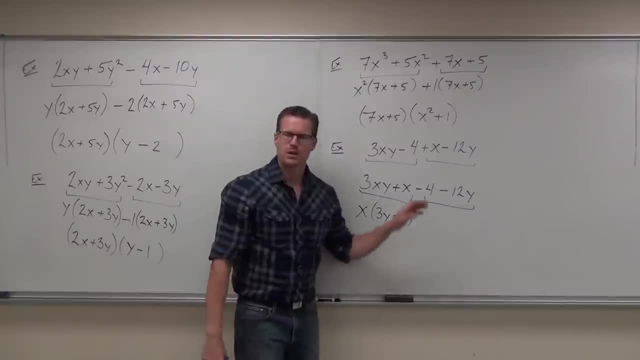 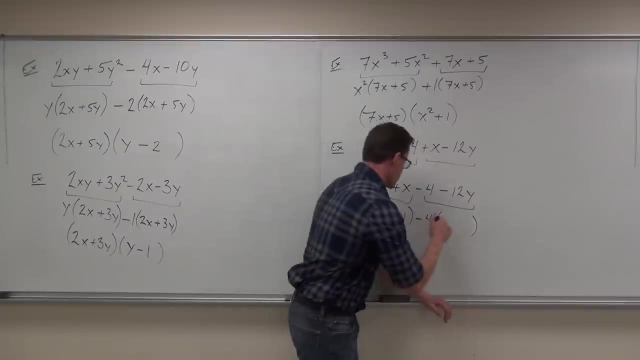 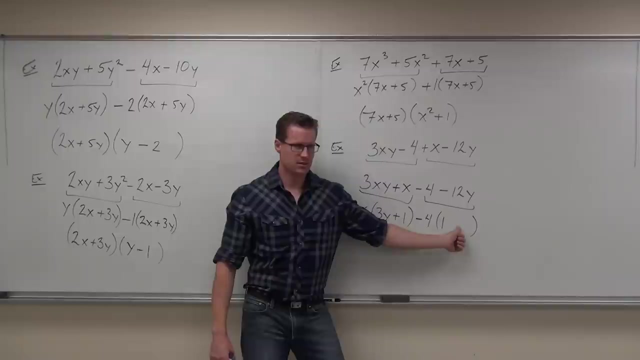 With me so far. Okay, Next up, when I factor out the four. when I factor out the four, the first term is going to be 1.. Next term, this one Y is going to be plus. That's good. 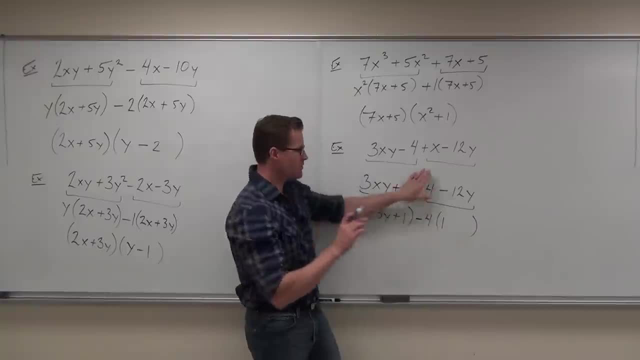 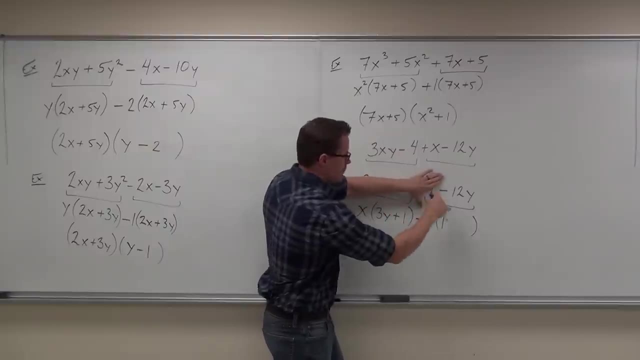 This is important for you to see. okay, If that's a minus, it means you're not just going to be factoring out four, you have to factor out negative four. Negative four divided by negative four is positive one. We think about it like negative 12.. 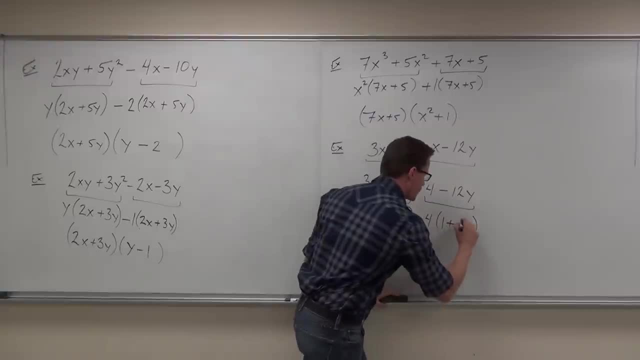 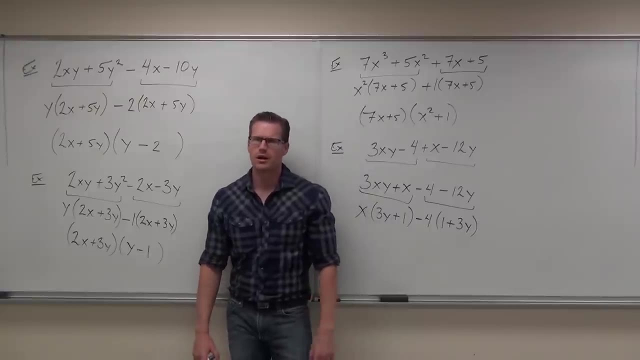 Negative 12y divided by negative four is positive, or plus 3y. Quick head note, if you're okay with it so far, Now next question: Do we have in these two large terms a common factor? Yes, Yes, Wait a minute. 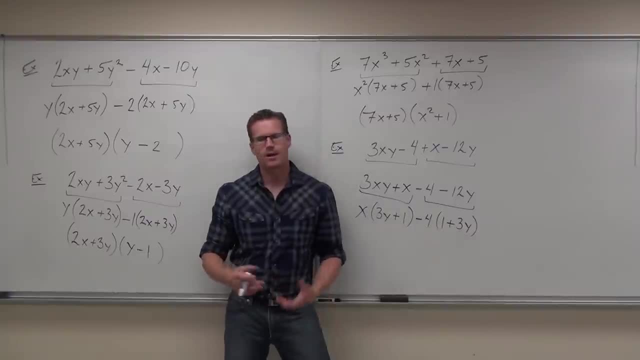 That's 3y plus 1.. That's 1 plus 3y. Wait a minute. Addition is commutative. Addition is commutative, Which means that we can switch them around and make no difference. So when you come across this, yeah, that's the same. 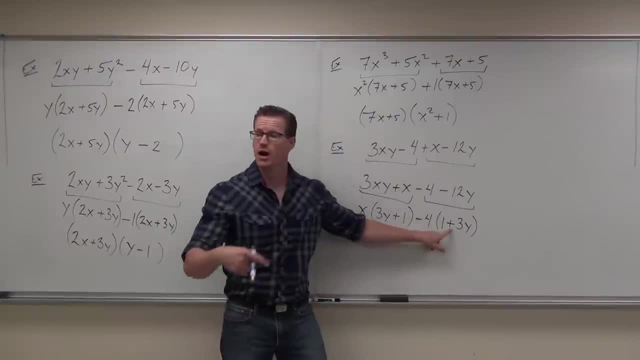 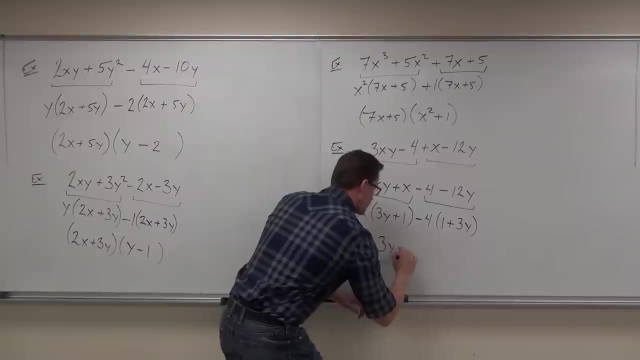 What if that was a minus? No, it would not be the same, because those are not commute subtractions, not commutative. So be careful on this. But yeah, you can switch those around with no problem. So we write our common factor first: 3y plus 1.. 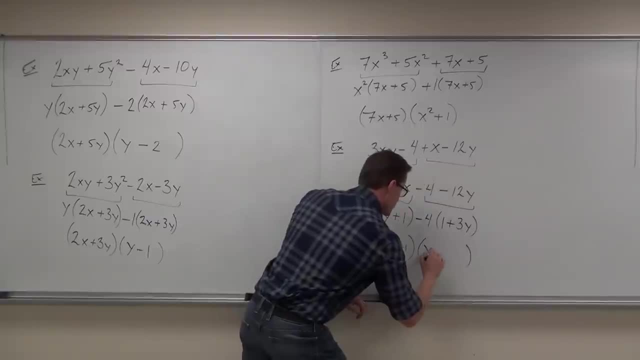 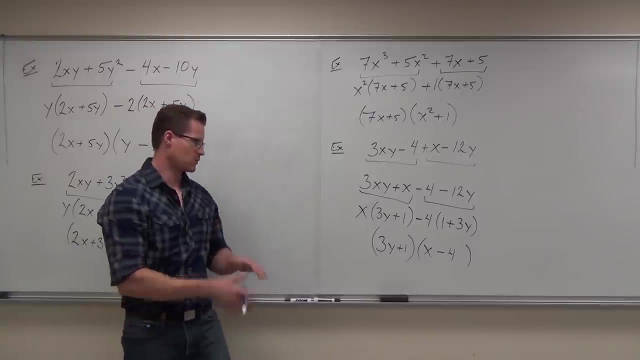 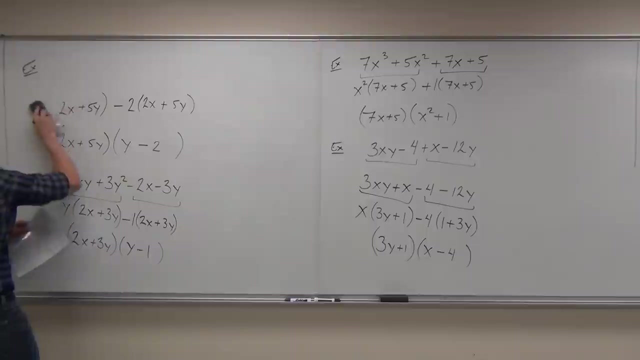 We're going to think about like 3y plus 1.. And then we create a new set of parentheses and factor out for our x minus 4.. So far, so good. on that one. Mm-hmm, Okay, cool, Okay, last one before we move on to a different technique here. 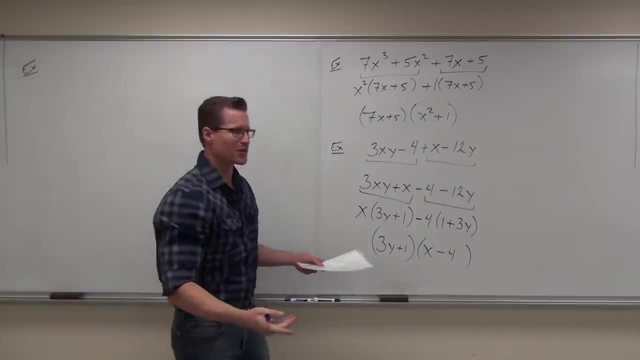 By the way, the reason why- if you haven't noticed, it's taken us a long time to go over this- The reason why we covered GCF to this extent and grouping to this extent, is because you use GCF for all factors. 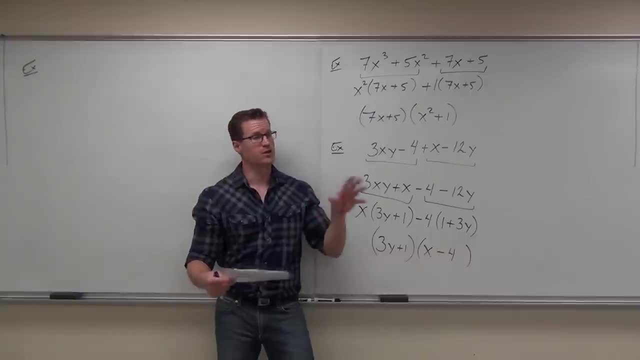 It's always going to be there. And then we also use factor by grouping in one of our techniques later on, And so we're always kind of relying on these two things. Question: You mentioned factor. Did you mention like terms earlier? Will we ever encounter like terms while factoring? 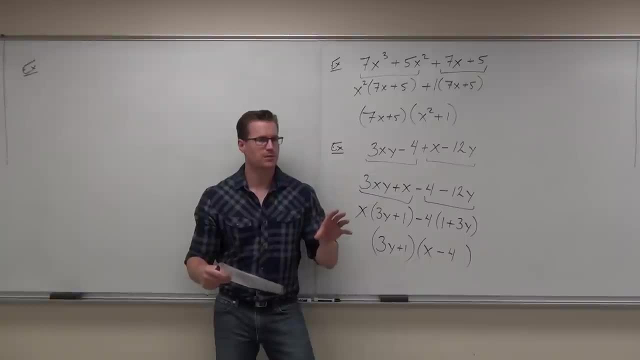 It's going to be assumed that when you get something to factor, it's already been combined like terms. So, like in our problems, we're always combining like terms first and then we factor. Okay, So yeah, you look for that. So when I say four terms, it's kind of implied that there are four non-like terms. 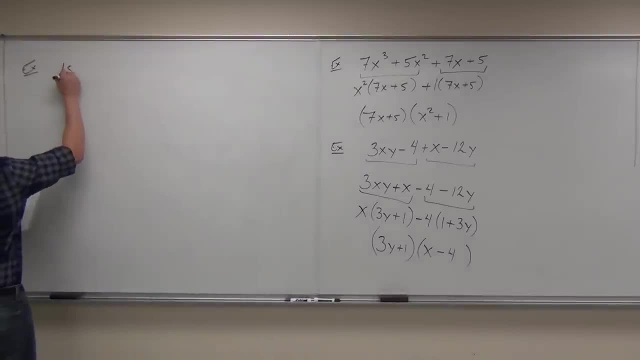 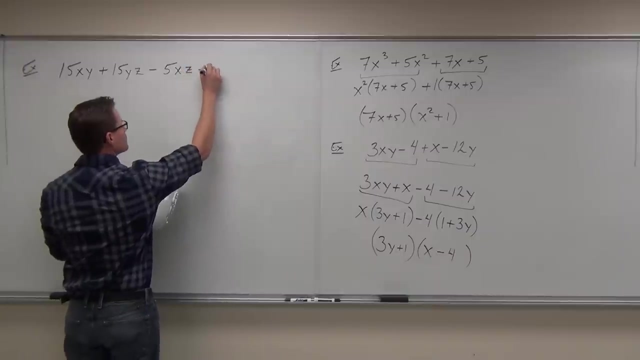 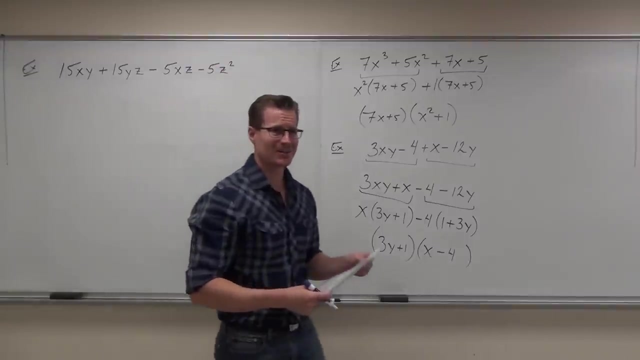 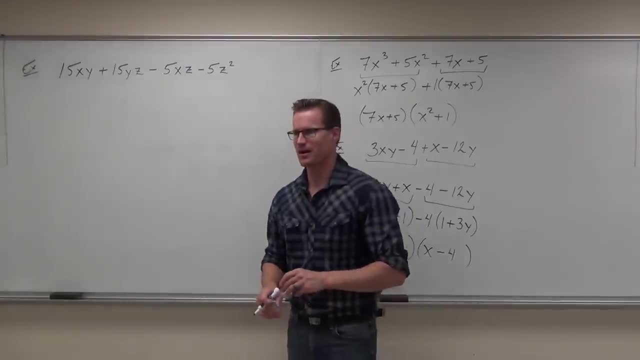 But you know, if I gave this to you in the first day of class and said, factor it, you might go. oh crap, I don't know how to do that one. Well, let's take a look at it. 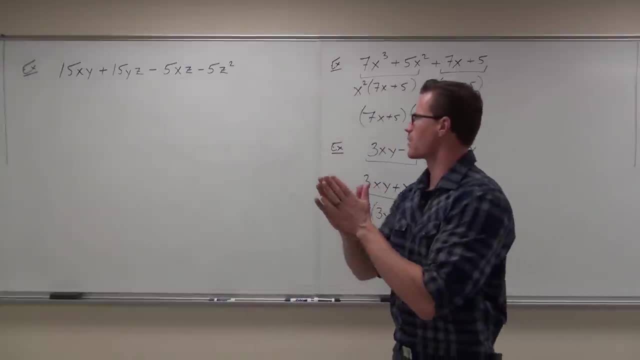 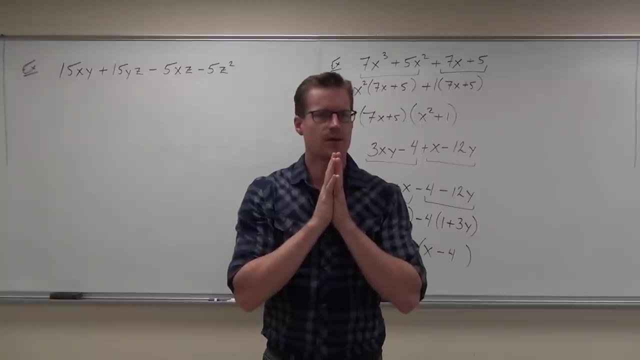 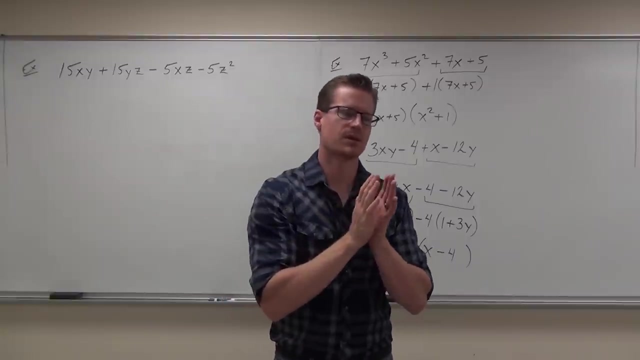 Let's take a look at this together. what is the first thing that you check for all the time, without fail, when I ask you to factor anything? GCF. how many terms are there? does this have a GCF with it? please do that first. factor the GCF first. and here's listen, I'm not. 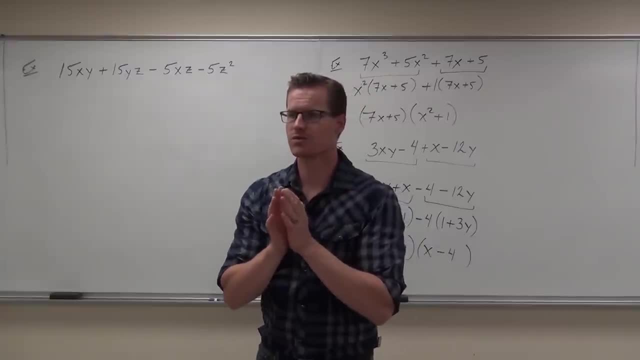 going to show you the other way because, frankly, I don't have the time to show you a mistake. okay, but here's the mistake. the mistake would be, and I know you're also working on it right now, but just focus on this for a second, okay, a. 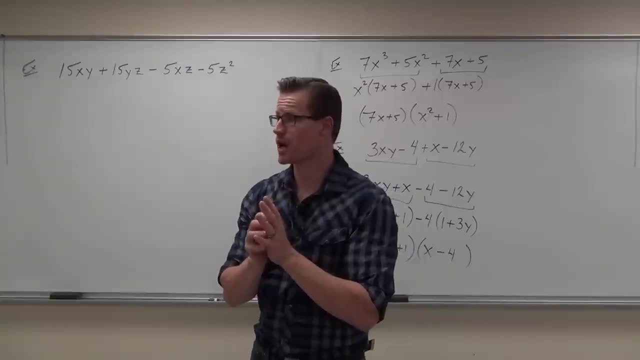 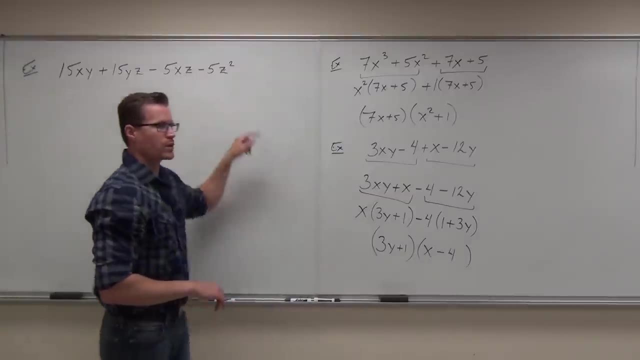 lot of people will skip this on a test and cause themselves more time. stick the right answer, but a lot of people won't take the time to do it. yeah, here's what would happen if you factored by grouping right now. what's going to happen is that, within one of those factors you're still going to have 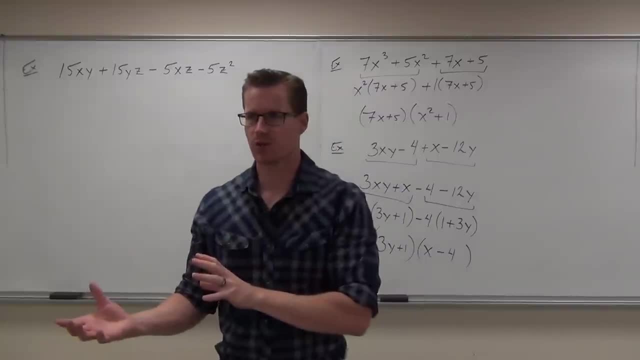 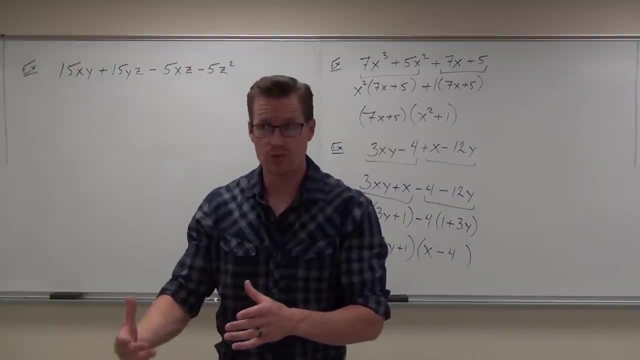 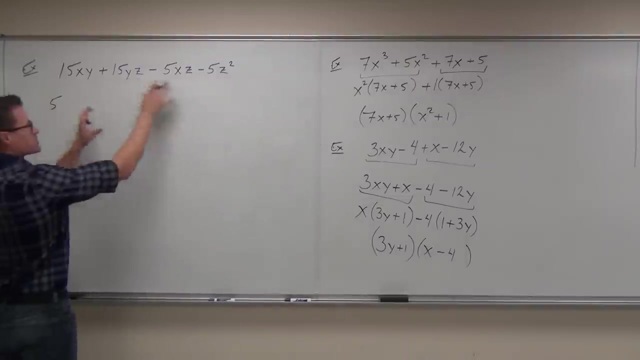 a common factor which you need to take out later. so take out the GCF now and it saves you time later. it saves you a mistake potentially later make sense. we're always doing the GCF first. what is the greatest common factor in this example? so if we factored five, not only does it make all these terms smaller, but 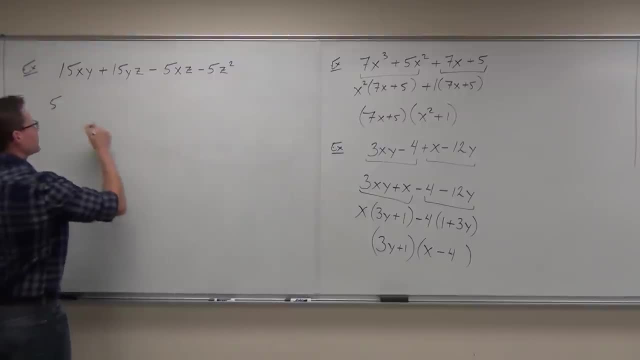 it allowed. it makes it so that you can do it faster, and you can do it faster, that later on we won't have to refactor again. we don't know. so what I'm going to do is I'm going to make up some brackets, brackets. I'm going to factor out the five. 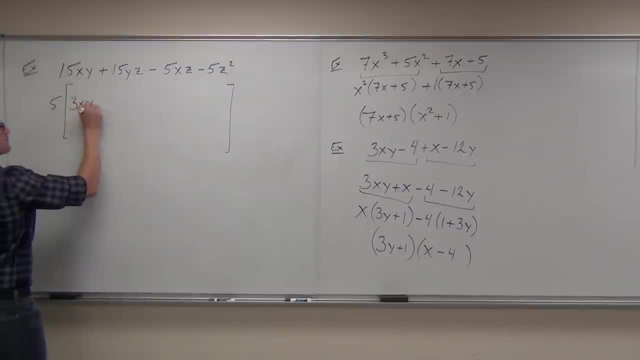 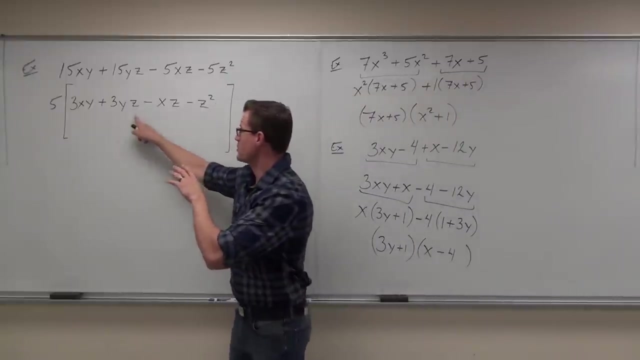 so basically just divided by five. I want to know if you're okay with that. so far, okay. next up, is it true that this has no greatest common factor, so we can't have another greatest common factor? but we've done that. how many terms do we have? still, four: factor never destroys terms, so now we can go ahead. 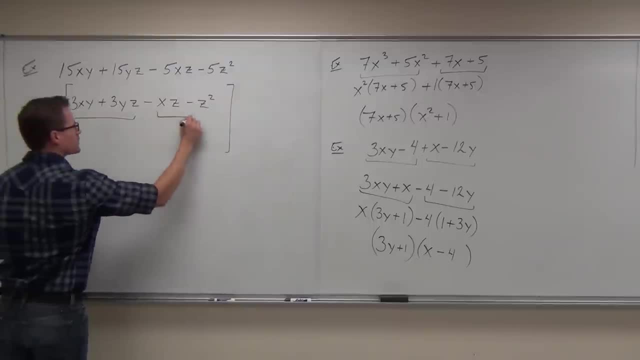 and do our factoring by grouping. so we look here and we look here: just keep that five floating out front, don't, don't lose it. but you really don't have to work with it right now. so if we factor, look at the first two. is there anything? 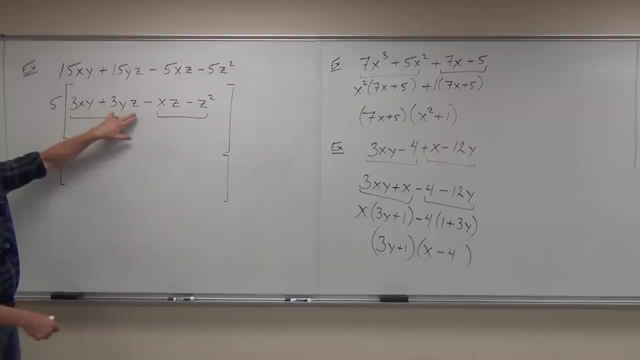 that goes into both three XY and three YZ. we're looking for the GCF for just these two terms, because we're grouping right now three pi and if we factor out the three Y and then we're divided by three Y, what's remaining for this term? say what: X plus, X plus, and yeah, look in the three Y, we're. 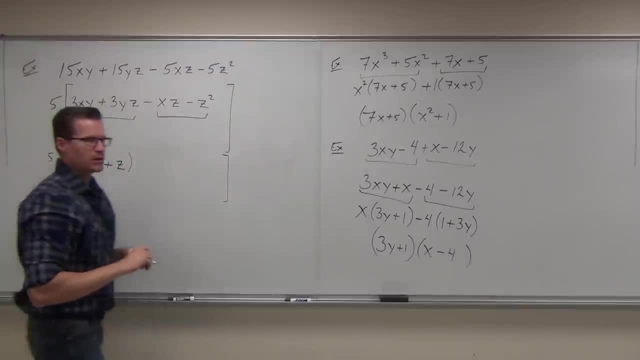 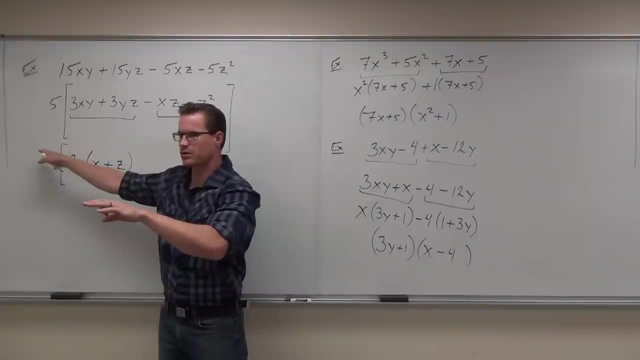 factoring that away, what is it perfect? can you verify that for me real quick, people, that we we factored three Y, we get X plus Z. yes, no, yeah, we've already take care of the five, so we don't worry about that now. next one is there. 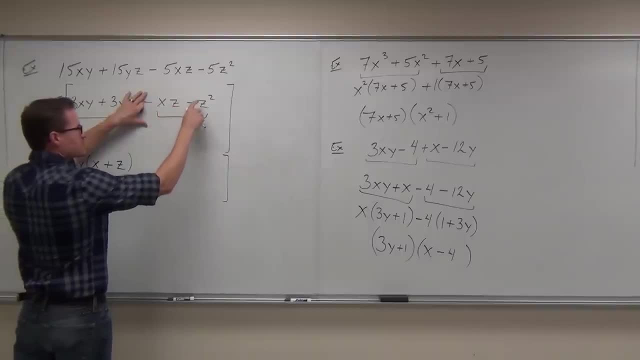 anything that goes into both X Z and X Z and minus z, squared Z, negative z. Okay, so that minus that really drops down for us and says, if you have z that goes into both these, it's forcing you to factor a negative z. 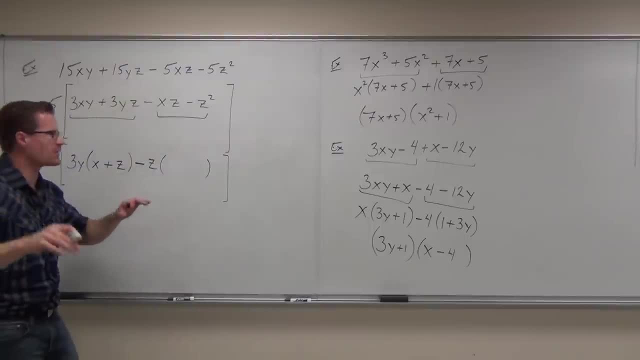 So we're forced to factor a negative z. Let's do that together, everybody together. What's gonna remain here after we factor out a negative z? Positive x? Oh, like I said, positive x, that's great. And somebody else who didn't speak just now. 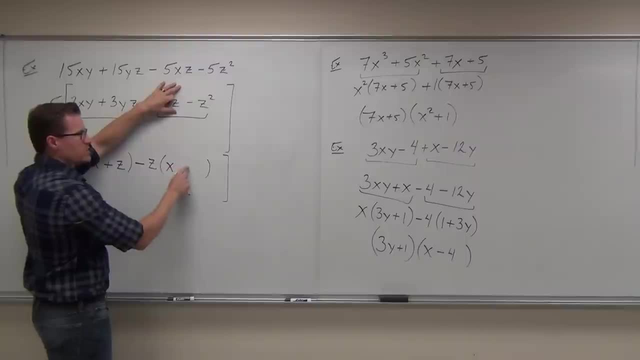 if we have a negative z and we're factoring out a minus z or a negative z, what goes here Z? Why does the sign change, please? Because you pulled out a negative. you factored with a negative. That's right. negative divided by negative is positive. 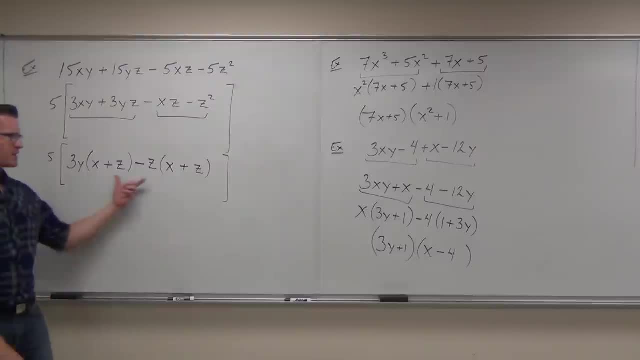 We're factoring out that negative. Did it work? Yes, Can you see that we made the right move here? This is great. We have two large terms, We've got a common factor. We're gonna keep the five, but it doesn't really do much. 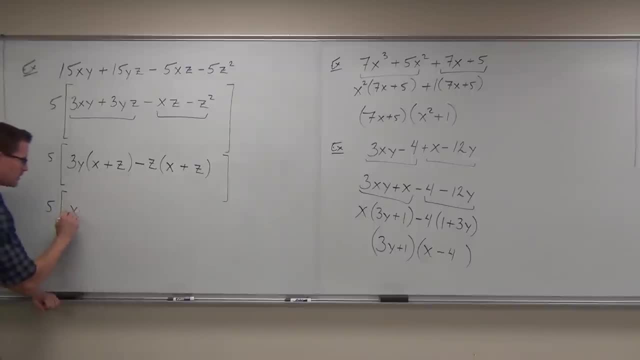 We'll put a bracket. We're gonna factor this x plus z and put it first. Factoring always creates another set of parentheses. If we factor away the x plus z, we get three y. If we factor away the x plus z, we get minus z. 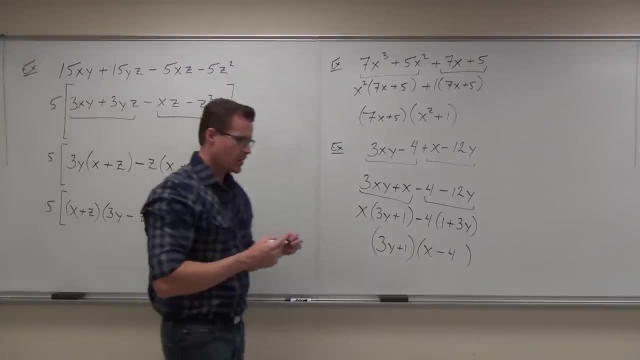 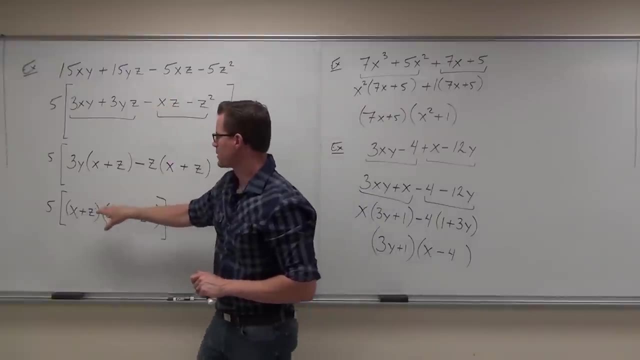 I need to show if Anza would feel okay with that one. Okay, what happens if you don't do? the GCF is down here. depending on which order these are in, one of these two large factors, like here or here, will still have a common factor. 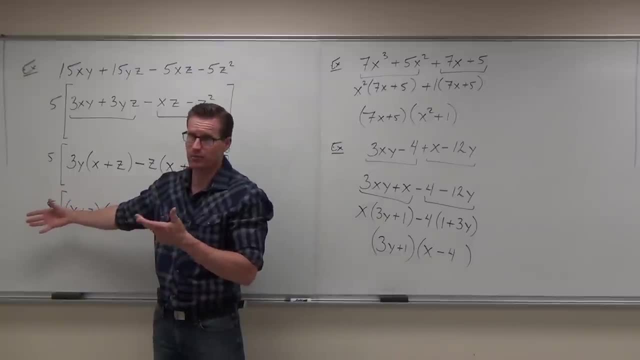 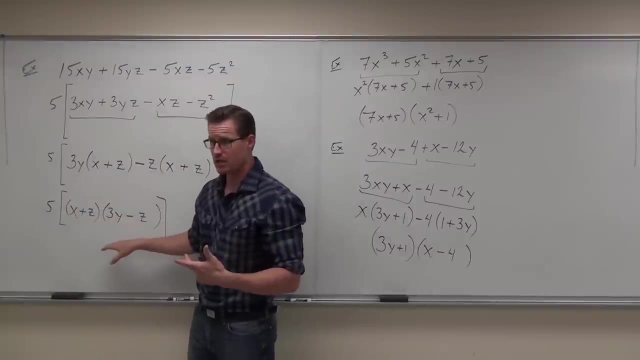 and you would have to factor that out anyway. Does that make sense? One, or maybe both in some cases, but taking care of the GCF first makes sure that when you get down to this point you're actually done and you don't have to keep rechecking.